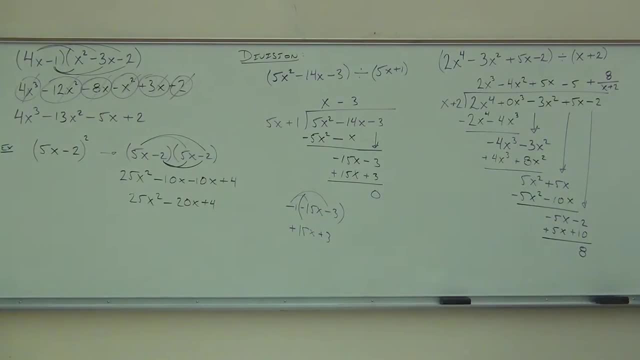 And Chapter 7 starts off with something called Rational Functions and Simplification. What in the world is a rational function? Firstly, what's the key word to rational? Yeah, that's exactly right, You guys are on the ball today. I drank extra coffee today, didn't y'all? 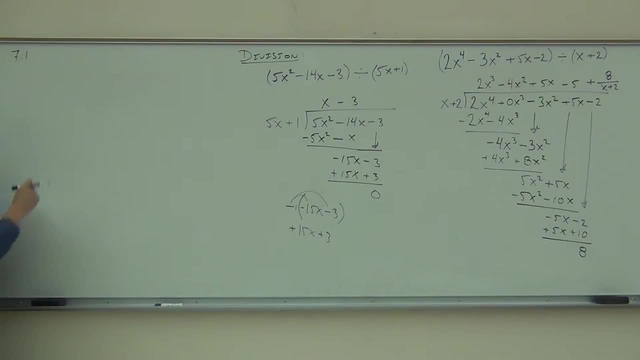 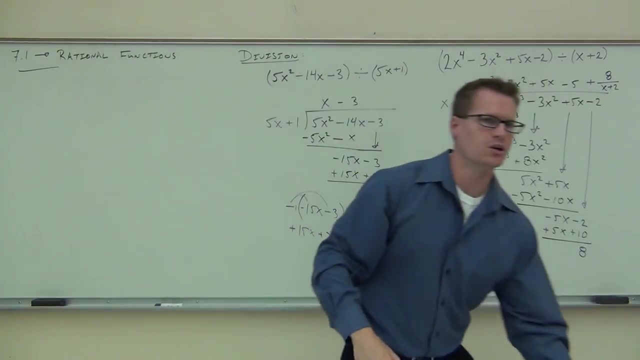 Me. neither Can you imagine if I did. Sometimes on the weekend I do drink coffee and then it's just off the wall. Rational functions. So some people have already said the key word in rational is ratio. Have you ever heard of a ratio? 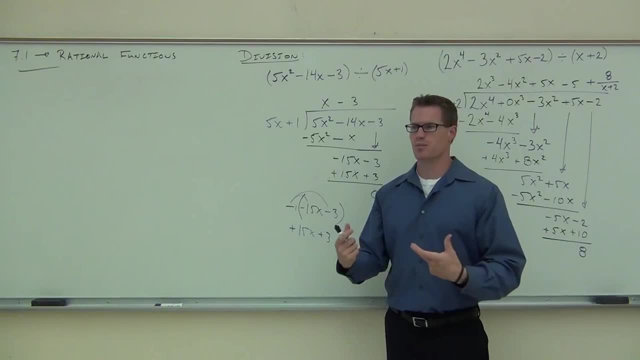 You made it into this class. What a ratio is is a comparison of two numbers or two quantities, or, in the simplest words, it's a fraction. So what we're going to be talking about in Chapter 7 for the whole thing is functions that are fractions, or fraction functions. 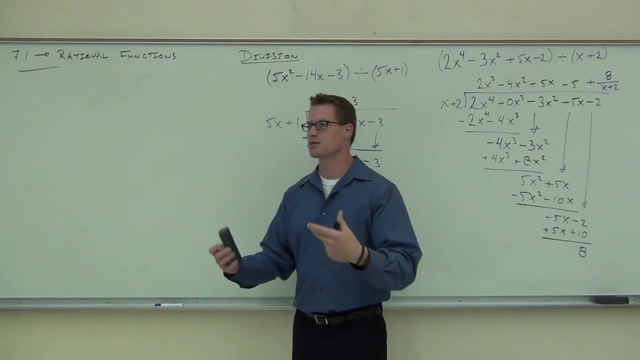 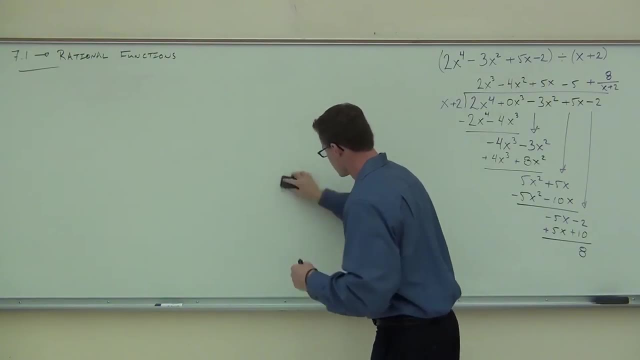 That's what we're talking about: These fractions that we're going to be able to look at and manipulate. Now, more specifically, they're not just fractions. They're fractions where the numerator. Does that word make sense to you? hopefully, That's the top or the bottom number. 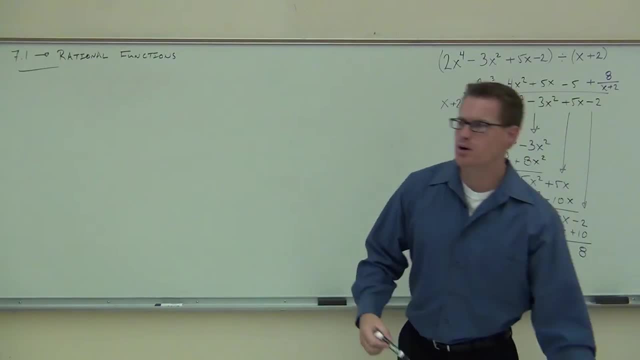 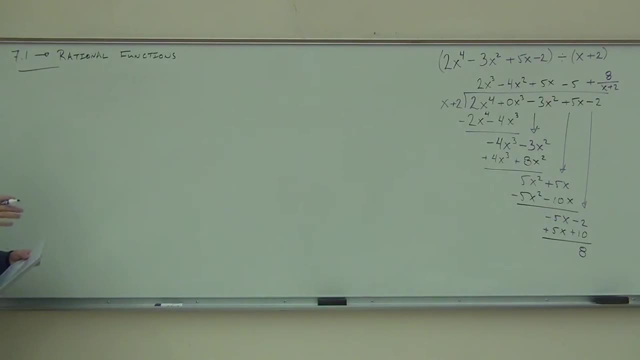 Or the top part of a fraction Where the numerator and the denominator are both polynomials- Those things we've been dealing with so far. So rational function is a fraction where both the numerator and denominator are polynomials. Rational functions: Both the numerator and denominator are polynomials. 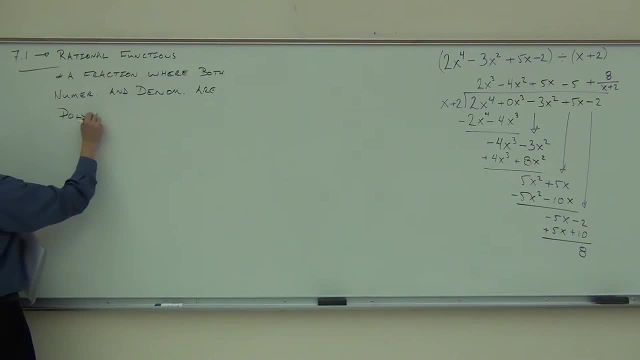 So something like p over q or p is a polynomial. Rational function r is the sum of the zeros. Rational function r is the sum of the zeros, where P is a polynomial and Q is a polynomial. Remember, a polynomial is just one term or more terms. 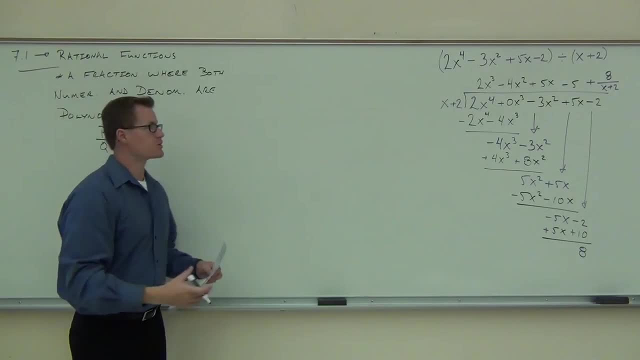 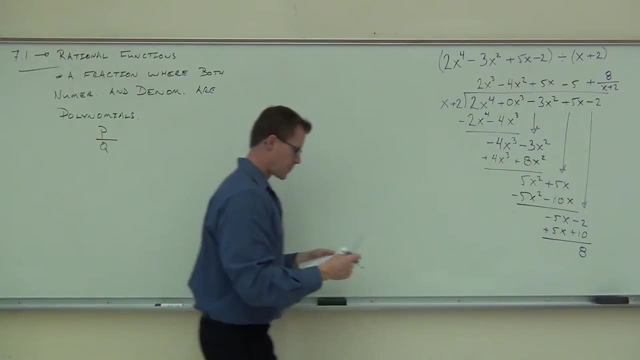 connected by some pluses and minuses. That's really all we're talking about. So this right here would be a rational function. if I put it in a different form, That would be just fine. First, let me start with some rational expressions. 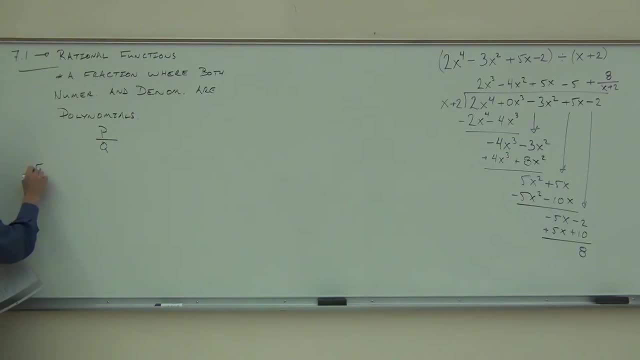 Here's some examples of what we're talking about. So, polynomial, Yes or no? what do you think? Sure, yeah, Polynomial Actually, yeah, it is. If you're a little confused with that, anything one or more terms. 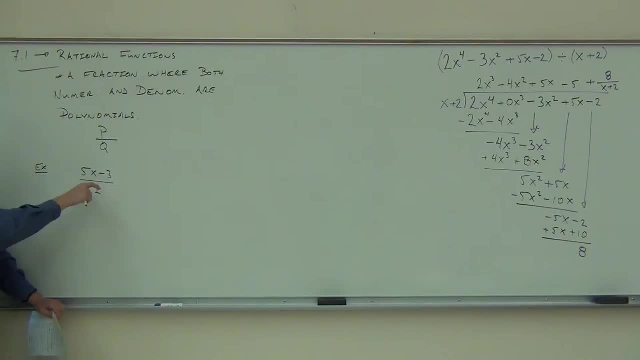 whether it has an X or not, can be considered a polynomial. This is the most simple polynomial you can have. It's just a constant. But this is a rational, what's called expression. We haven't got to rational functions yet. I'll show you what that is. 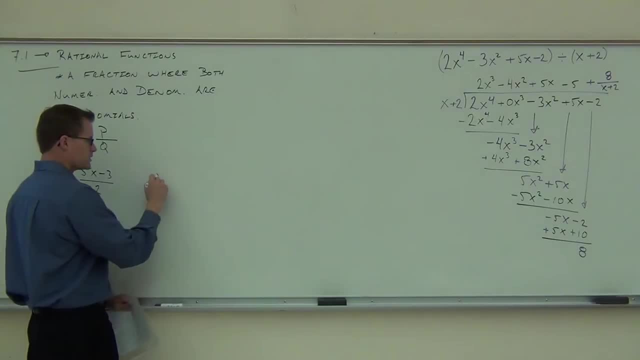 This is a rational expression. We can make it a little bit more complicated. We can do X squared minus 1 over X plus 1.. That looks more like your typical rational expression there, where you have a polynomial on the top and a polynomial on the bottom. 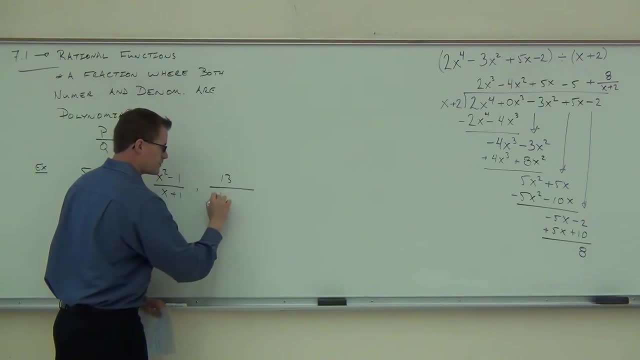 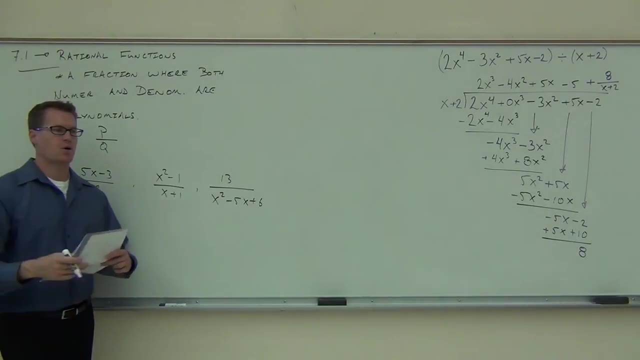 You can do it the other way too. You can have a constant on the top and something like X squared minus 5X plus 6.. It's also a rational expression Anything that has polynomials. so basically, what I'm saying is no square roots. 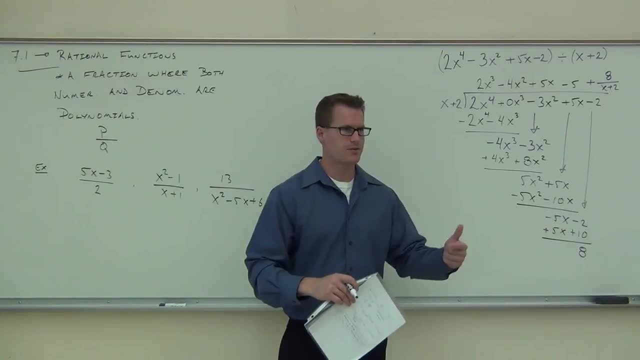 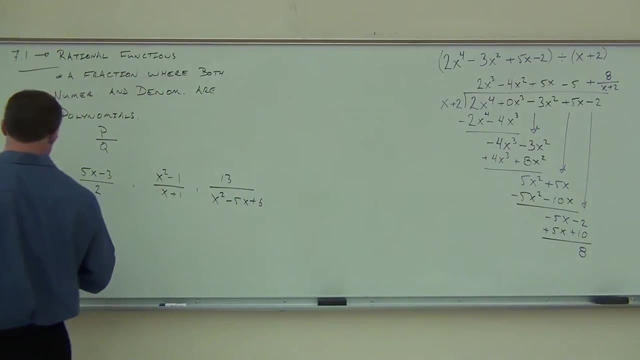 no fractional exponents. no, I's no weird stuff in there, and you have it in a fraction form. that's a rational expression In order to make this a function. have you ever seen this notation? Have you ever seen that before? 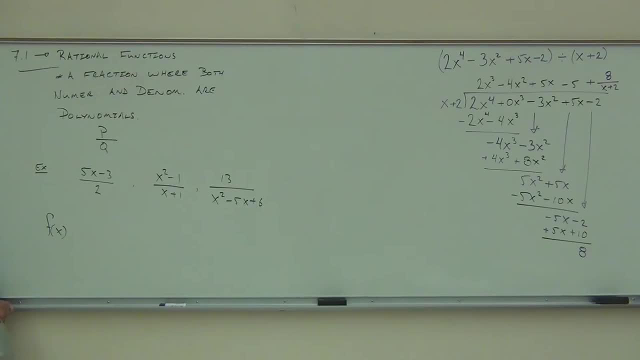 What's that mean? F of X is how you say it. It means a function whose variable is. That's what it is. So this says the following thing: is a function and the variable is X. Okey-dokey, That's what this notation means. 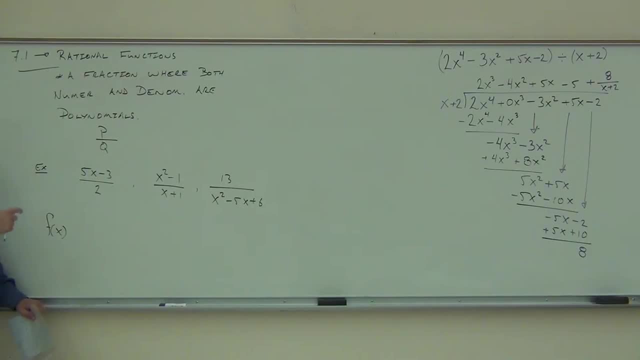 F is like the name of the function. You could have G there or H, It's just the name. Like you guys have a name, like my name is Brandon, This function's name is F. Okay, that's. it would suck to have a name like F, wouldn't it? 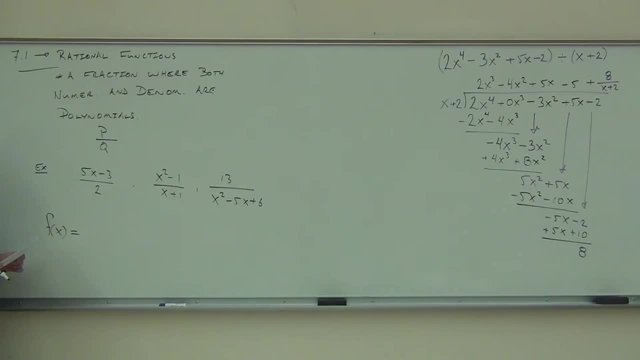 Well, at least if you were in school, that would suck to have a name like F. Anyway, this is a rational function. As soon as we have this function notation and then we follow it by a rational expression like X minus E over X cubed. 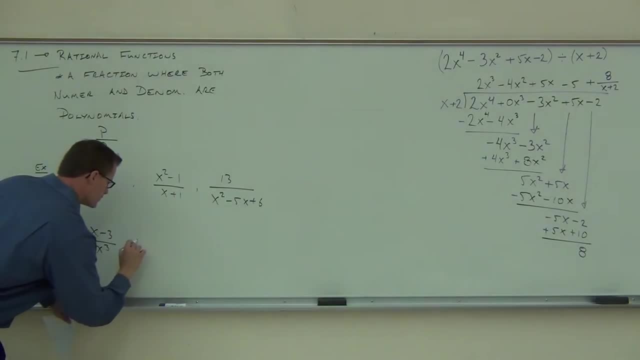 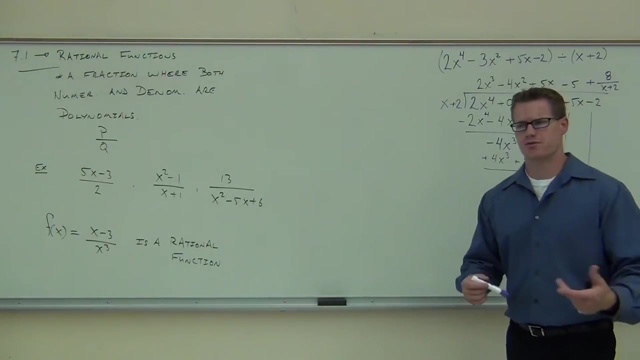 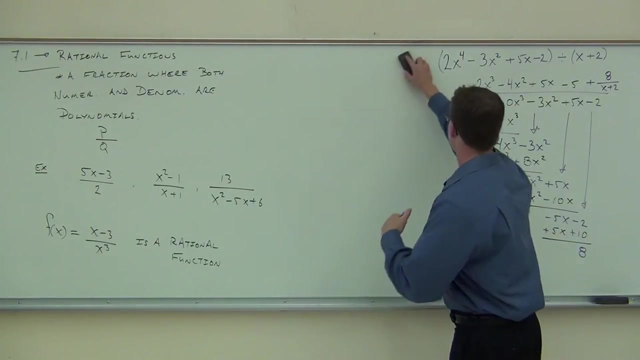 That's a rational function. Now, when you were first introduced fractions- actually before you were even introduced fractions, I know because I did this on Monday in my math dating class- Before you even talk about doing fractions, you learn one thing about them. 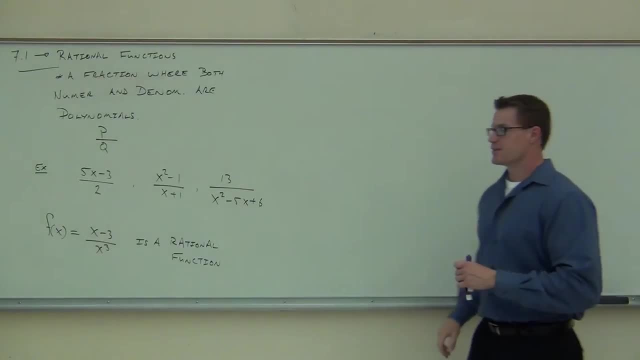 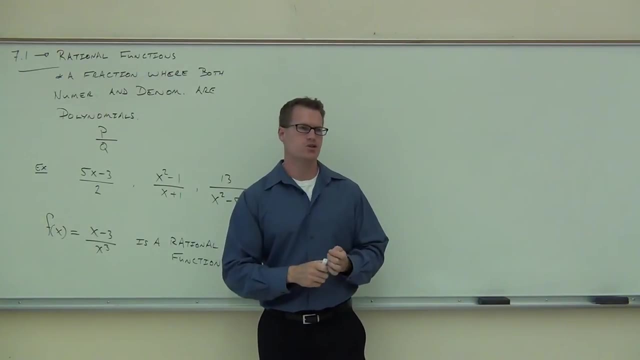 Specifically, you learn that if you have a fraction, there's one thing that you can never, ever, ever, ever do. Do you remember what's the one thing you can't ever do in fractions? It's not add them. You can add them. 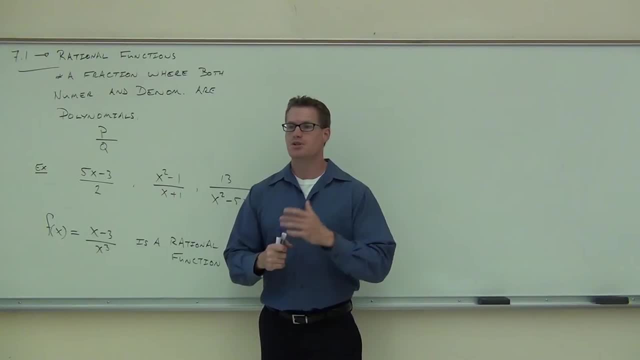 You can subtract them, You can multiply them, You can divide them. You can divide them, But you can't divide by this one specific number: Zero, Zero, Zero. Can you ever have a number over zero? Can you ever have a denominator of zero? 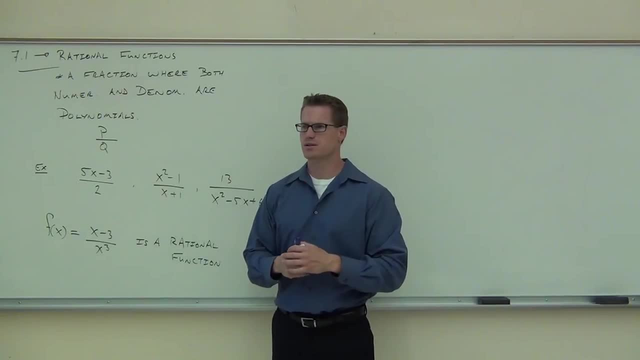 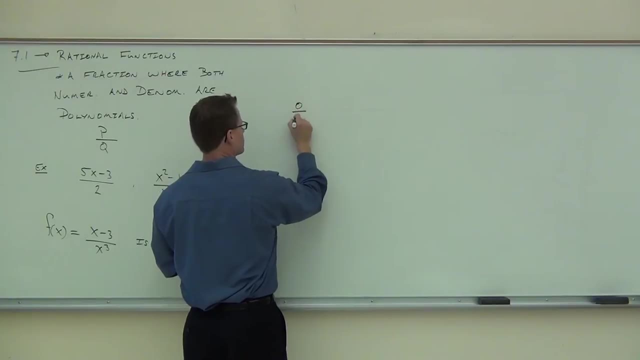 You call that undefined right, Because you can say: oh, divided by zero is like, it's like the difference between these two things. If you have zero divided by four, it's like you have zero dollars and you split it amongst four different bank accounts. 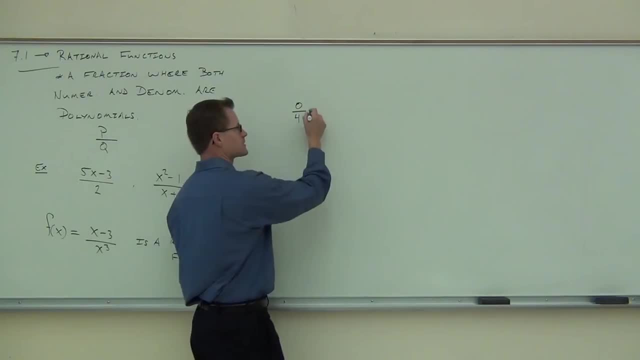 How much is going to be in each bank account? That's fine, That makes sense to even ask that, right? If I have no money across four bank accounts, I have no money in either any of them. That makes sense. But when you say this, I have four dollars. I want you to put it. 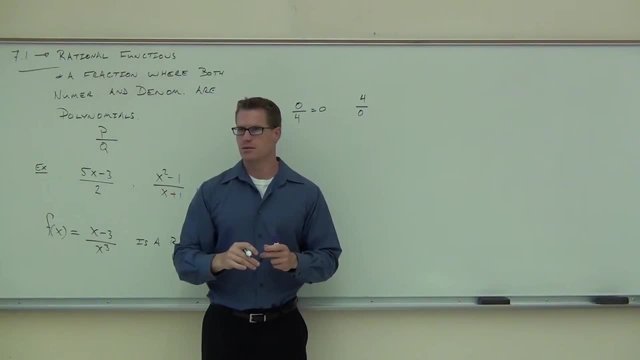 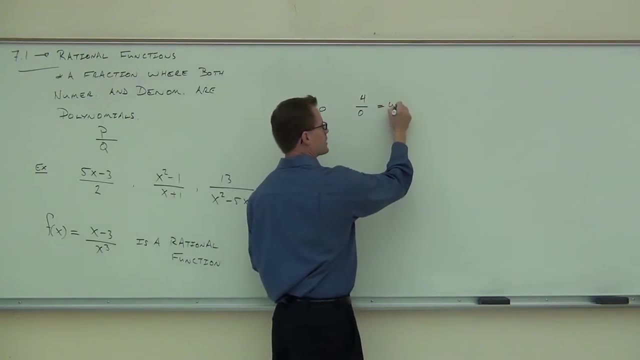 in zero bank accounts. How much money is in each bank account? Do you have a bank account? No, That doesn't make sense to ask how much money is in each one of them, does it? So this one is undefined. You can't even answer that question. 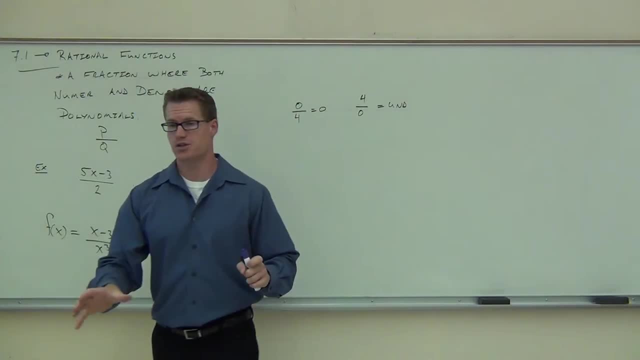 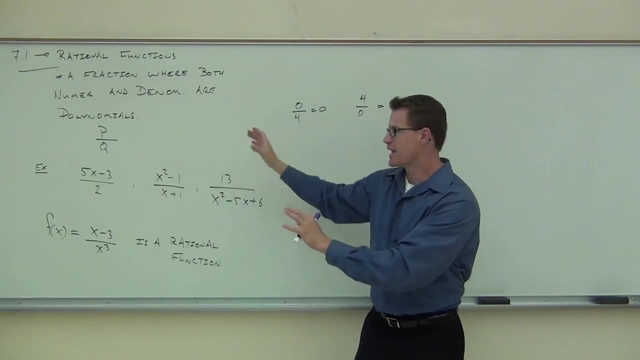 What this says to us is that, just like with any other fraction, you can never have zero on the denominator of your rational function. okay, Because it is a fraction, You can't ever have zero on the denominator. Let me write that out and we'll talk a little bit about that. 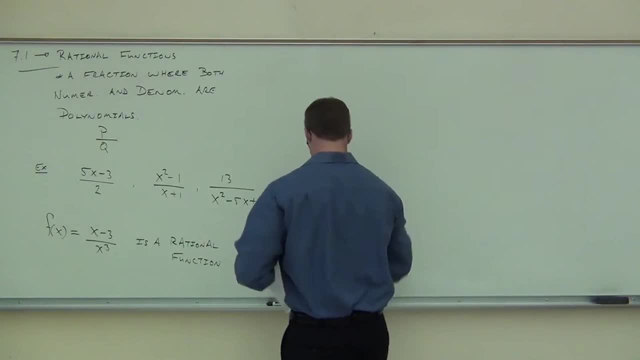 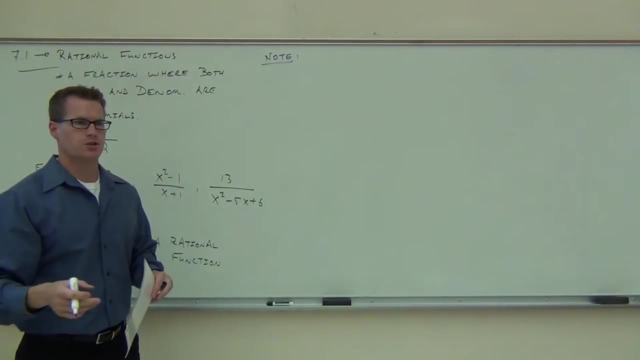 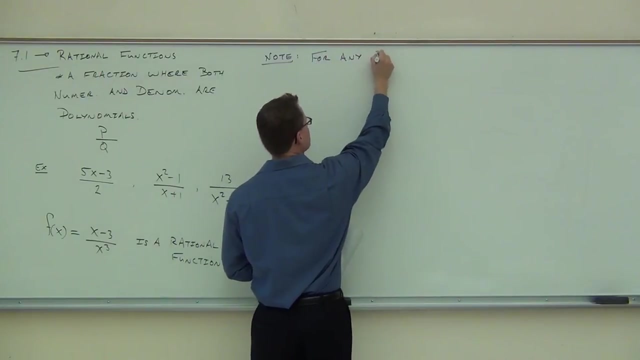 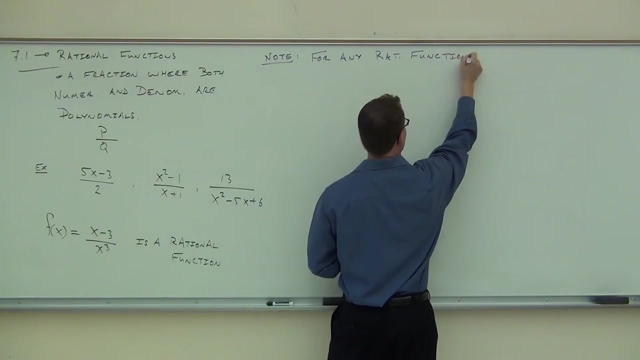 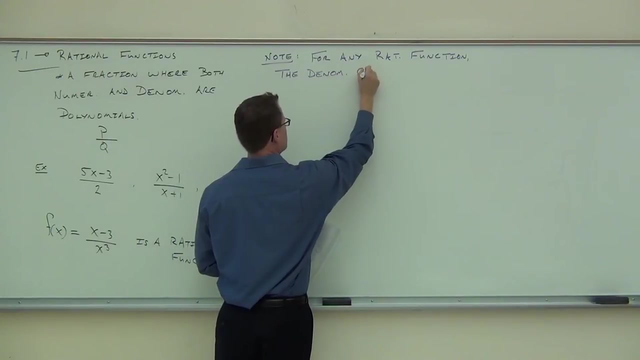 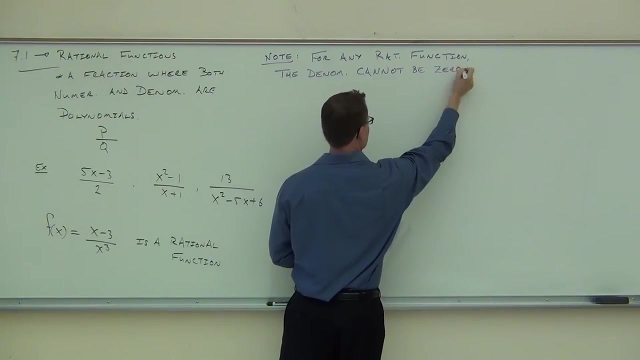 So a major note for us today: for any rational function, the denominator can never be zero. For any rational function, the denominator cannot be zero, Just like every other fraction you've ever seen in your life. You just can't have it, otherwise it's undefined. 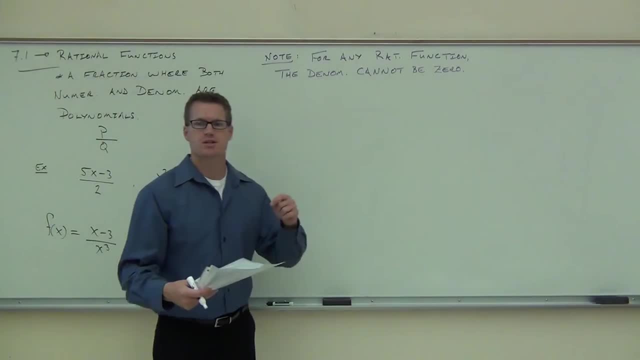 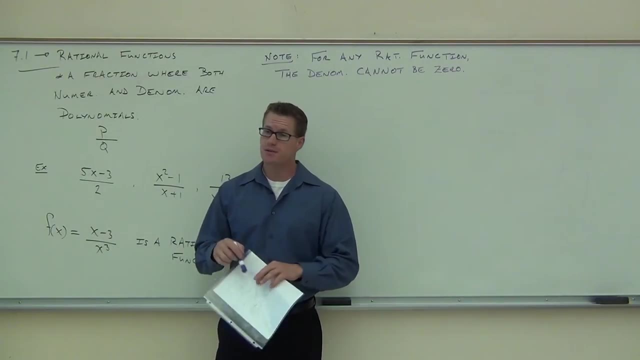 That's the next thing I'm going to write. If you do have a denominator that does equal zero at some point, look at, look. here's the difference between a rational function and a typical fraction. The difference is that sometimes the value 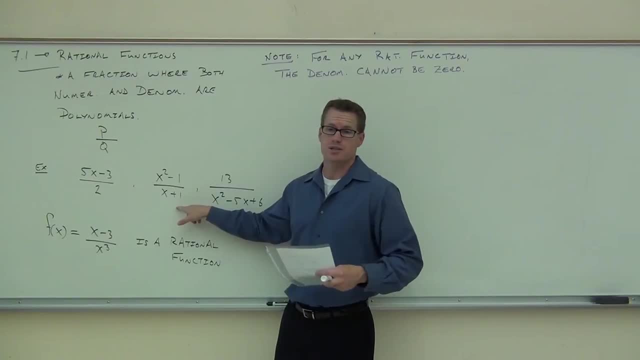 of your denominator can change. Are you with me on that? So it's not always going to be zero. It might be zero at only one point or two points or three points maybe, but it's not going to be zero everywhere. 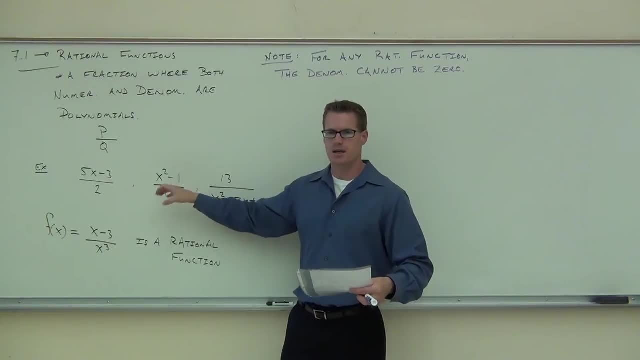 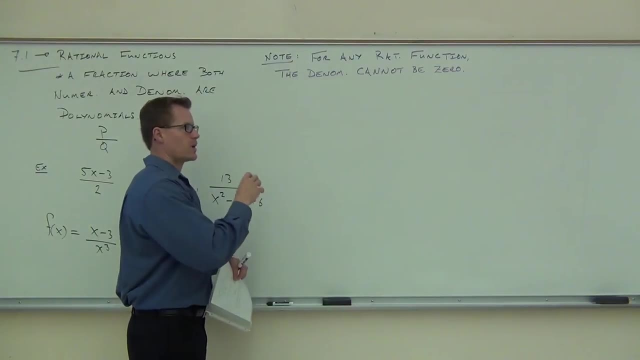 unless there's just a big fat zero down there, and then of course it will. But if it's not, then you might have some points where it's undefined. That's what I'm going to write now, If your rational function. I'm sorry. 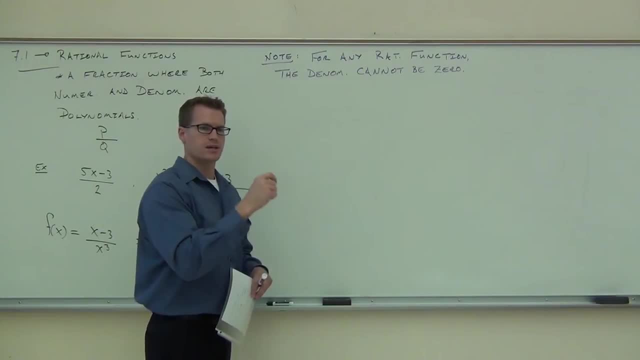 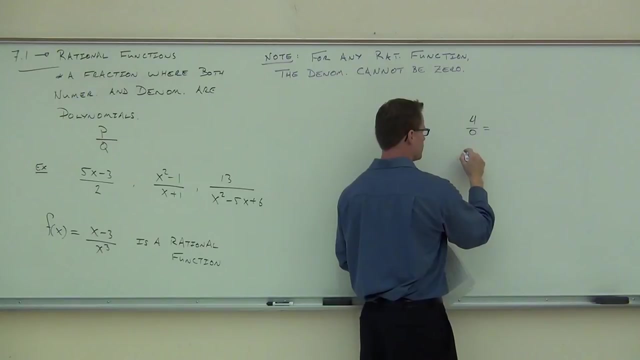 if your denominator does equal zero at some point, we say it is undefined. at that point, Do you see the difference between a regular fraction and a rational function, Rational functions, we don't just go undefined, We go it's going to be undefined at like one point. 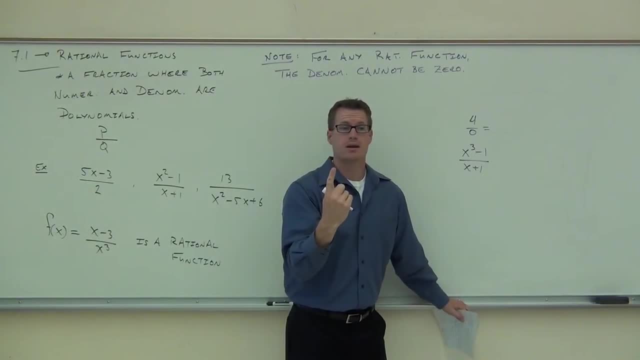 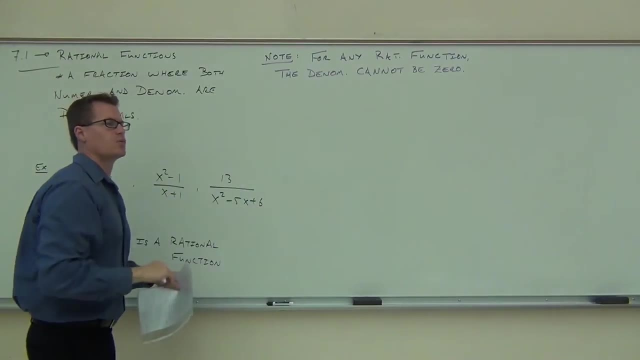 Not every point, just one point. You with me on this. I'll show you how to do that in just a second. So for any rational function, of course the denominator can't be zero, but if it is zero at some point, 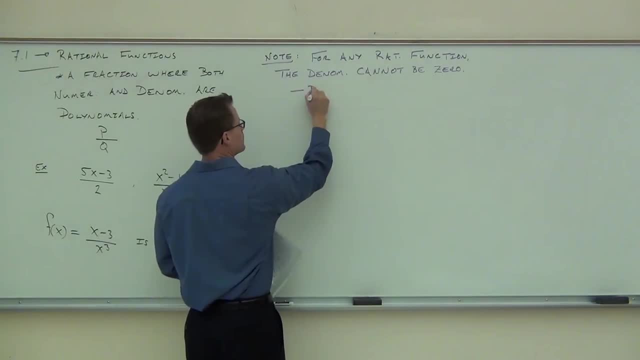 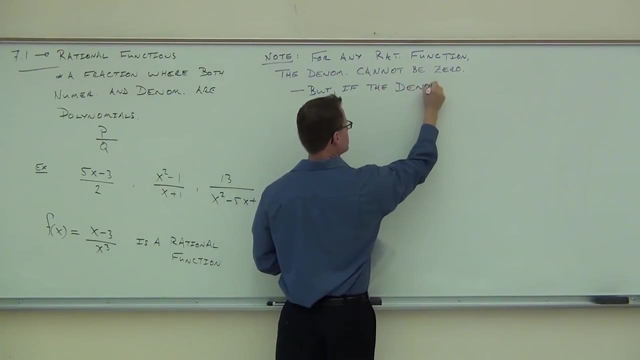 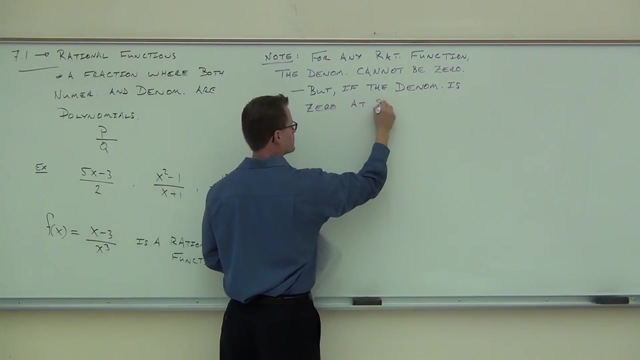 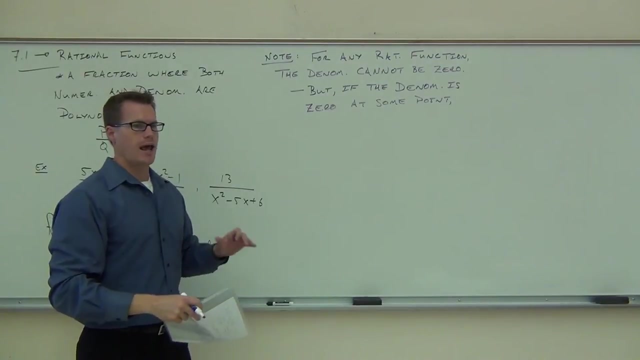 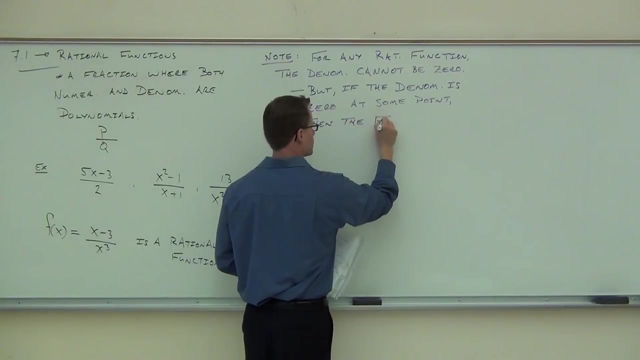 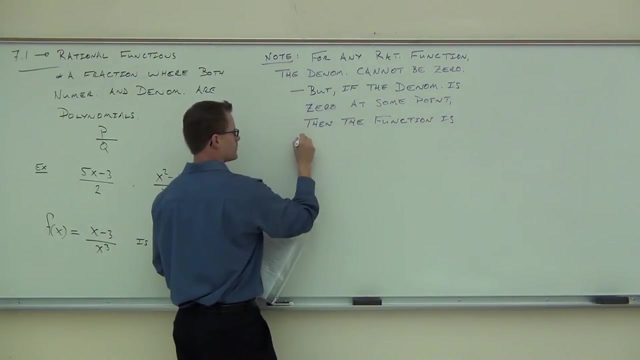 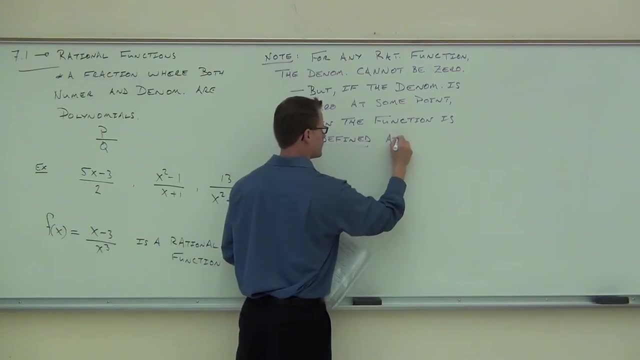 it's undefined at that point. But if the denominator is zero at some point, then the function is undefined at that point. I'm going to underline at that point a couple of times, so you know it's not at every point, it's just at that specific point. 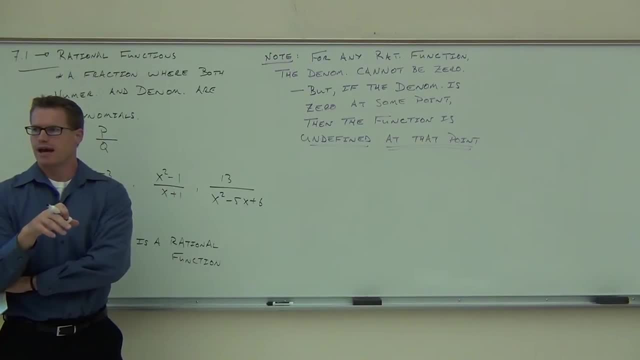 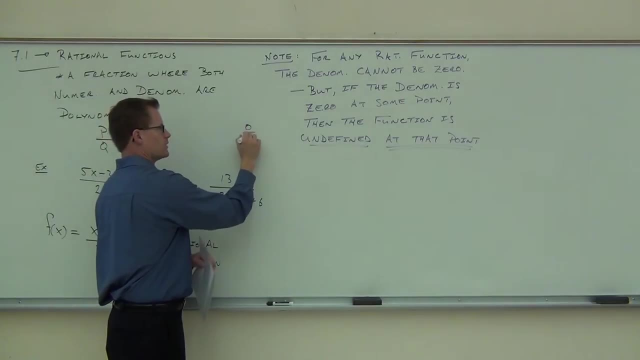 By the way, in fractions, is it okay to have the numerator equal to zero? Is that okay? No, Like the one I wrote earlier, is that okay? Yeah, Sure, that just equals how much Zero. By the way, anything, when you have zero over a number, it equals zero. 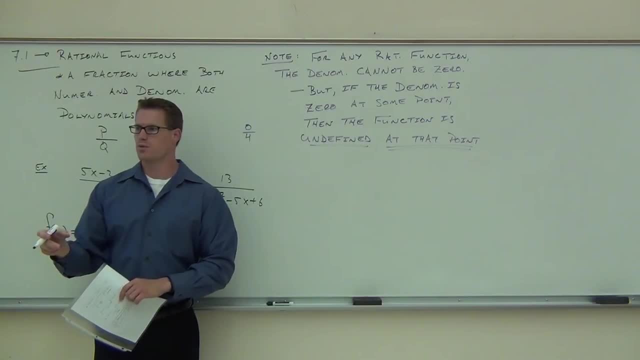 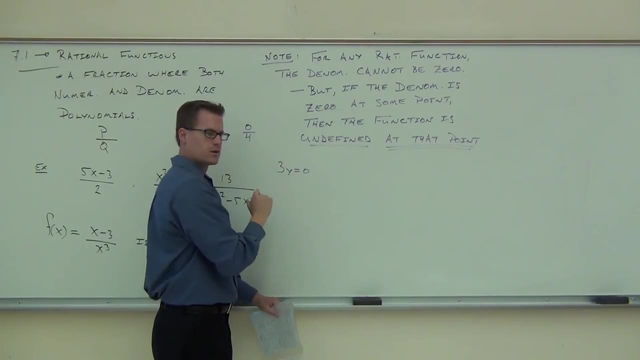 So some of you on it was one of the problems on your homework. you were solving it down. you had three y equals zero, like this: You remember that problem And you divide by three. some of you said there's no solution. 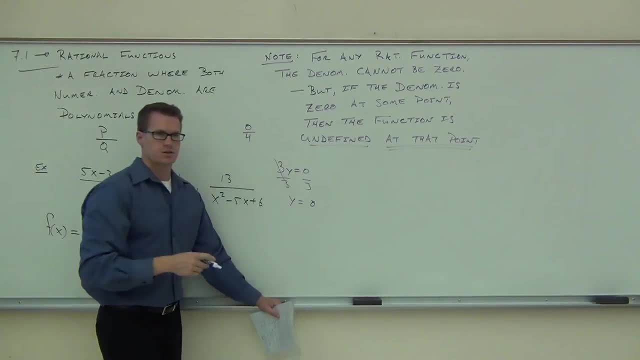 No, there is a solution. Zero divided by three is just zero, Okay. so when you get that again, don't leave it as zero over three. okay, it's actually just zero, So be aware of that. So, yeah, it's okay for a numerator to equal zero. 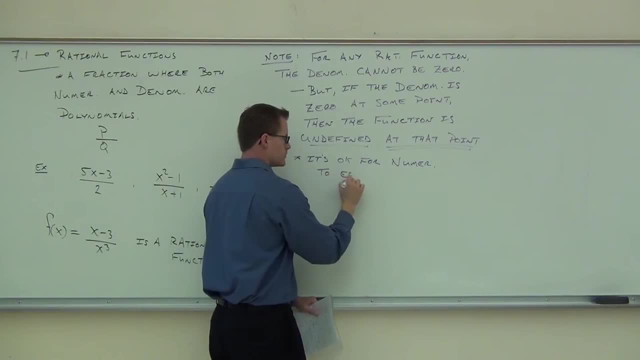 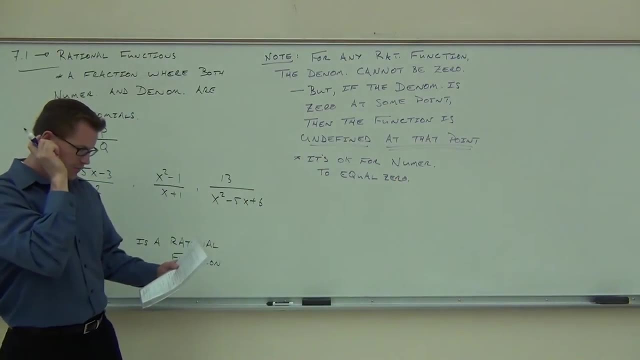 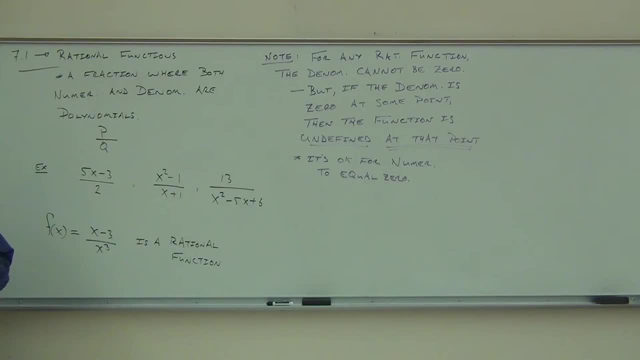 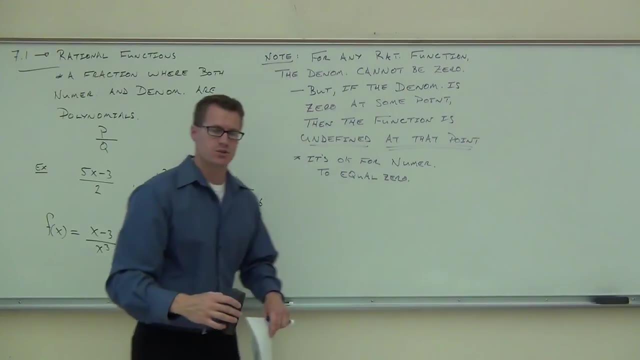 Did you get the idea here? Rational functions are basically just our fractions. we call them a function. that's it. There's two. there's one thing that cannot happen. One thing that can't happen is our denominators can't equal zero. 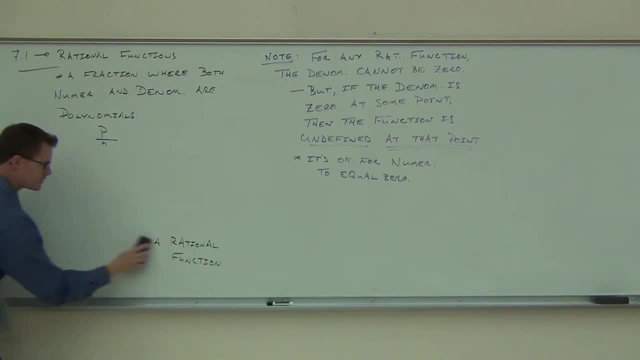 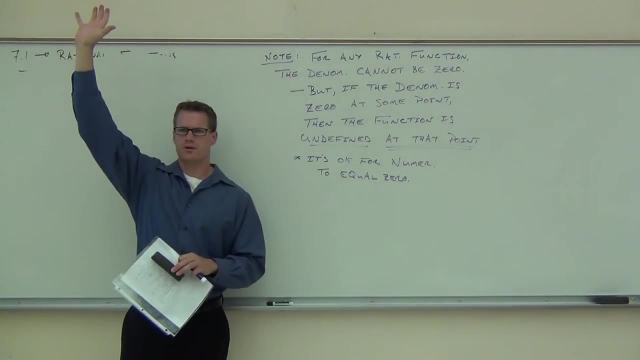 If they do at some point point we say it's undefined. at that point We're going to take a look right now at something that's called the domain. Raise your hand if you ever heard of the domain before. Raise your hand if you've forgotten what the domain is. That's fine. 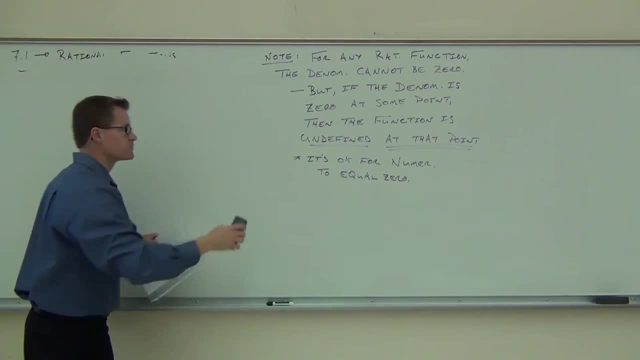 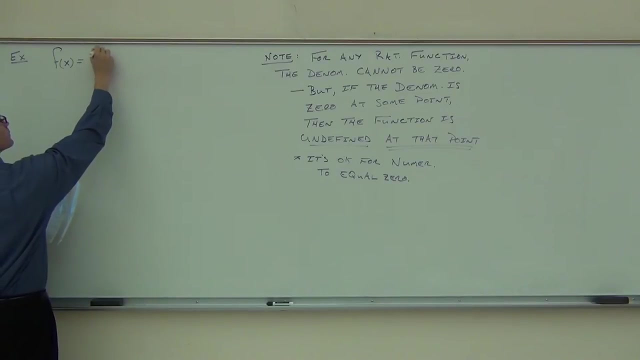 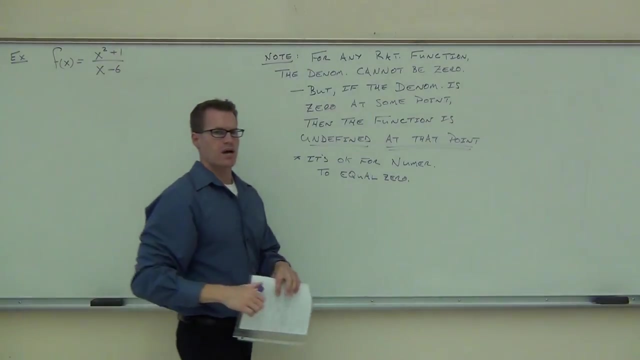 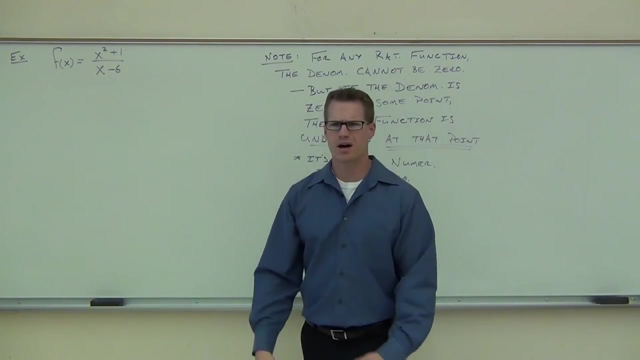 Okay, let's talk about domain. It's not a hard concept. I'll explain it to you in like two minutes. Would you say this is a rational expression or a rational function? Why would you say that's a rational function? Okay, and why not just a rational expression? What's making? 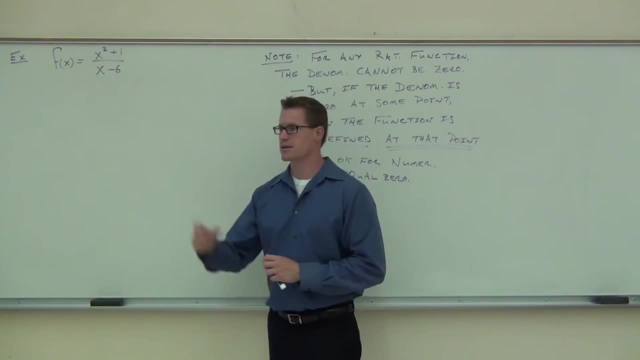 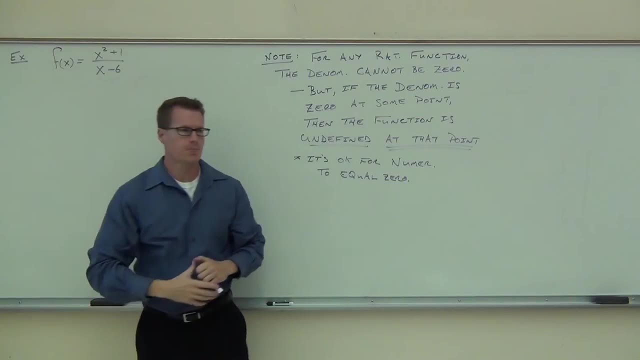 this a function specifically. Yeah, okay, so it has a function name out there. That means it's a function. So this, if I cover that up, that's an expression, That's now a function. That's the difference. Now we're going to talk about domain. Domain has a capital. 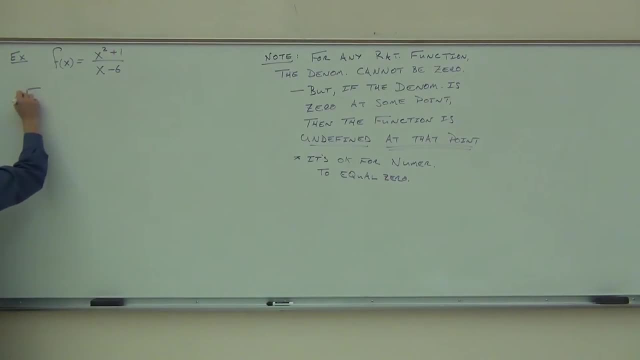 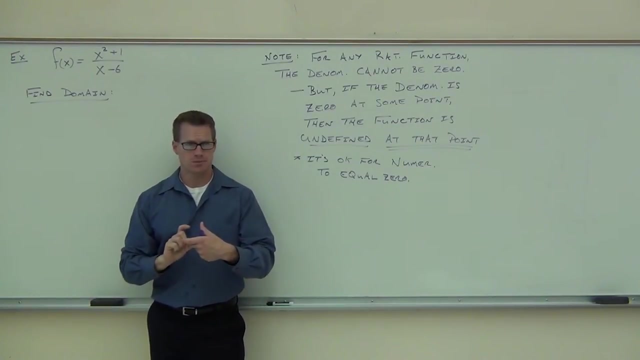 letter D. So we're going to find the domain. Here's kind of a layman's term definition of domain. What the domain is is every value, every input that you can plug in for x and get something out of the function. That's really all it means. It says what are the values you can. 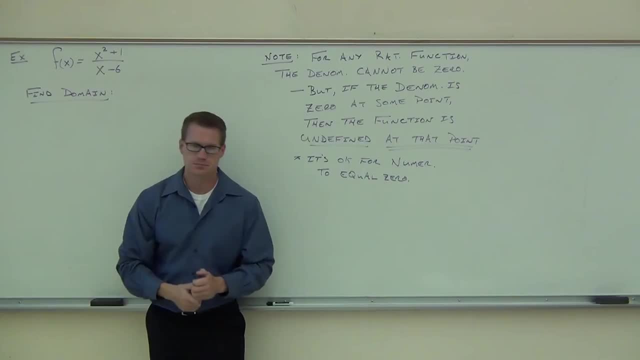 plug in and be okay. You get an output. We say domain. Domain is like this: Here's how we're going to write domain in this class. This is the set version way of writing domain. You write this kind of nice-looking bracket. 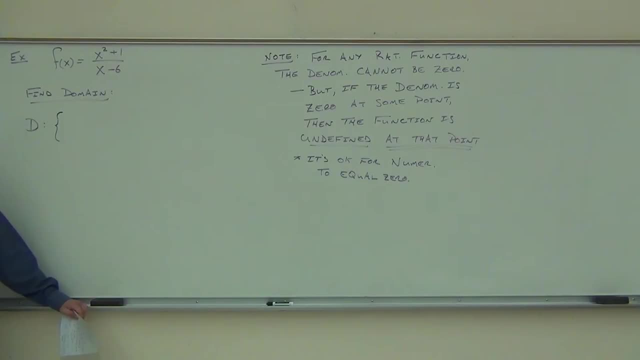 there, which is hard for some people to draw. I know that It ends up looking like a green thing. Okay, that's fine. Just try your best. Remember this when you get your master's degree in math: how to do that. It's all we do. It's horrible, I'm just kidding, but it's fine. 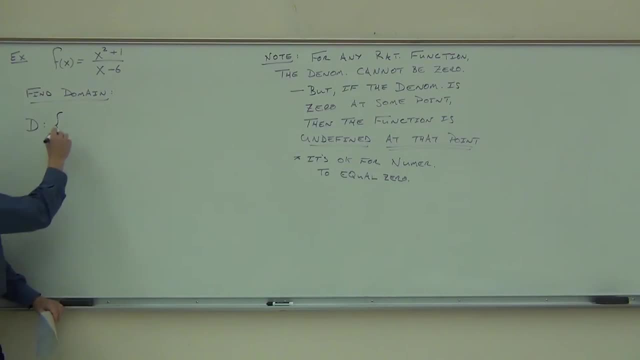 Then you write your variable. What variable are we using here? x. You write your x, You write this vertical line that says such, that It says x, such that. Here's how you're going to finish this off: x is a real number. I'm going to use a symbol. 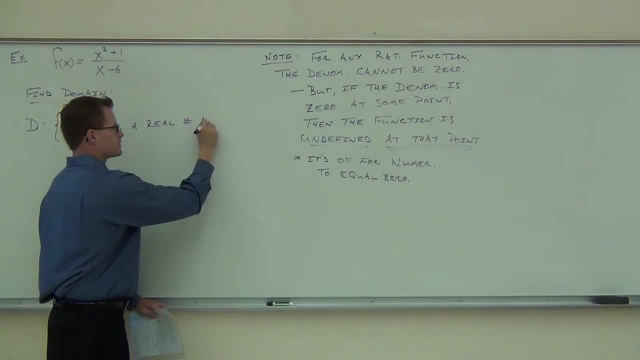 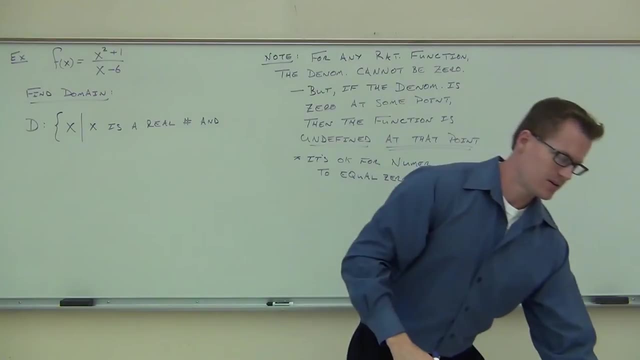 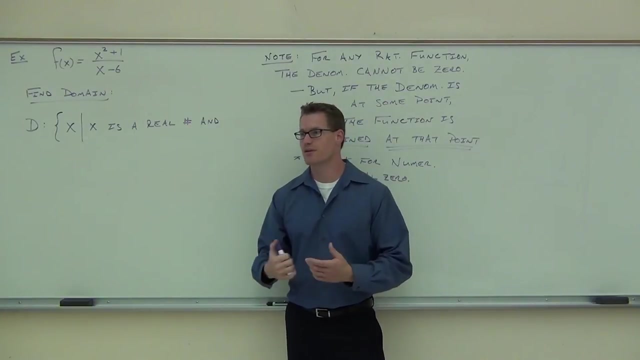 because I'm lazy- Real number. I'll show you how to complete that, and in just a second a second. Firstly, the real number, part Real number. Why do we say x is a real number? Is there anything like a fake number? The answer is no, there's nothing like a fake. 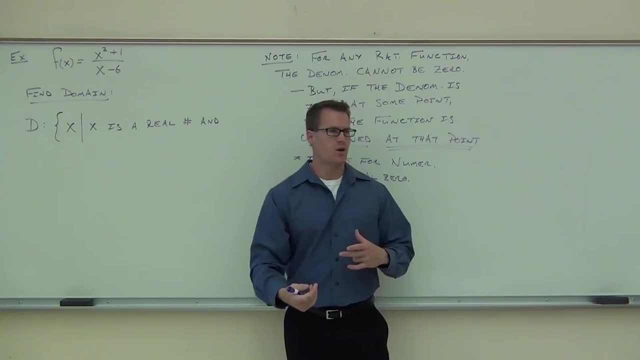 number, But we are going to talk about what are called complex numbers or imaginary numbers, And that's a little bit different. So what we're doing is we're saying x is in the class of real numbers. here, A real number is every number you've ever dealt with in your whole. 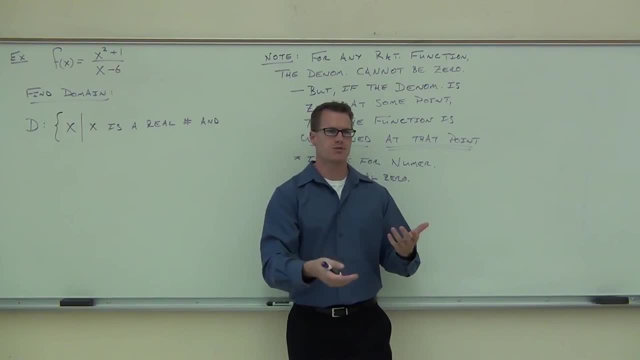 life. So all the whole numbers: 1,, 2,, 3,, 4, 5, all the negatives, negative 1, negative 2, negative 3, all the fractions: 1 quarter, 3 quarters, 7, eighths, all the decimals, you. 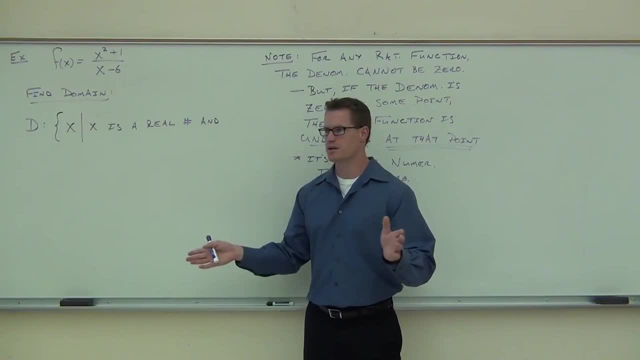 can think of pi, square root of 2, non-terminating, non-repeating decimals. Every number you can possibly think of, all put together is the group of real numbers. Am I getting that across to you? So when we say real numbers, we say x is anything you want it to be, And we're 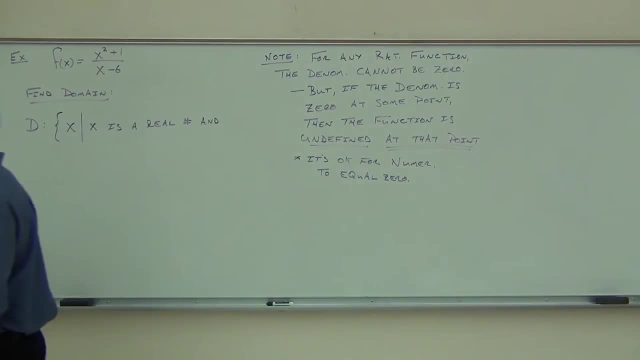 going to put conditions on this. I'll show you in just a second. I want you to look back at this problem. okay, We're going to look at this problem and we're going to think: are there any numbers that I cannot? 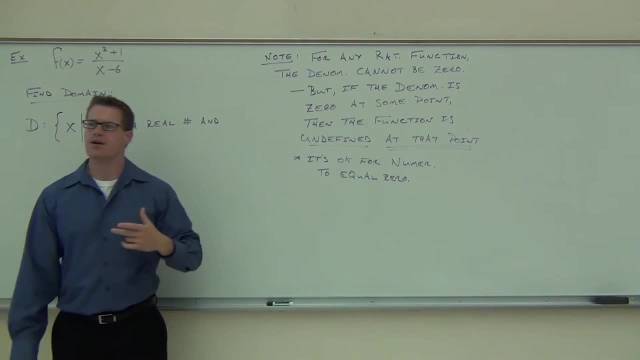 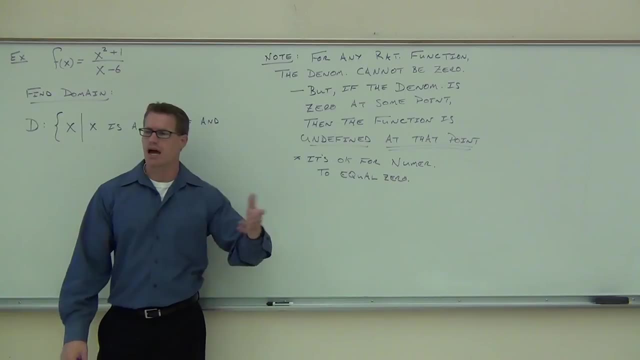 plug into this problem because it would create the one error I cannot have in fractions. And, by the way, what's the one error I cannot have in fractions? Zero, I can't have. how about the top? Does the top matter? No, 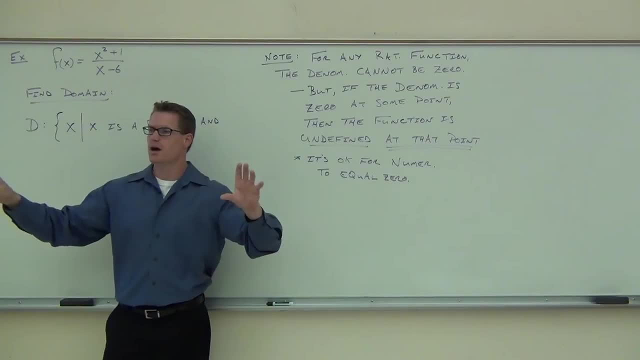 No, numerators are fine. You can have zero there. I'm not even going to look at the numerator when I'm going to have a fraction. I'm looking for domain. Don't even care. And our other problems, yeah, we care about. 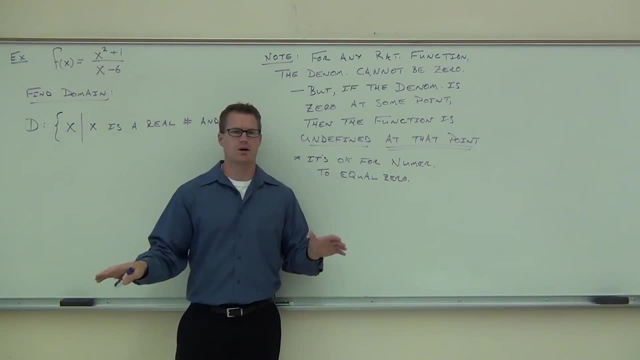 the numerator, But when you're just talking about domain, I don't care at all. What we're going to look at is the denominator. What is my denominator right now? Is there a number that I plug into there that is going to make the denominator equal to? 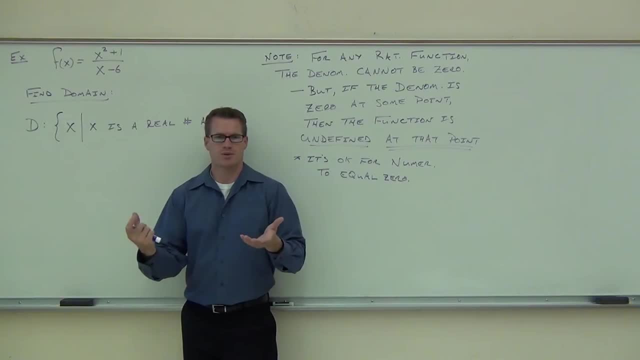 zero Six. Yeah, It's not zero, right, Because if I put zero in there, it'd be negative six. That's fine. It's not one, because that would give me negative five, But if I plug in six into that, we'll have six right here. Notice how six minus six is equal to zero, right? So 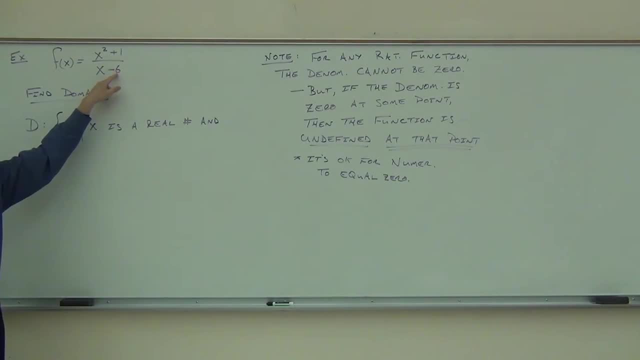 six minus six is zero, right. Is that okay to have? No, Nope, It's not okay to have. So what we're going to do is we're going to say: x is a real number. I can plug in anything else, right. 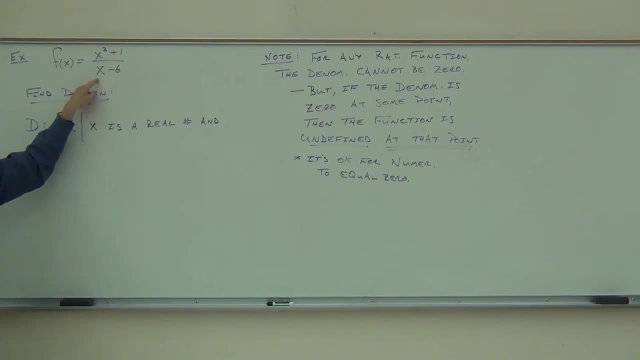 Yeah, I can plug in. if I plug in two here, is it okay, Mm-hmm? If I plug in negative six, is it okay, Mm-hmm? Excuse me, negative 12.. The only number I cannot plug in is positive six. Nod your. 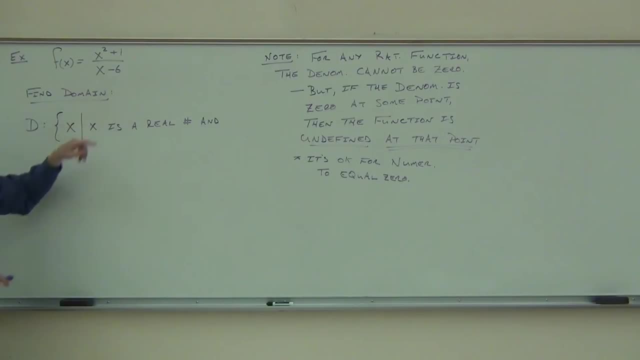 head. if you're with me on that, That's the only number that would be bad. So we go. x is a real number, anything, and x cannot equal six. That says, if x equals six, I get a bad problem here. I get something that's undefined, That's. 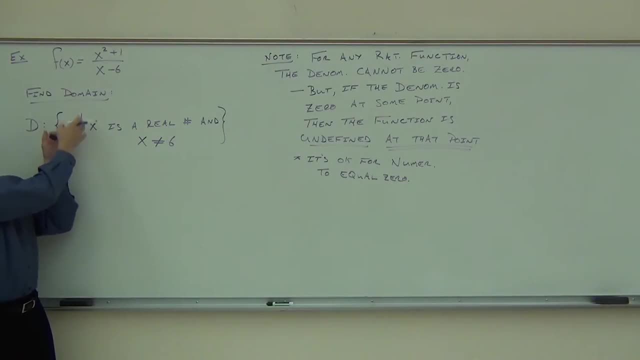 how you write your domain. You write x, that's from a variable, such that x is a real number, except x can't equal six. That's basically what you're saying in this problem. Now, one way you can show your work on this without having to just think about it: what you do. 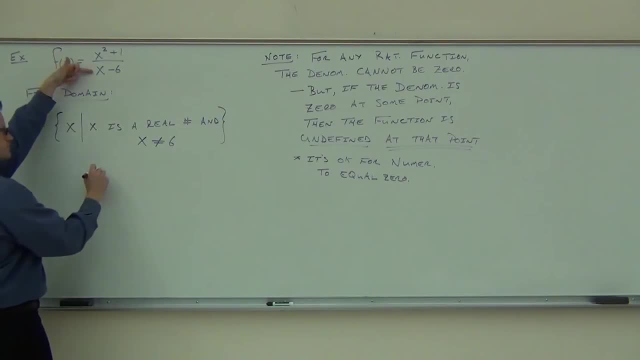 this is going to seem kind of weird to you. you take your denominator, you set it not equal to zero. Why? Because what's the one thing? the denominator cannot be Zero. So set it not equal to zero, Then you solve it like you would any other equation. You. 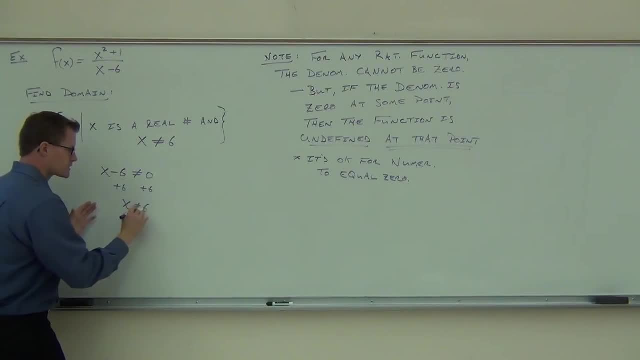 add six to both sides, you get: x cannot equal six, and that goes right there. Does that make sense to you, Mm-hmm? So you just set denominator not equal to zero. solve it. So to find domain you have to write: 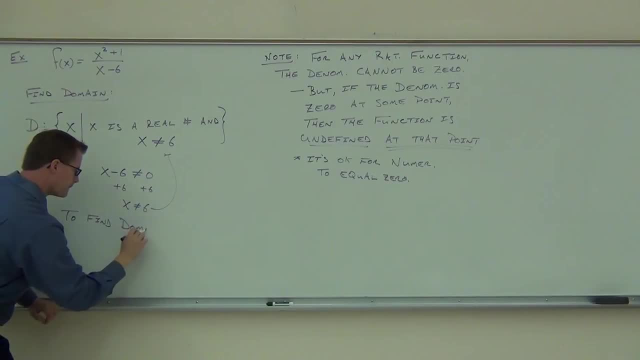 the statement. by the way, Okay, Set denominator not equal to zero and solve it. And you know what We're going to practice: a lot of this next time. How many of you feel okay with what we talked about today? So you, 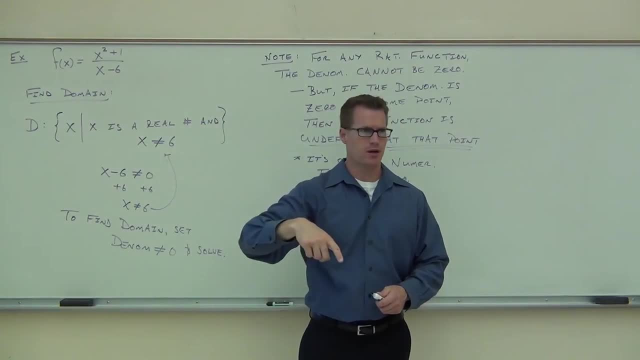 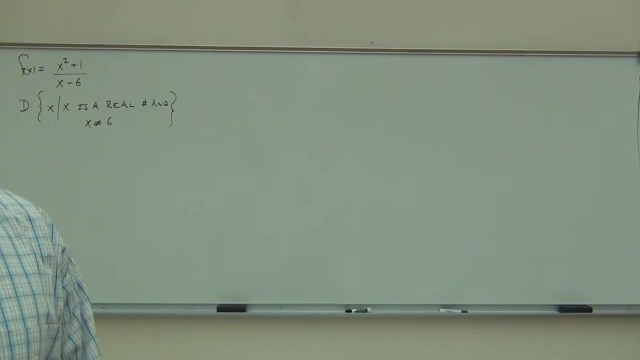 feel okay with the dividing polynomials that we started with right And now the whole domain idea with rational functions. We're going to get onto more of that next time, Okay, All right, All right, Okay. So if you do remember from yesterday, we did do that problem and we said that domain. 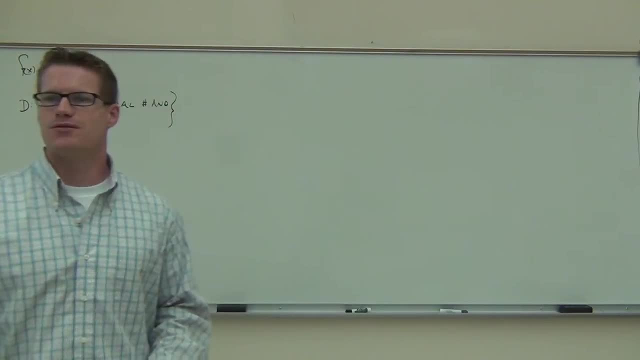 is really all the numbers that I can plug into a function and get something valid out, So pretty much anything that's not undefined. And when we went through this we said there's one thing with fractions that we cannot have and that's zero on the denominator of a fraction. 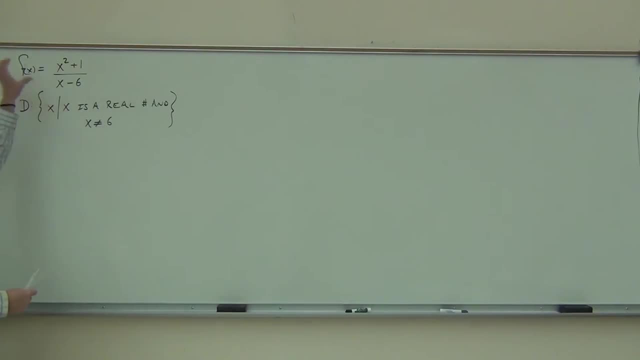 And so, when we look at the problem with domain at least, we really don't care about numerators. We look right at the denominators and what we know is that our denominator cannot be equal to zero. So what I've told you to do is: it sounds a little weird, but set your denominator, not. 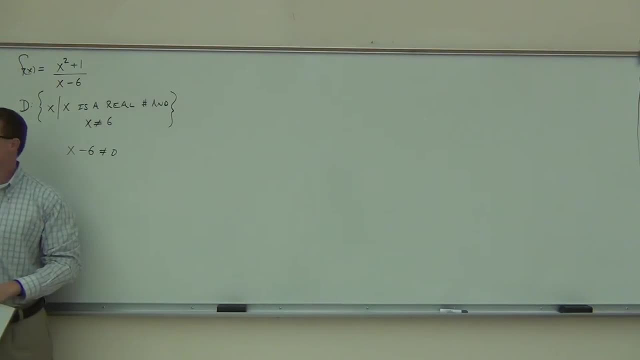 equal to zero. like this and solve it. This will give you the point, or points that you cannot plug into your function. Are you with me on this? Everything else will work, except this point. So we add six to both sides and sure enough, we get. x does not equal six. 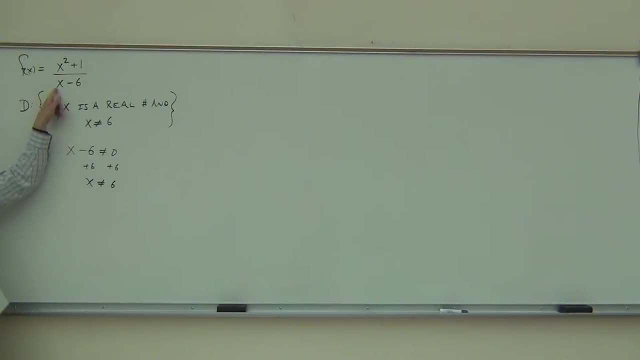 and that's what we had there originally. And that makes sense, because six is the only number I can plug in when the denominator does equal zero. That's our problem. Are you with me on this one? so far, All right, let's practice a couple more to see what the hang of this, And again we're. 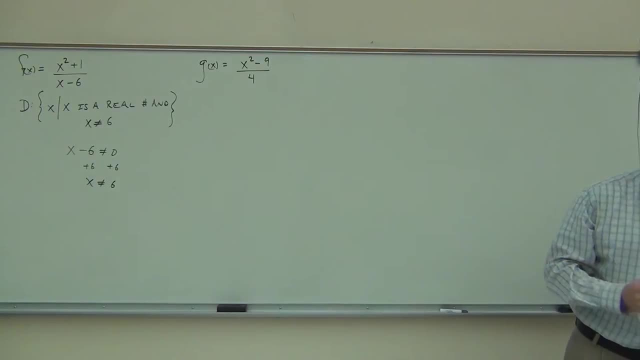 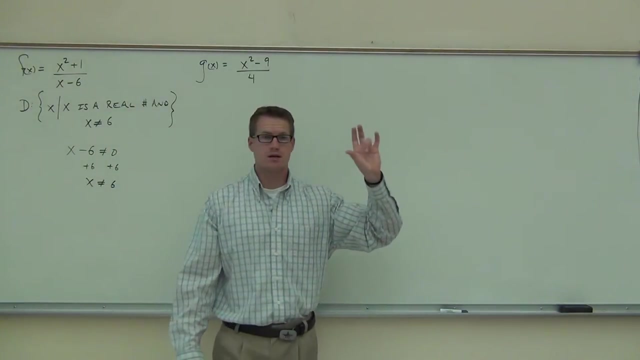 looking for domain. We have g of x equals x squared minus nine over four. Hey, by the way, is it okay for the numerator to equal zero? Yes, The numerator That's the top of our fraction. Is that okay? Yeah? 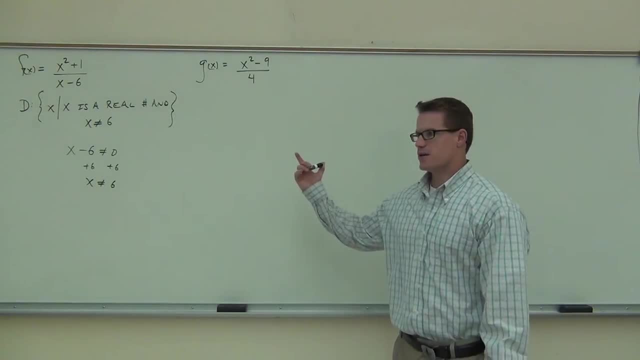 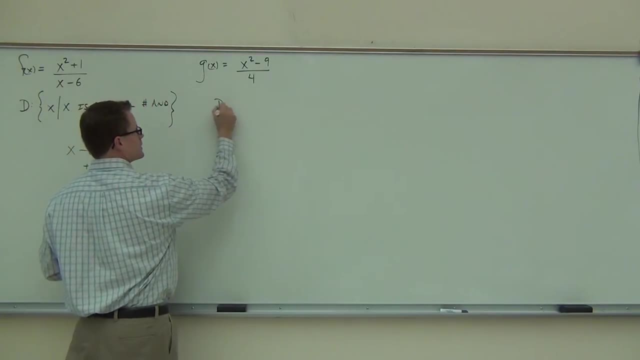 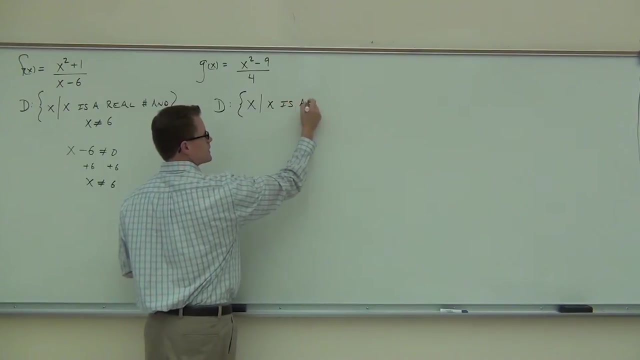 Okay, How about the denominator No? Is this denominator ever going to equal zero? No, Okay. So when we write our domain, here's how we'd start it out. We'd say: the domain is. we're going to write the same thing every single time: x, such that x is a real number. 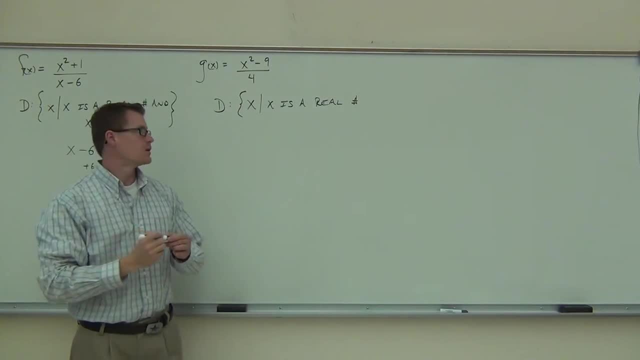 and we would put any problems that we have. Now I'm going to ask you a question: Is it okay if x equals zero? Yeah, Is it okay if x equals four? How about negative four? Think about it. If I plug in negative four, I know there's a four right here, but if I 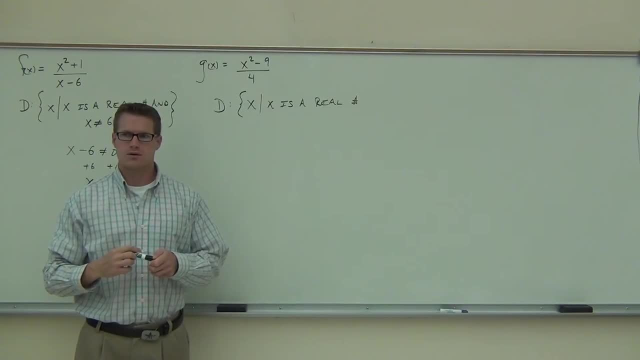 plug in negative four. is the denominator going to be zero? No, Then I don't care. Yeah, that's fine. How about three? Plug in three. It's wrong. No, Is that okay or not? No, Yeah, This is going to be zero. 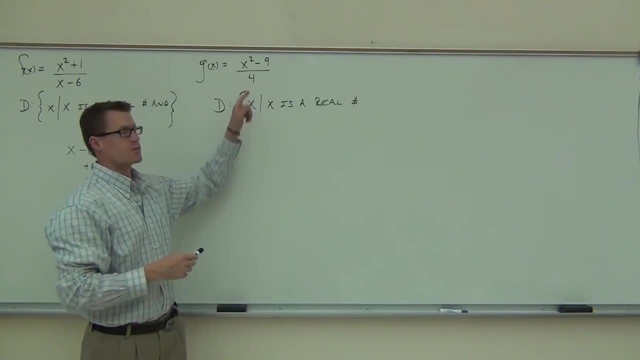 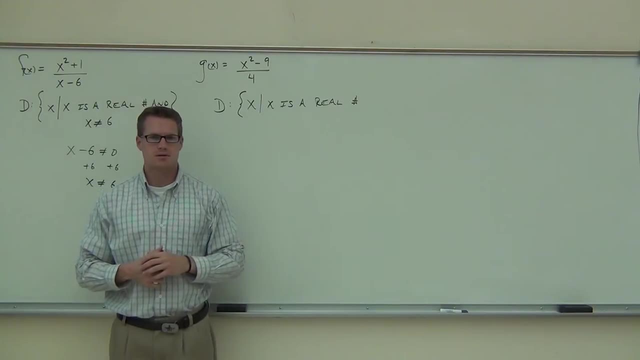 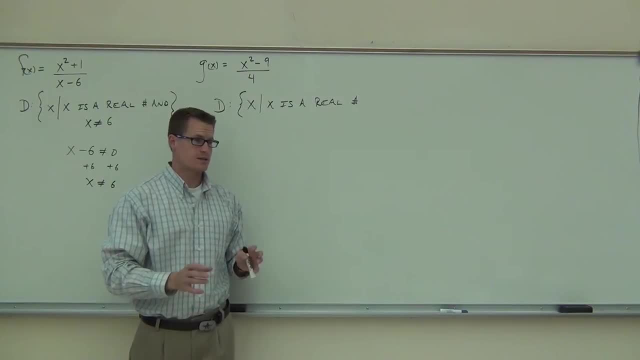 No, No, No. Is the denominator going to be zero? No, Then that number's fine. Okay, It's only the denominator that I'm checking forward with domain. That's it, Just the denominator I'm checking forward with domain. 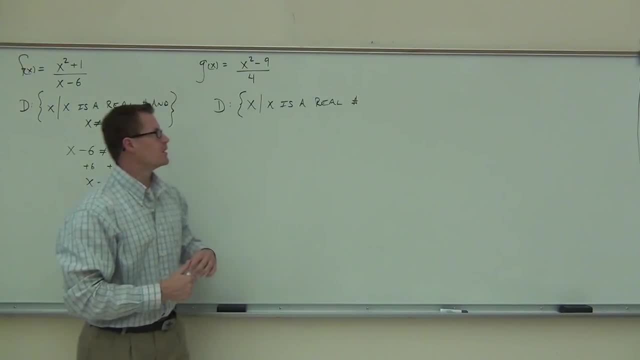 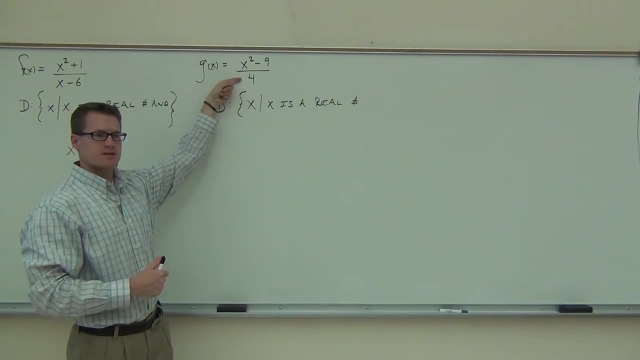 If the denominator is not zero, your numbers are valid. So can you see here on this problem, that no matter what I plug in, this number is never going to change. Are you with me on that? No matter what I plug in, That means that this denominator will never be zero, which? 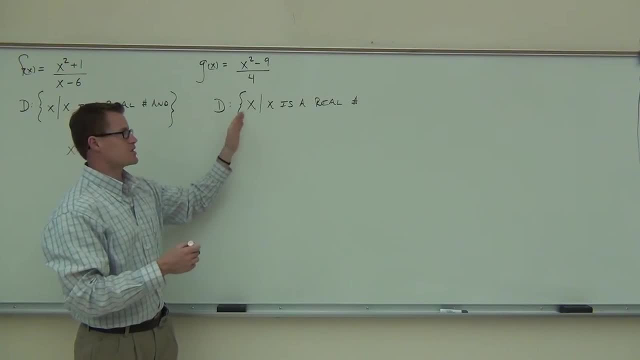 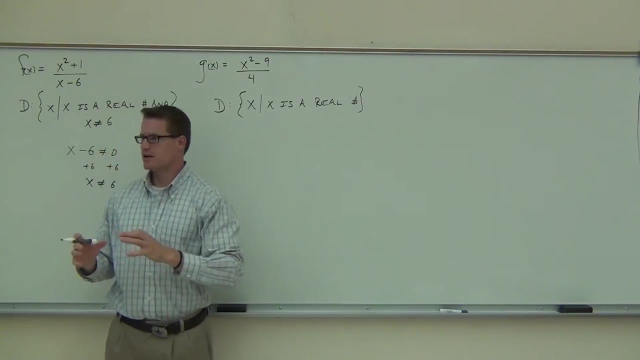 means that any number works. Now we've saved that as x. As x is a real number, So this says in a nutshell: any number will work. If you plug in anything, you'll get something out of it. that's valid. 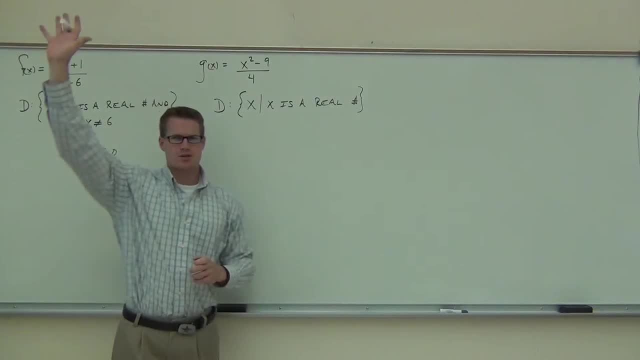 Even if we get zero. that's fine, but you will get something out of it. I think we'll understood that one. Okay, why we don't have this, Why we don't have this part of it? Well, you had a variable down here. 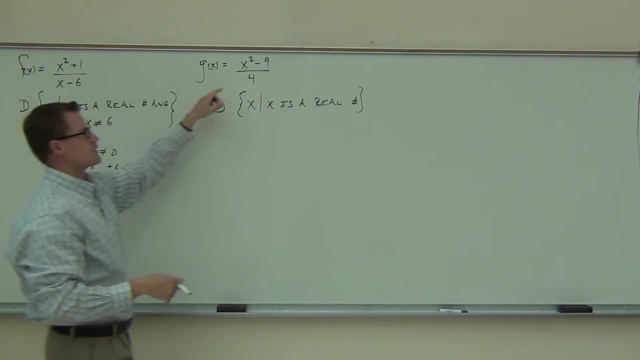 If you plug something into that, specifically six, it's going to be zero. Here you don't have a variable, It's a constant. That number's not going to change. That number's never going to be equal to zero, no matter what I plug in. 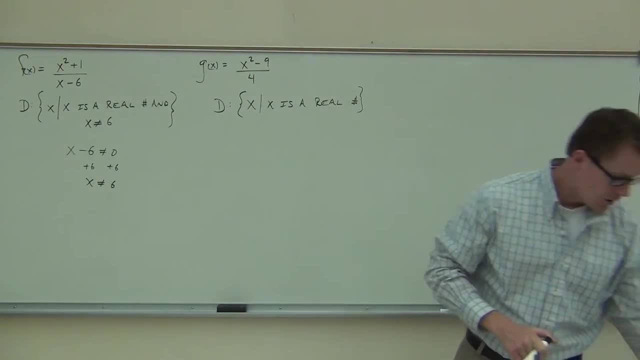 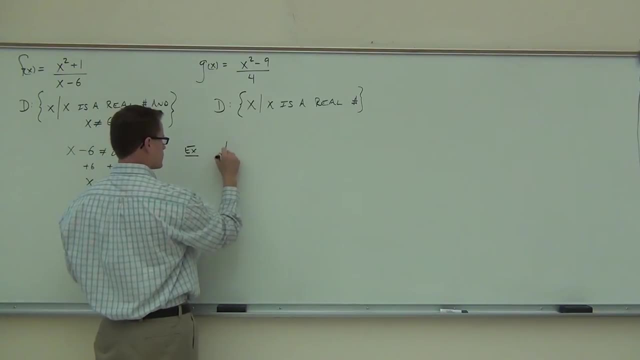 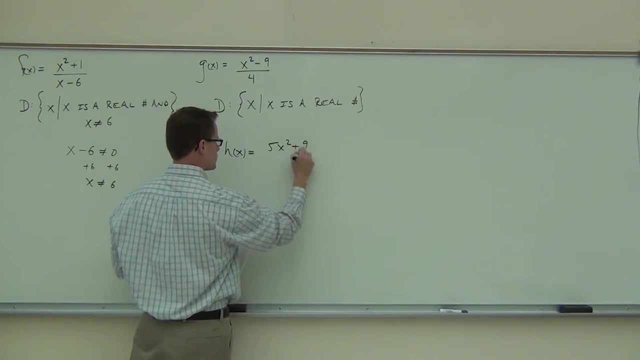 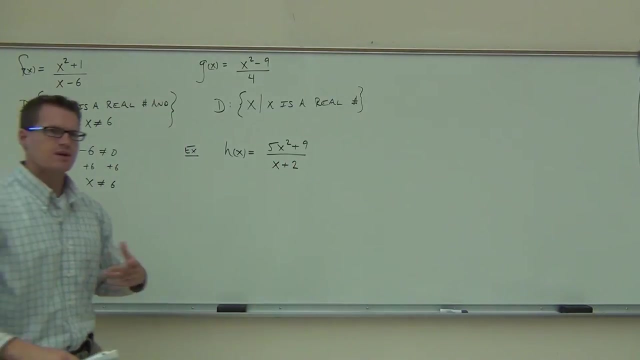 Follow. Okay, I'd like you to try one on your own, Just so you get the hang of it. I want you to find the domain for. I'm going to write the domain for H of X here. So we're going to write the capital D, We're going. 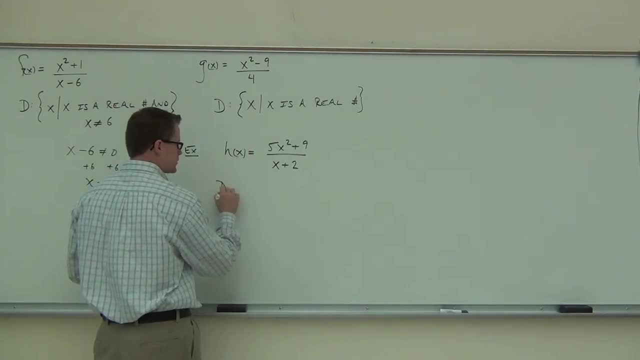 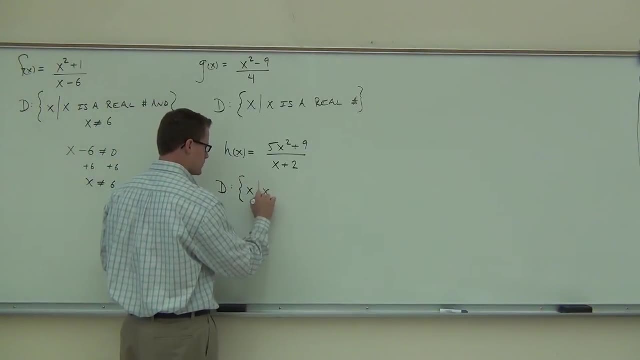 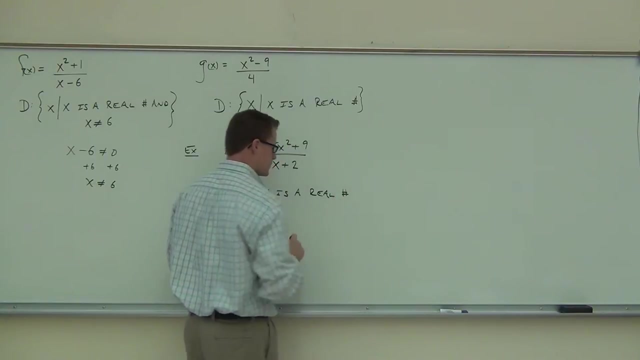 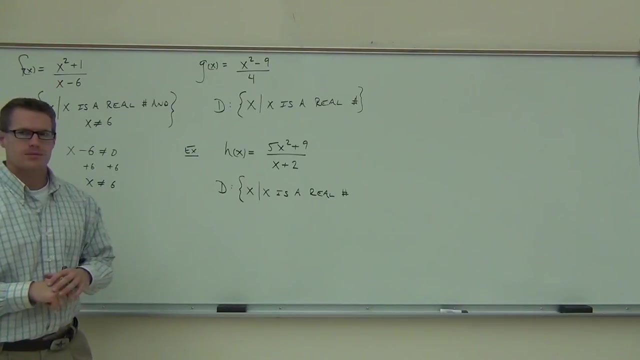 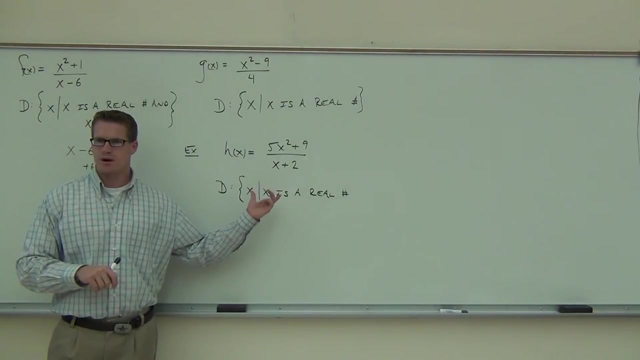 to write the same thing, X, such that X is a real number, And then you're going to find out if there's any points that are problematic here. Hey, is this problem all real numbers, like the last one was No, Or do we have problems here? 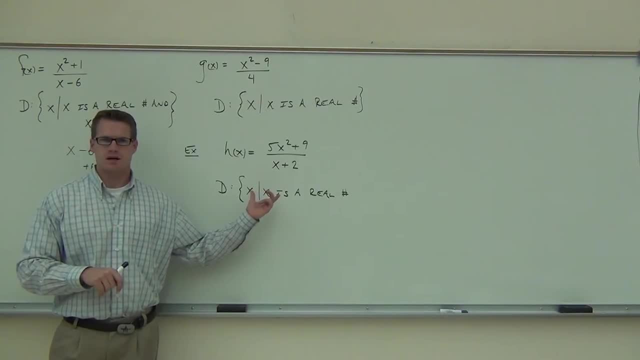 Probably. Yeah, I have some people going yes, some people going no. Well, we've got to look at one spot specifically. Do we care about? for domain I'm talking about only do we care about the numerator if I'm asking for domain? 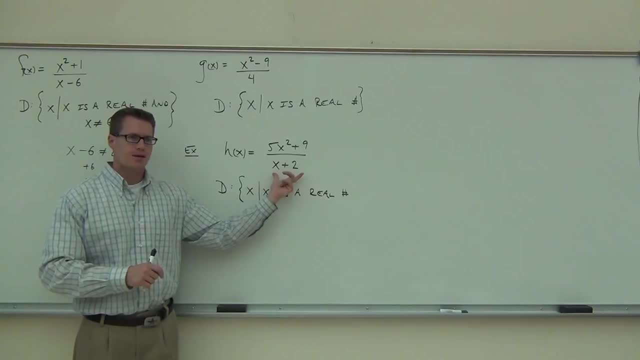 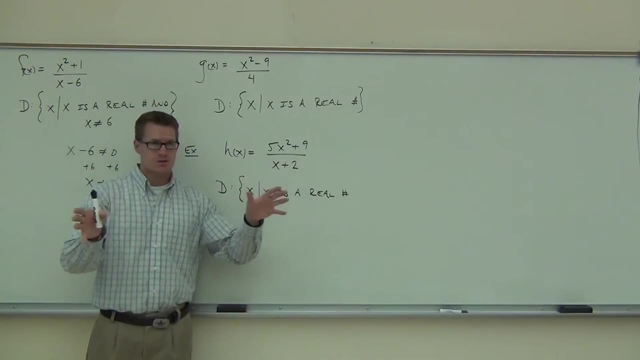 No, We care about the denominator, that's right. And the question is: are there any points, any values that are going to make this part of it zero? Yeah, that's great, And the way you find that out, because this is very easy. 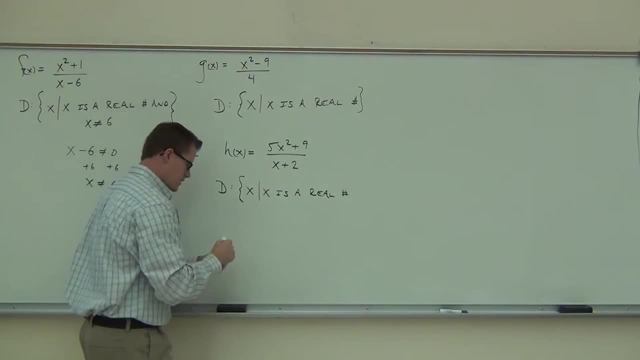 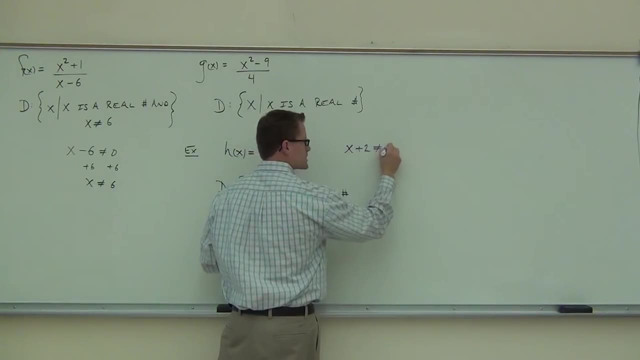 we can do this one in our head, but the process is, what we do is we take the denominator, just the denominator, and we set it not equal to zero. Why do we set it not equal to zero? Because that is the one thing that we cannot have it equal to. 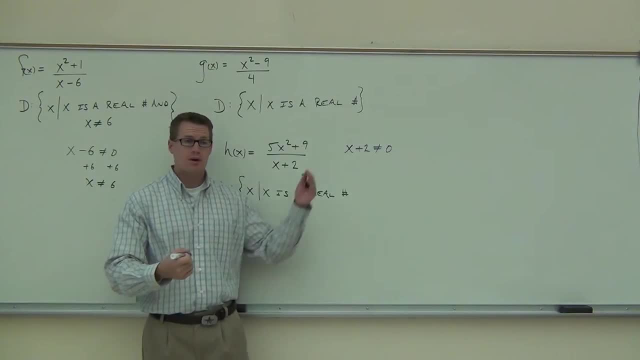 Are you with me on that? It's kind of a weird thing to set it not equal to zero, But when we solve that down, that's okay, That works out for us and it goes right here. So if X plus 2 cannot equal zero and you solve it. 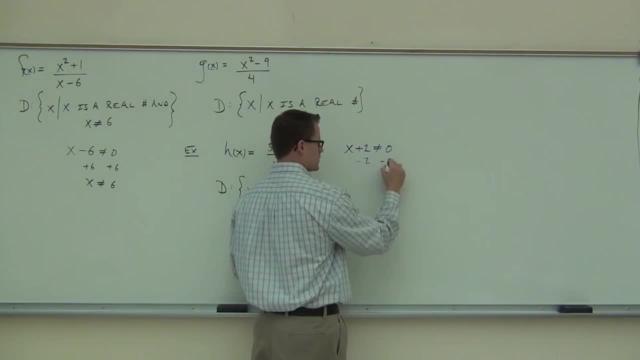 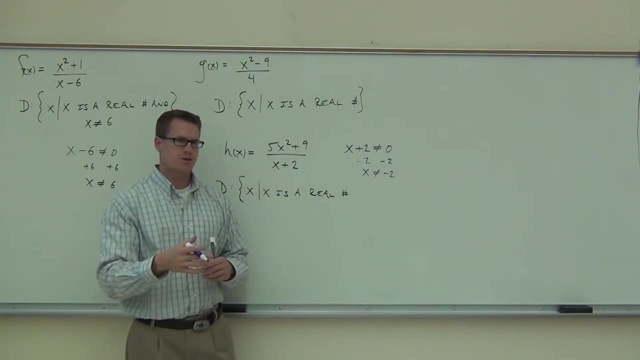 that means you're going to subtract 2 from both sides and you're going to get that X cannot equal negative 2.. Why it cannot equal negative 2 is because if you plug in negative 2, look what happens. Put negative 2 there and do the math. 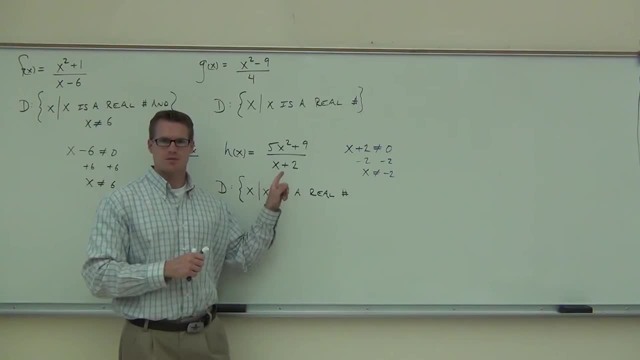 How much do you get? Zero. Is that a problem? It's a big problem. So we set the denominator not equal to zero, We solve it and we get this piece of the puzzle here And we write that we finish this off. 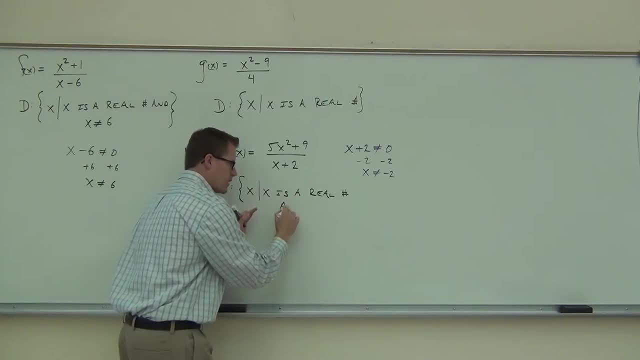 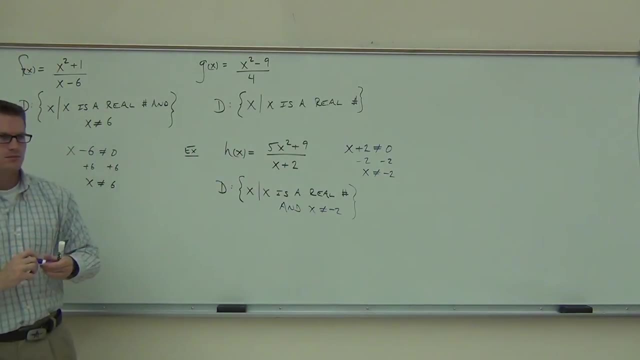 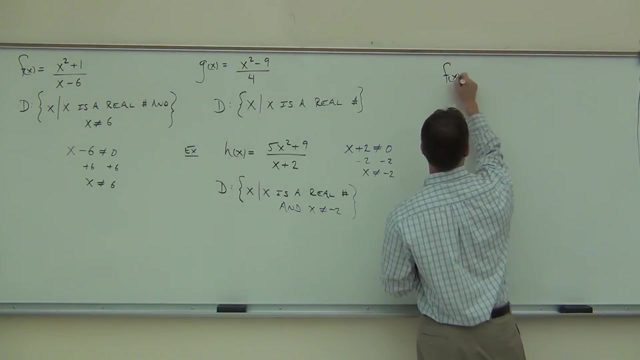 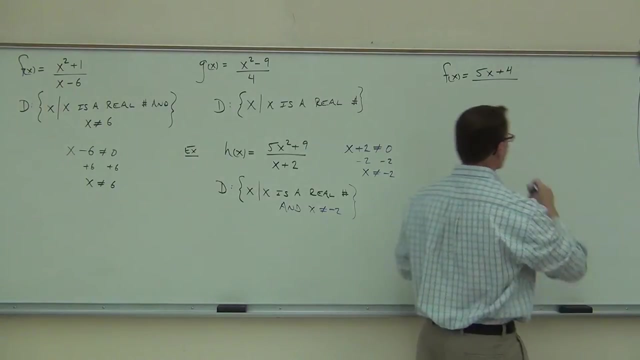 X is a real number, That means everything. but we go and X does not equal negative 2. And we finish that off. Now, what would happen in this case? We have, like H of X or F of X, whatever, 5X plus 4.. 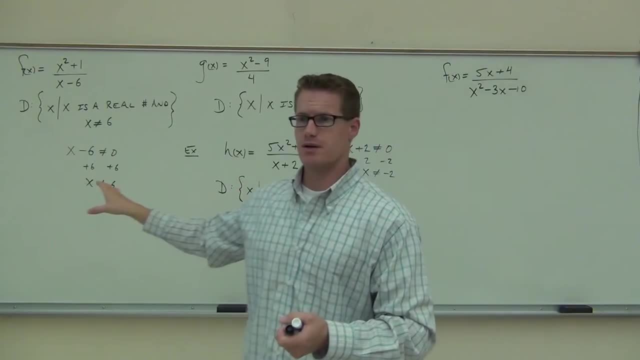 This is where I'm going to see if you were really paying attention to what I was saying over here, Because if you just looked at this and go: well, yeah, Mr Leonard, these are easy. That one's 6.. That one's negative: 2.. 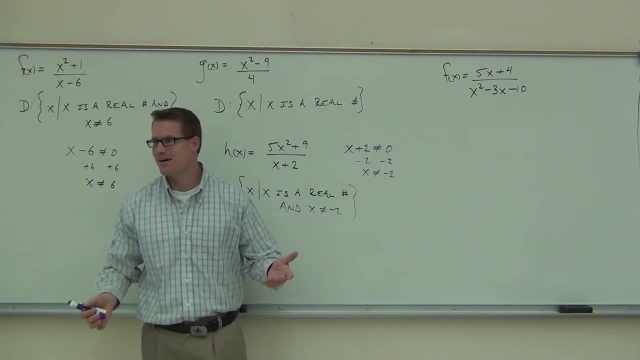 Duh, I mean, if you plug that in, you're going to get zero. I know that, I know that. Well, can you do that here? No, Not so much, I mean, unless you're like really, really quick, which some of you are. 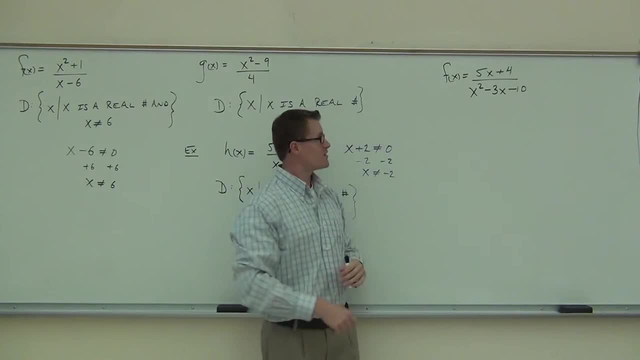 Just go. oh yeah, that's going to be well, I don't even know, But you're going to have to do the math on that. Actually, I think I know, But we'll find out. But the idea is the same as doing this step and doing this step. 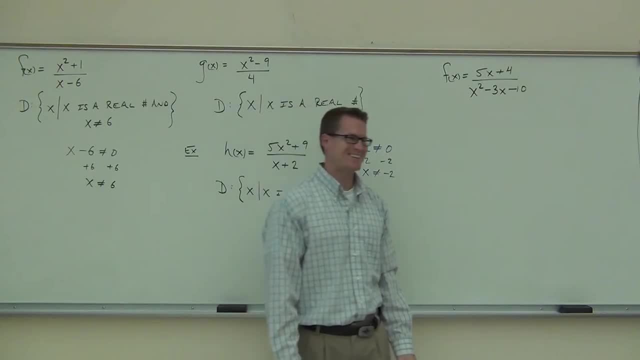 OK, That's what's going to lead you to this problem. So, when we look at this problem, we're asking for the domain which I am again OK, So we're going to look at this problem. We're going to look at this problem. 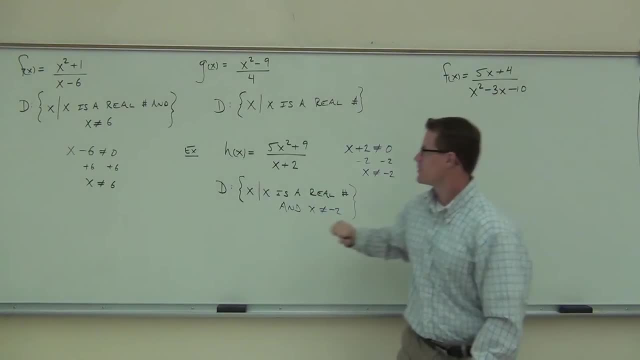 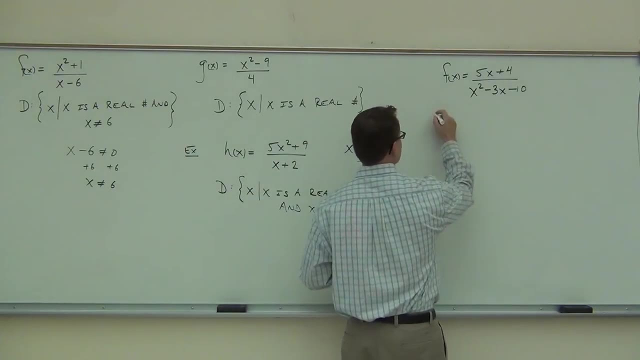 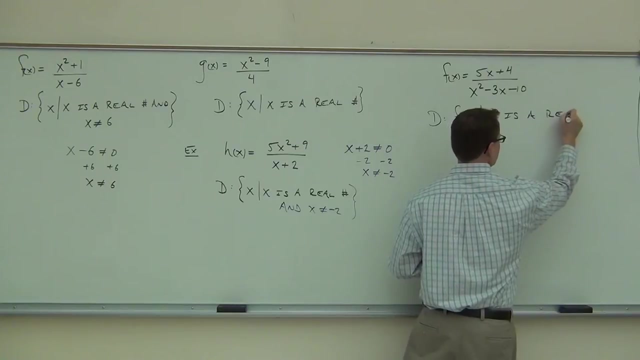 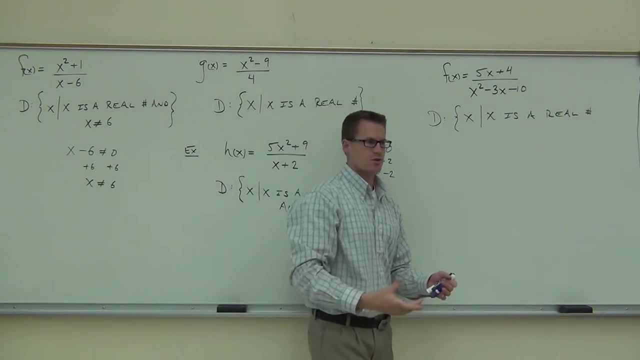 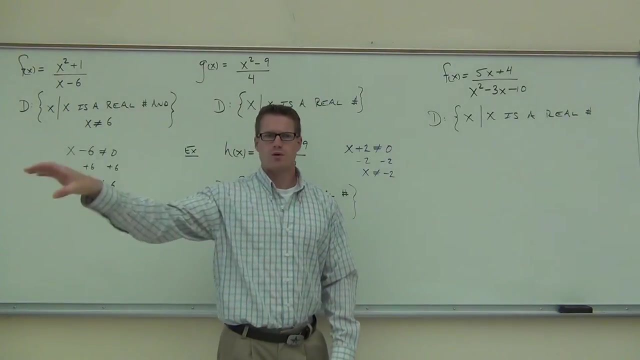 We're going to look at this problem Again. we're going to write x such that x is a real number. that pretty much says everything. And then the next part says your exceptions, your constraints, if you will. Now, what are we going to set not equal to zero? the top, our numerator or the bottom? 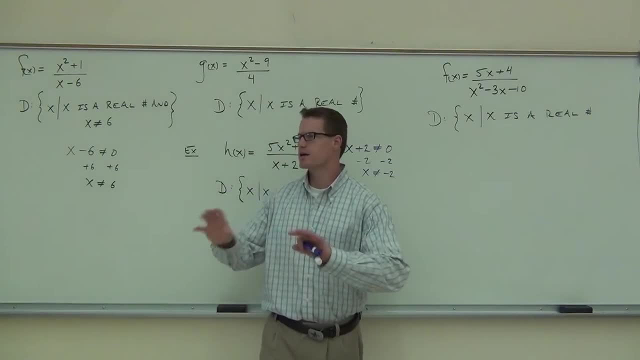 our denominator, Denominator, Denominator. OK, For domain we do not care about the numerator. For other problems, yeah, of course we're going to include the numerator, But for the domain we don't care about that. 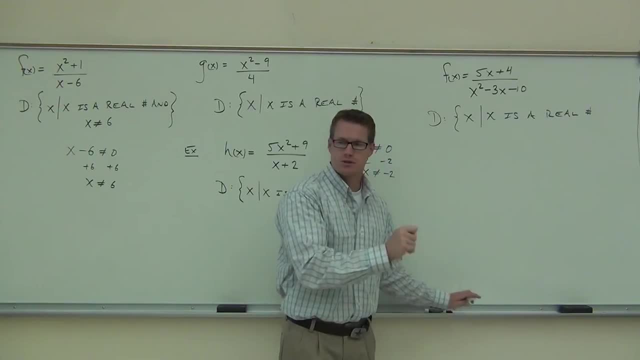 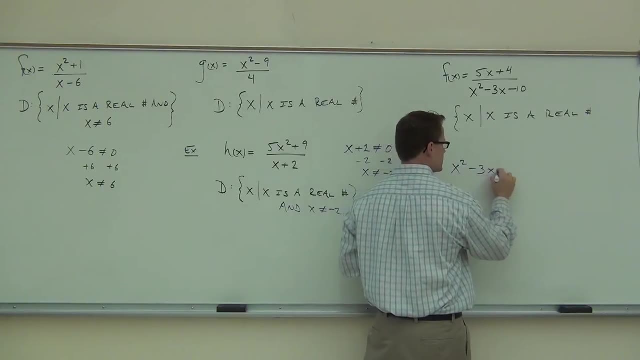 The top can be zero. It's the bottom, our denominator, that we cannot have equal to zero. And so what we're going to do, just like the last couple of examples, we're going to set that denominator not equal to zero. 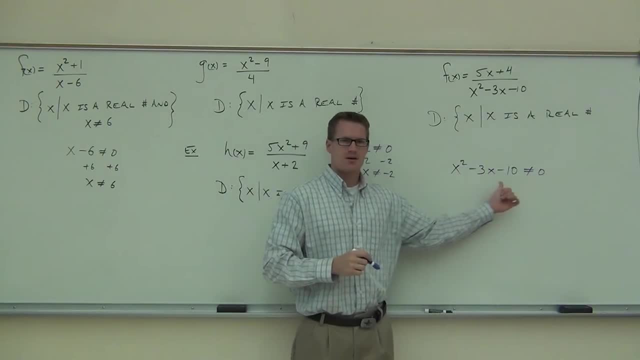 And we're going to solve it. But guess what, Hey, have you solved things like that before in here? Sure, That was your C.1 homework, right? When you remember how to solve something like this, How do you solve something like this? 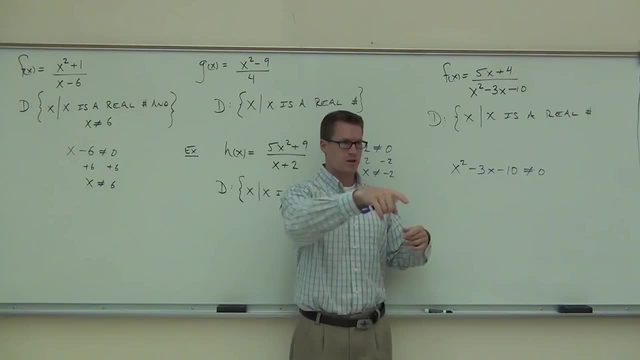 A diamond vector- That's right, Both of you are right- A factory, which, in this case, is going to be the diamond vector. OK, Now I do need to show you something. I don't have your homework back today. I forgot it. 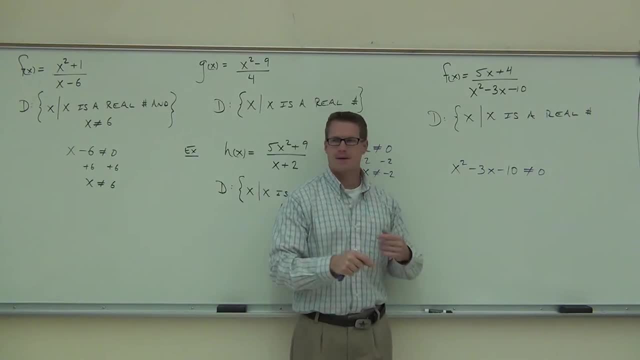 It'll be back tomorrow, But I need to show you something about whether you have the extra step or not, and this is a great problem for us. You do remember how to factor right Instead of the diamond problem, I hope. And what goes here is the negative 3 and the negative 10.. 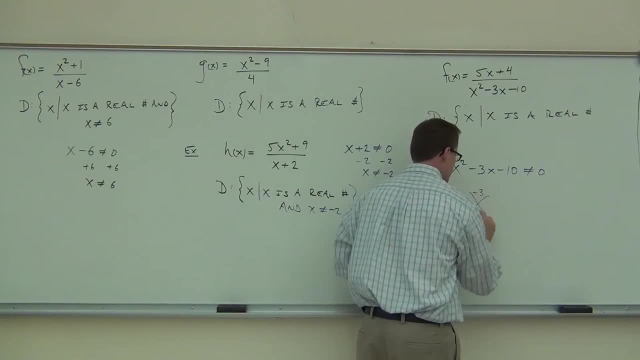 You see, a lot of you are spending a whole lot of extra time. Firstly, do you know how I'm getting the negative 3 and the negative 10?? OK, Negative 3, that middle number goes here. 1 times negative 10 goes here. 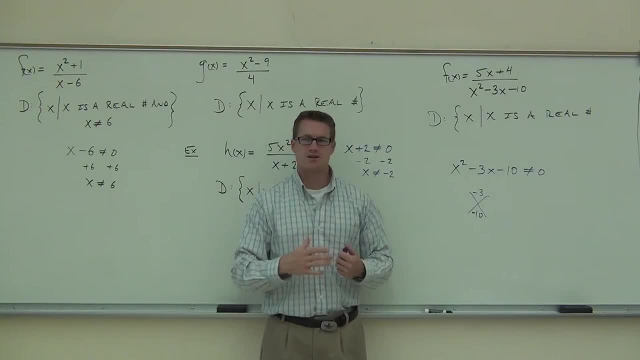 That's right. Negative 3, that middle number goes here. 1 times negative 10 goes here. Negative 3, that middle number goes here. 1 times negative 10 goes here. A lot of you are spending extra time doing that extra step when you don't have to. 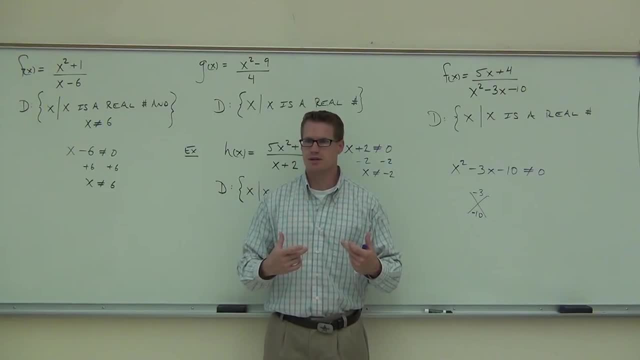 If you don't have to do the factor by grouping, jeez, don't do it. That takes like two minutes. You don't want to waste your time, right? I'm saving your lives here again. See what kind of a guy I am. 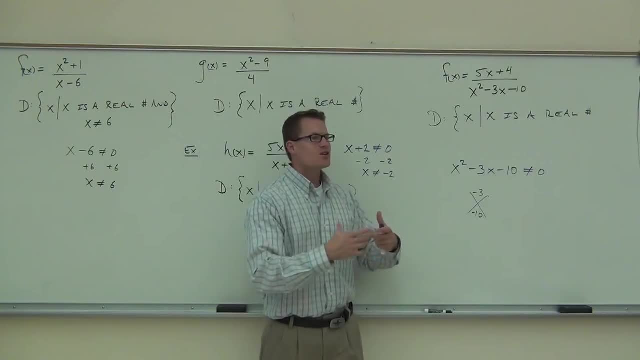 I'm helping you So you don't want to waste your time. if you don't need to right, That's just a waste of time on the test or something that you spend checking your answers or whatnot. So in this case, when you look at this problem, there's no coefficient besides this 1.. 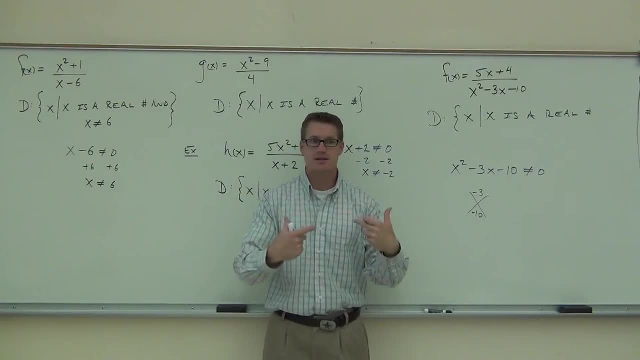 You do not have to split the middle term and use grouping. That is a waste of time for you. Am I getting through to you? You go directly to your factors. If you do have the number up front, then, yeah, you do. 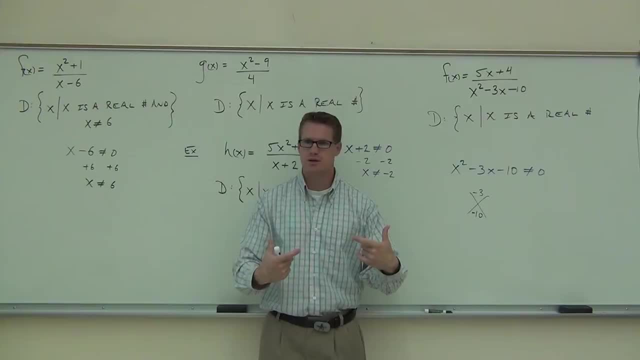 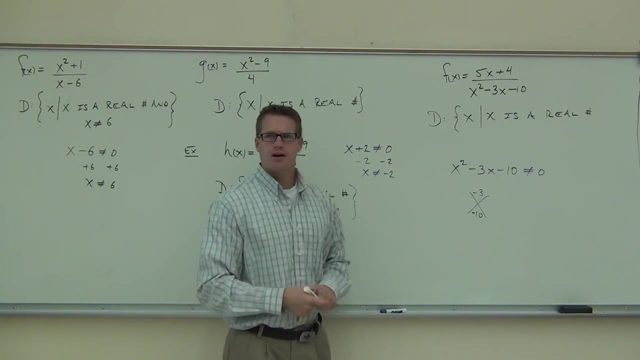 You split the middle term, then you factor by grouping. That's the only way we can do it in this class. So after you find these numbers. by the way, have you thought of these numbers as a rambling on there? Negative 2.. 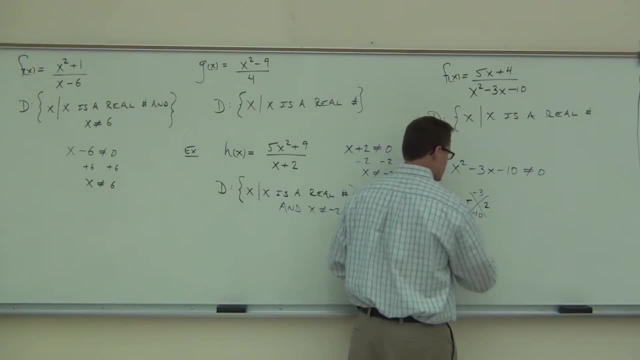 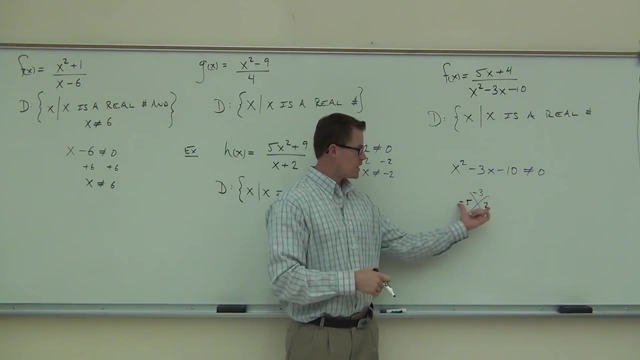 Negative 2.. Good, We're going to double check, make sure we get this right. Negative 5 plus 2 is negative 3.. Yeah, that works. Negative 5 times 2 is negative 10.. Yeah, that works too. 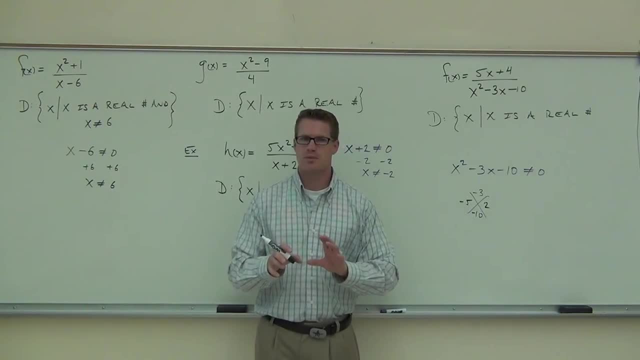 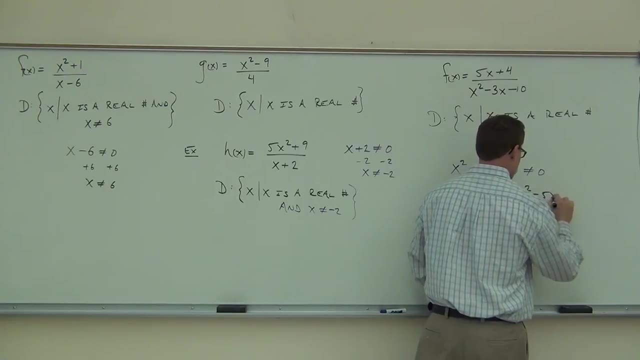 So those are the right numbers. Here's what I'm talking about: the extra step versus the not extra step. Some of you are still doing this. Please watch on the board. Some of you are doing this and still doing x squared minus 5x plus 2x minus 10.. 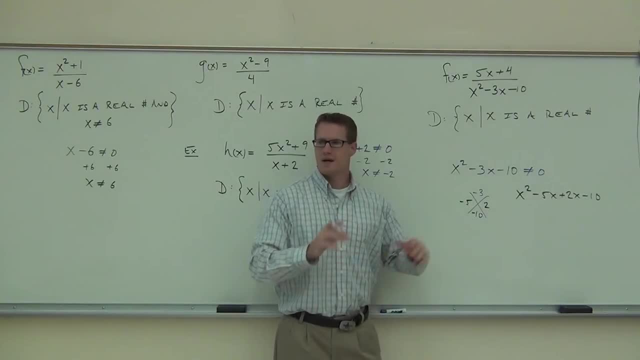 If you're doing this step on this type of a problem, you're wasting time. You're wasting it. Are you with me on this? You're wasting your time. You don't have to do this. This is too much work. If you had a number up front, yes, you would be doing this step, but you don't. 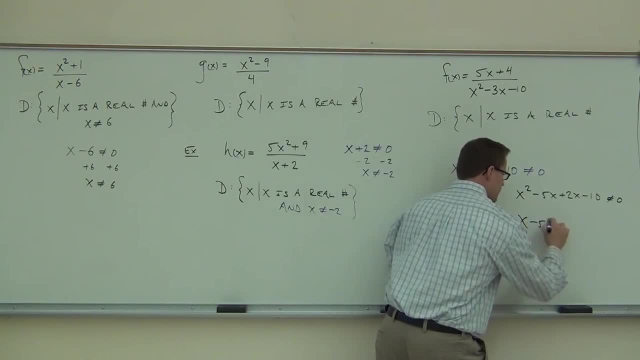 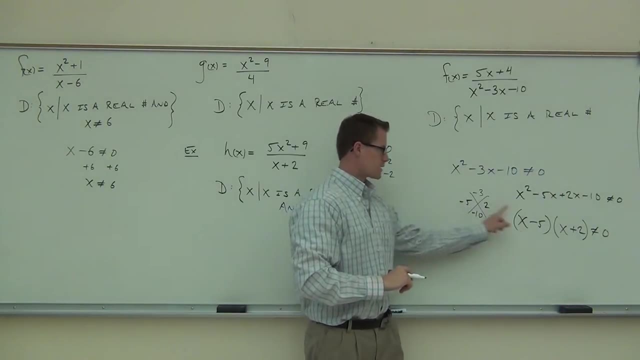 All you're going to do now is go x minus 5x plus 2.. You're going to go directly to your factors themselves. Why does that work? that work? it's because we don't have the number on the front. That's why it doesn't hurt us to do this. 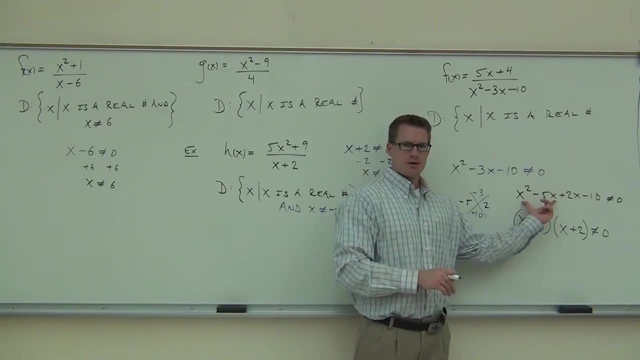 If you factored by grouping, you could still do it. it's just wasting your time. I wasted a whole bunch of time there Wasted a whole bunch of time. Some people waste a whole bunch of time because they do this every time and you're going. 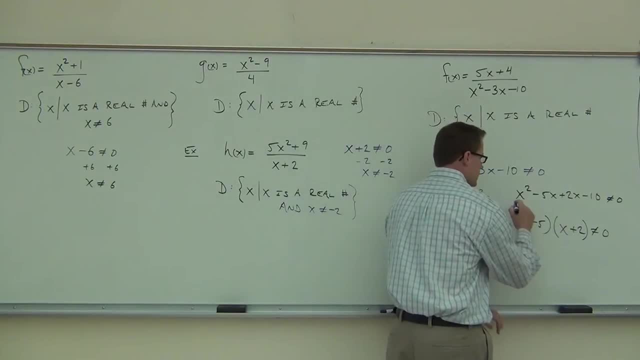 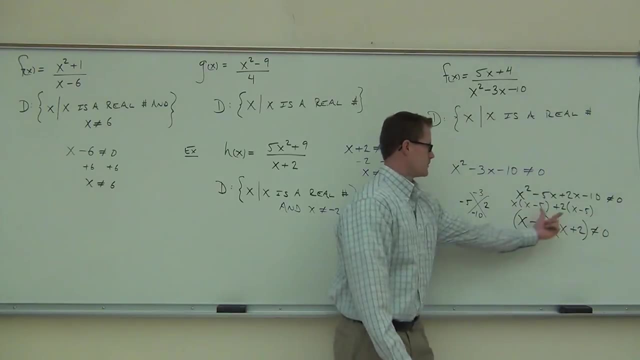 to get the same thing I proved to you right now. If you factored this out, you get X times X minus 5 plus X minus 5, look at it: X minus 5, X plus 2, but you don't need that. 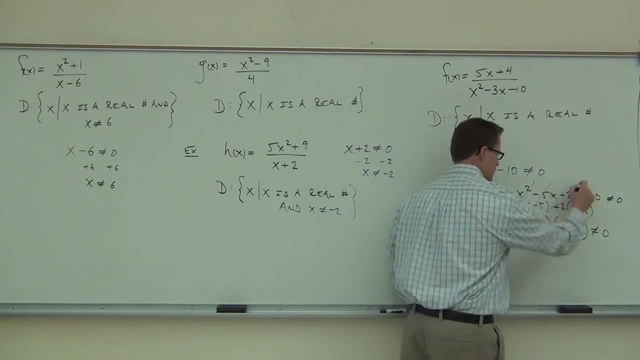 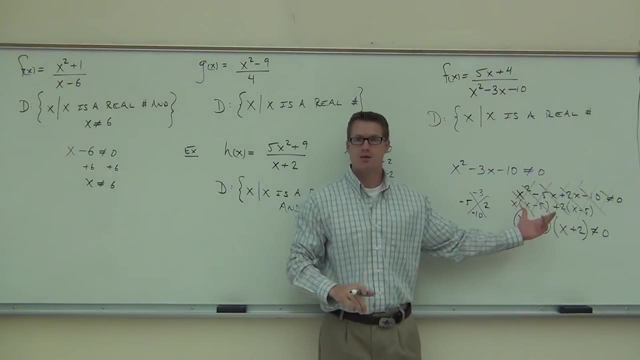 Okay, this is kind of a waste of time. Now can you do the extra step every time if you really really want to Sure, but if you want to waste two minutes of problem, then do it that way. If you want to be quicker on a lot of cases 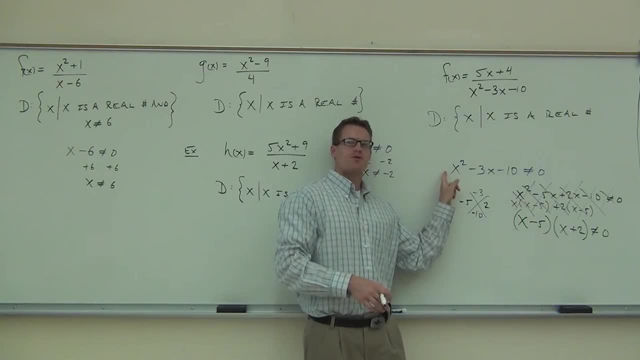 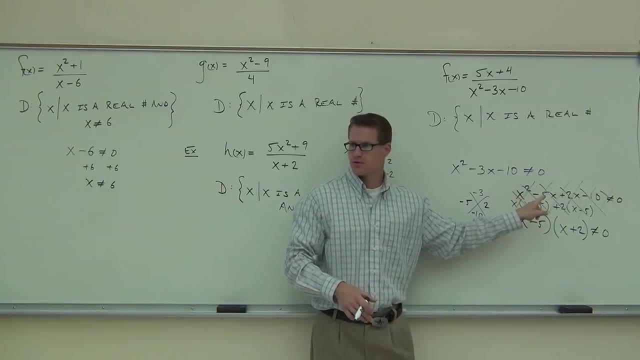 and just get this stuff done. then when you don't have a number out front, you go directly to here. If you have a number out front, you go and you do this stuff. Nod your head if you're okay on that. 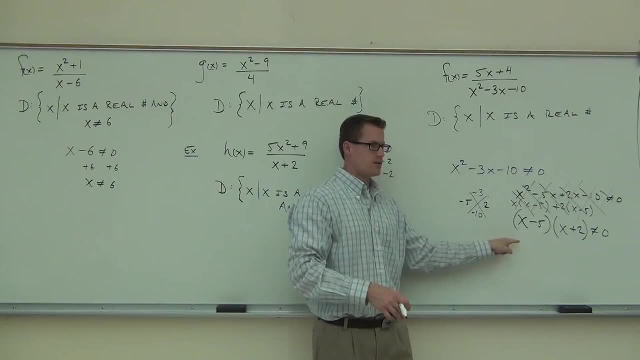 There's still time. There's still time. There's still two cases Number out front, this No number up front, this Okey-dokey Review, that lesson on factoring, if you haven't done so already online, if you've been doing this stuff. 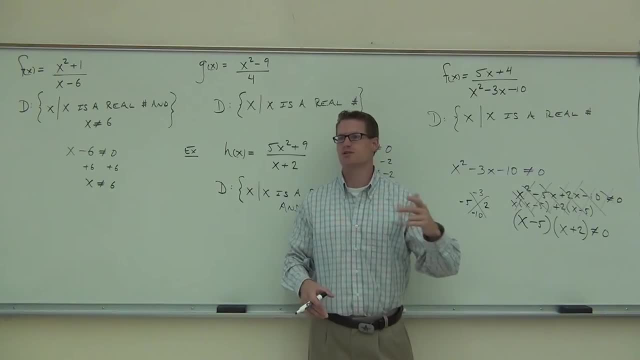 It's on there. I promise It's all in the C.1.. There's like 11 parts to it. They're all 14 minutes. The factoring is in the middle of that, So look through that. Okay. now, when we continue, we know about the zero product property. 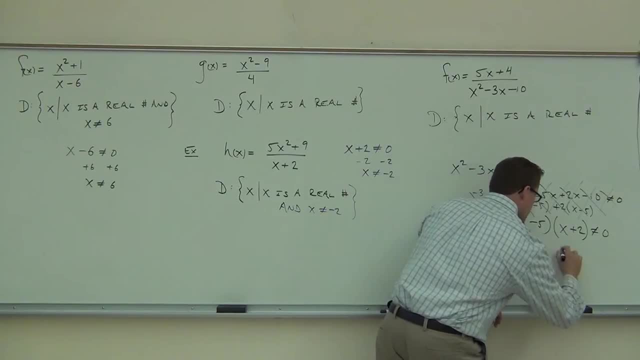 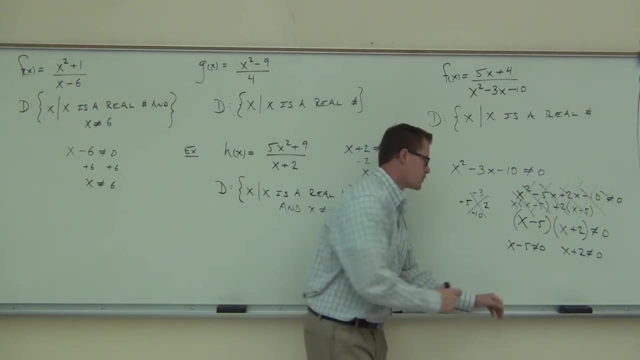 which will still work. we'll do: X minus 5 equals 0.. We'll do X plus 2.. Actually, not equal to 0. And if we solve that we're going to add 5 to both sides, We'll get X cannot equal 5, and X cannot equal negative 2.. 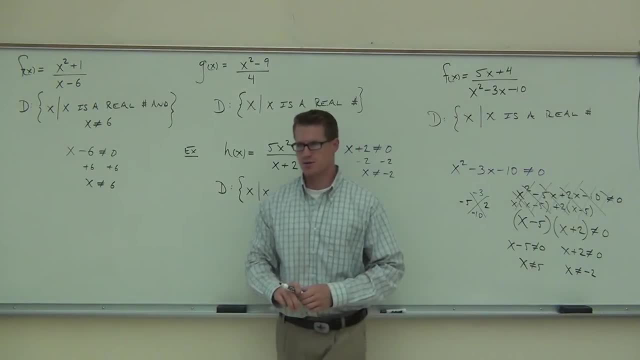 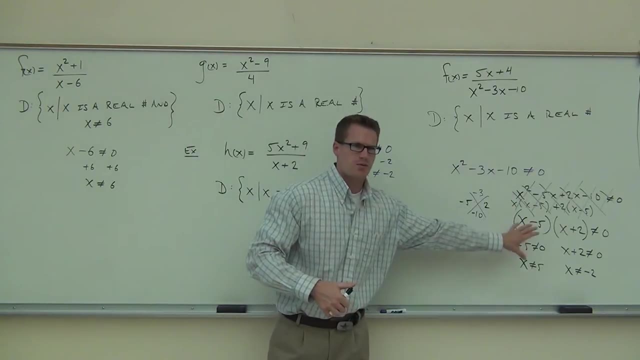 I'm just adding 5,, subtracting 2, and we get those two pieces of the total. This part you should feel. okay, on right, because we've done this already. This is our review. This was well, it was review when we covered it. 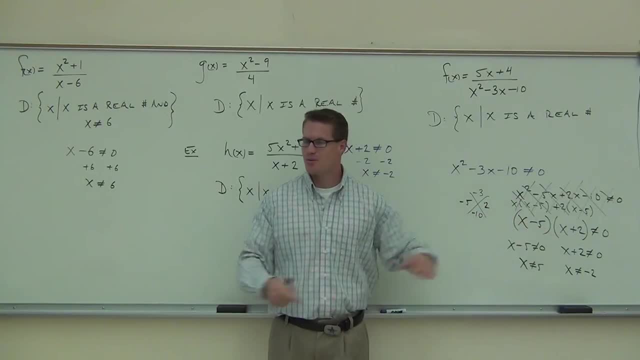 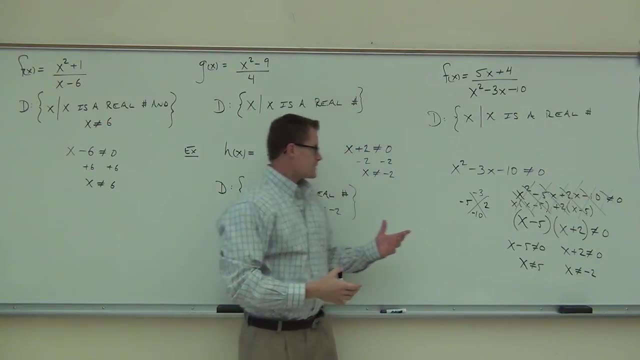 This is now review of our review. so double review, right? How many of you feel okay at the beginning of these points, Solid on that? Okay, Now what we do with that same thing we did with this one. It's only in this case how many points are not going to work. 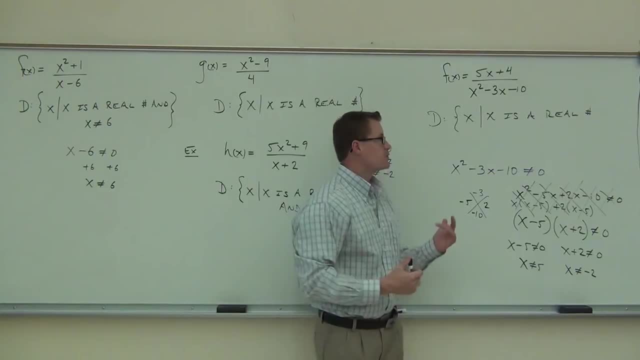 How many values are not going to work in my function? Yeah, In fact, if you plug those in the reason why they don't work, check this out: What's 5 squared 25.. Minus this will be 15.. 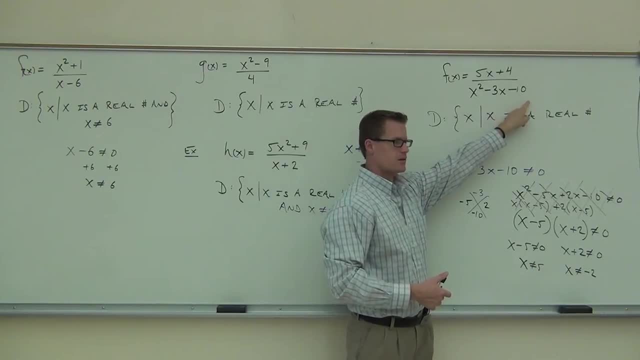 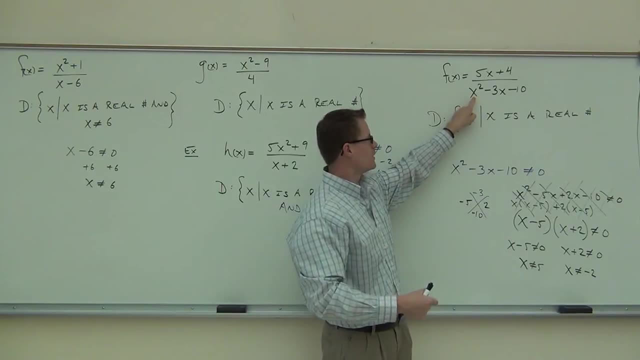 25 minus 15, 10.. And then minus 10? 10.. That's why this one doesn't work. Same thing happens with the negative 2.. You do 4.. Negative 2 squared is 4. You would do plus 6.. 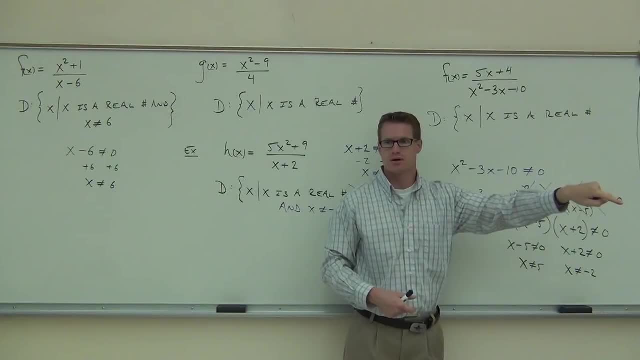 Negative and a negative that's plus 6, that's 10.. Minus 10 is 0. So again that one doesn't work. That's why we have two values that don't satisfy our function. They're undefined. 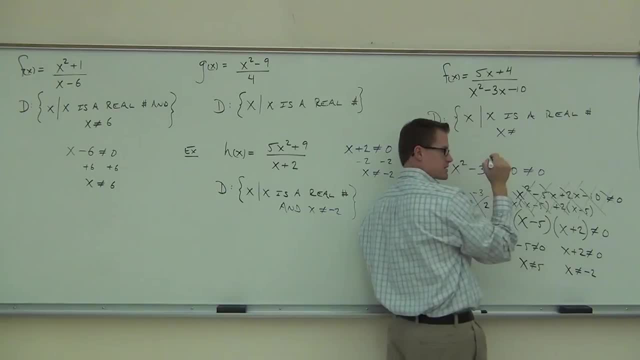 So we'd say x is a real number and x is not equal 5. And you just list them out: x is not equal negative. 2. Close our bracket. That's how you find domain. Do you guys feel okay about finding domain? 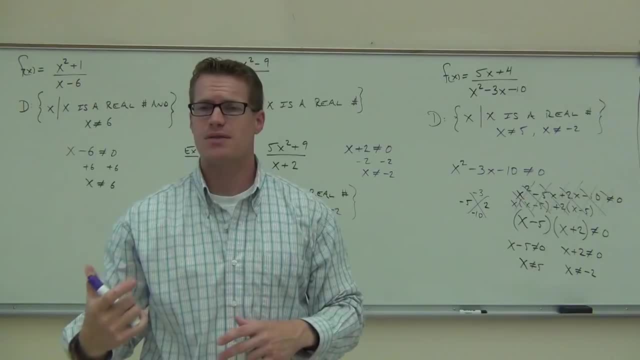 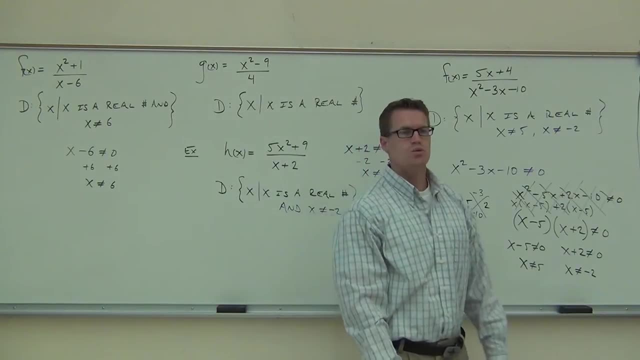 Not sure. if you do, You feel all right with this. Okay, So the whole idea is: set the denominator not equal to 0 and solve it. You might have to factor, You might not. On your test you will have a domain problem. 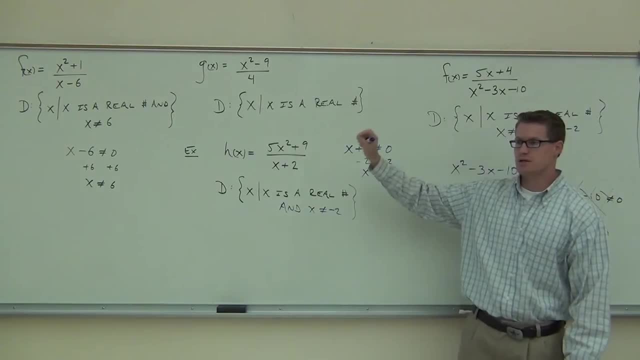 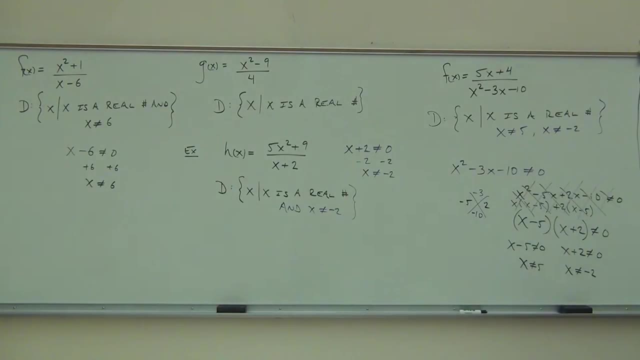 So if you want to write this down, you will have a problem like one of these three. Probably not that one, because there's no word to it, but one of these two on your test. Do you guys have any questions about domain? before we go on, 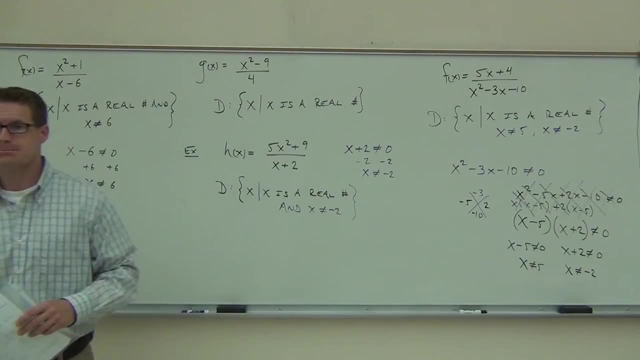 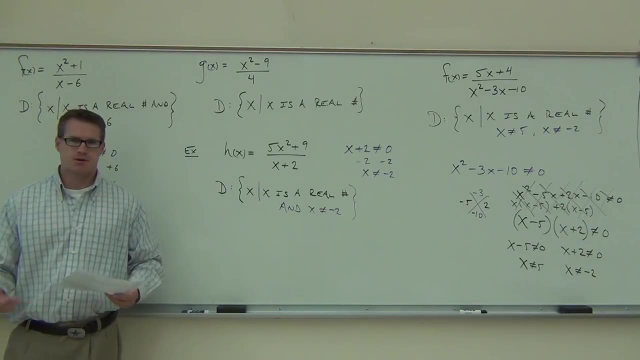 So if it's just a number at the bottom, is it pretty much going to be like. that's it right there. There's no variable on the denominator, right? That means the denominator can't change. If the denominator can't change, yeah, you're good. 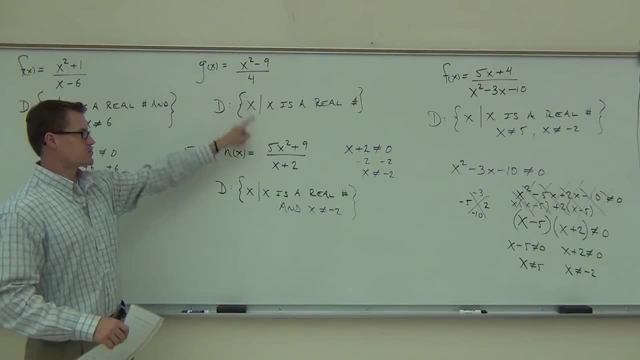 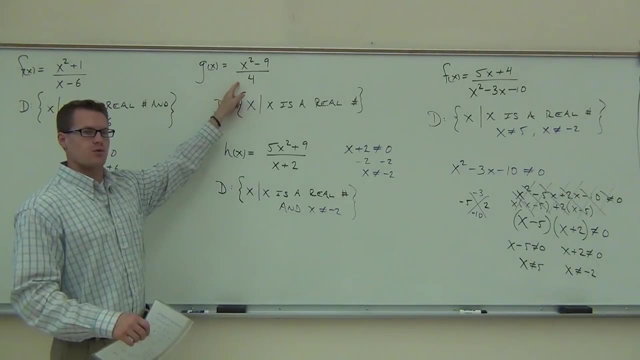 I mean here yeah, Here no, It can't change: Here yeah, Here of course, And here yeah, But this one, that denominator, is never changing from 4.. That means you're going to get all real numbers. 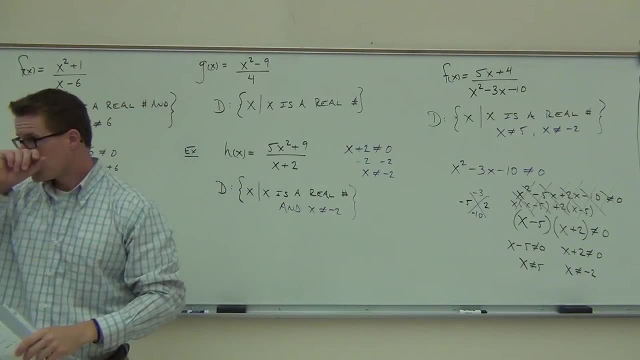 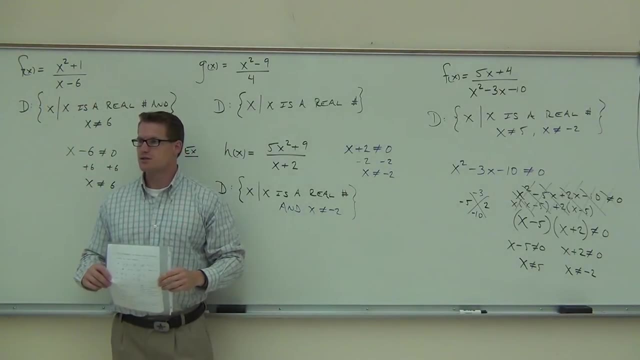 Anything is going to work there. That's a great question. Any other questions: Will we ever think of a case where we'll have 10 to the 0 minus 1 as it's on there- 10 to the 0 minus 1?? 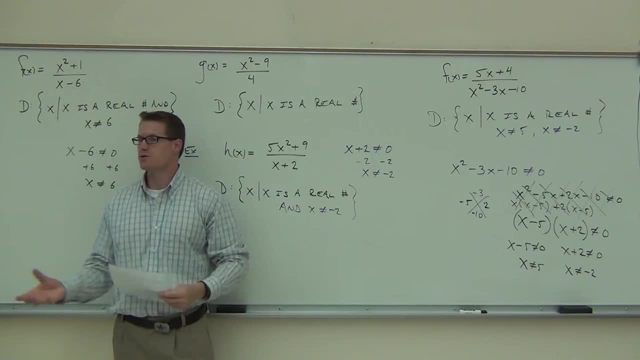 Yeah, No, Well, that inherently wouldn't be a function, right, because it's completely undefined everywhere. So I won't ever give you something like that. So we won't find that for a domain problem. Not for a domain problem. no. 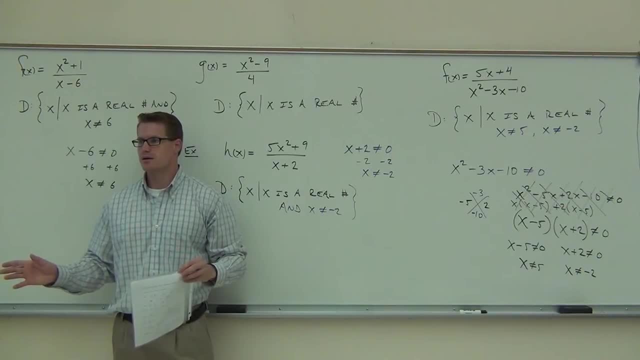 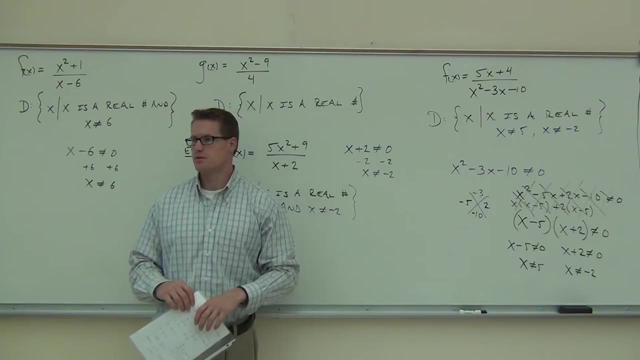 If you do, then you say this function is completely undefined. Okay, It's 0 always, because that wouldn't be changing. Yeah, Like if you had- Well, if you had- 10 to the x minus 1.. Now, we haven't covered exponentials, but if that x ever became 0,. 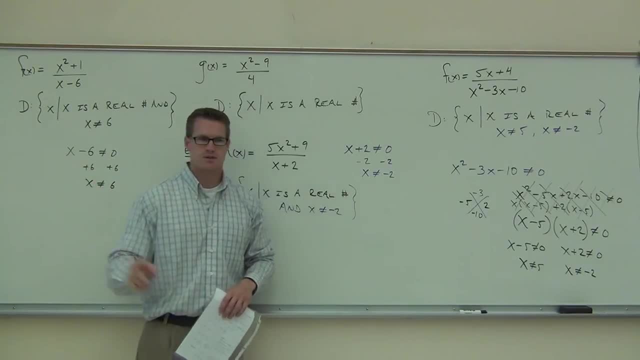 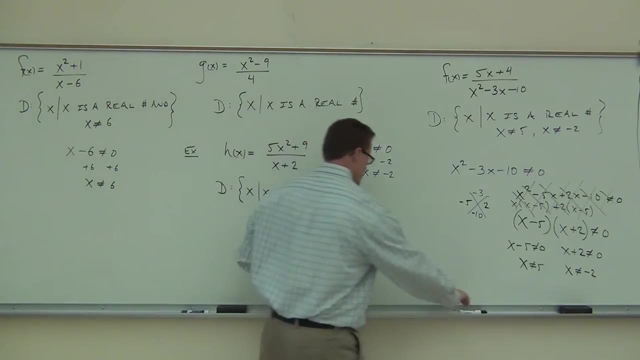 then it would be undefined at 0, but everywhere else would be fine. Okay, That's a good question. Any other questions? Let's go on to simplification. all right, Move away from our domain for a while. We had a bit of it though. 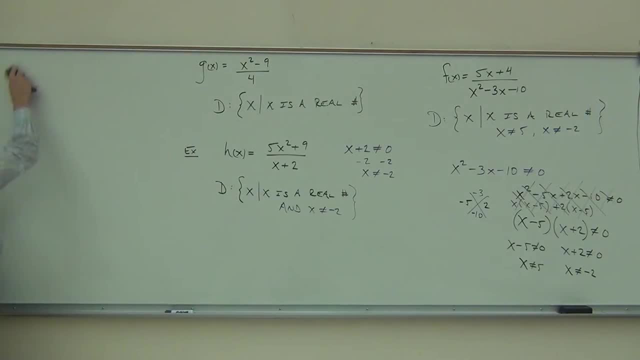 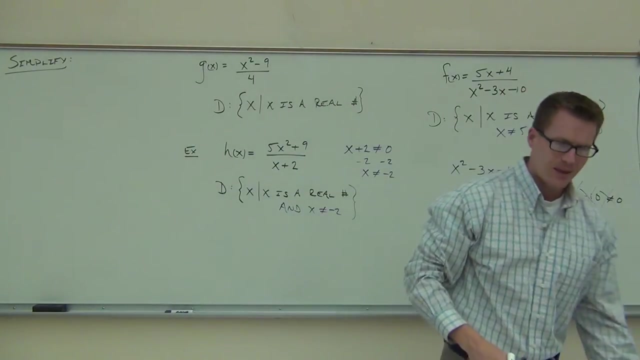 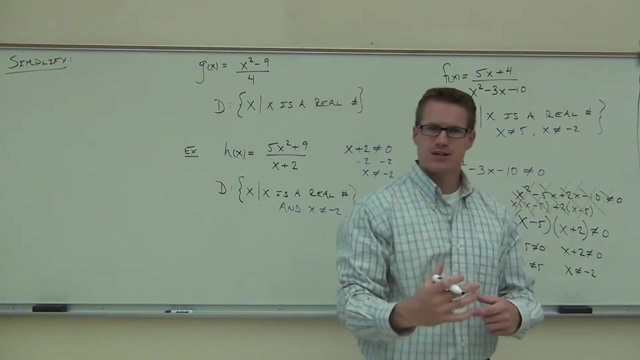 Here we go, Here we go. So we're going to learn how to simplify some rational expressions. Now, because rational expressions really are fractions, just some polynomials. we can simplify them very similarly to fractions. You know, we can simplify fractions, right. 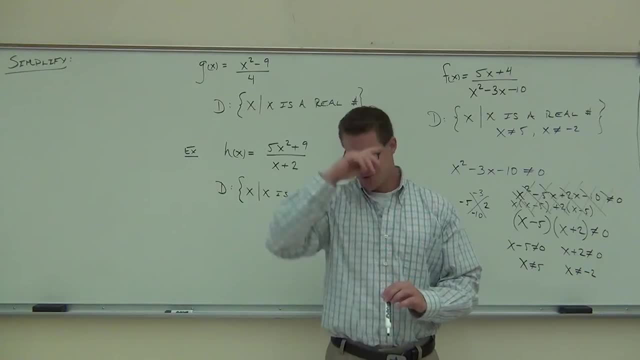 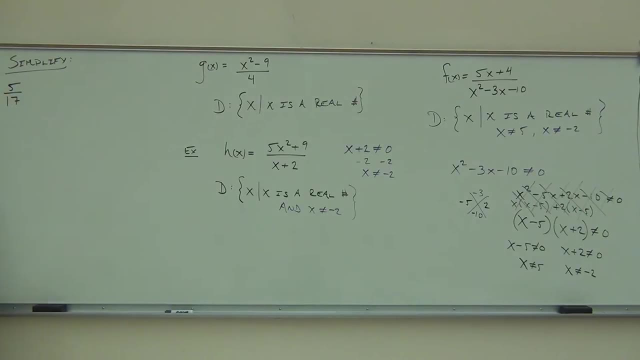 I hope you know We can simplify fractions, right, Yeah, Okay, good, Got that. So you tell me, Can that fraction be simplified? No, No, Okay, That's the right answer. Very good, Can this fraction be simplified? 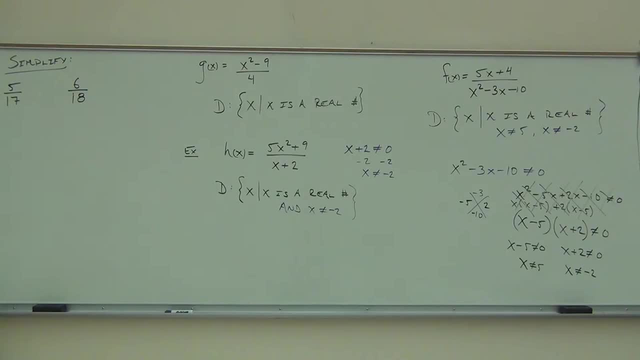 Yes, What's the difference? It can be a fraction. What happens here? that doesn't happen here. Top one goes to the bottom one. Okay, so They don't have a common factor Factor. Yeah, you guys both said it. 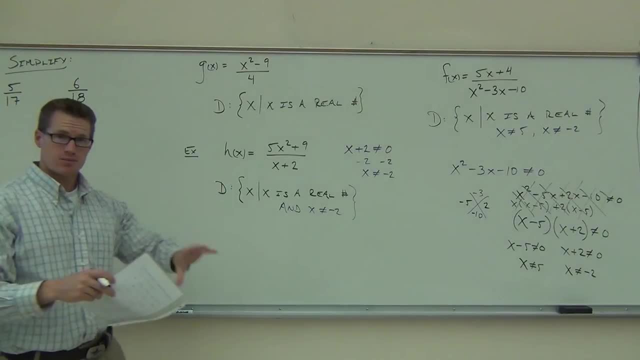 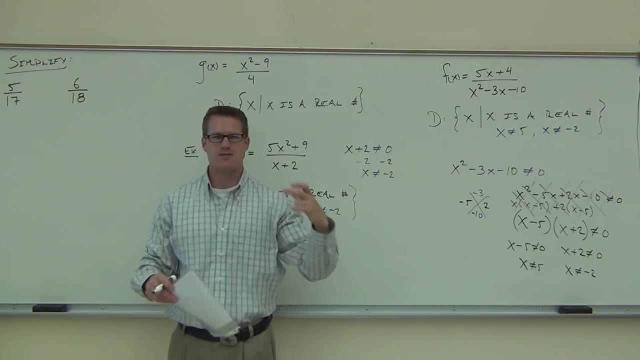 So we're looking for common factors. That's how we simplify fractions. If the numerator and denominator Have common factors, We simplify it. We can simplify that by making a very fancy one out of it. basically, I'll show you that in a second. 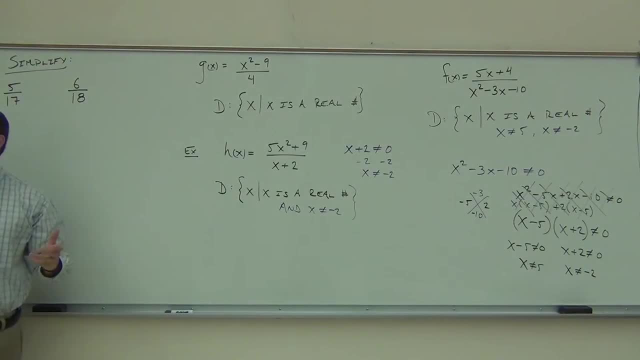 When they don't have common factors, we say it's reduced, It's simplified, and we leave it alone. We're going to simplify our radical, sorry, rational expressions exactly the same way here. So these can be simplified when the top and bottom 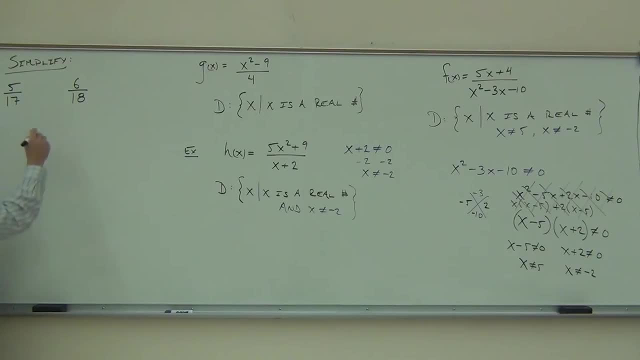 our numerator and denominator have common factors. Okay, Good, Good, Yeah, keep it simple. Yeah, keep it simple, Keep it simple. Yeah, Keep it simple. Guys, we're going to have some common factors and we're going to simplify those. 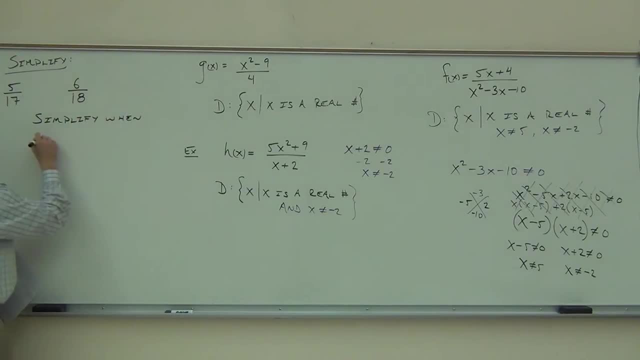 So we're going to simplify. when the numerator and denominator have common. I underlined factors there- Factors, factors, factors. Because that's what we're going to be looking for when we get to our rational expressions. It's factors, By the way. how do we do this? 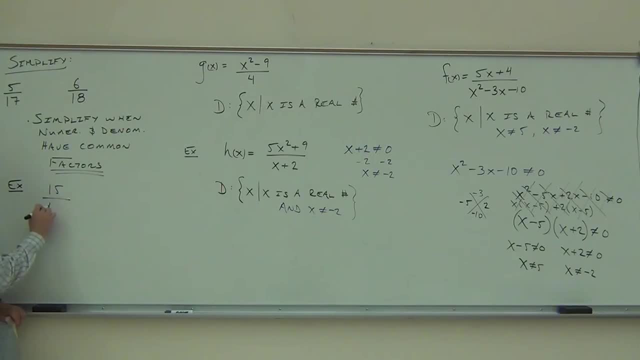 Let me give you another example. Can this one also be simplified? Yes, What is the shared factor here? Five, Five, Hopefully five, Yeah, Five, And the way we actually do this. I know you guys are used to just crossing things out. 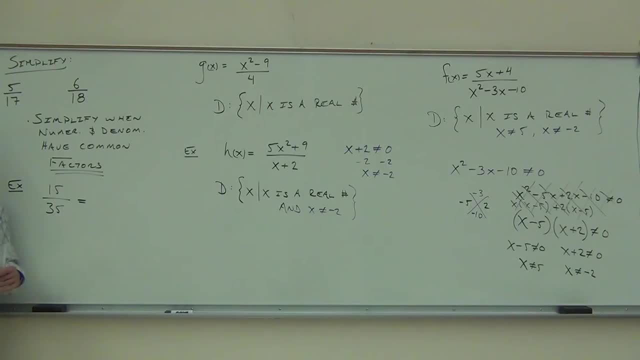 Right, Which is awesome for fractions like this, But really, when you think about this, how you were taught, how to simplify, you were taught. okay, I'm going to write 15 and 35 differently, because I know five goes into both of them. 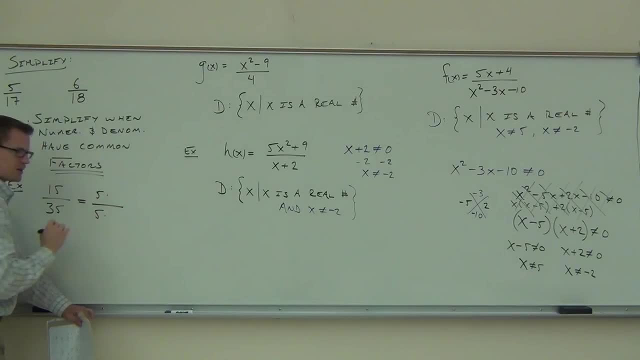 I'm going to write this as five times something and five times something- You with me on that- And we're going to do five times. well, this is a three up here and this is a seven down here, Because our answer is going to be three sevens. 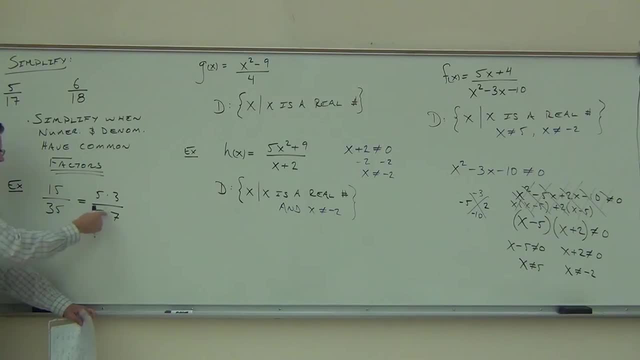 But what we're really doing is we're taking this common factor and splitting it off from our fraction. We're going the opposite direction. We're going the opposite of multiplying fractions, basically, And we're doing five over five times three over seven. You know, you can split up fractions that way. 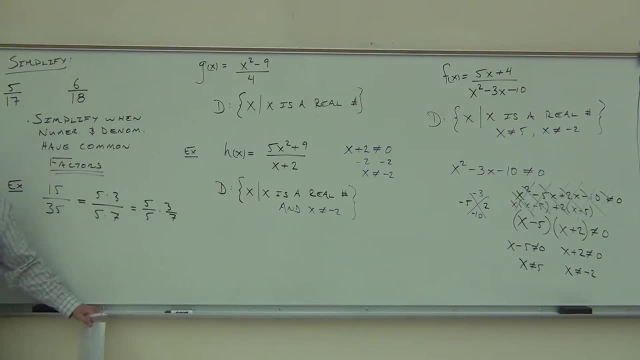 That's possible with multiplication. You go: oh okay, How much is five over five? One? It's a very fancy one. Yeah, Five over five is one. So you have one times three sevens, and we all know that one times anything is just that. 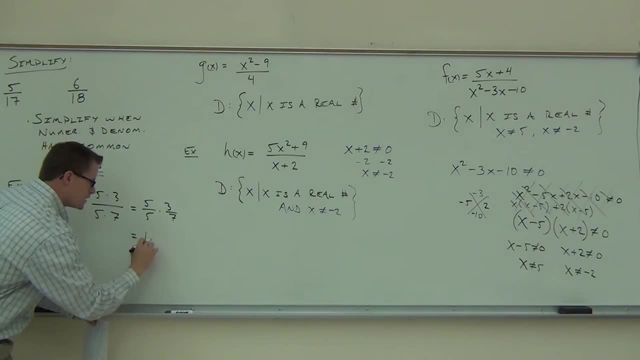 anything, We get three sevens. That's how simplifying fractions actually works. Right, You don't just cross stuff out? Yeah, this is fun, I need to cross stuff out, But we do cross stuff out. typically We don't show all this work. 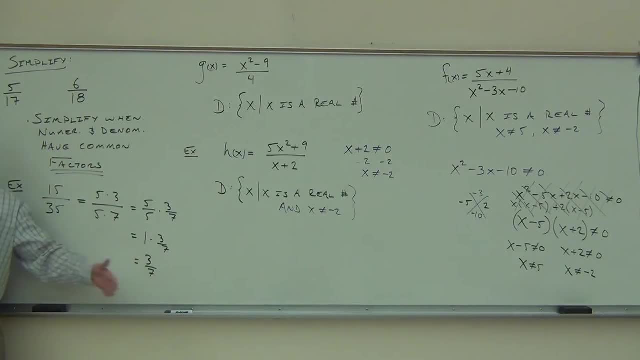 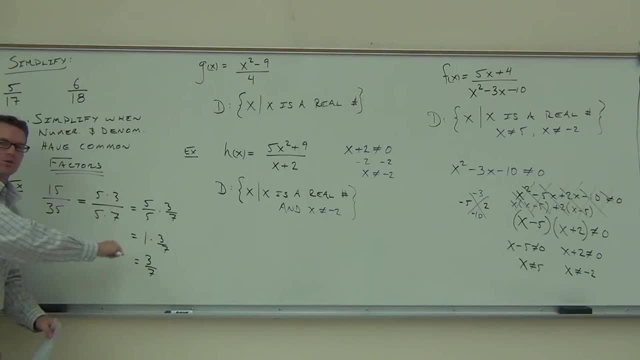 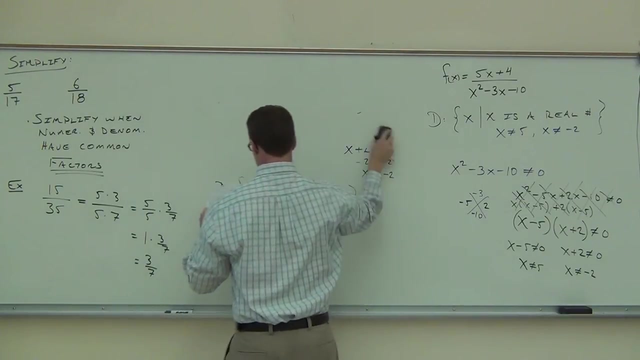 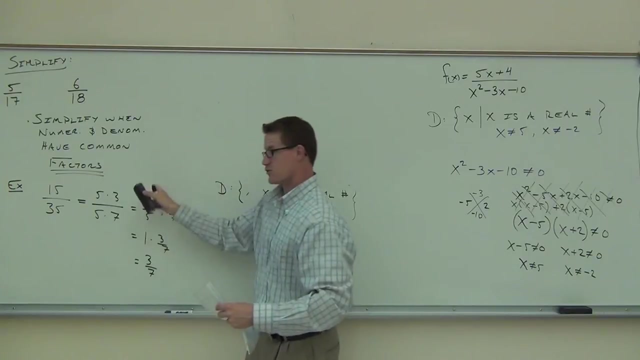 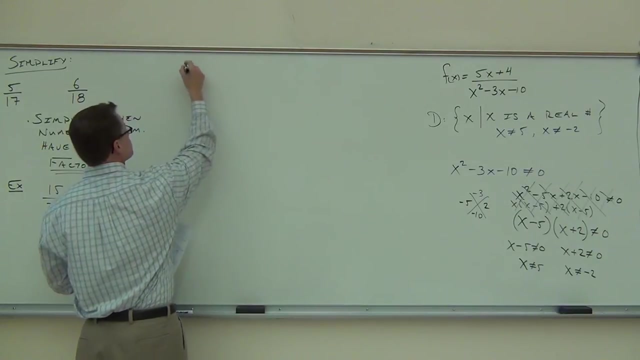 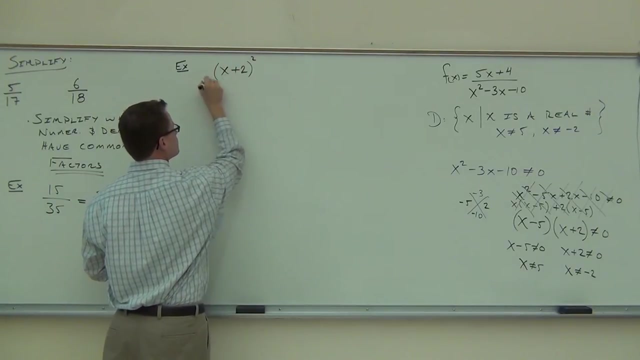 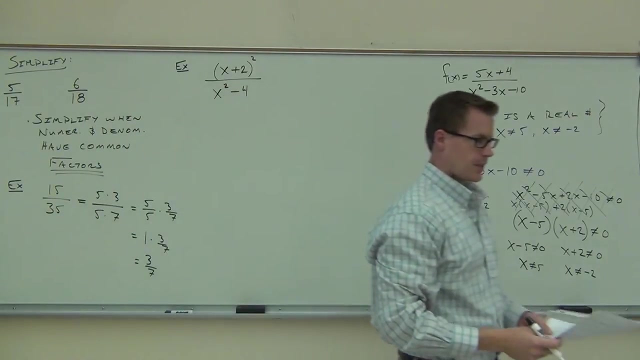 Did you understand this, by the way? Yeah, Okay, So really, we are simplifying by removing factors of one. That's a factor of one here. That's what we're doing. Hey, would you be able to find the domain to that problem? 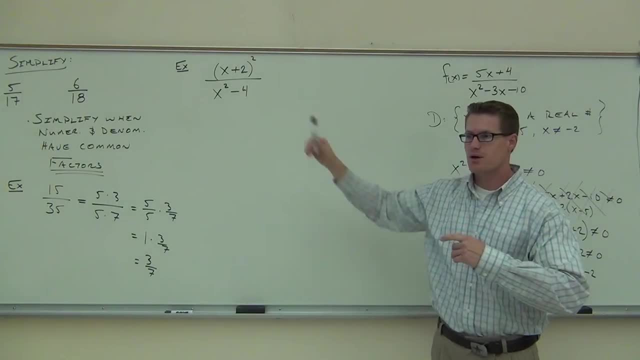 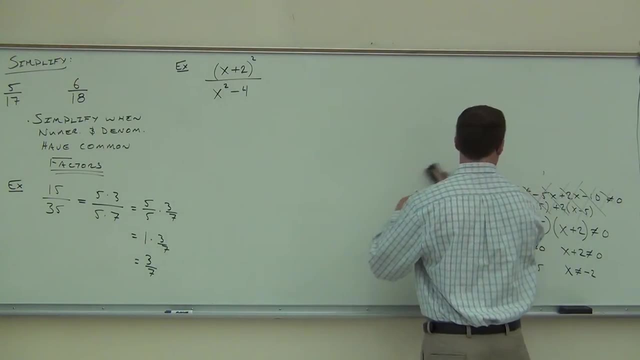 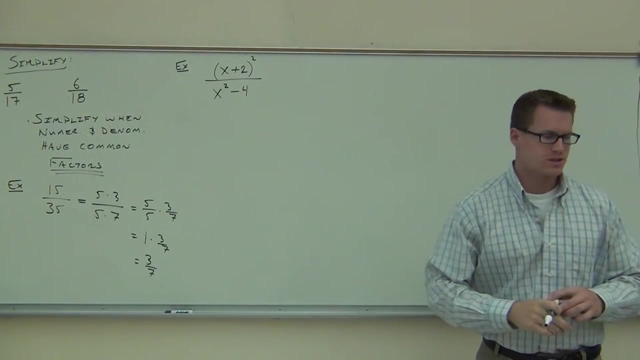 I'm not going to ask you that right now. I just want you to think about it. Would you be able to find the domain to that problem? Think about that. as I'm erasing this over here, Are there one, two or more points that are not going to work in this expression? 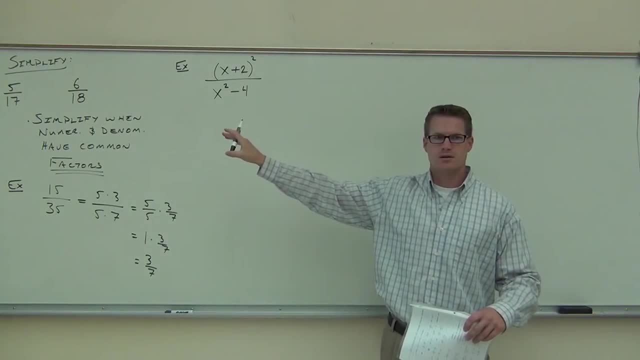 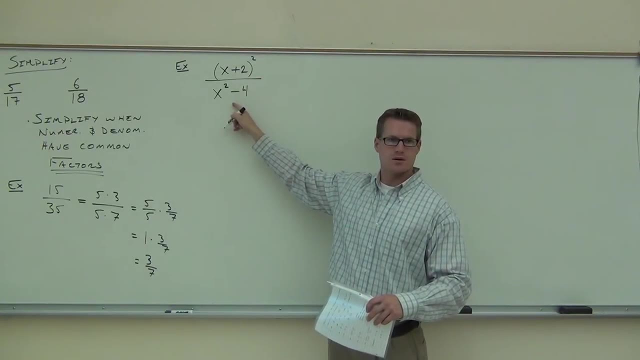 There's more than one. We're looking at the denominator right. We're not looking here, We're looking here. You can plug in what inside the work Two and also negative two, Because when you square that it becomes four as well. 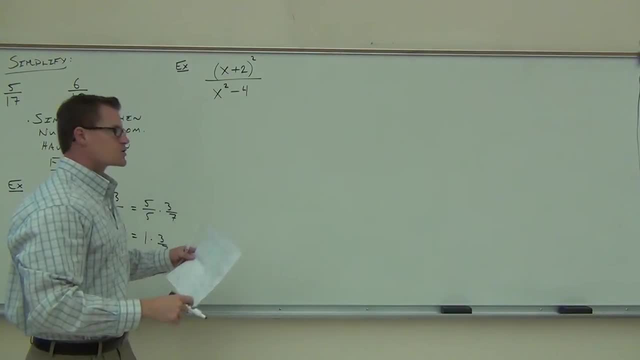 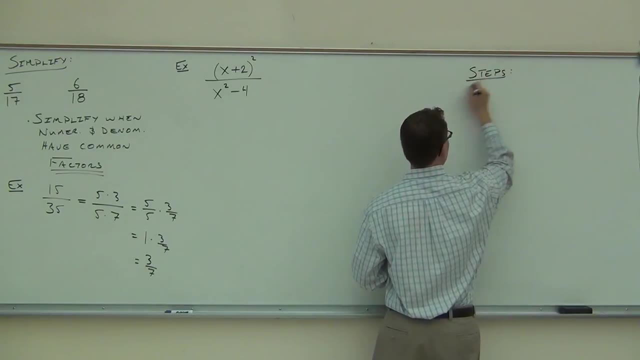 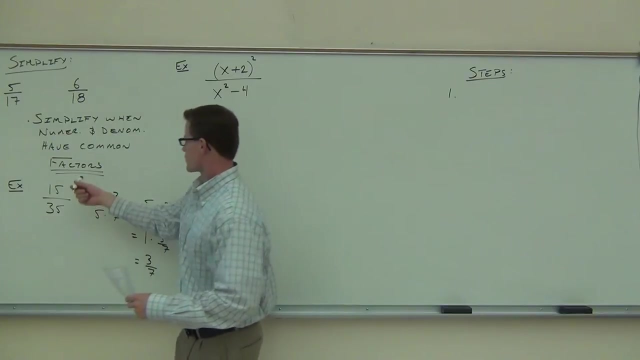 So yeah, that's two. Okay, so here's what we're going to do. I'm going to give you your steps as well, Steps for simplifying your rational expressions. The first thing that you've got to do- and this is why I underlined this word right here- 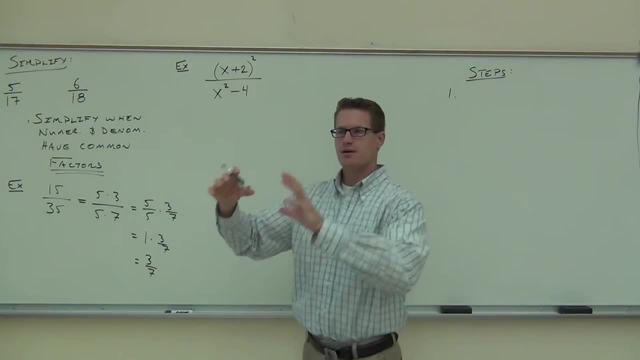 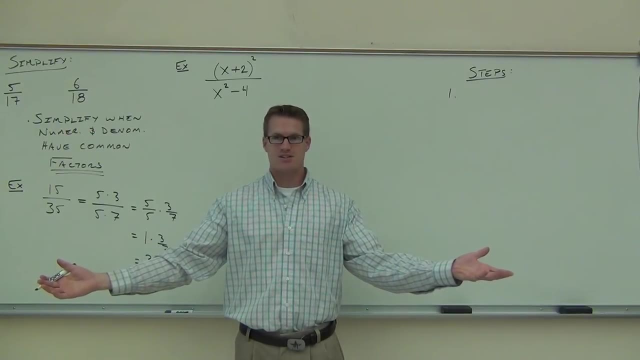 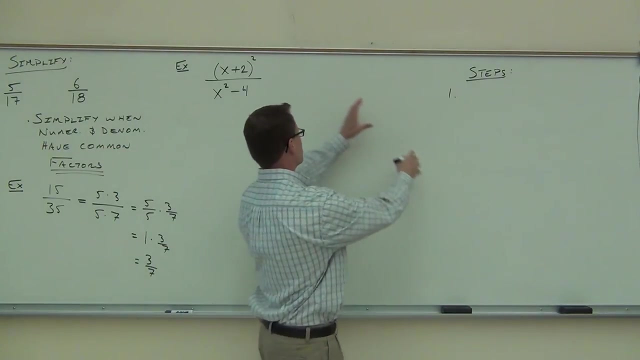 If we're supposed to simplify out common factors, how are we going to do that if our expression is not Finish this sentence? If we're supposed to simplify common factors, how are we supposed to do that if our expression is not completely factored? 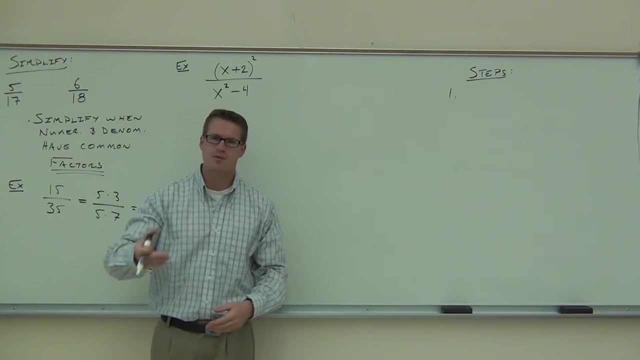 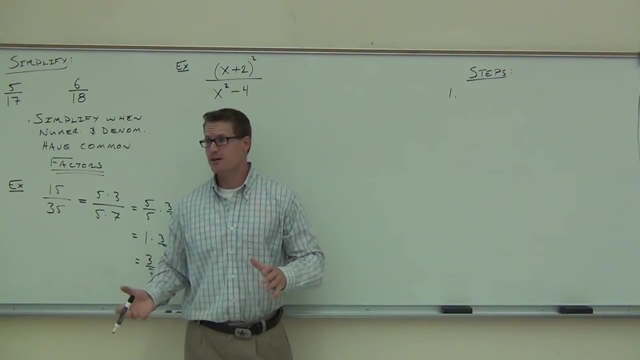 You're going to have to factor that right, Because we're going to try to match up common factors like we did here. We're going to try to match up common factors. The first thing you have to do in order to see common factors is you've got to factor it. 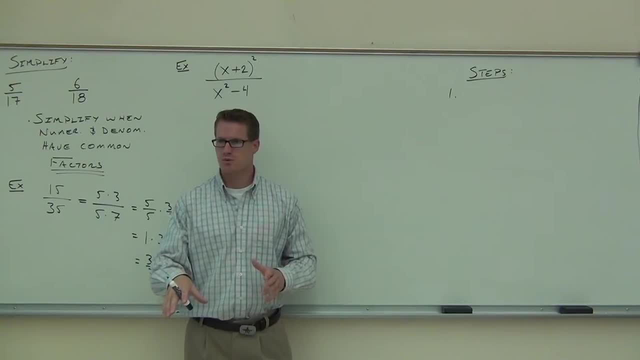 which is why we spent so much darn time factoring in this class, which is why we did the review first. I need to make sure you know how to factor, Otherwise you're going to plummet in this class. You have to know factoring very, very, very well and get it right every single time. 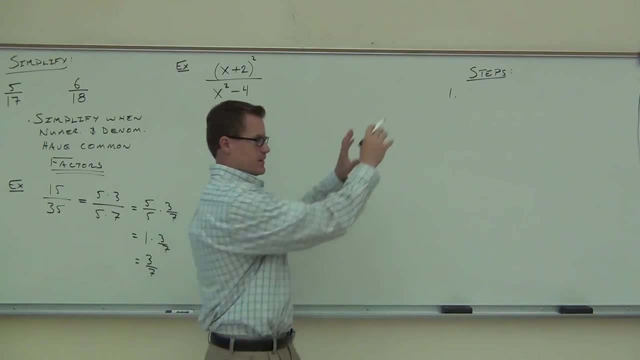 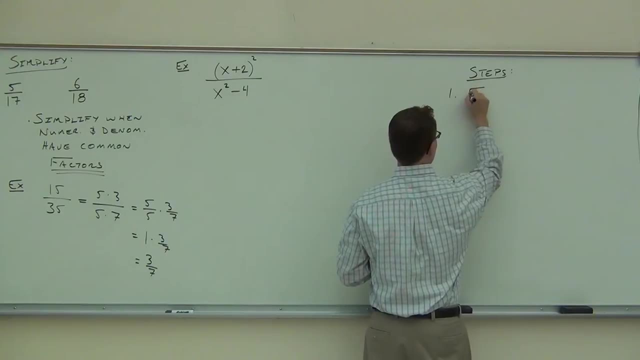 So factoring, that's a huge part of this, And so the first step when we get to Chapter 7, essentially, is factor, And what I mean is factor, both the numerator and the denominator, completely. So let's look at it one more time. 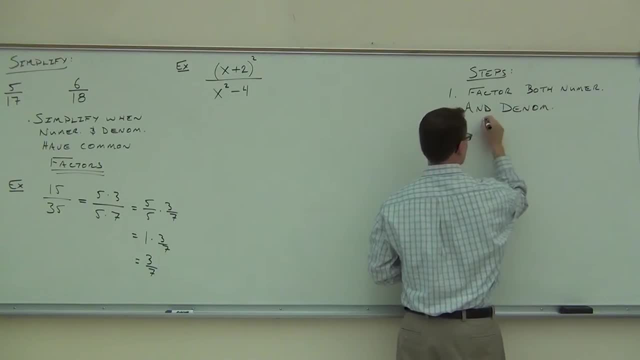 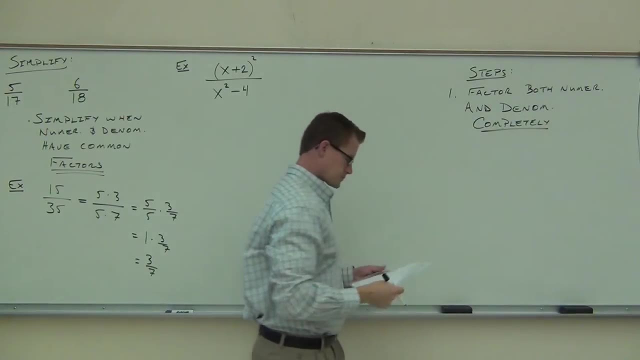 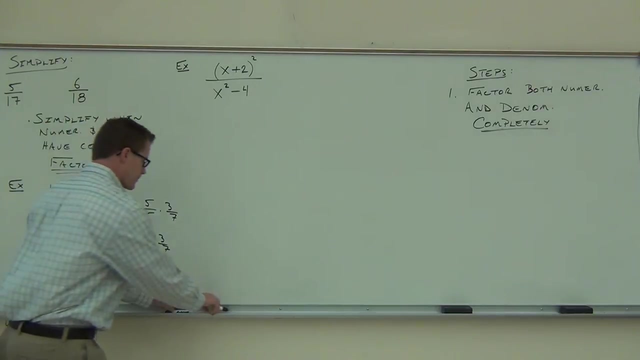 We do this when the denominator is the numerator. If we go back on the numerator, we'd say that the denominator is X plus 2 squared. So let's do that together. OK, I'd like to factor this thing. Let's look at the numerator. 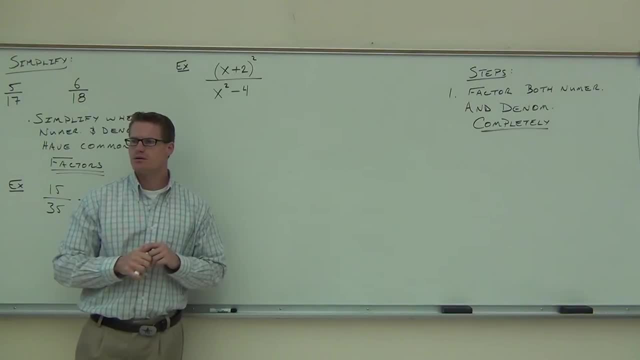 Now the numerator is X plus 2 squared. Can I factor that at all? I don't mean distribute, That's not what I mean. I mean make it even more simpler. I could do that. I could separate x plus 2 times x plus 2, that's possible, I can do. 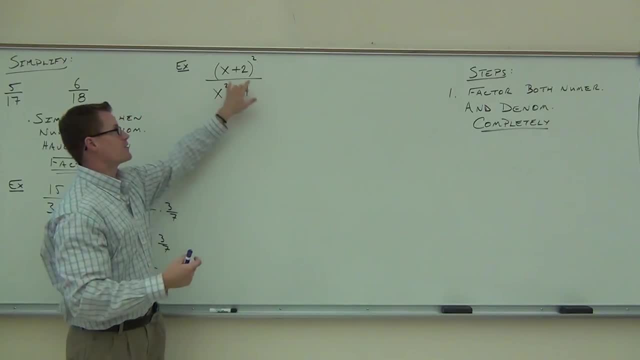 that, or you can leave it alone. either way is fine. What I mean is: can I factor the x plus 2 anymore? No, No, It's two terms, right? It's not a difference of squares, it's not a sum of cubes. it's not a difference of cubes. 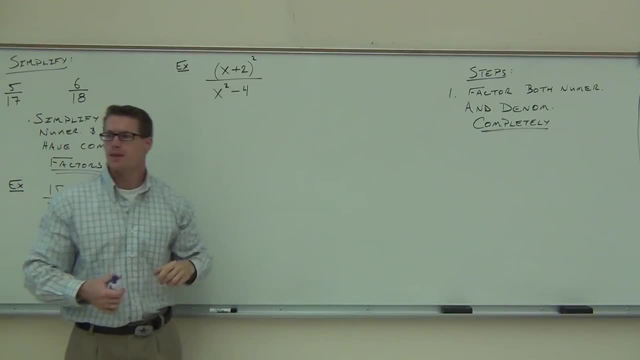 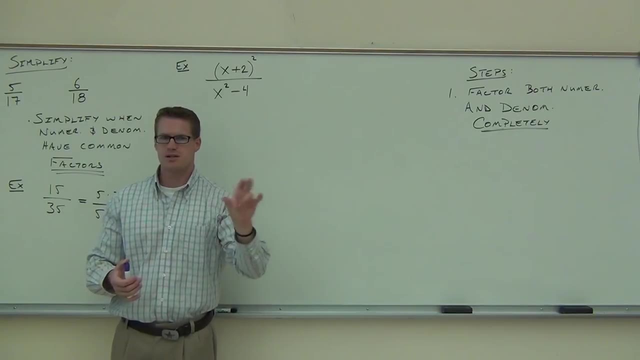 it doesn't have a ratio common factor. I'm done with that one. Let's look at the denominator. Can I factor the denominator? Is there a GCF? You look at that first. No, GCF is something that divides both terms. is there that? 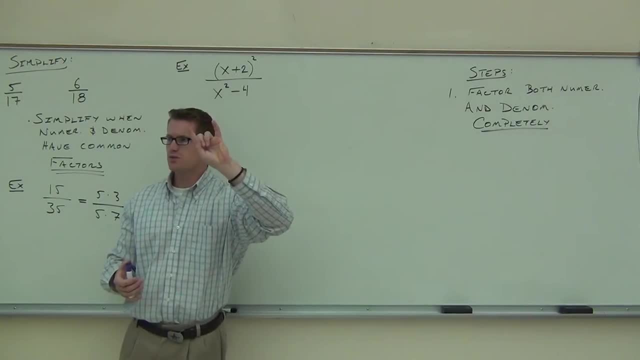 No, It has two terms. The thing you check for two terms. is it a sum of cubes, a difference of cubes or a difference of squares? This is one of those three. which is this one? A difference of squares? Definitely a difference of squares. I hope you're seeing the difference of squares really. 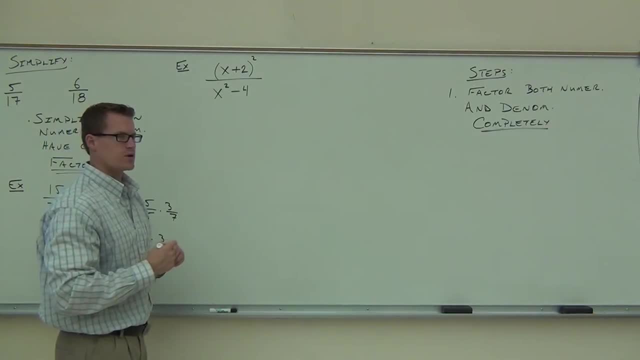 easily on this. I don't know if we've factored this particular one or not, but we're going to have the x plus 2 squared on the bottom. you need to know that a difference of squares is a sum of cubes. 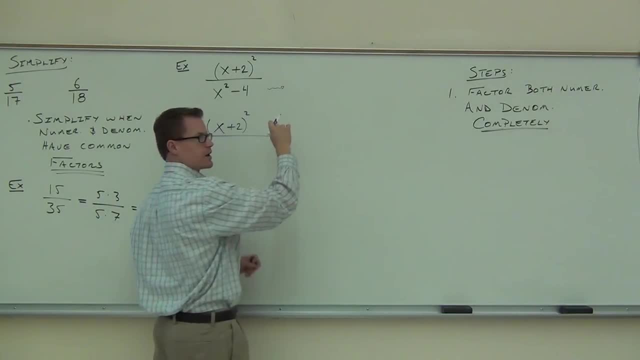 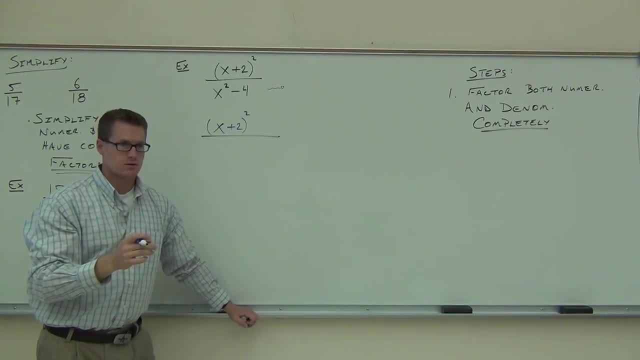 Whenever you can write this as x squared. and how am I going to write the 4? To make it look like a difference of squares: 2 squared, 2 squared- very good, So this could be written as x squared minus 2 squared, and we found out a way that we 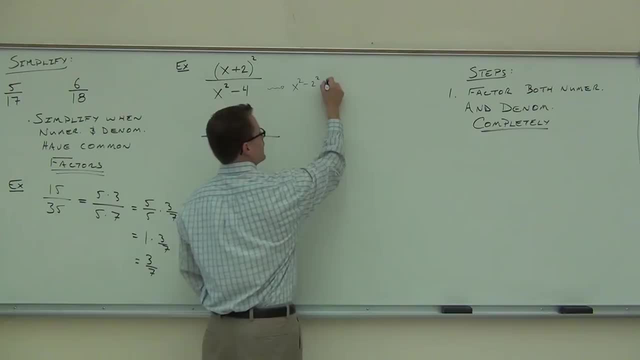 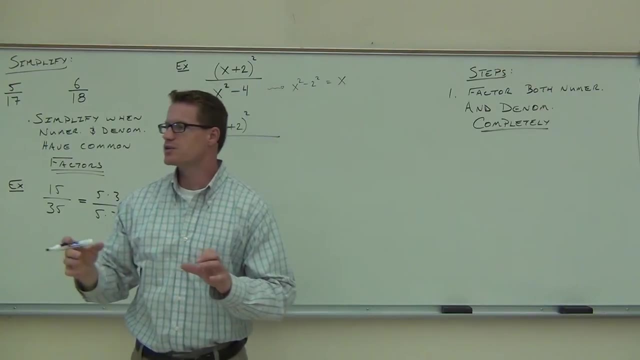 can factor this every single time, it's not a problem. We factor this as x. a lot of people get confused. they put x minus 4, x plus 4, that's not it. that's not it, folks. It's going to be x minus 2 and x plus 2, that's how you multiply and you get that 4.. 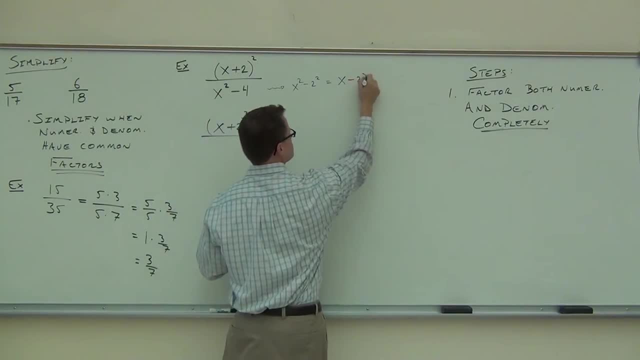 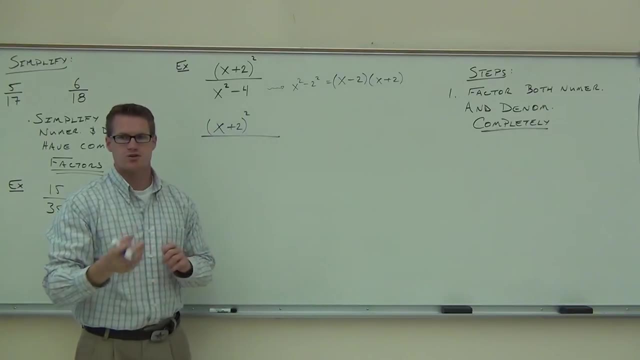 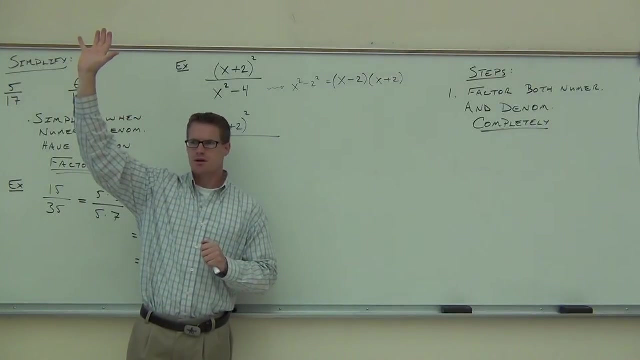 You with me on this. So we're going to do x minus 2, remember: same sign, different sign. that's how you cancel out those middle terms when you distribute again, Just by show of hands. how many people are okay with the difference of squares? 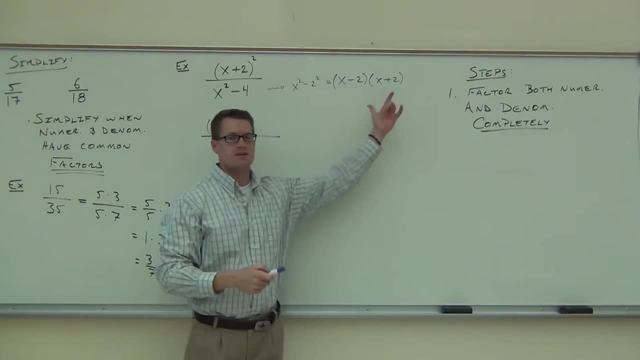 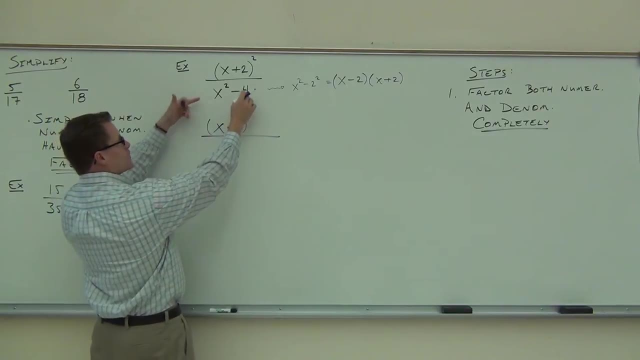 Good, very good. If you're still a little bit like, how in the world are you getting this? come and see me, Or refresh your memory by looking at that video. the very first time I know that x squared minus 4, and you're going to be able to do this without this step. 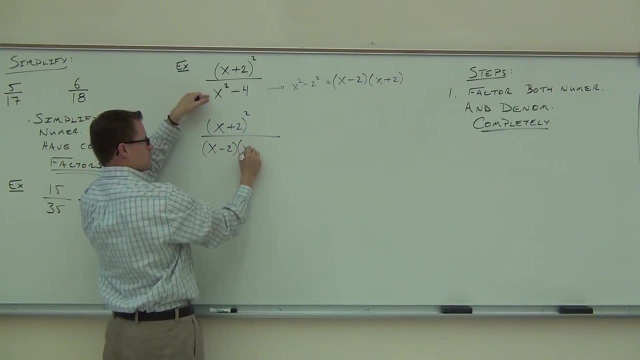 after a while is x minus 2,, x plus 2.. We can double check it: x squared plus 2x minus 2x. that simplifies to 0, minus 4, and that's exactly what we have here. 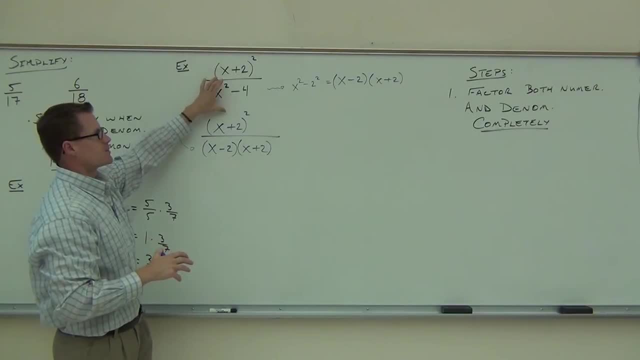 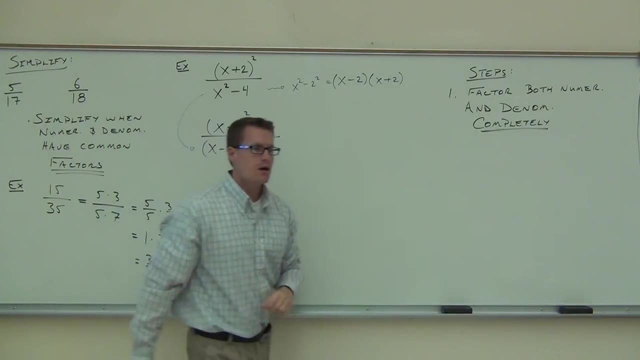 So the very first step is we're going to factor the numerator and denominator completely. This one was done. This one was the difference of squares. we have that right here. nod your head if you're okay, Okay, good. The second and last step is what we're going to do now is we're going to cross out. we're. 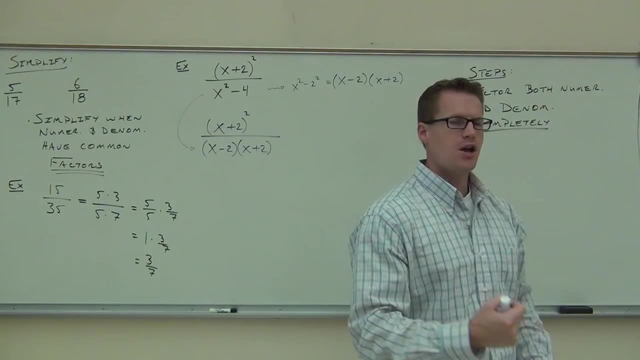 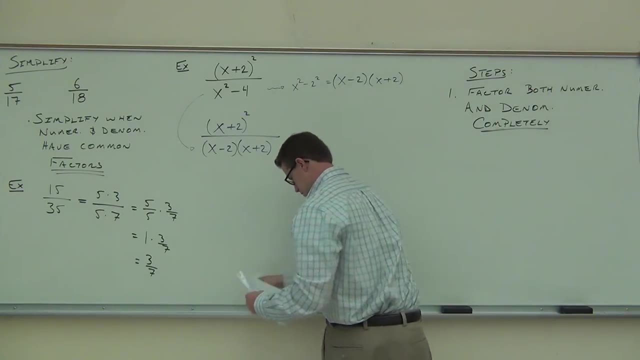 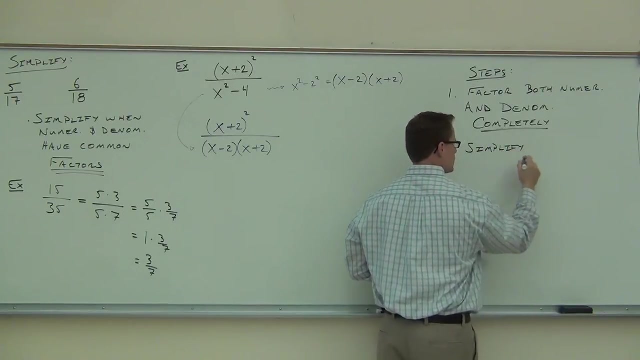 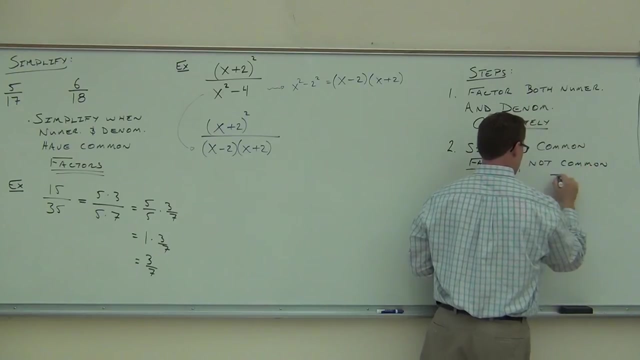 going to simplify out any common factors, not common terms. common factors. I'll show you the difference in just a second, but write this down. I'm going to just sit down. You're going to simplify, Okay. Okay, Not common terms. 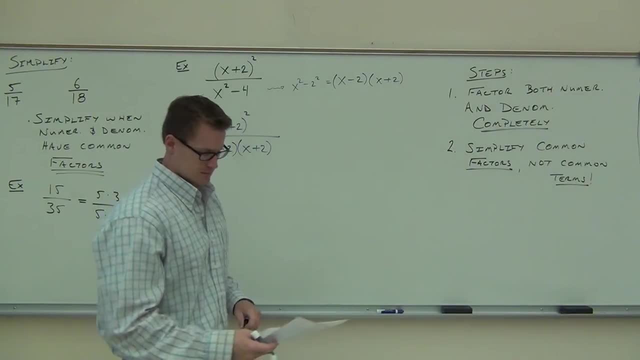 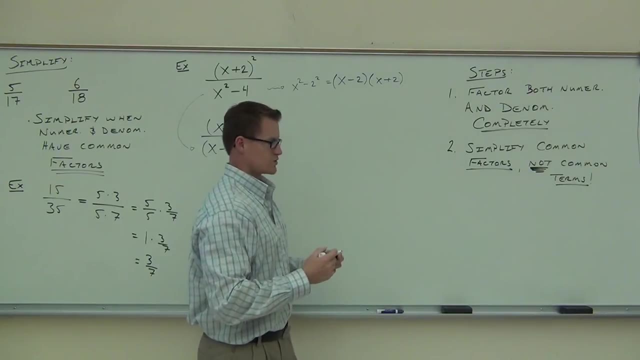 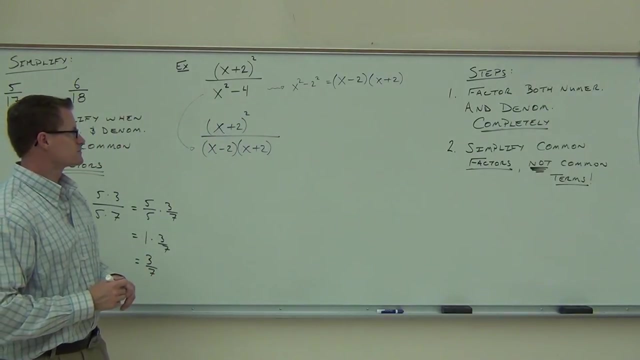 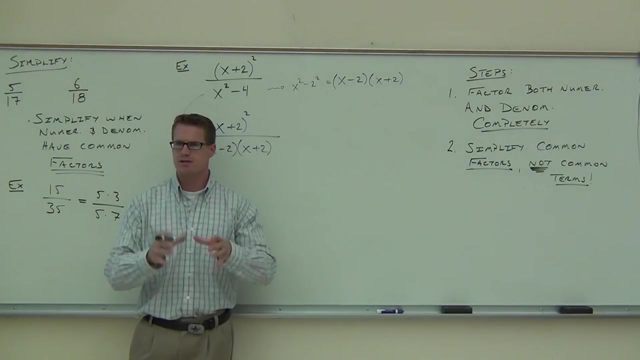 Okay, Common. Okay, All right, Common. So let's do this thing. Do you see any common factors up here? Things that are exactly the same on both the numerator and denominator. that are factors. Factors are things that are multiplied together. 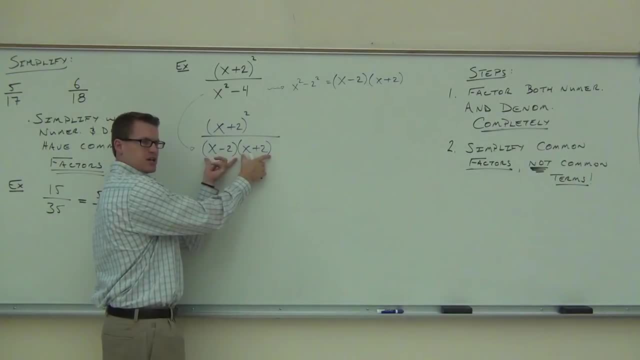 So multiply together. So this right here and this right here, these big pieces notice how they're being multiplied. Those are factors. What you can do, you can simplify all of a factor or nothing at all. You can't go through and simplify parts. 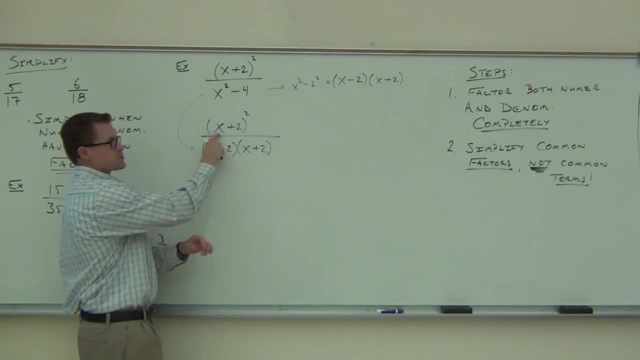 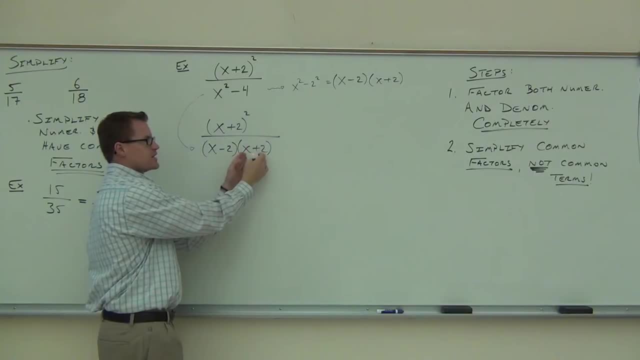 What you can never, ever, ever do is factor something or simplify something that's connected by an addition or subtraction, because that is a term. So what you couldn't do is cross out the twos. You can't do that. Those are terms. 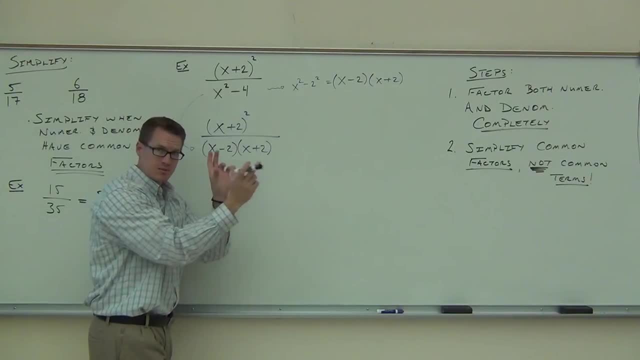 Those are not factors. Factors are pieces that are big pieces, typically, that are multiplied together, Not your head. You okay with that, Are you sure? Shake your head if you're not. Okay, So do we have something? that's exactly the same. 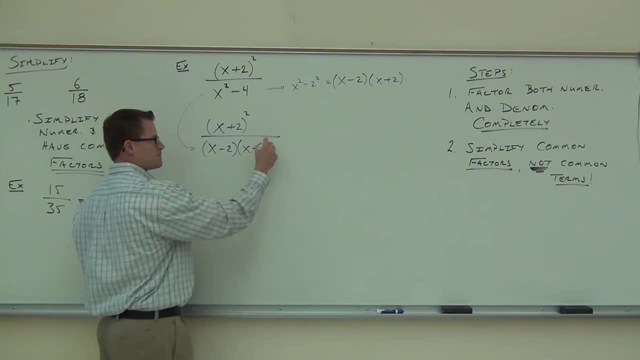 Two similar factors. We have one of them here. Now, if you wrote this as two different ones, that's fine. also, That doesn't really matter. We can simplify this out just like we did. the five: That one's gone. Are both of these gone? 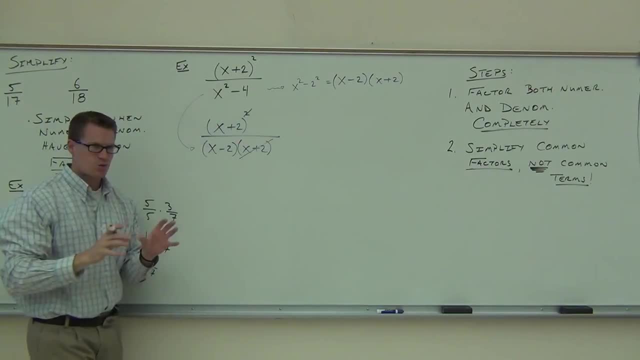 Just one. So I'm just going to simplify out that squared portion of it. That's leaving me one x plus two. Oh, how many times do you think that would happen in a row? That's like a quarter, and it landed on edge. 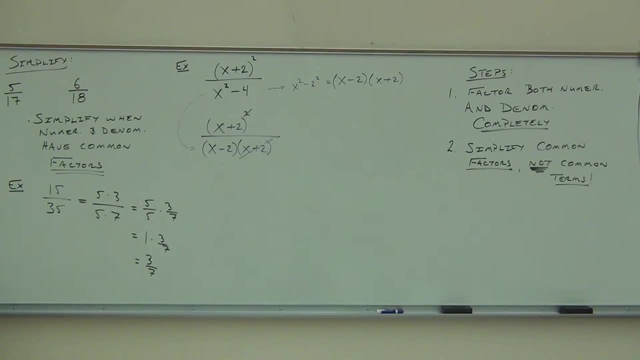 Okay, So do you all agree that there's an x plus two left on our numerator? What's left on our denominator? The important question for you. Can I simplify these x's? No, No, No, No, No, No. 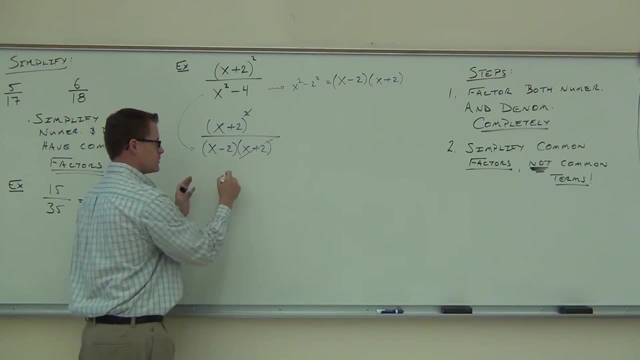 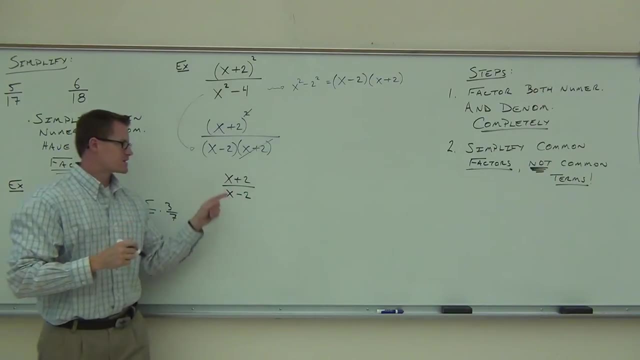 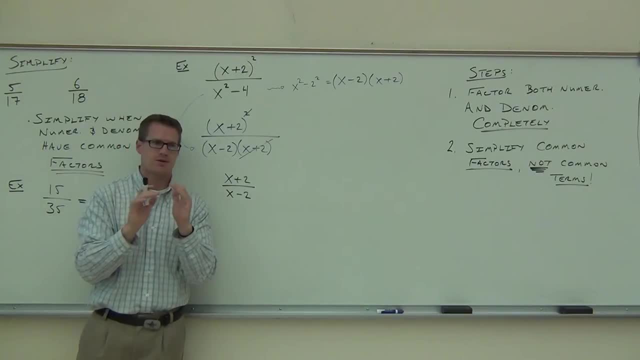 They're not factors. Factors will be multiplied. Typically for us right now, they're in parentheses or they're in the beginning of our problems. All right, They're not included within our parentheses. That would be terms. We're completely simplified there. 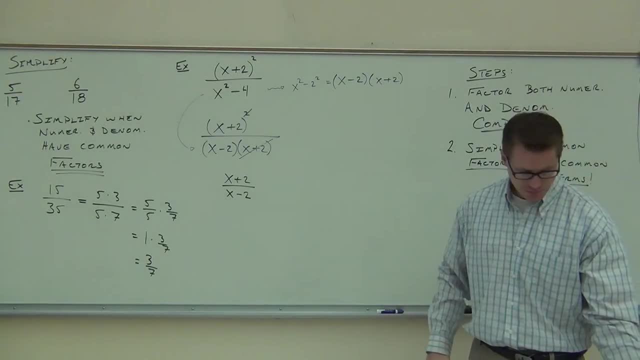 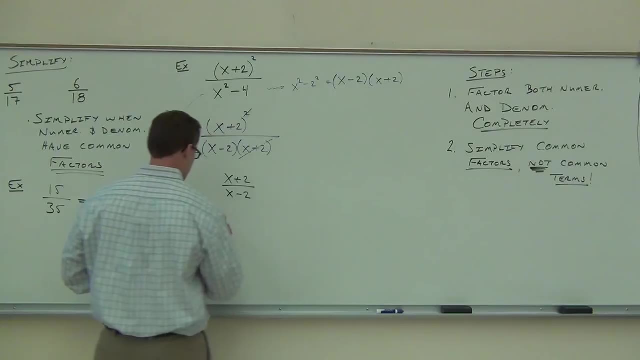 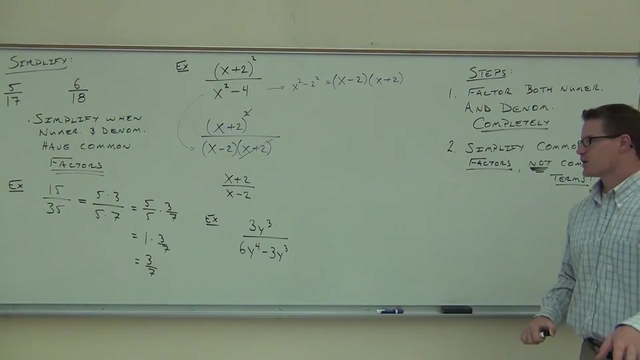 X plus two over x minus two. Let's try a few more, all right? Okay, right off the bat. I've got a question for you. Would it be okay to simplify the 3y cubed with this 3y cubed? 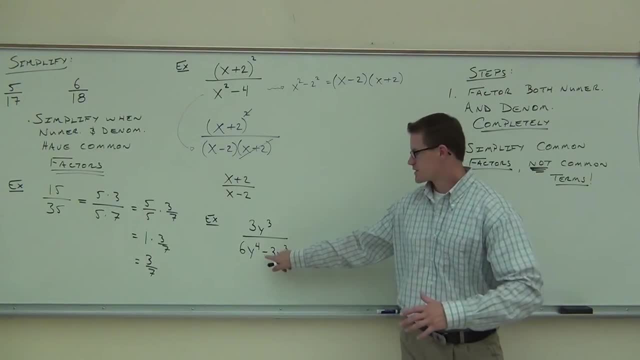 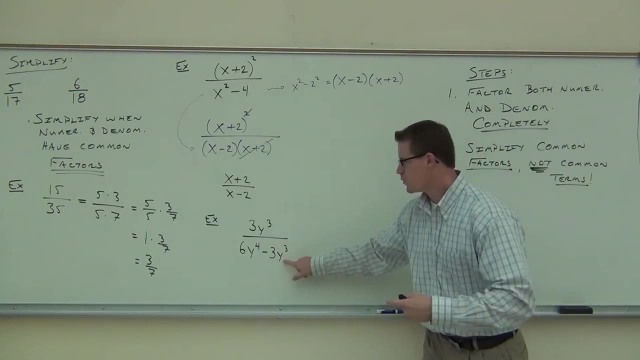 Is that okay or not? What do you think? Clearly no, No, no, no. This has a subtraction right in front of it, but there's no way we can simplify that We can't even do. look at the board. we can't even do. the y cubed and the y cubed, right. 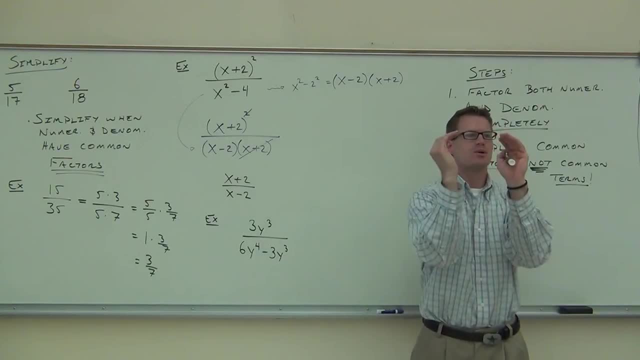 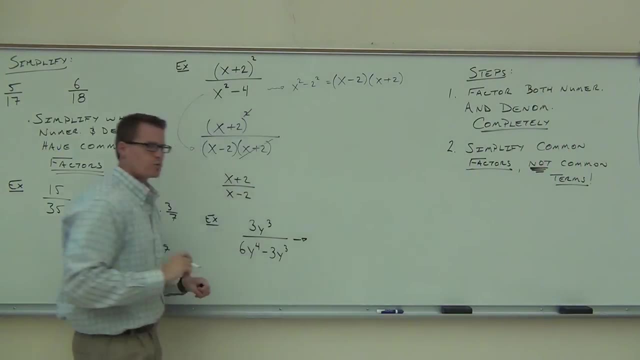 Because this piece still has that subtraction right there. It's got to be completely multiplied. so everything or nothing. That's the idea. So what we're going to try to do is factor this thing Does the numerator factor Numerator. numerator is how many terms? 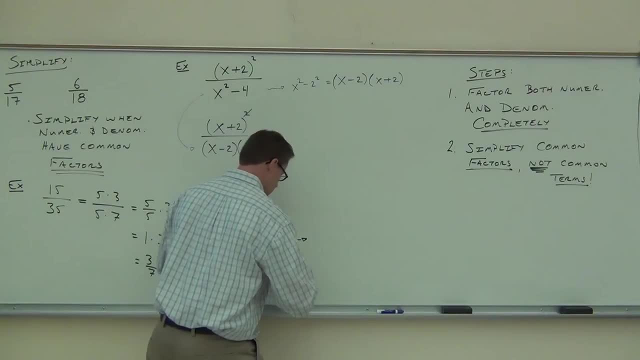 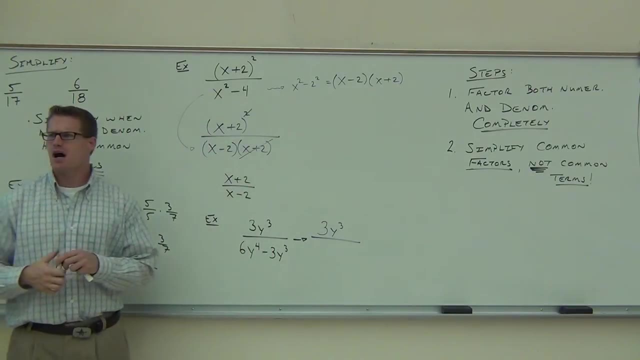 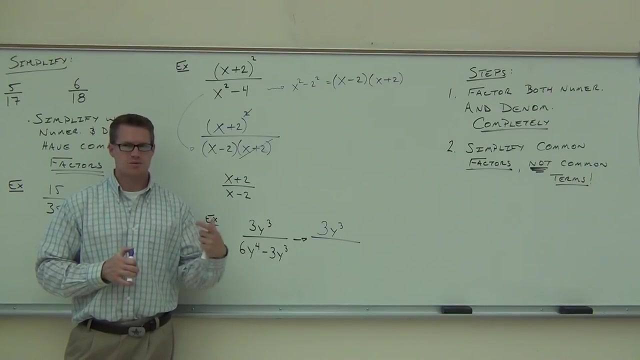 Can't really factor one term. We're going to leave that alone. How about the denominator? Does the denominator factor? Yes, Sure, That actually has. what's that called? again, when you have something similar to both terms, You say that. say it louder. 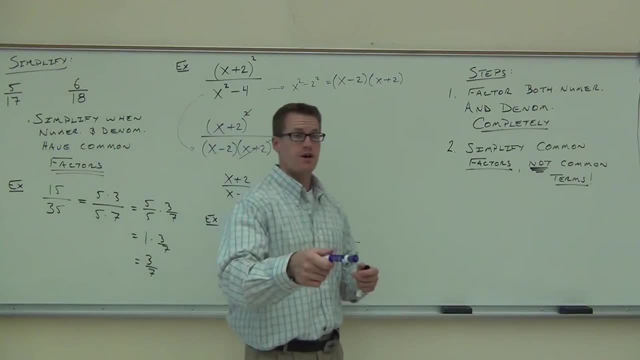 That's right. Yeah, Greatest common factor or the GCF? this has one, So let's factor out the GCF. Let's look carefully at the denominator. What's the denominator Three? What's the number that goes in both these terms? 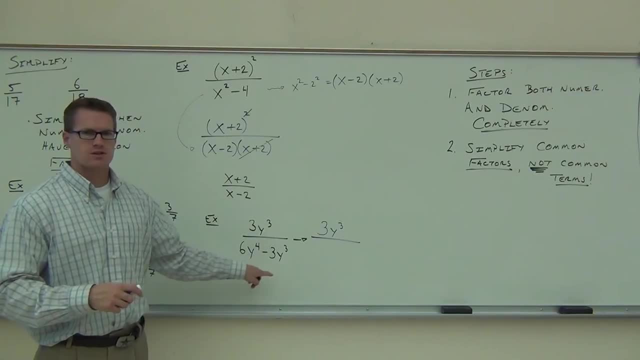 Three. How about the large variable that's common to both Y squared cubed? So we're going to factor out three y cubed. Remember factor. and we're creating parentheses. This should be like old news to you guys, I hope. 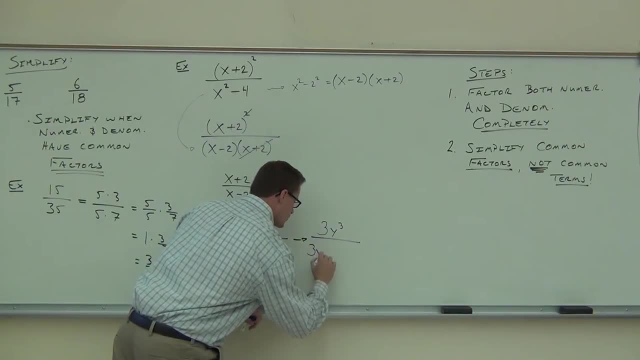 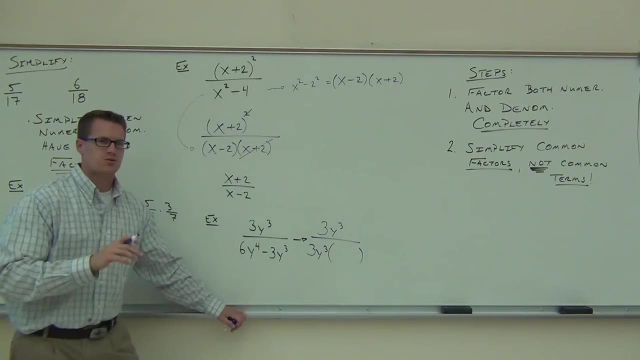 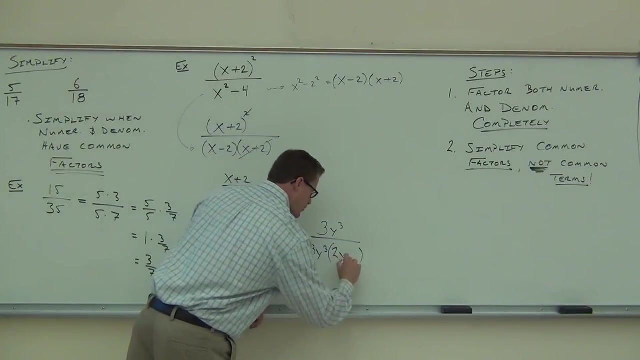 If you factor out three y cubed from our first term- do this on the side, if you want to, or do it in your head- this is how much? Two y Two y, Two y Good, And then we'll have a minus. how much? 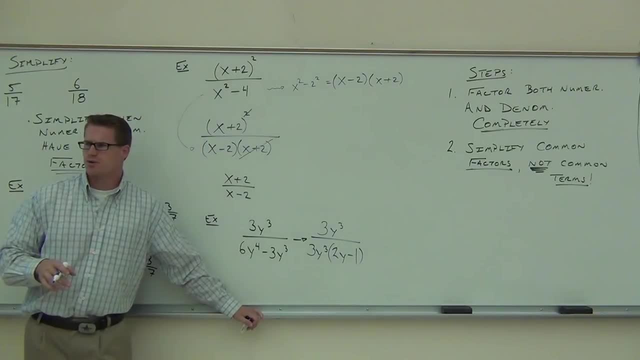 One One. Very good. Are you okay on getting the two y minus one folks? Mm-hmm. Good, So we factor out three y squared or three y cubed. I'm sorry, we're going to get the. 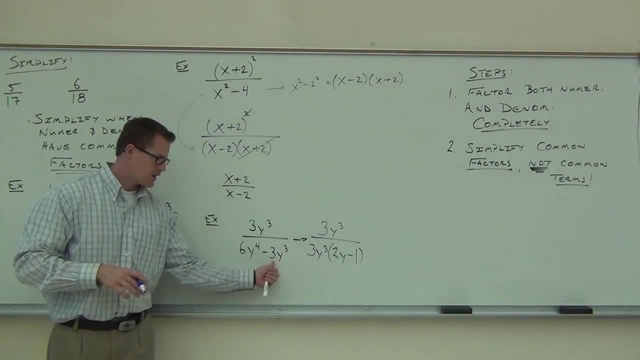 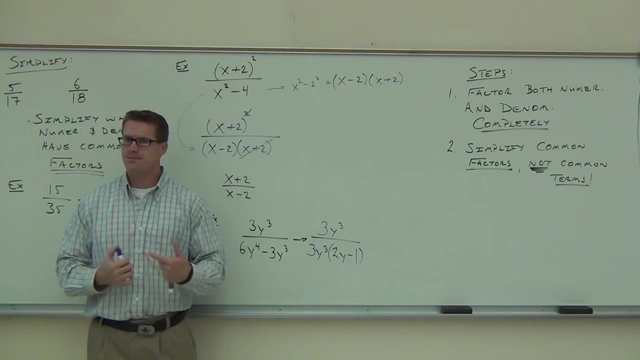 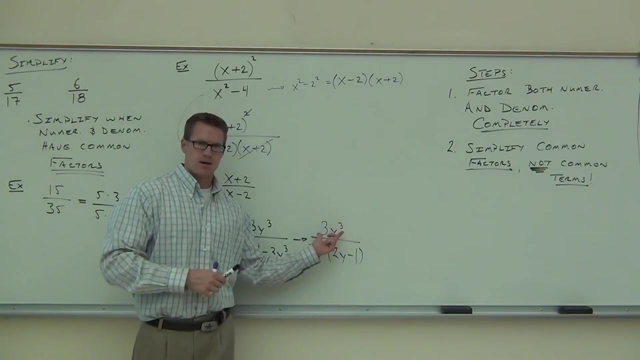 two, y, we're going to get the minus one, and now we're going to look for any common factors on the numerator and denominator. Do we have any common factors on the numerator and denominator? Three, Three, Same thing so far, One. 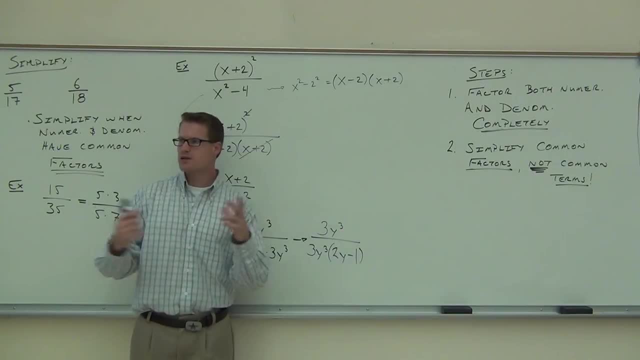 Two, Two, three. We're going to try this later because, since we have too many mathemploids at the bottom of our dialog box, we'll have to go multiple carriers and you'll have a good idea about what they mean, Uh-huh. 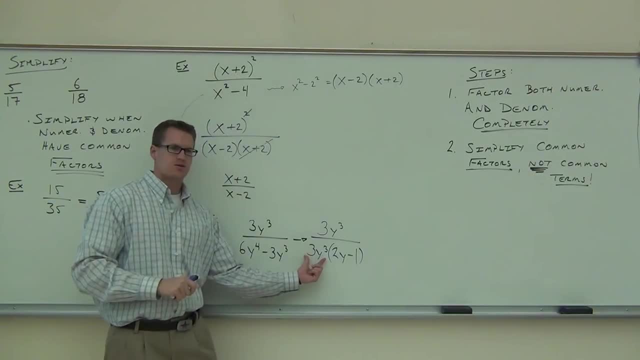 We're just going to grab our question now, make those quiz and just put them in here, and then we're going to do a Hazard's adalah. All right, You picked the, which You can say Instagram, you can use Facebook, you can use Twitter, you can either use WhatsApp. 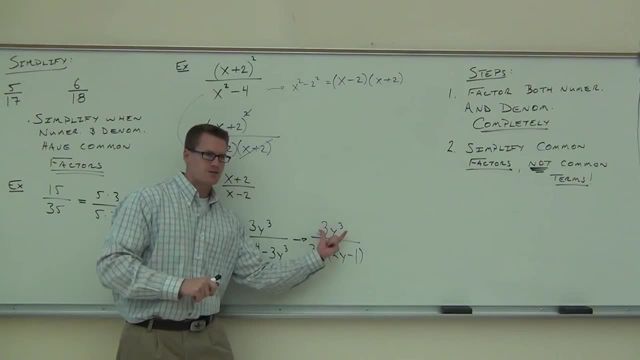 or you can use Facebook, and I can't find Facebook. If it used to be Instagram, but now it's sound like it's not No this, you have to call it Na'vi. I know I love asking that question now. 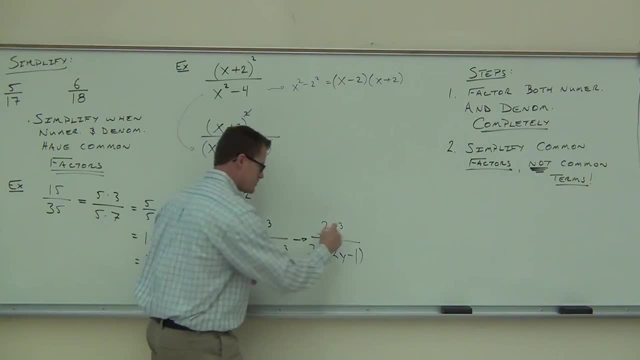 Thank you, Val. This is the best part of the class We get to make things look better, Darn. Would you have to change the sign because the other one's on the bottom, the 2y minus 1?? Change the sign. 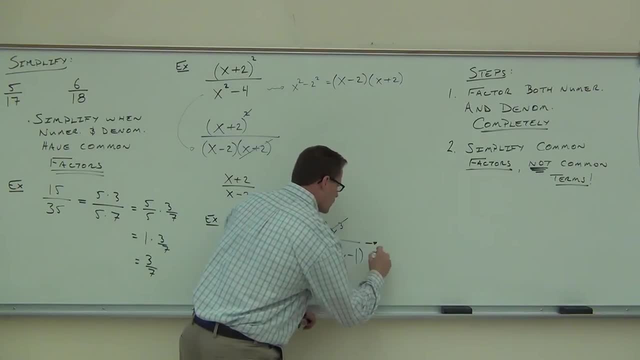 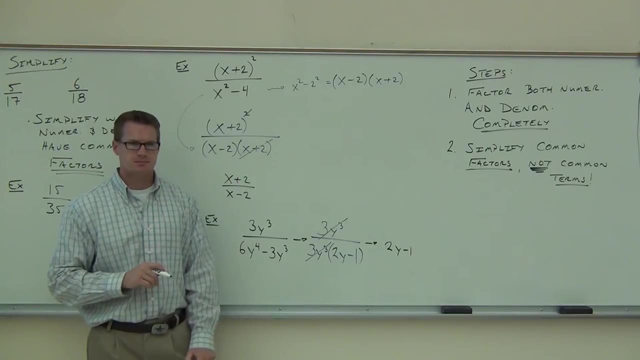 No, we don't have to change any signs. I don't have to do anything, because it's What I am going to ask you is: is this equal to 2y minus 1, like that? No, Explain that, Because the 2y is on the bottom, not on the top. 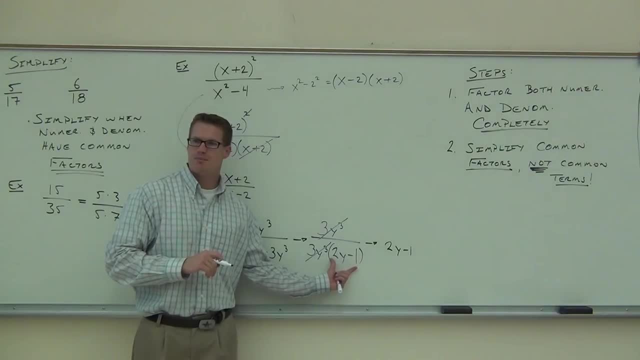 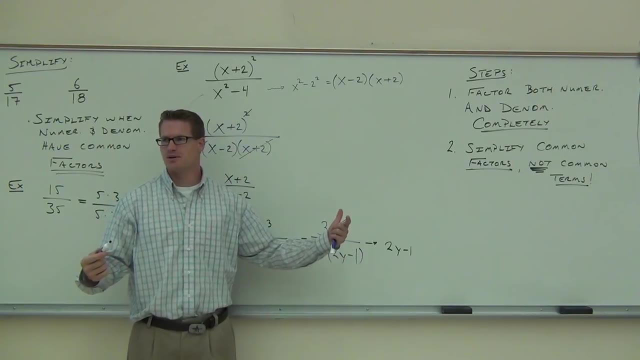 Aha. So since this is on the denominator of a fraction, we can't magically just move it to the top right. We're not Harry Potter. We don't have, like a math wand. Bam, That would be awesome, but we don't have that. 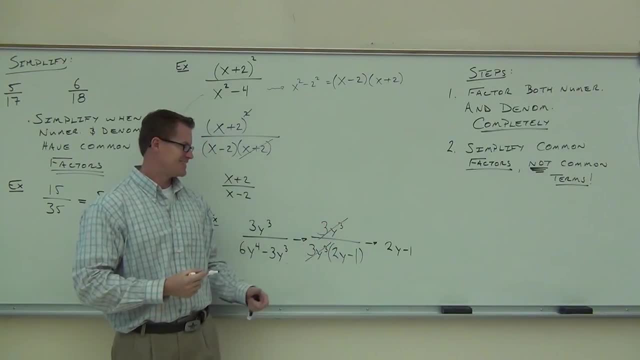 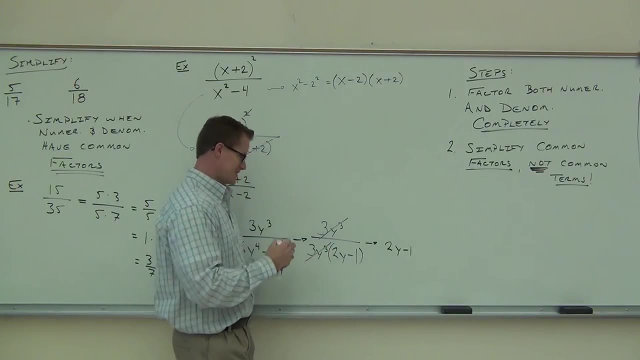 I've got the glasses, but not the More like Voldemort. anyway, I'm just kidding, I'm not. I had an early face. You see that, See the movie. It's crazy, Anyway. so the problem is is: yeah, we can't move this. 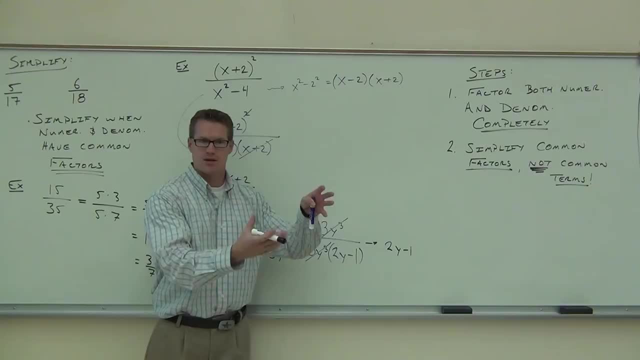 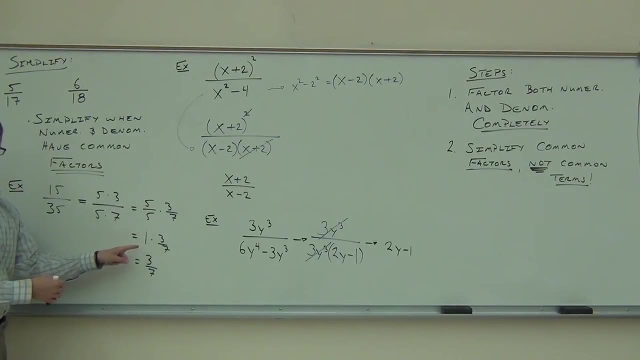 to the new. this would be a numerator fraction. That's right, Like just the value itself can't do that. What actually happens here is that when we simplify, just like we simplified here, we get ones right. We get 1 over 1.. 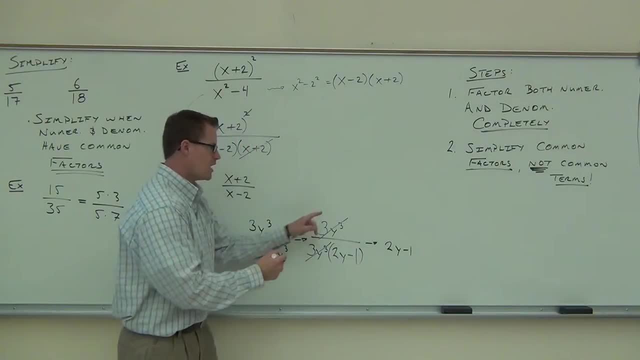 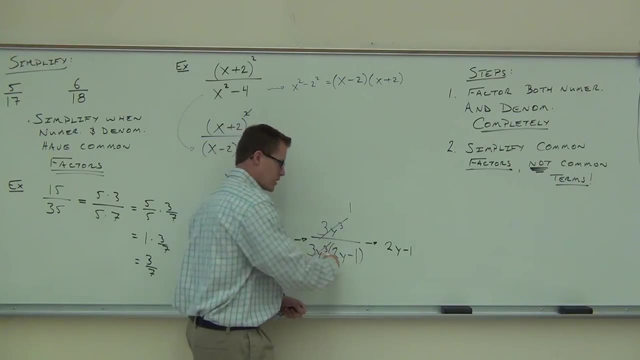 And so this would become a 1, which is why we're getting the 2y minus 1.. But this is also a 1, so be careful: When you simplify, you will get stuff like this on your homework. Don't just eliminate the numerator and put the denominator. 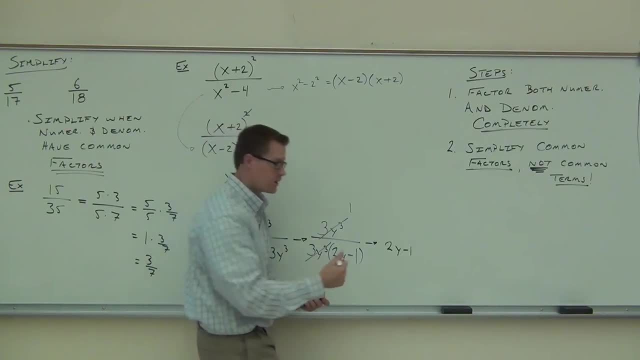 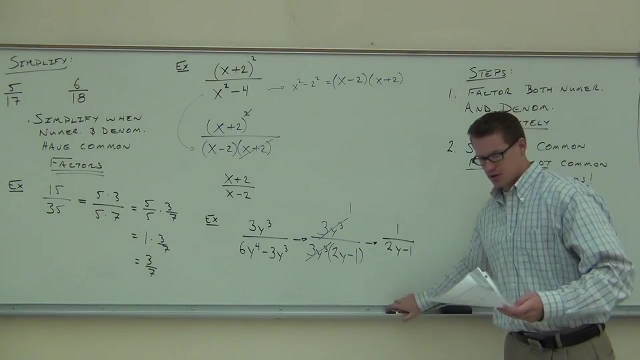 If you eliminate the numerator, you really haven't eliminated it, You just made it a 1.. And so this is 1 over that. That's the proper way to write that. So we're factoring the numerator and the denominator and then we're going to simplify: common factors, not common terms. 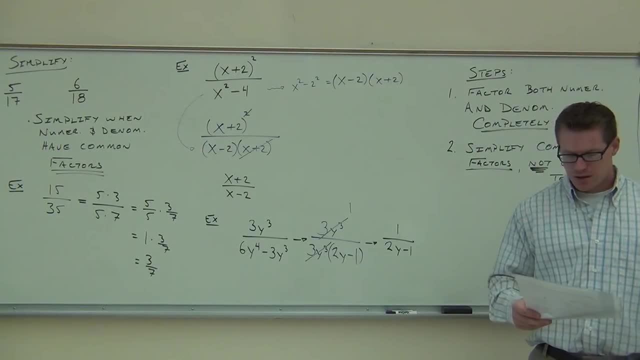 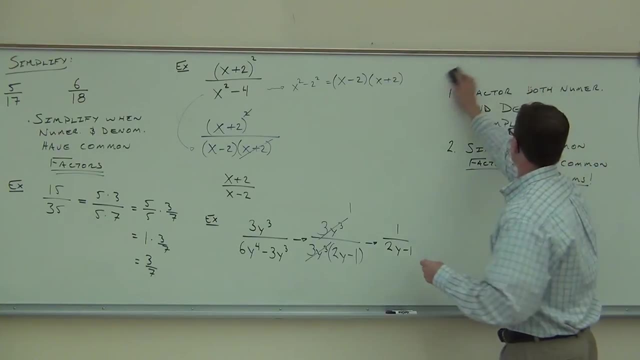 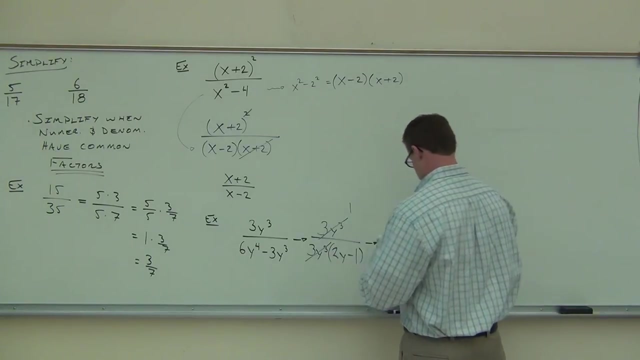 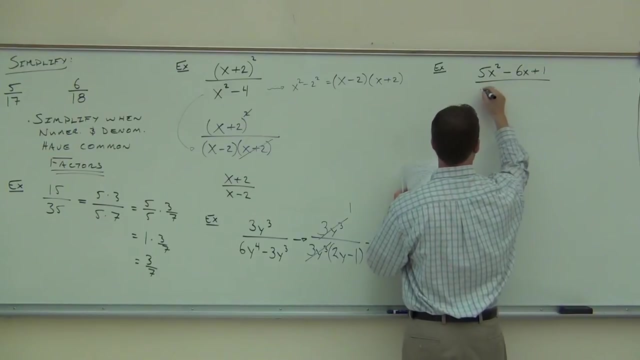 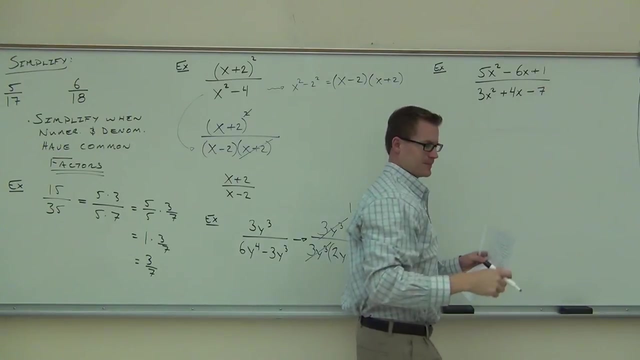 Let's try. we're going to have several more of these things. Let's try a couple more right now. I'll show you one more thing, do two more after that and be about done Here 1, much 1.. 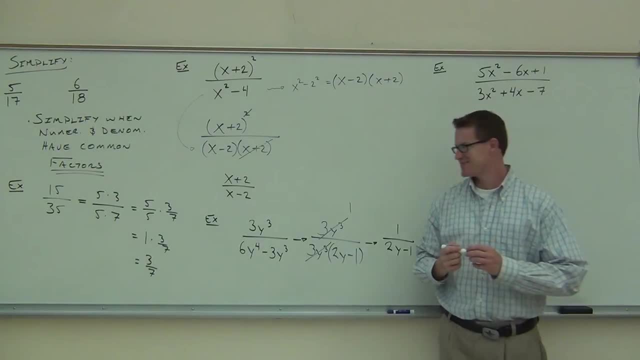 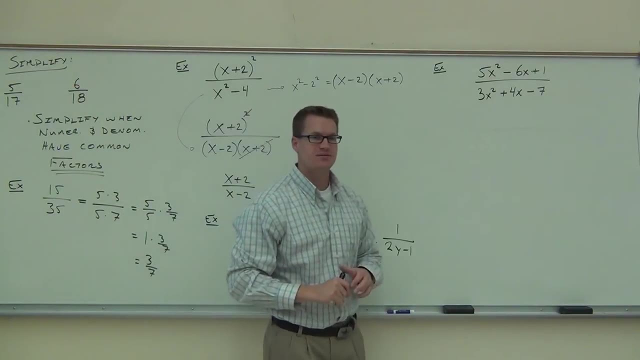 Yeah, yeah, We like those ones right. Can we simplify anything the way it is right now? What about the x squared and the x squared? Can we just cross those out? We'd love to, but no, we can't. 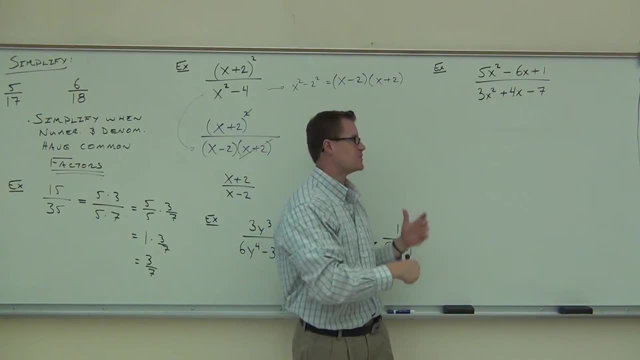 It has to be look like it's in parentheses, or at least be a factor, something like we've had before. So what are we going to do with this problem? if I'm asking you to simplify it, Factor Ha, How do we factor these things? 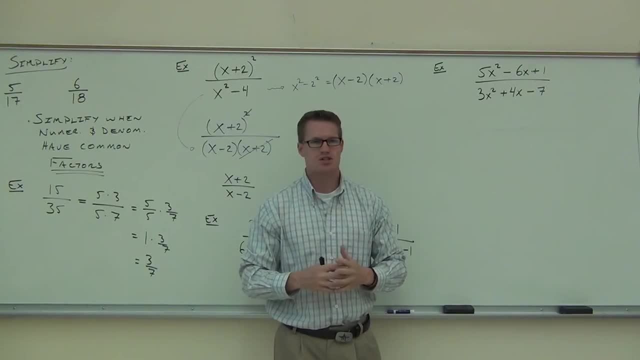 Say it again: Time method. Let's do the time method Now. here's the question. We just learned this. we relearned this like 10 minutes ago. Do I need the extra step to split the middle terms or not? 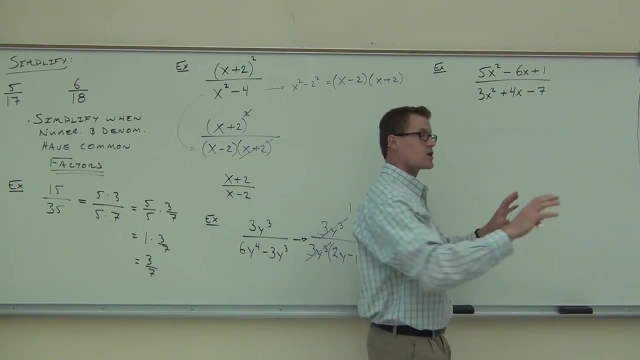 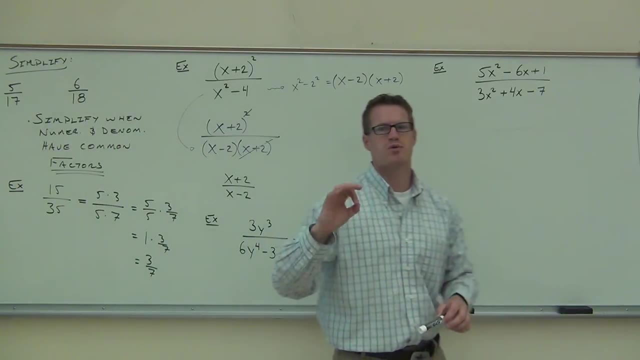 Yes In this one. yeah, I do. I do need the extra step. Don't waste your time when you don't, but you do here. Take two minutes, see if you can factor these. You should be pros at this right now. 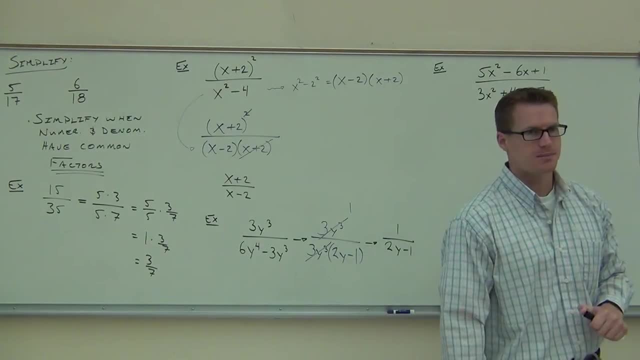 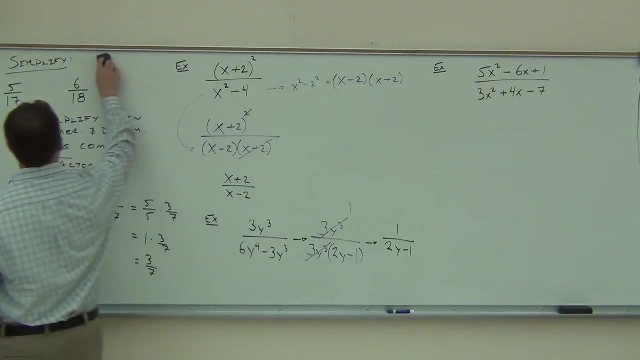 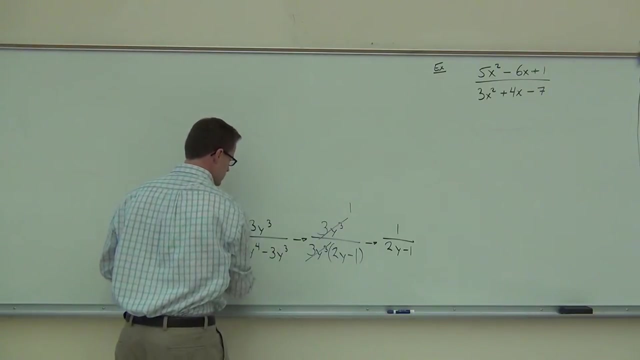 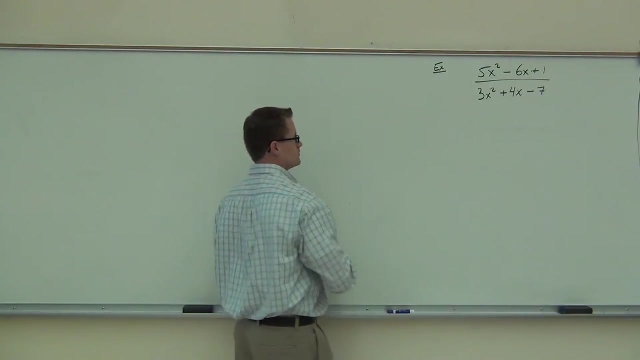 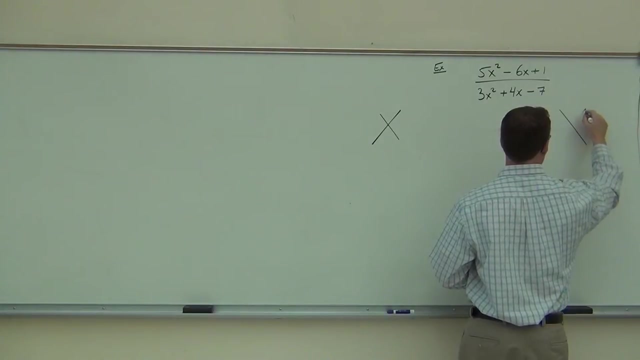 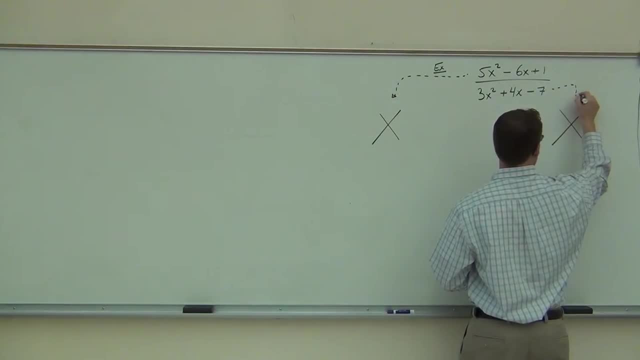 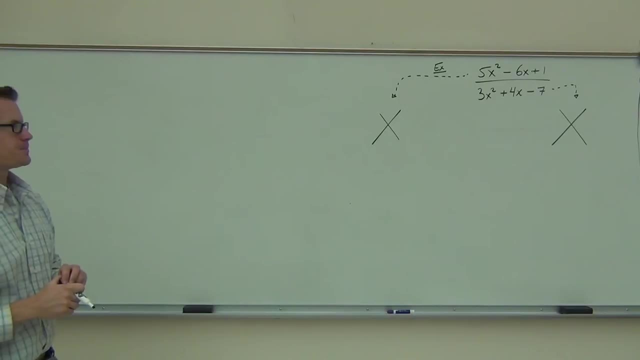 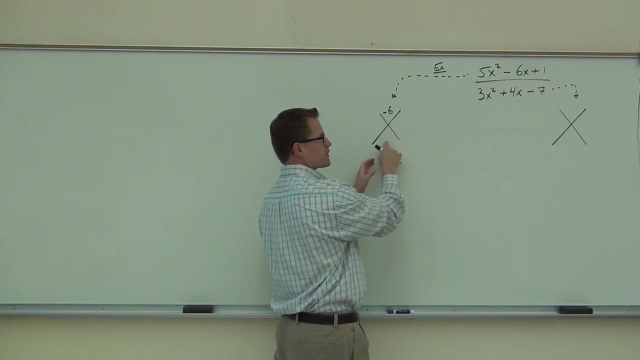 I hope you remembered how to set this up. Just help me out with this one step. What goes on the top for the numerator Negative, 6. Negative 6.. Okay, and on the bottom here One 5 to the bottom 5.. 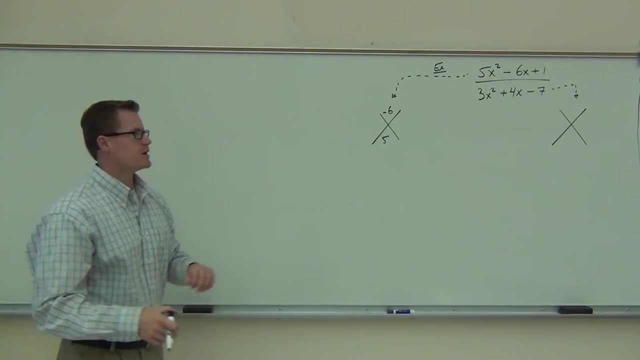 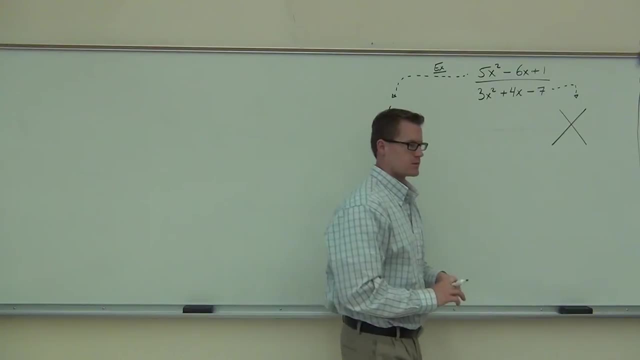 Five to the bottom Five. Five- I don't remember how to do that. The B goes here, the A times C goes here, So we factored both, Both. yeah, This is pretty much like three problems in one, Which is why I said: you gotta learn. 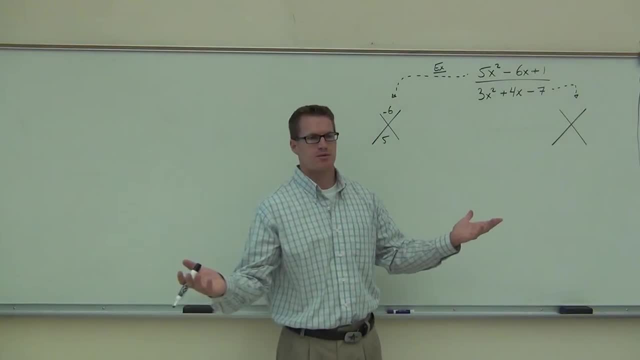 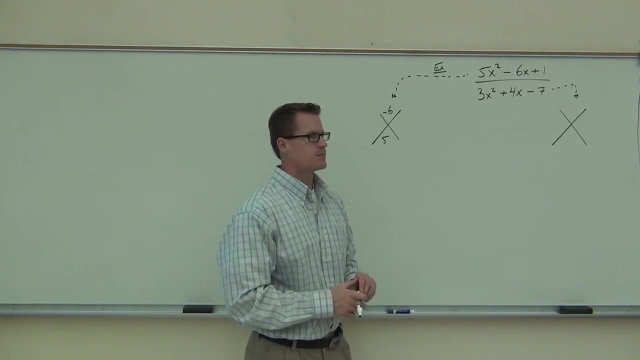 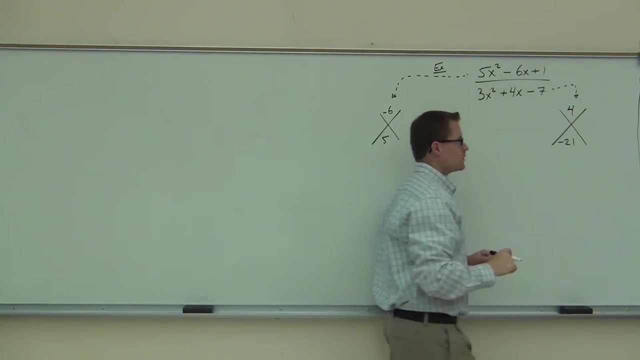 how to factor correctly, right, Because if you don't know how to factor this, how are you supposed to simplify it In the other one? you need four and you need what was down here. Twenty-one Negative four Seven, No. 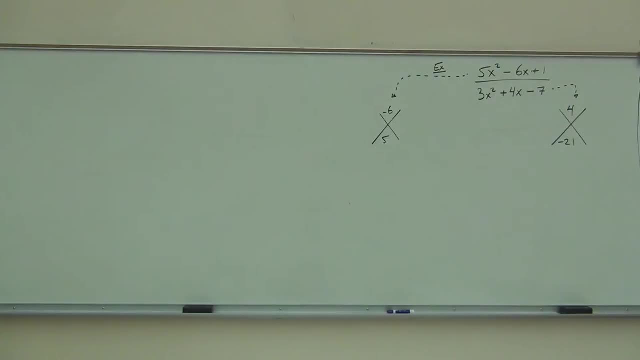 You multiply those. You multiply those: A times C: Energy times one. Negative four. Negative four. Now you know how to get to zero. Negative four. Now will you multiply this by two. Negative four. Negative four. Negative four. 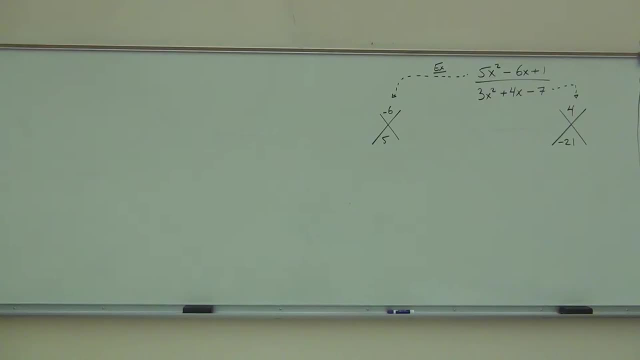 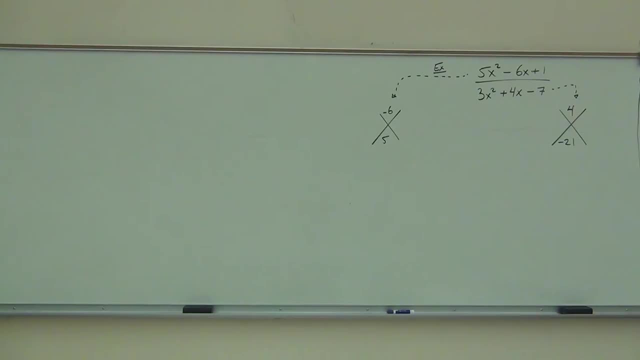 Get them done. If you guys are having trouble with the notes, you can write them in the comments. I think we have about 24 minutes now. The next thing we're gonna do is you might want to get your notes signed off. 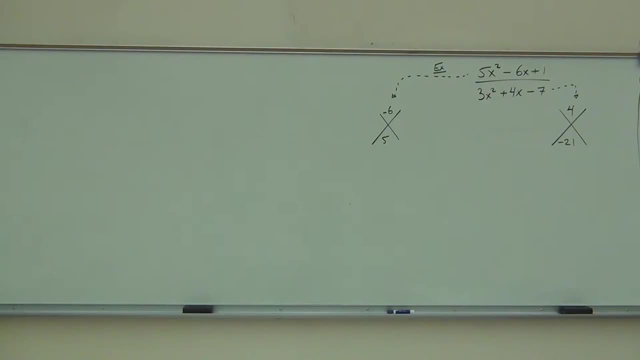 when we're finished, But I understand you want to write them in the comments. Okay, we're about to get going on this thing and let's get started up here on the board If you're still going. cool, work on it. 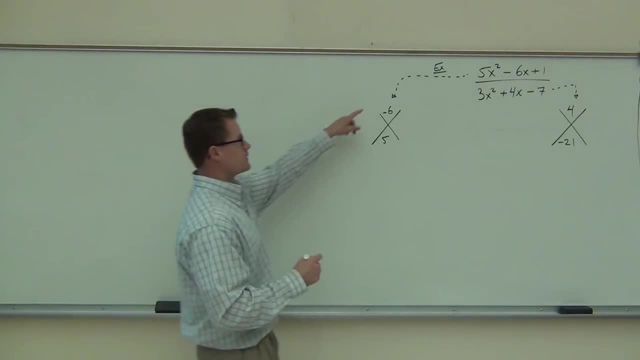 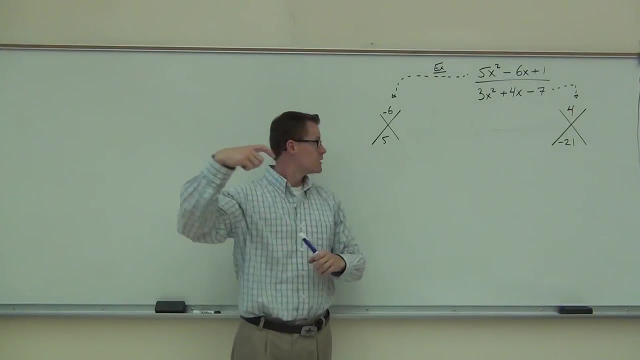 Make sure you can factor these correctly. Okay, so up here we have the negative 6 and the 5.. Are you okay in getting those two numbers folks? Good, We're going to find two numbers that add to negative 6, right, and multiply to 5.. 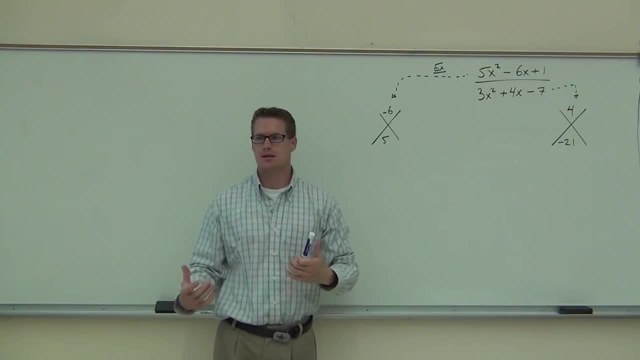 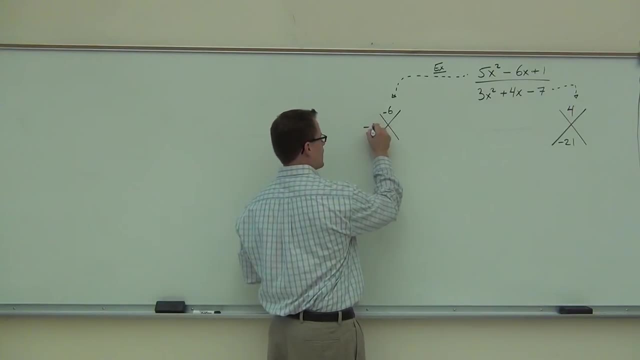 The only thing that's going to multiply to 5 is like 5 and 1, that's it. So I know they both have to be negative, because this is a positive and that's a negative. So we're going to do negative 5 and negative 1.. 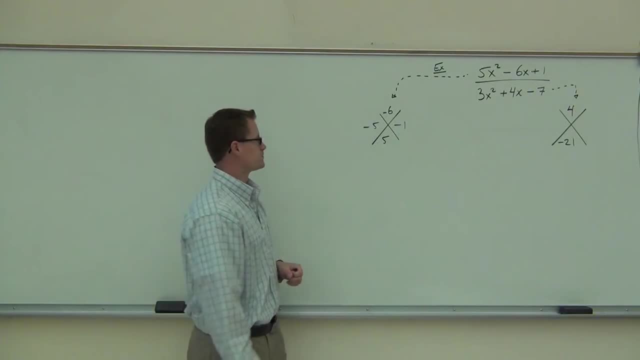 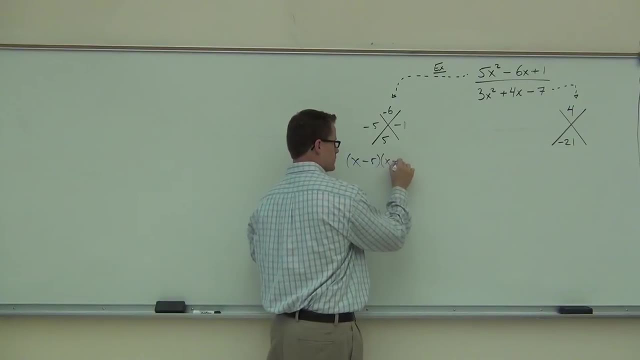 Did you get negative 5 and negative 1? Good, We cannot do this, Okay, So what we're going to do in this particular case? because we have a coefficient of 5, we just covered that again- right, so we can't do this one here. 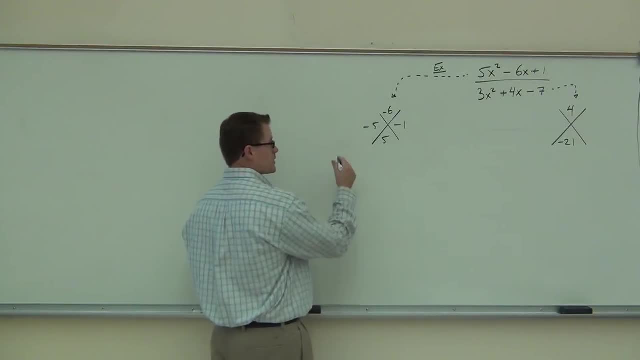 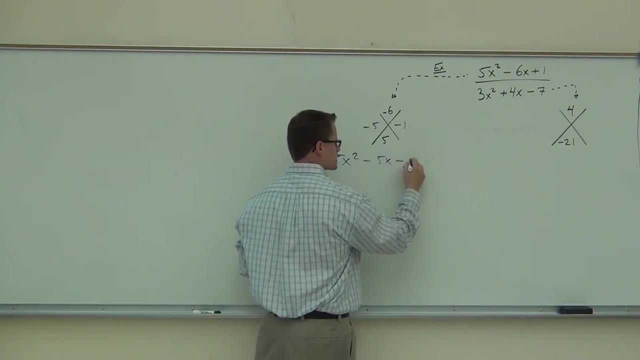 But what we do as we split that middle term up. this is where I said we had the extra steps. So we have a 5x squared, minus 5x minus 1x. I'm going to put the 1 there just to make sure we see that plus 1.. 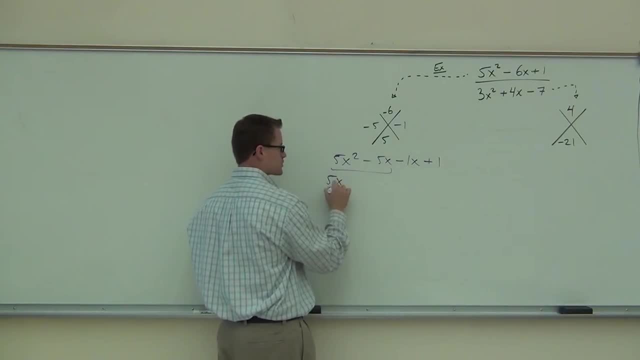 And we're going to factor by grouping. We have a 5x. We're pulling out of that, We're factoring that out. We get x minus 1.. Over here, notice, we have to factor out a negative. Did you guys see that? 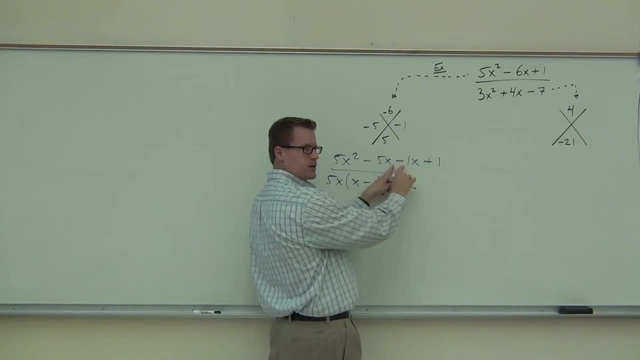 We've got to factor out a negative And the only thing that's going in both is 1.. We're going to get x and minus 1- again The minus, because we factored a negative out. we're basically dividing by a negative. 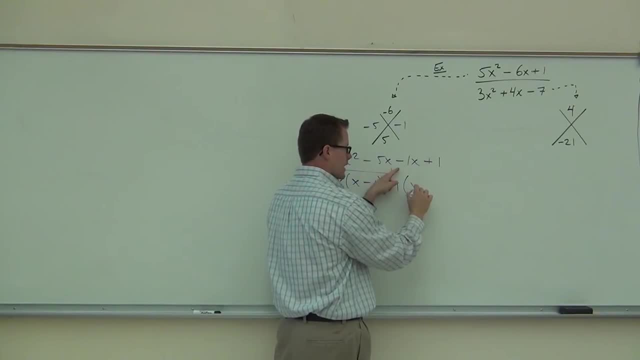 that's changing the sign. We have exactly the same thing here and here. That's what we wanted. We're going to get x minus 1 and 5x minus 1.. How many people made it that far? Okay, So we're going to get x minus 1 and 5x minus 1.. 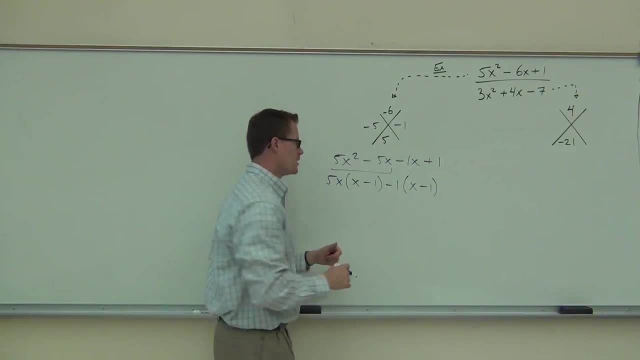 How many people made it that far? Okay, So we're going to get x minus 1 and 5x minus 1.. We have exactly the same thing here and here. That's what we wanted. We're going to get x minus 1 and 5x minus 1.. 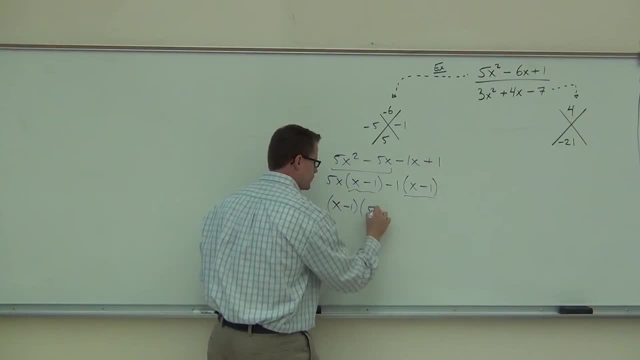 How many people made it that far? Good for you If you didn't go back and work on this on your own next time. See that you get that right. You have to, Okay. Next one: we have 4 and negative 21.. 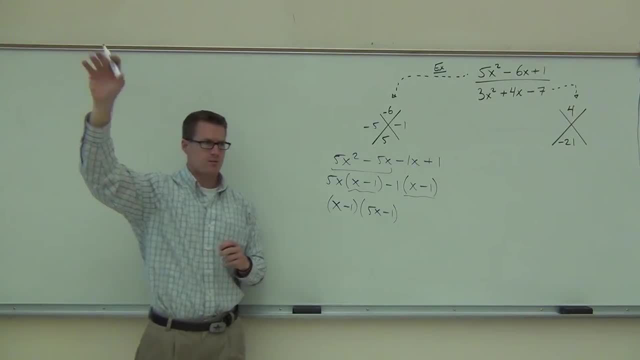 I'm looking at that. I'm seeing a 7 and a 3. somehow. Are you seeing a 7 and a 3? also Probably seeing a positive 7 and a negative 3.. Again, we have to split that. We're going to get x minus 1 and 5x minus 1.. 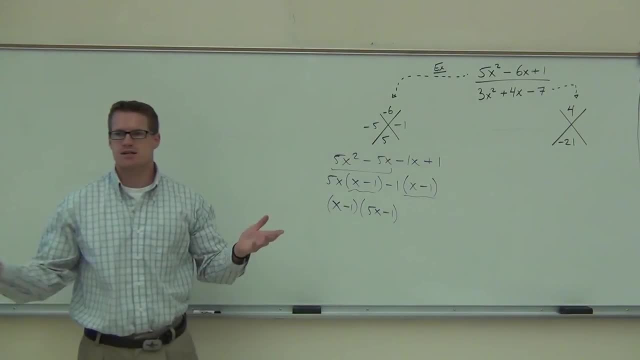 How many people made it that far? Good for you If you didn't go back and work on this on your own next time. See that you get that right. You have to. I'm looking at that. You have to. I'm seeing a 7 and a 3 also. 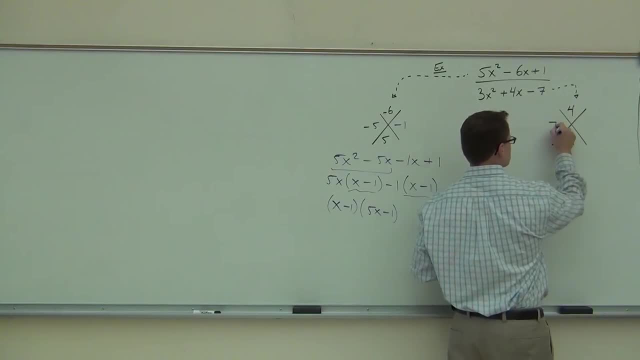 Probably seeing a positive 7 and a negative 3.. Again, we have to split our middle term up: 3x squared plus 7x minus 3x minus 7.. We're going to factor. The only thing that factors out of our first two terms is x. 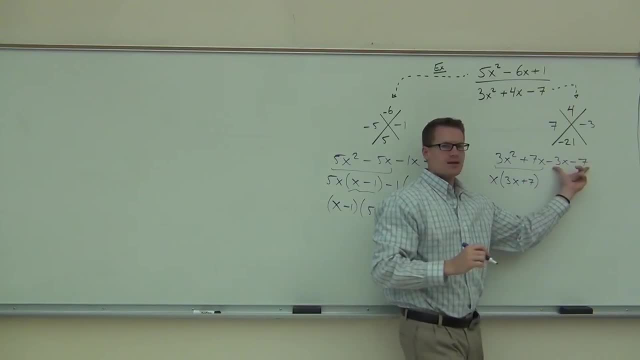 We get 3x plus 7.. What factors out of our last two terms? it has to be a negative because we have a minus there. The only thing that's going into both is 1.. So we're going to factor a negative 1.. 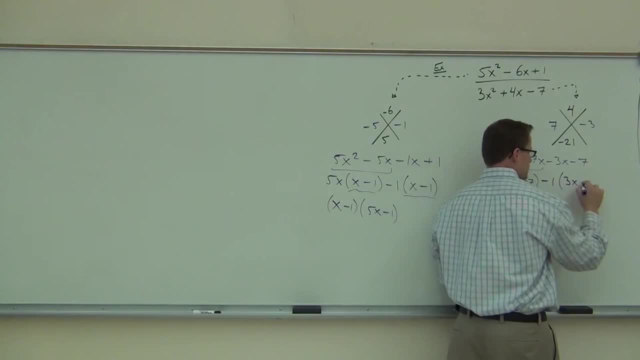 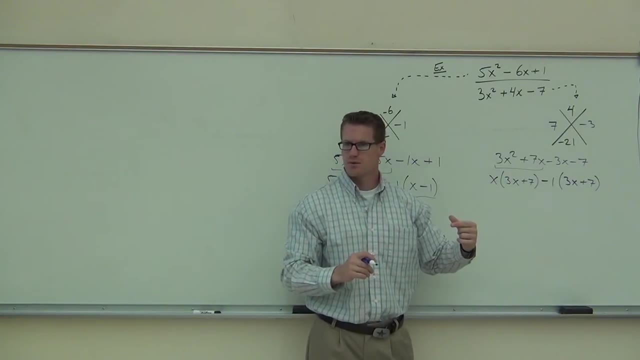 I'm going to put the minus 1, and I'll have 3x plus 7.. Again, those signs change because you're factoring by a negative. Get used to that. That happens a lot. Are you okay so far with that? 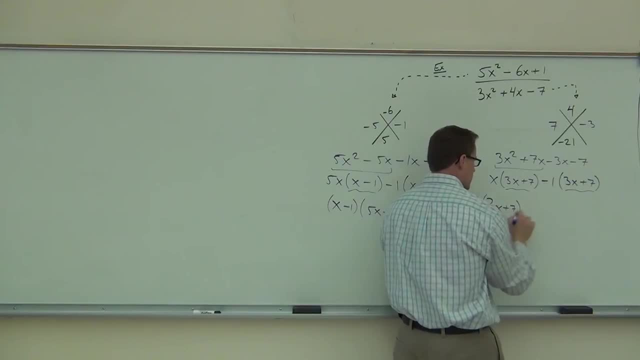 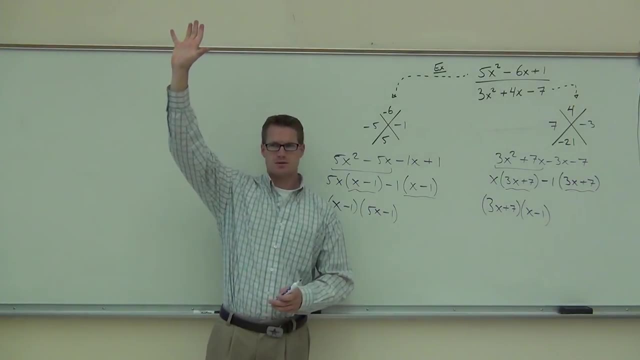 When I factor by grouping, I get 3x plus 7.. I get x minus 1, and I'm done. I factored that stuff. How many people made it down on both of those? Good, If you didn't, if you didn't. if you're like: oh my gosh, I messed something up, please. 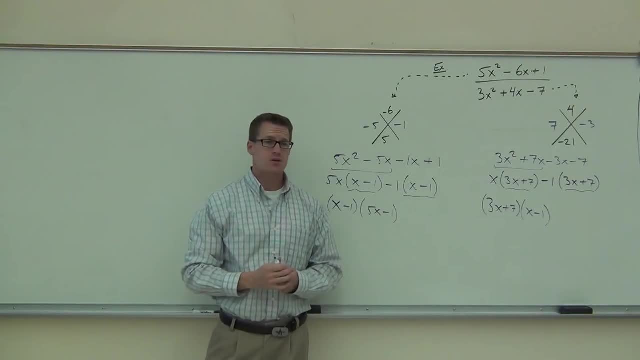 go back, I can fix that. Go back tonight and work on that: Your factorings right now. it's the biggest thing you can do. It's the biggest thing you can do. Simplification's easy if you know how to factor. 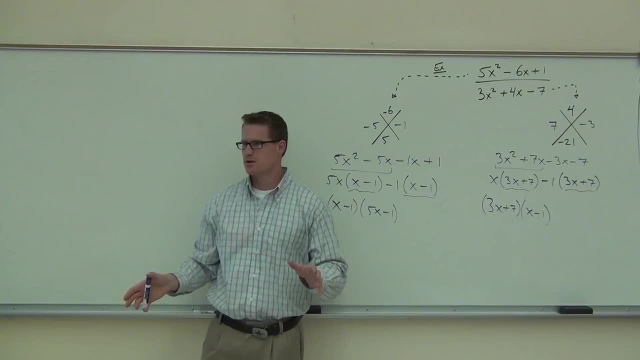 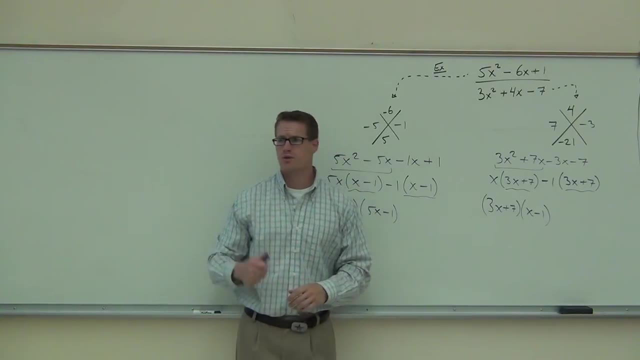 Multiplication, division of rational expressions, is easy if you know how to factor Addition-subtraction. well, we have some other stuff to do, but the simplification part of that is easy if you know how to factor. If you don't, you're going to struggle with all that stuff and I can't afford to have. 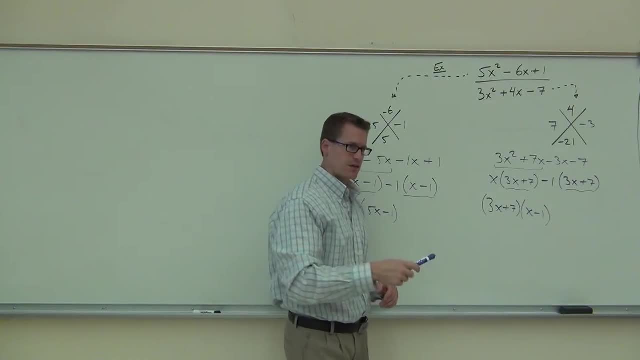 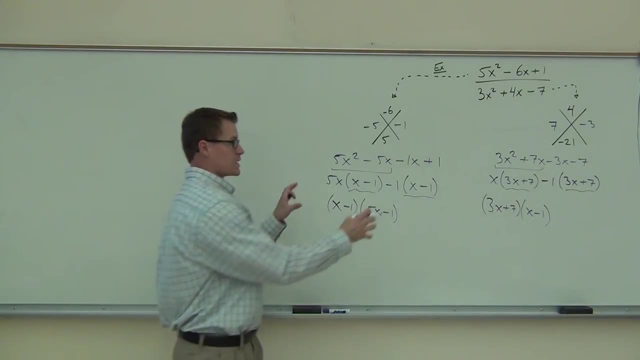 you do that, So you need to be reviewing these lessons online, if that's your case, or coming and seeing it, or something. I'm trying to do this. OK, Now we're almost done. What we're going to do. we're going to take these factored versions. 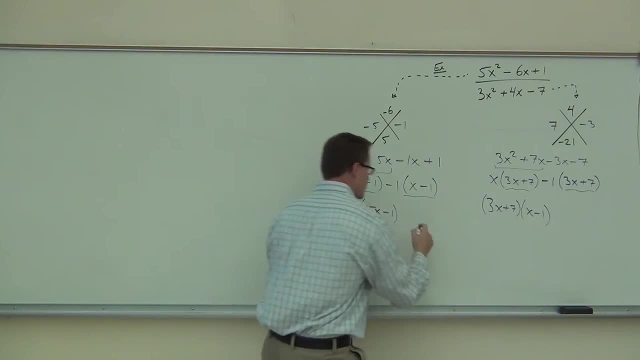 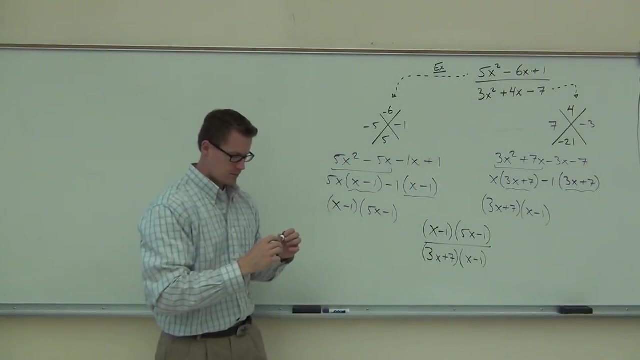 We're going to put them back in our fraction form. So from our numerator, we have the x minus 1, and we have the 5x minus 1.. From our denominator, we have 3x plus 7, and we have x minus 1.. 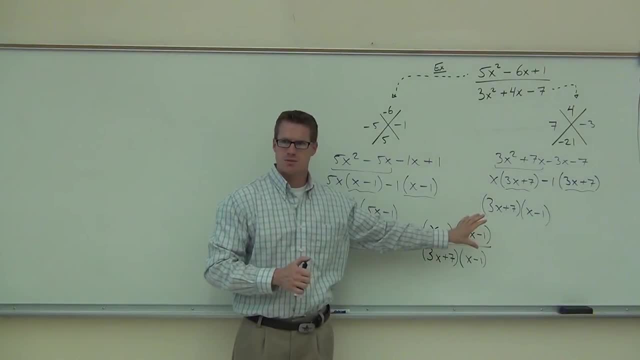 If you didn't get these right, can you follow them down and see that this is the answer, See that this is the appropriate way to go? Are you guys all right with that? You sure? OK, Now, do we have any common factors? 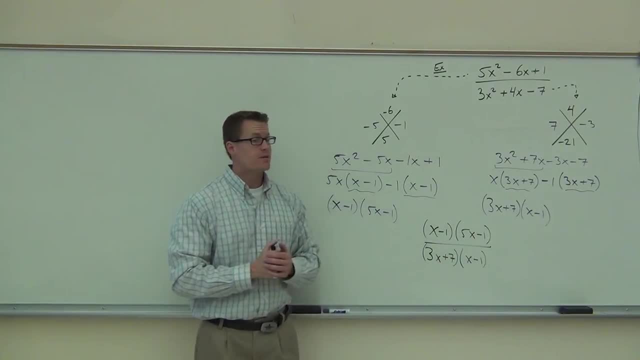 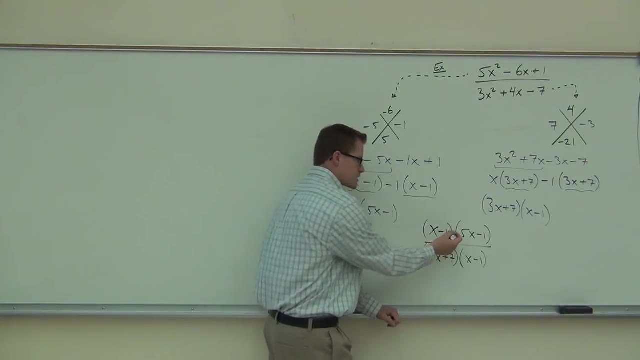 Is there anything we can simplify? That's great. X minus 1's are factors because they're multiplied here and here We can take the entire factor and simplify it out. That's what we want to do. So x minus 1's are gone. 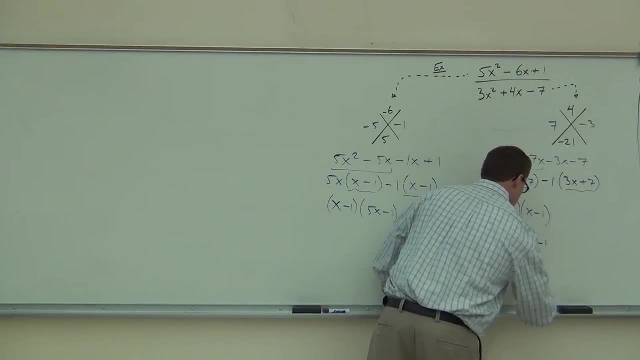 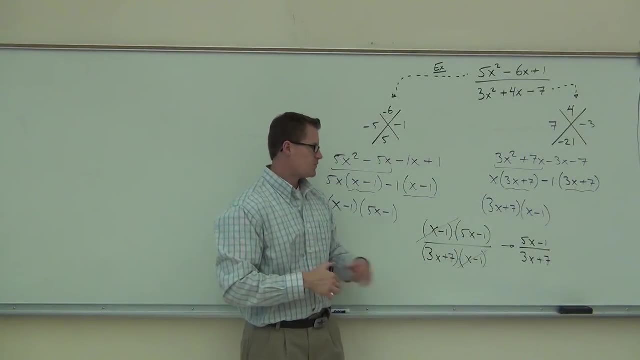 We're going to get 5x minus 1.. OK, Cool, 3x plus 7.. Can we simplify any further in this problem? If you could, you would have done it here. Okay, this takes care of all your simplification at once. 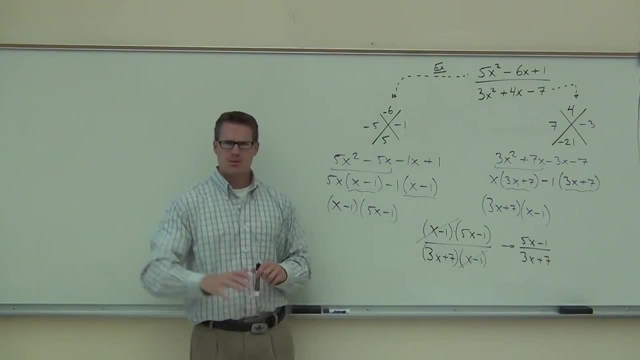 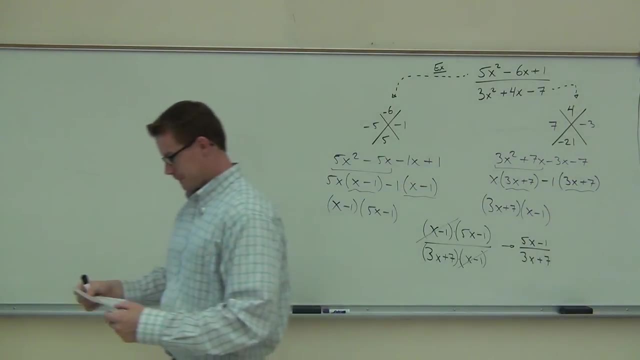 provided you've completely factored How many people are okay with that. Feel all right with this one. so far, Good, all right, that's fantastic. I have a question? Yeah, So when we simplify and we move over to the final answer, 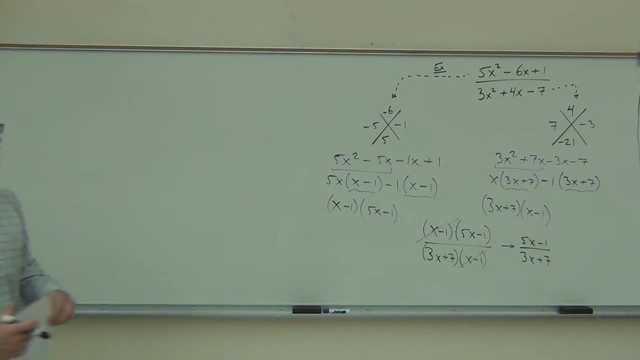 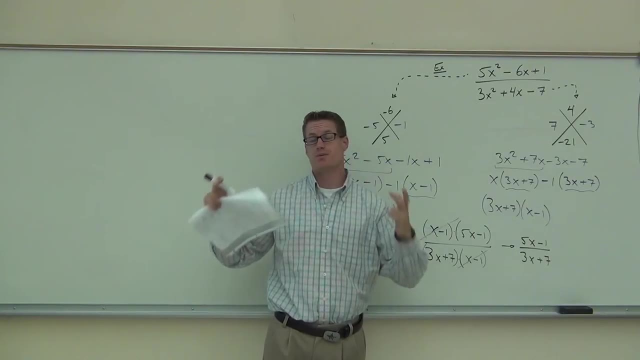 the parentheses just disappear. If you have just one factor, you can do that. Yeah, because it's just saying: this is my factor, right? You're multiplying by one. That really doesn't make a difference. That's a great question. 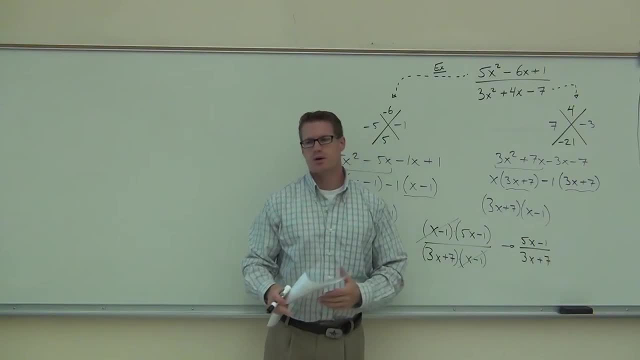 If I had like three factors and I just simplified one of them, yeah, you'd want to keep the parentheses. Okay, let's end with this one. I want you to work on one on your own. Just see what happens on that. 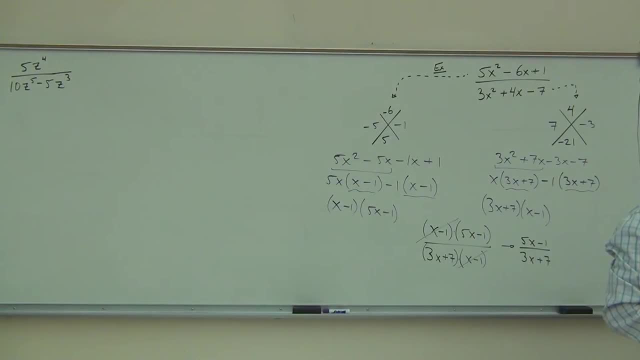 I want you to factor if you need to and say: fine, Yeah, That will do it All right. good, that's good, All right, All right, Okay, Thank you, Thank you, Thanks everyone, Thank you. 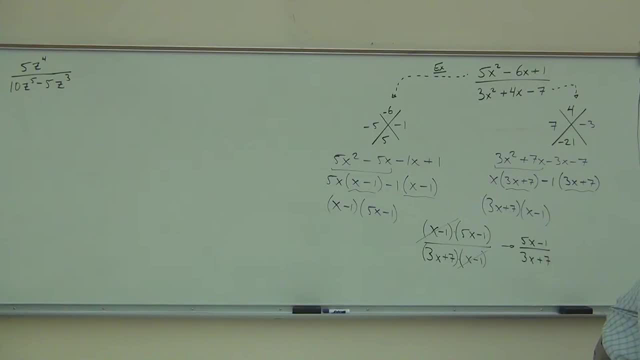 And add it to the whole. Okay, Okay, Thank you, Thank you, Thank you. I see lots of good factors. That's great, That's fantastic. Well, factors out of here. I hope that you saw this: You factor out a 5,. 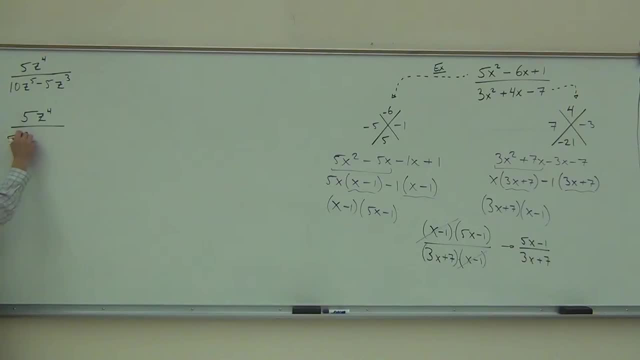 and then, And the largest power of z that's common to both is z to the third. Did you get that? Yes, You have two z squared minus one. Did you factor that correctly? Yes, Good, now does anything simplify it? 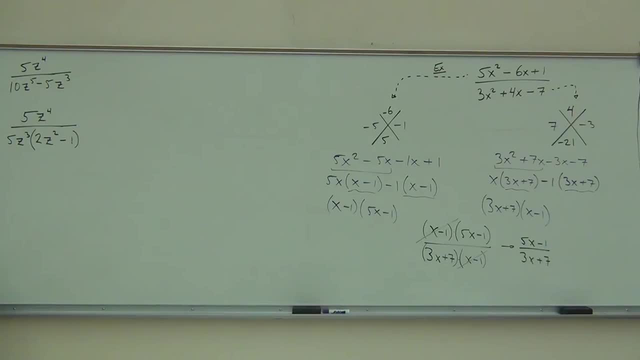 No, The fives, Sure fives. do The z's? yeah, look at it Now, what you have here. really, you could think of it like this, if you wanted. You could think of it as five, five, five z to the third time, z. 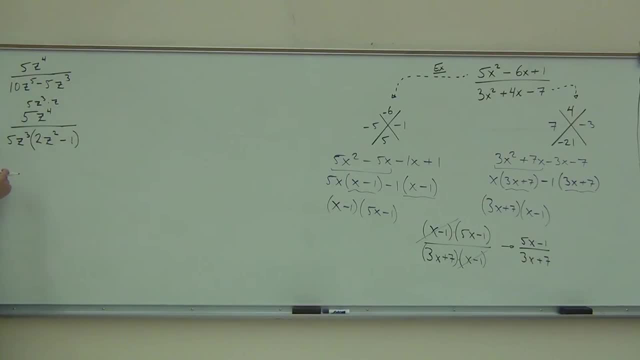 You could think of that, isn't that? five z to the fourth. In that case you go: oh, you know what, These are all gone. I have a z left, Or a different way you could think of it: fives are gone. all but one z is left. 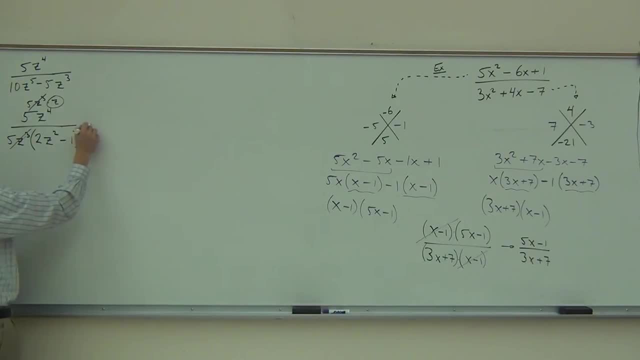 So what's gonna be on the numerator of our fraction? Just a z, that's right. Two z squared minus one. One last question: do these z's simplify? No, But they're right on top of each other. They're on top of each other. 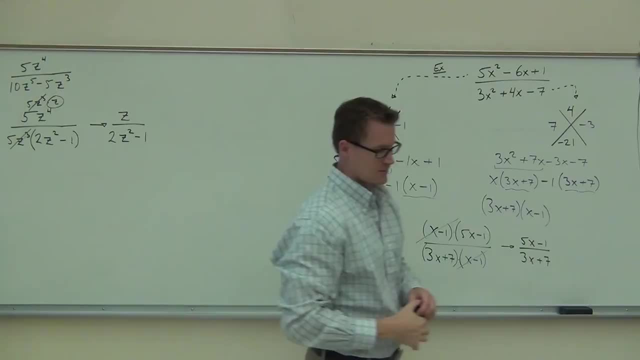 Can't do that. the minus one, It's a minus one. all right, We'll talk about one last thing right now. This will lead us into what we're gonna do tomorrow. How much is that One? Explain that It is. it is right. 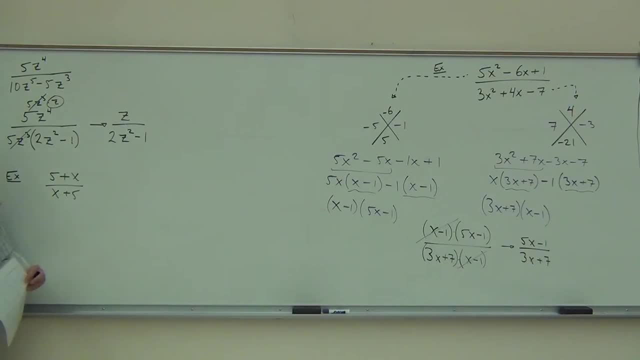 Why? Because when you do addition, addition's called what, when you do this, Communicate, You could switch that, couldn't you? Because it doesn't make a difference, because it's addition, No problem, That equals one. Does the same thing happen with that? 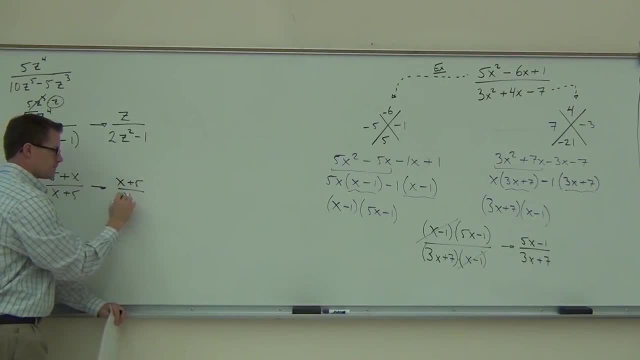 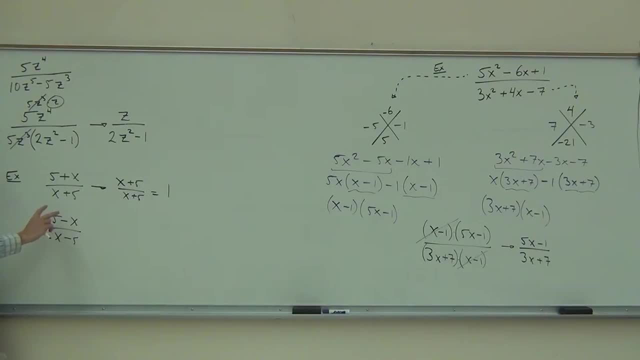 Subtraction says: when I do this, the signs go with those values, so I'm gonna get negative x plus five over x minus five. Now, that's clearly not one That doesn't equal the same thing, But there's one thing that we can do to simplify this. 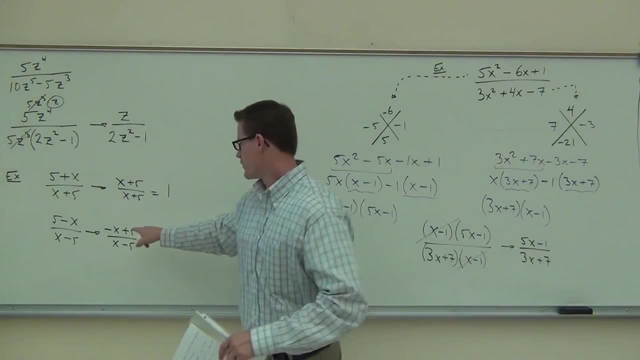 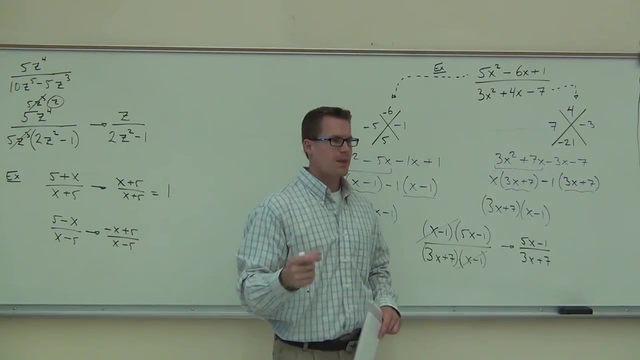 What we can do. whenever you are off, notice how our variables and our numbers are exactly the same, but every sign is different. Do you guys see that? Yes, When that happens, what you can do: factor out a negative 1.. 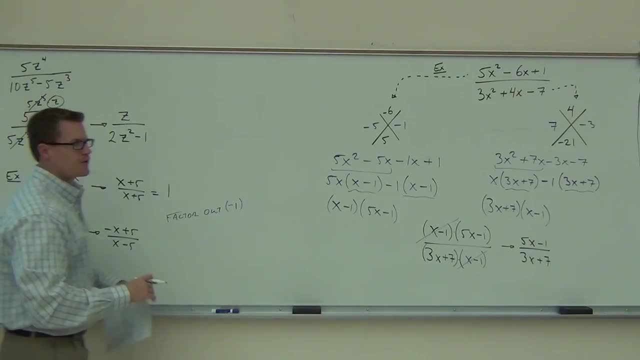 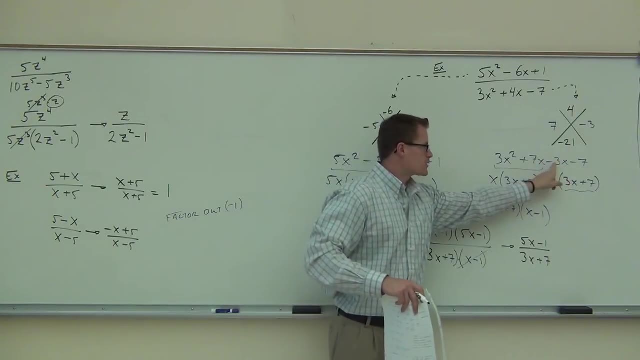 Factor out a negative 1.. If we factor a negative 1,, just like we factored a negative 1 from over here- all that's going to happen. look at the board right now. some of you aren't looking. When you factor a negative 1, all that's going. 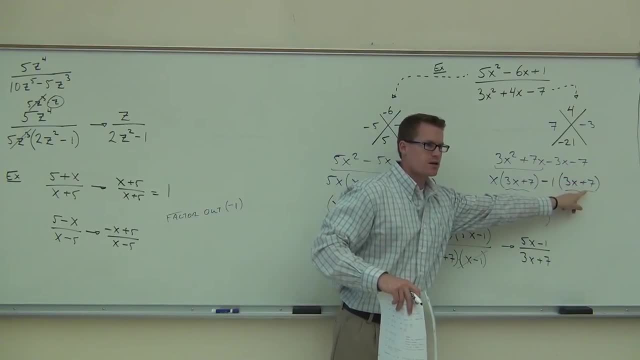 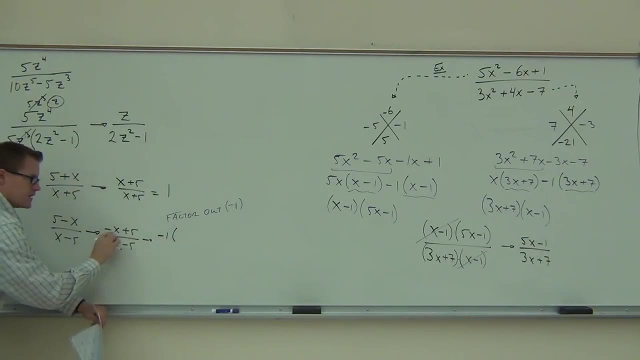 to happen is both signs change. Do you guys see that? So if we factor a negative 1 from here, let's factor a negative 1 and what we're going to get is, instead of negative x, we'll get x Instead of plus 5,. 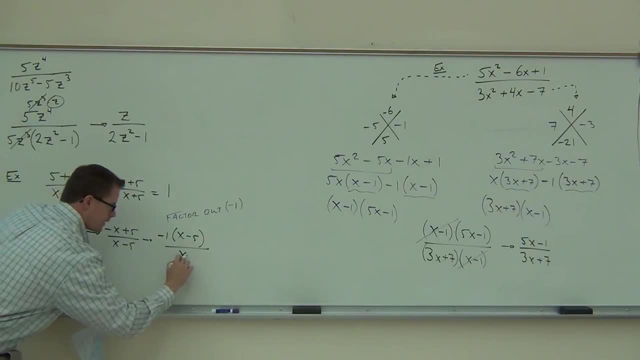 we'll get minus 5, all over x minus 5.. Now do you see that the x minus 5's are factors. We can simplify that And our answer that's negative, 1. So when our signs are different, but the values are the same. 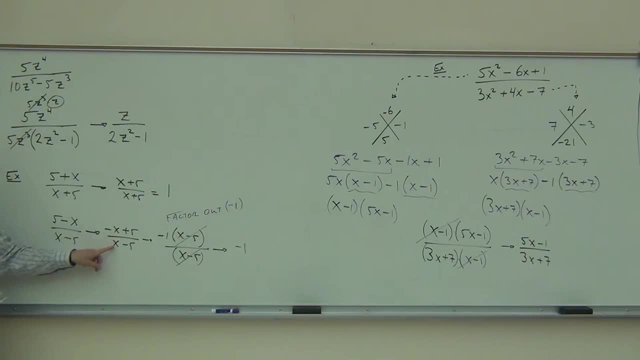 like x is the value of y speaking on me, like we have an x and x and a 5 and a 5, but the signs are different in each case. Factor a negative 1 and then you're going to see that Here's the big kicker that we're going to use next time. 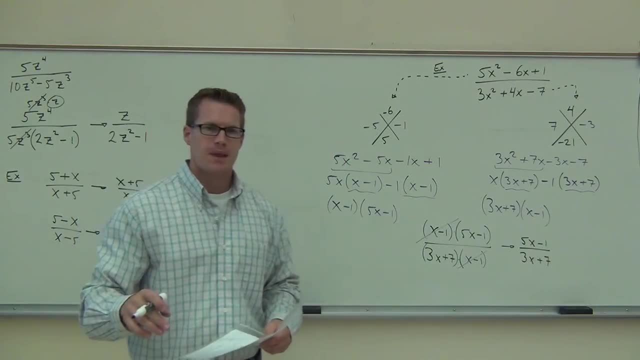 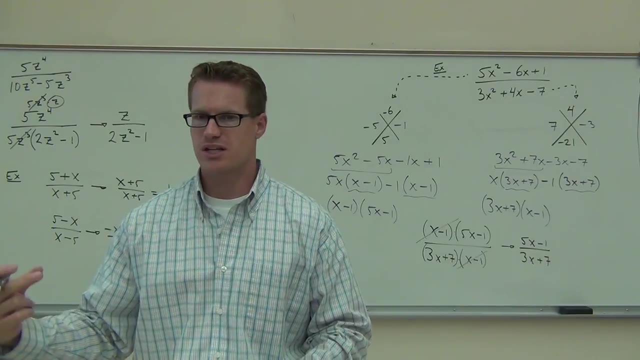 Just write this last statement down. What we're going to try to do when we're factoring is make sure that the term with the largest exponent is positive. Make sure the term with the largest exponent is positive. That's what I did here. 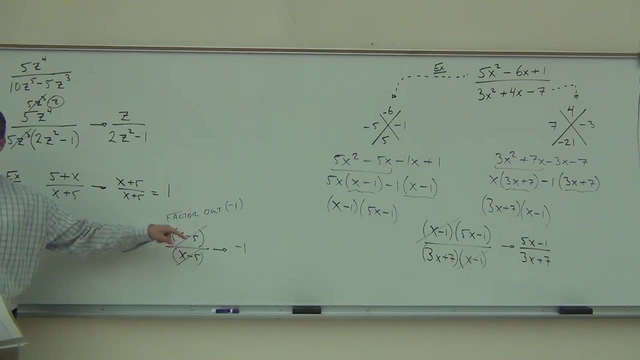 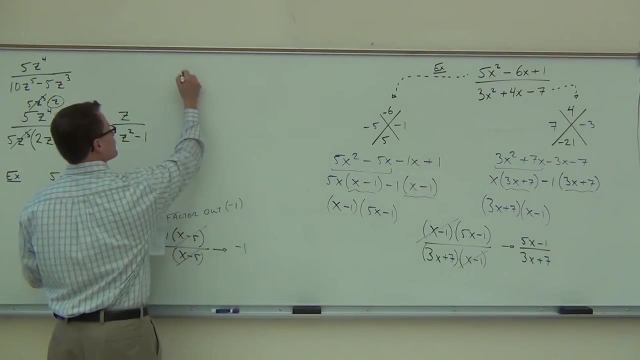 Look, X was negative, So I factored a negative 1. If you make sure the term with the largest exponent is positive, your life becomes easier. You can factor things way easier. So what I want you to do is factor to make the term. 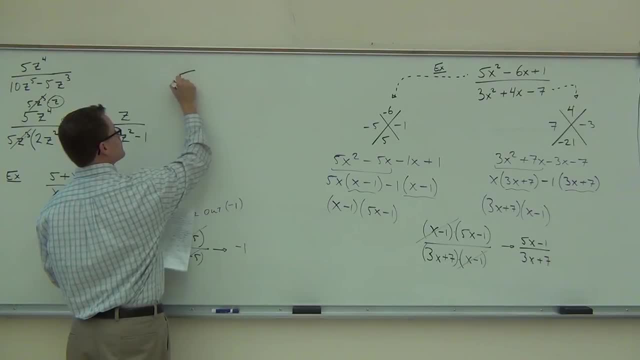 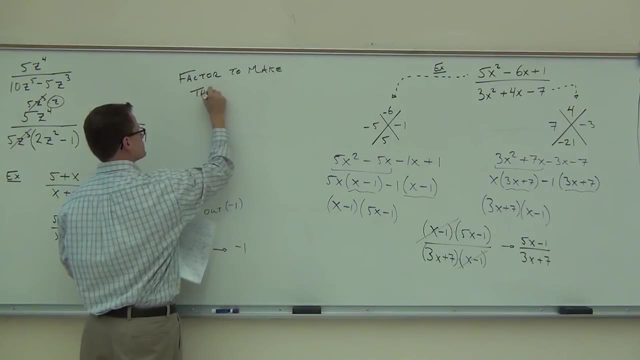 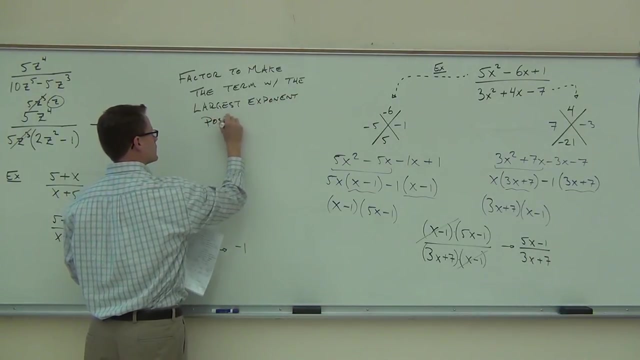 with the largest exponent: positive. This is actually pretty simple, but it's a good way. You're going to do this on absolutely any day. You're going to do this on every day, every day, So you're going to be able to do that on every day. 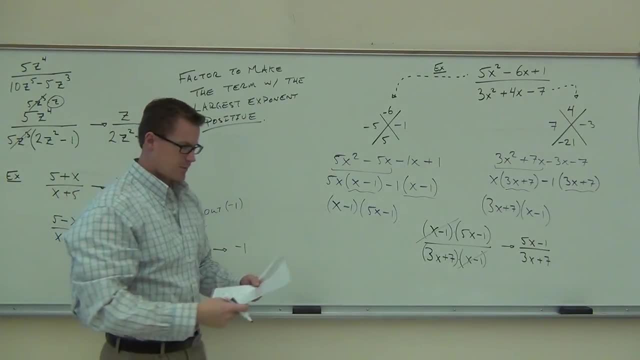 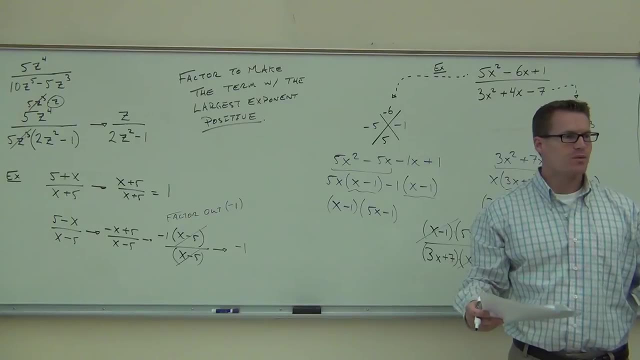 It's going to get organized and you're going to be able to do it on every day. on this day, You're going to be able to put all your assignments on there. That's going to look like this. So you're going to have one assignment divided. 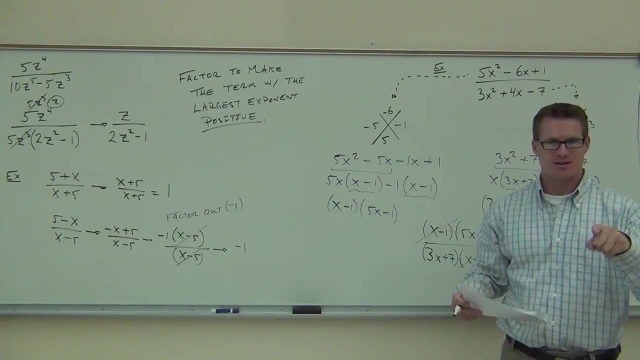 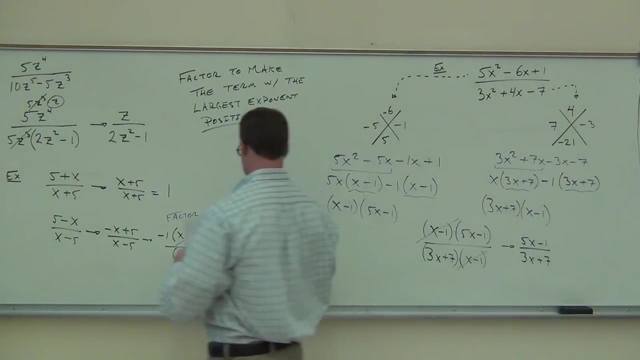 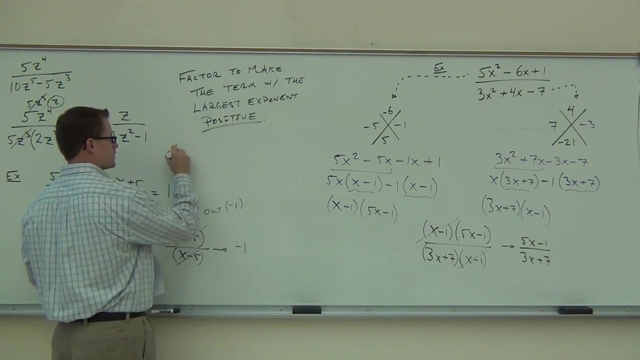 And then each day is going to have one assignment on the second S, So you're going to have your homework. That'll help us out. It's this: Is it due Monday or is it due tomorrow? Okay, just so you know. everything is lowercase. 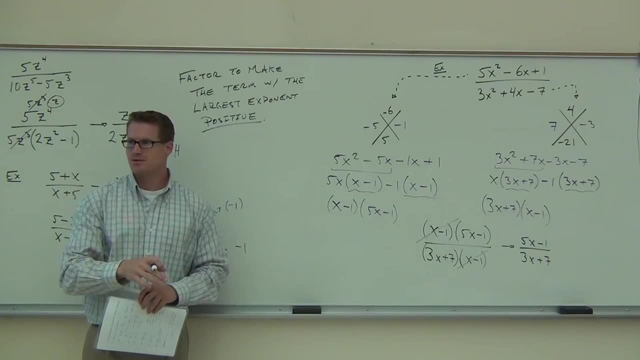 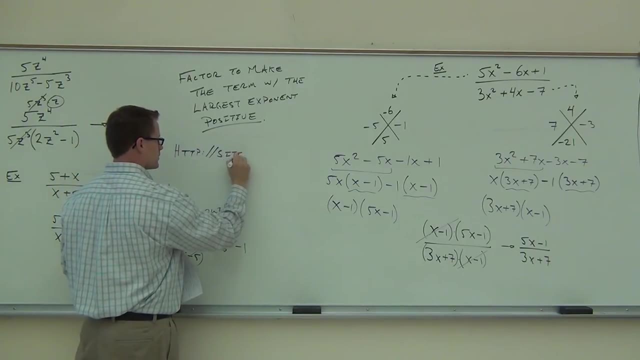 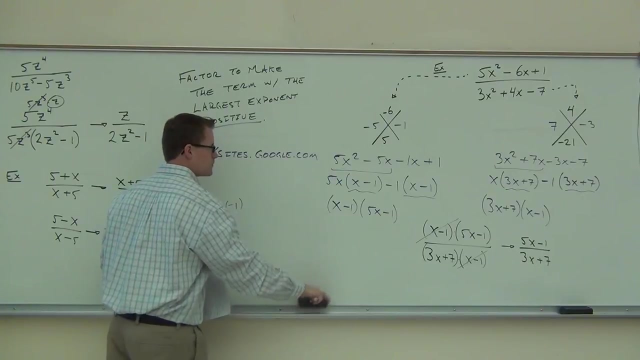 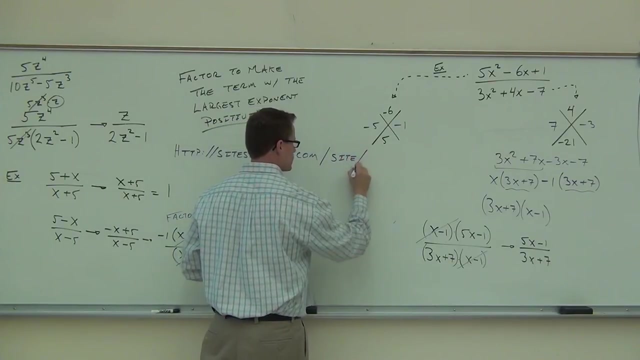 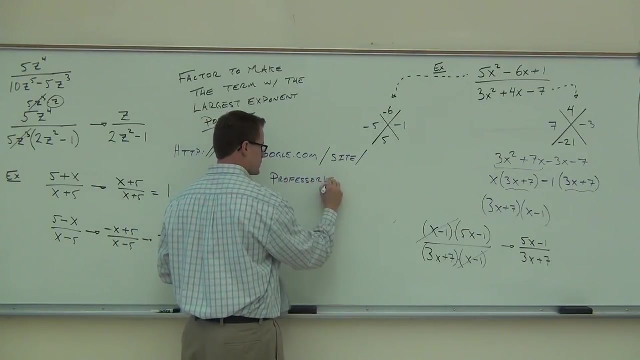 I just can't write in lowercase, So just everything is lowercase. It's sitesgooglecom backslash site singular backslash Professor Leonard 570.. Just like this, It's all one thing. You go to the top of your website browser. 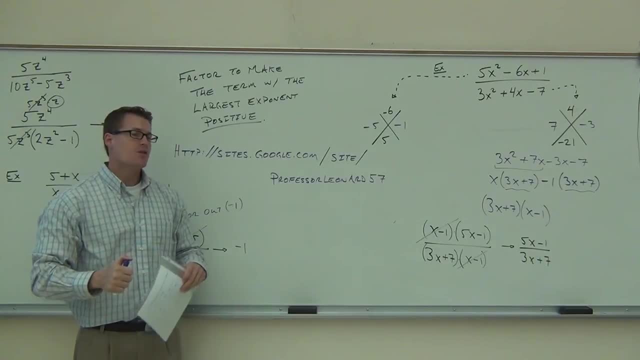 You plug that in, It will come up. Go ahead and find it. Go ahead and find that The homework is not due tomorrow. It will be due on Monday because we're not done with this section. okay, Remember, I told you at the beginning of the class that I would give you the assignment. 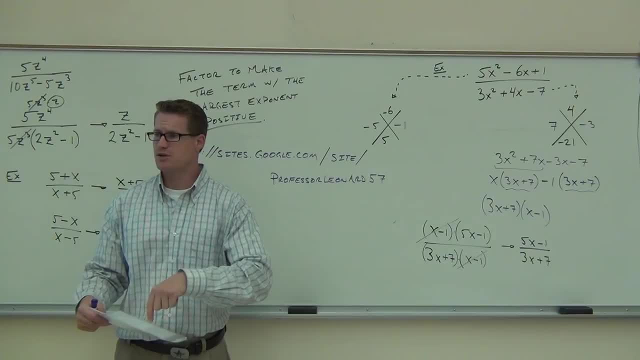 before it's due if we didn't finish the section, So the assignment will be on there this afternoon. If you want to get a head start, which I very much encourage you to do that, go on the website and get it from there. 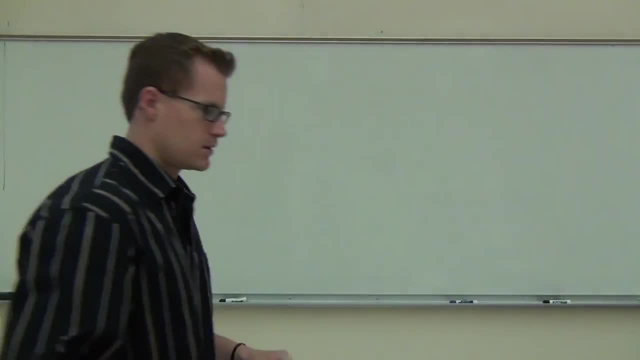 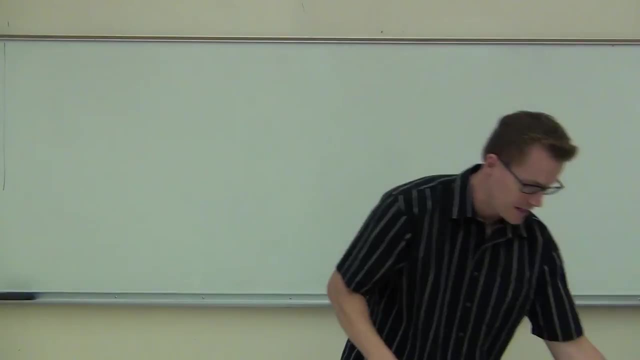 All right, guys, Have a great, great day. I'll see you tomorrow, All right, So I did say to make the term with the largest exponent positive And with that in mind, let's look at the next example. That's going to be this one. 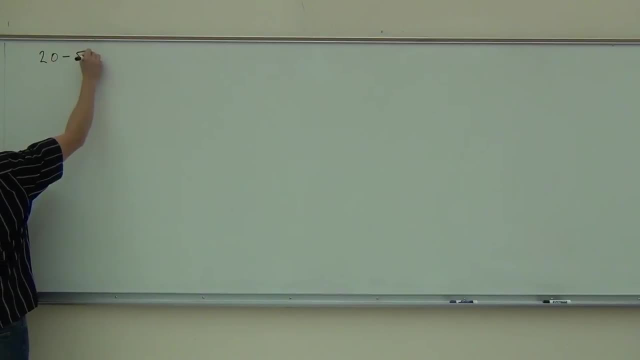 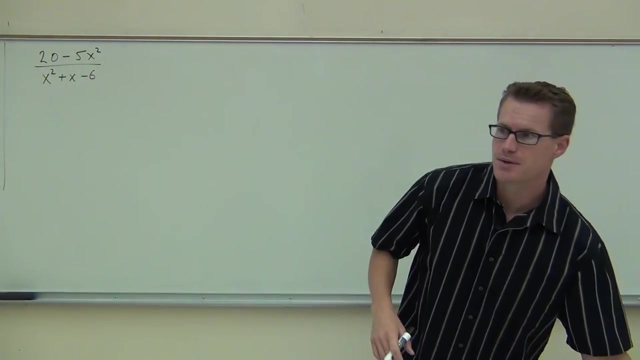 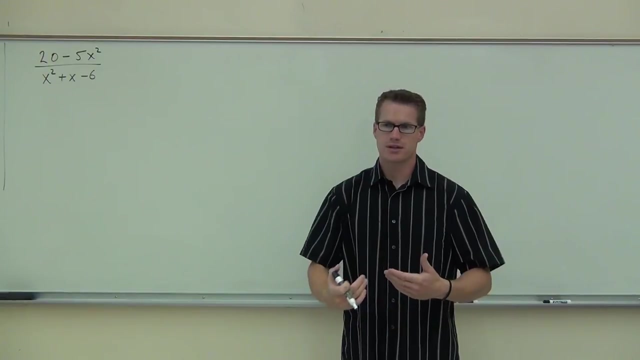 Now here's what I mean by that. When we look at this problem. of course, the first thing that we do when we simplify- I gave you these steps last time- is you have to factor both the numerator and denominator, because what you're going to be trying to do is simplify common factors, the factors, 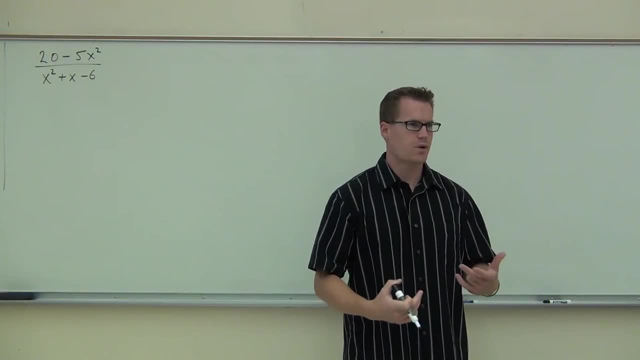 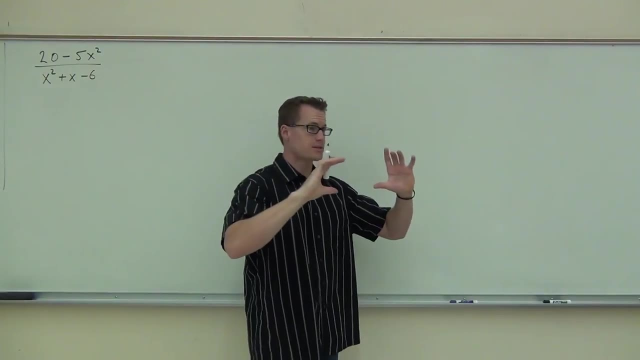 that are exactly the same. Now remember, it's not common terms, right? We can't just arbitrarily cross out x squared and x squared. We can't do that. It's things that are multiplied together that are exactly the same on the numerator and 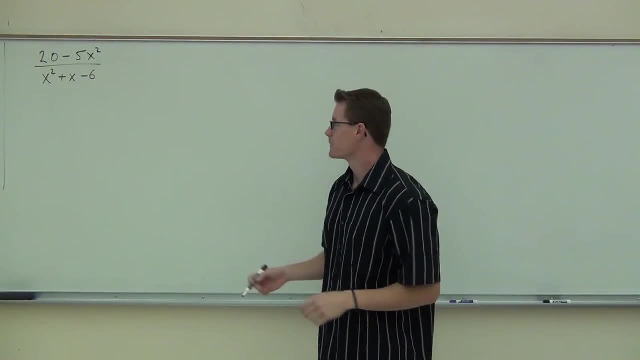 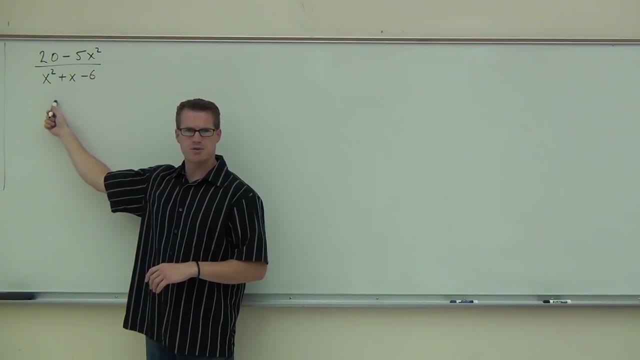 denominator, And that means we have to factor first everything. So when we look at the bottom we might be able to factor that one pretty easily with the diamond method. You guys see that already. Yeah, Is this going to have the extra step or not, do you think? 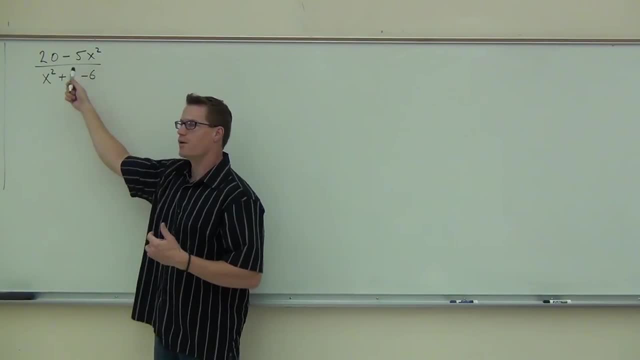 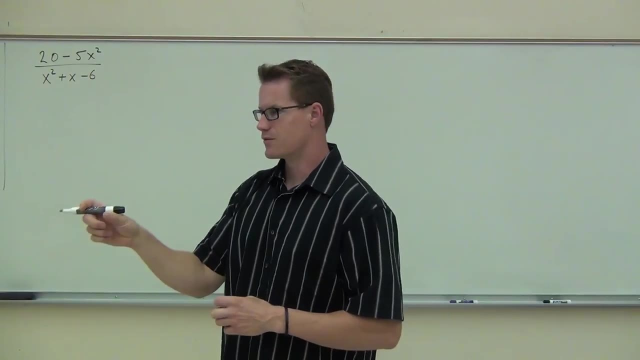 No, No, It's going to be pretty easy. The top one, though. would you look at that and look how the term with the exponent there, the term with the x squared, that's negative or has a minus in front of it. 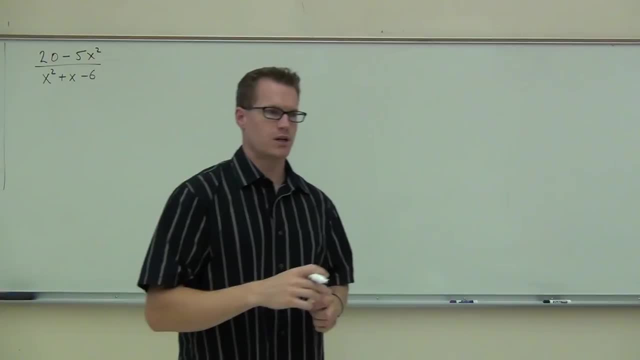 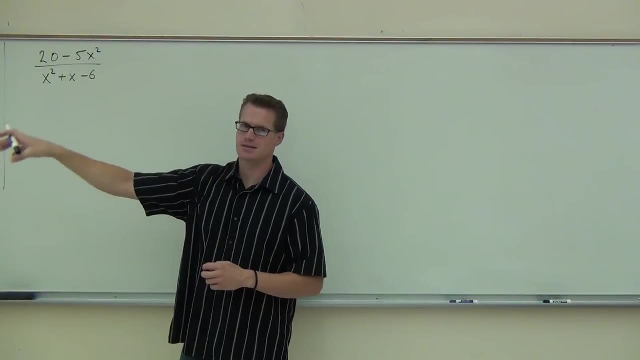 What we want to do to make this easier on ourselves is factor out a greatest common factor from that, but also take the negative out. Make that positive, because otherwise it's going to look like you can't simplify some things that we're actually going to be able to simplify. 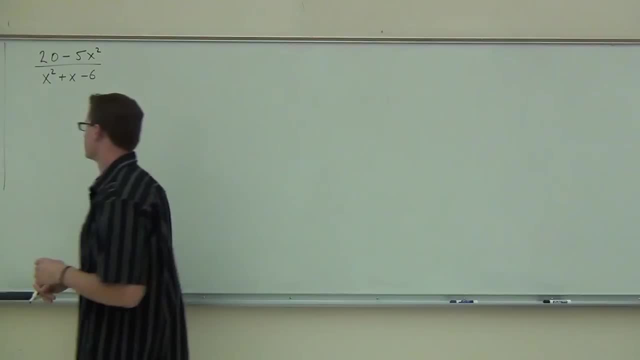 I might show you that in just a second. So let's look at the numerator here. Can you tell me what factors out of 20 minus 5x squared Five? Okay, We're not just going to take the five Negative. 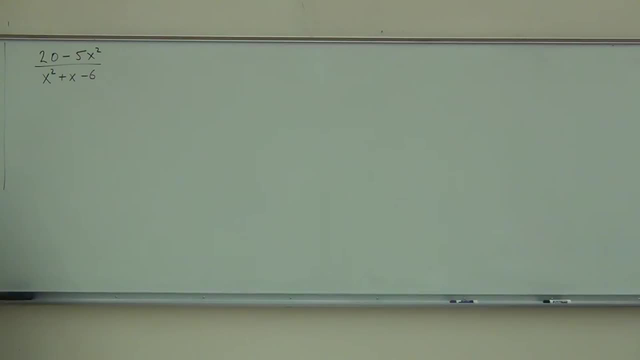 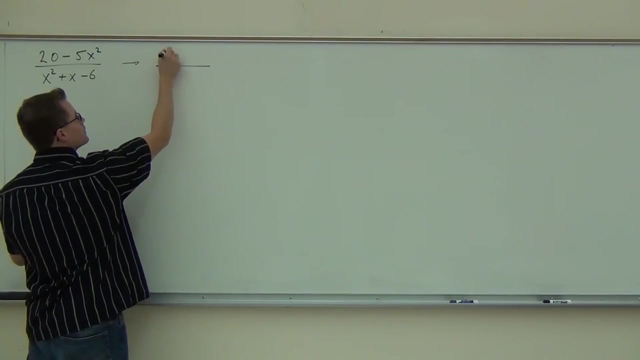 We're going to take the negative five. Okay, Let's see how that's going to look. Watch carefully: If we factor out 5,, we're going to get 4 minus x squared. You see that That's not exactly what I want. 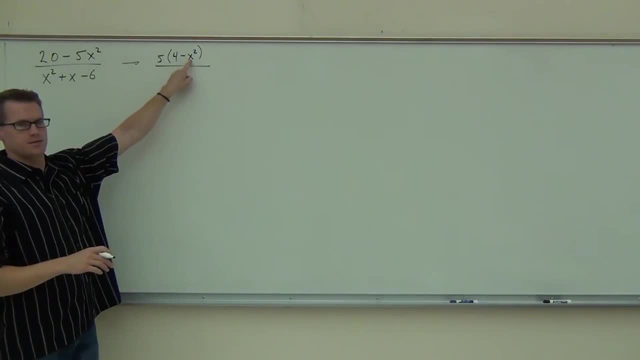 What I want is to make the x squared term positive. Make x squared term positive. You're going to see why in just a second. Right now, this is probably not apparent to you- that this is a difference of squares. Do you see a difference of squares here? 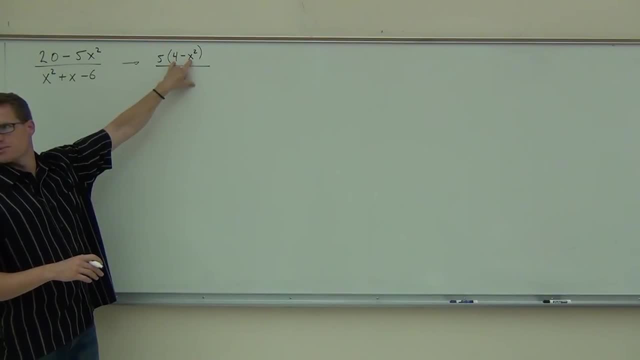 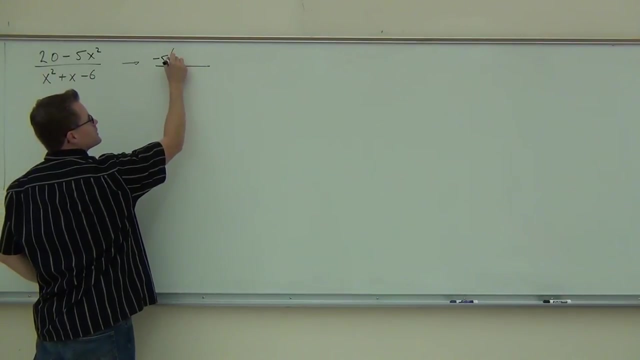 Some of you might. Some of you are like: what are you talking about? This is like giving squares to me. But if you factor out the negative 5, check it out, I'm going to rewrite this. If you factor out the negative 5, you get instead of 4, how much do you get there? 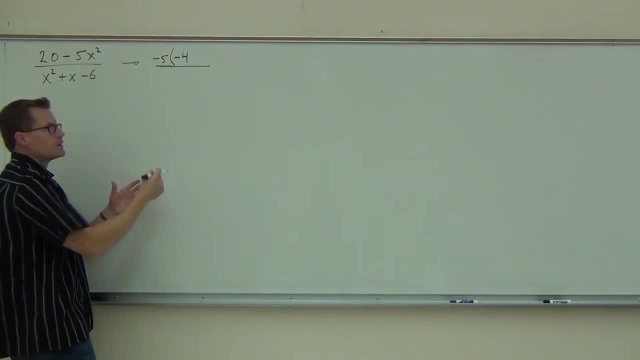 Negative 4.. Good, Now we're dividing and you're going to get plus x squared. You factored the negative out of it. It changed both sides inside You with me on this, folks. How many people are with me on that step, right there. 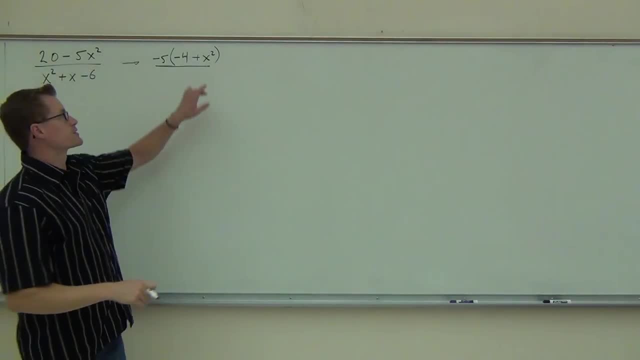 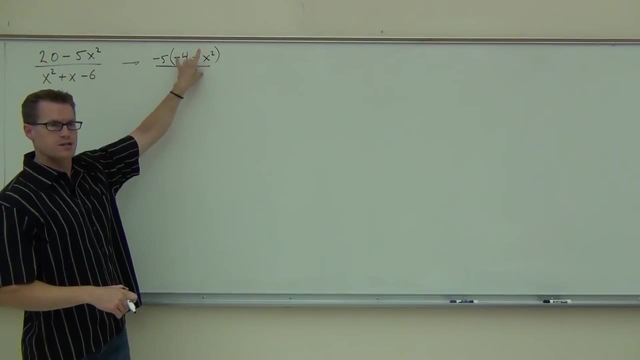 Good, OK. Now the last question I have for you about this: is it OK if I include the signs but flip these things around? Is that OK? So instead of negative 4 plus x squared, can I have x squared minus 4?? 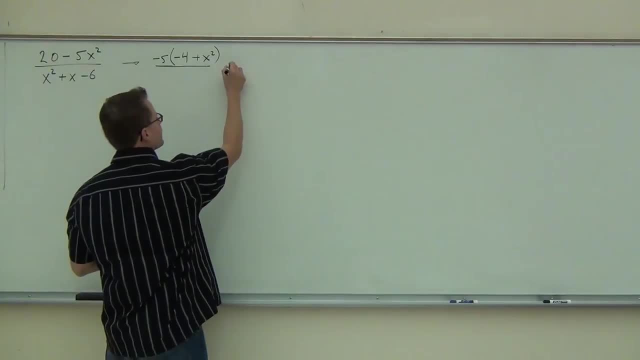 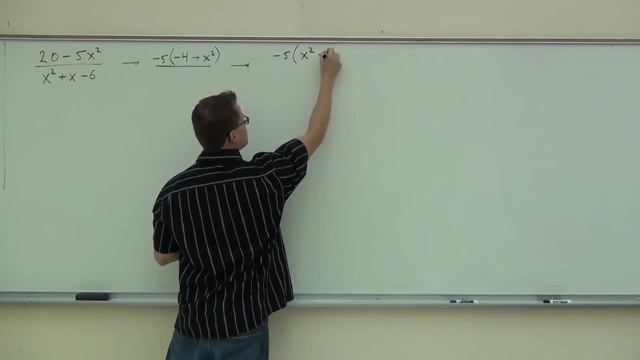 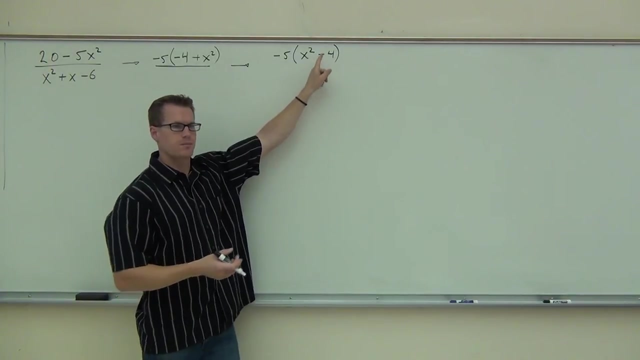 Yes, OK, I'm going to do that. So negative 5 stays there, x squared minus 4.. The reason why we do this, this thing, is a point. This thing is a whole lot easier to work with than this thing is. 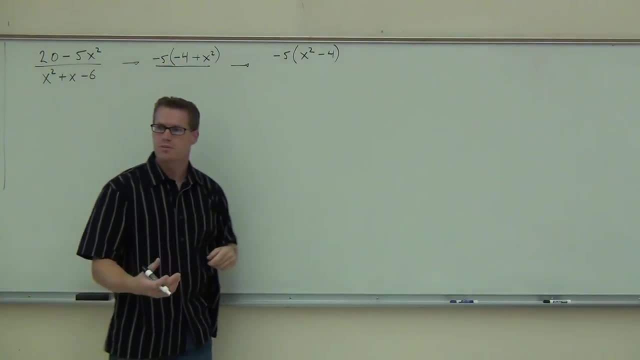 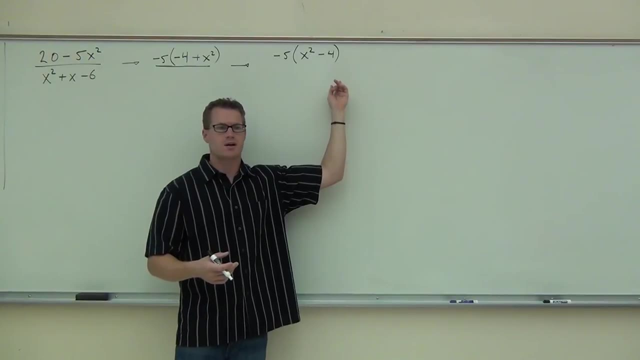 Oh well than the thing I had here before was. For most people this is a lot easier to see. that that's a difference of squares. Can you see it now a little bit easier? Yeah, And you know what. We're going to have to factor out a negative anyway. 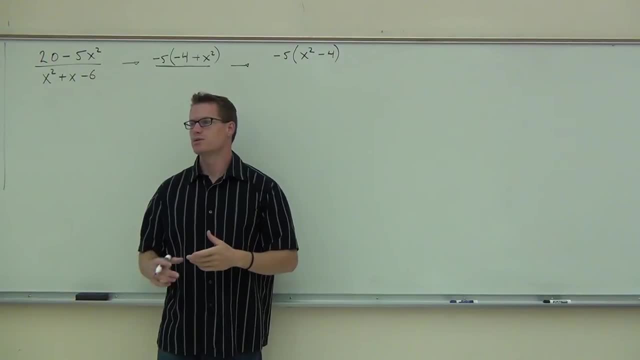 You're going to see this in a second. You are going to have to do that, So you may as well do it at the beginning rather than at the end. You're going to have to do it anyway, So do it at the very beginning. 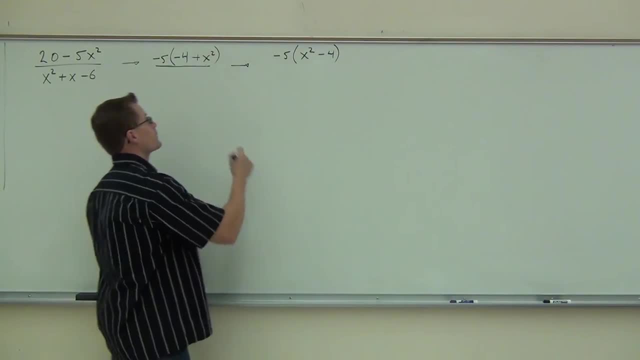 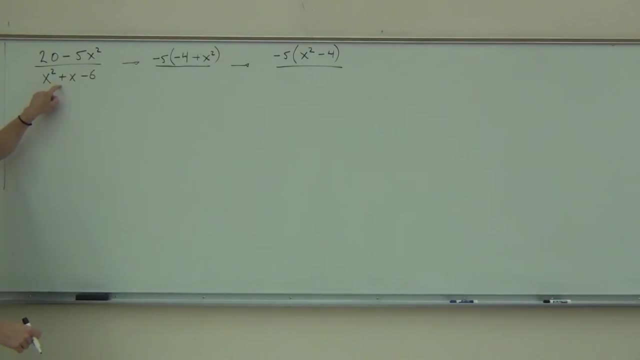 It's easier to work with and you don't make any mistakes on it. So we have the numerator done, Let's work on the denominator. now, With our denominator, can we factor that thing? Yeah, How, Denominator OK. 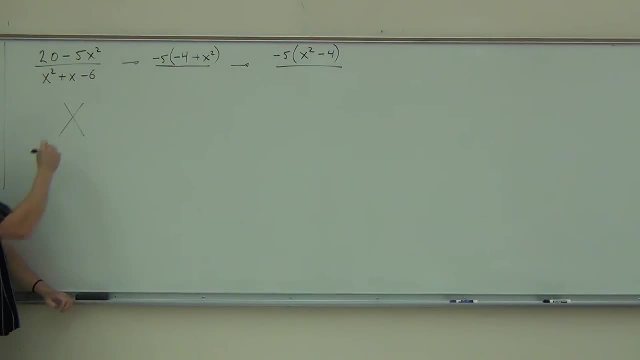 So let's do that. Can you all tell me what number goes on the top, please, 1. And on the bottom, Negative 6.. We look for two numbers. I'm going to start doing these more quickly because we've been practicing this for now. 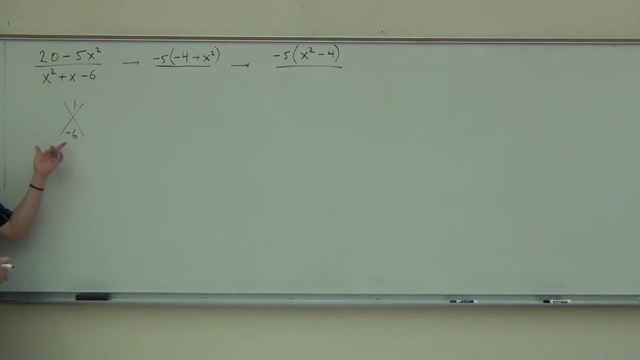 like every session, we've done The 1 and the negative 6, we're going to get 3 and 2.. 3 and 2.. 3 and 2 somehow. Yeah, It's going to be 3 and 2.. 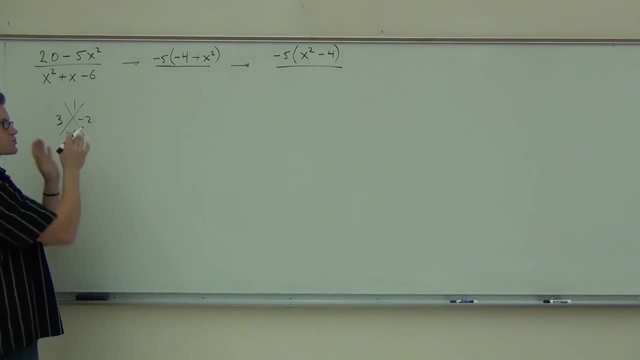 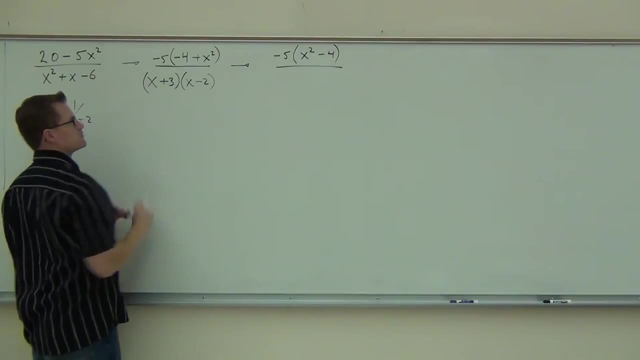 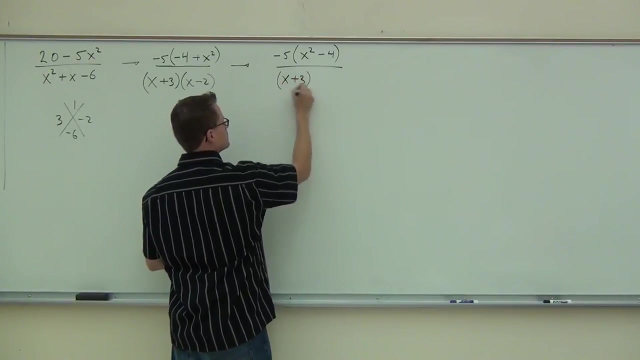 Now do I need to split this up and factor by grouping? No, No, This goes directly to my factor. So right here, I write x plus 3.. I write x minus 2.. And I can continue that on. Now, we did say factor completely. 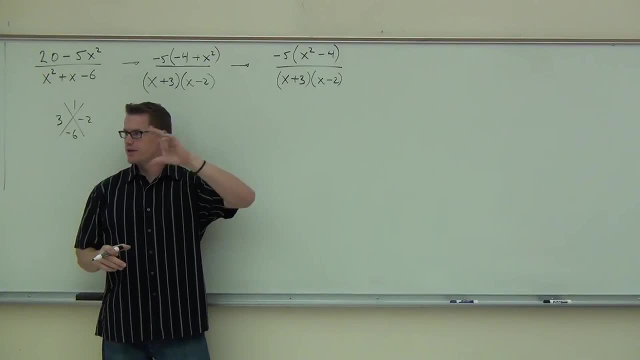 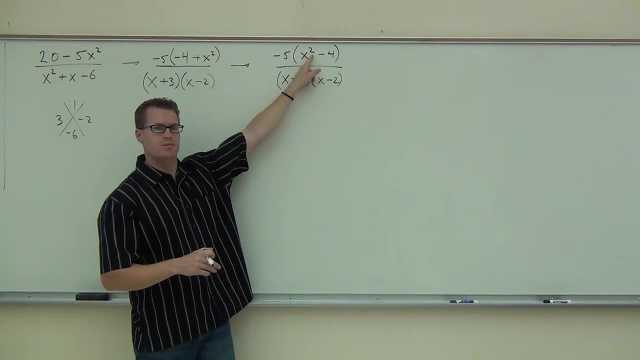 What we've done so far. We've factored out the negative out of the numerator, the negative 5.. We've factored the denominator completely. You can't do anything more with this, But there is something more I can do with that. the x squared minus 4.. 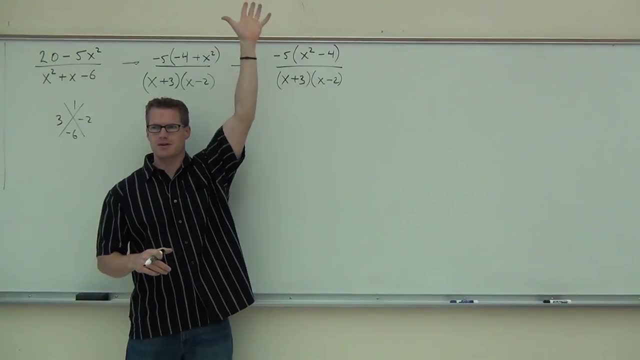 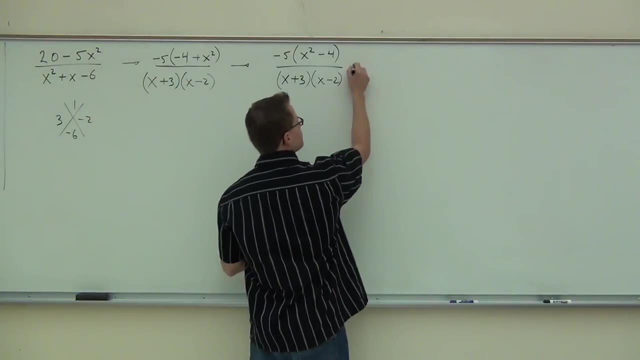 Do you remember how to factor that thing? How many people do remember how to factor that thing? I hope that you do. But that's the difference of squares, And you're going to start seeing this quicker and quicker as we go through this. 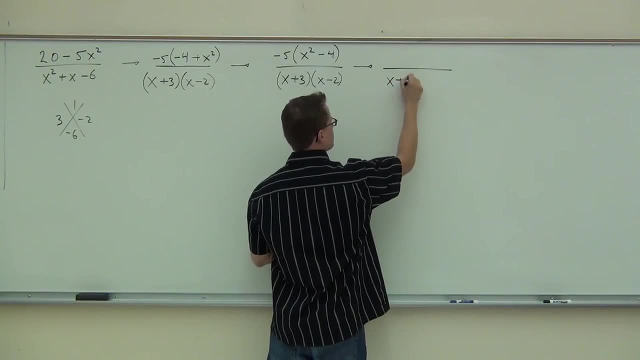 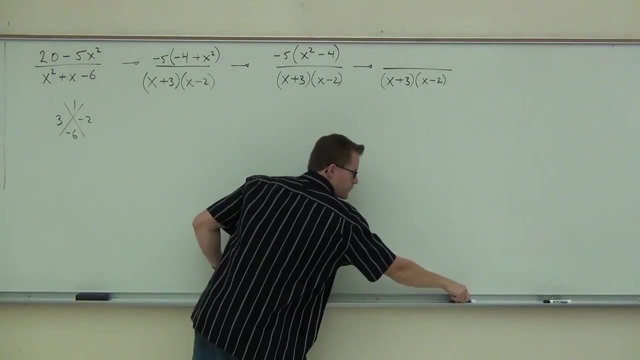 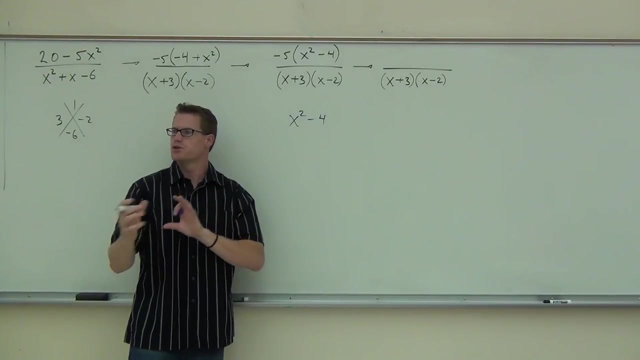 I'm going to take a little trip here, I'm going to take a little trip down here and do the factoring underneath this problem. So if I look at x squared minus 4, remember that a difference of squares is a difference of two squares, which means I'm really thinking of this as x squared minus 2 squared. 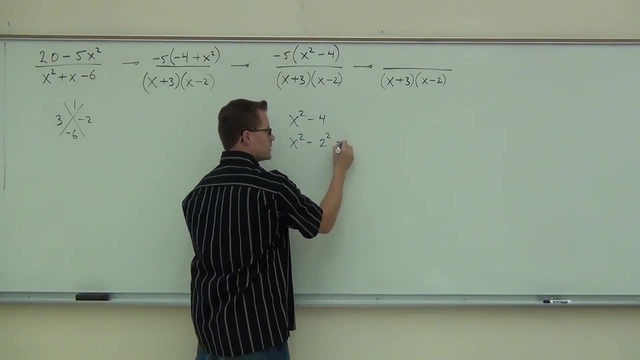 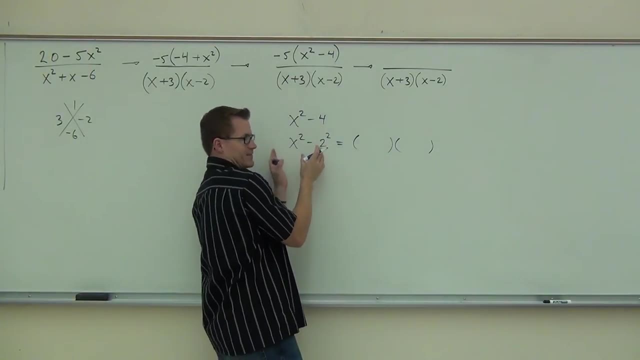 Same thing right Now. we've done this problem before in this class. When you factor a difference of squares, you end up getting two parentheses, just like here. but it's already kind of given to you what you're going to have. 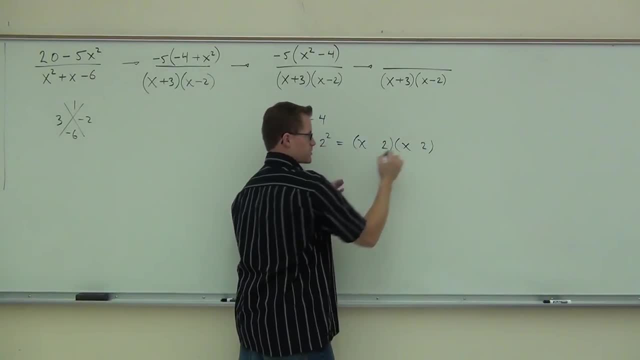 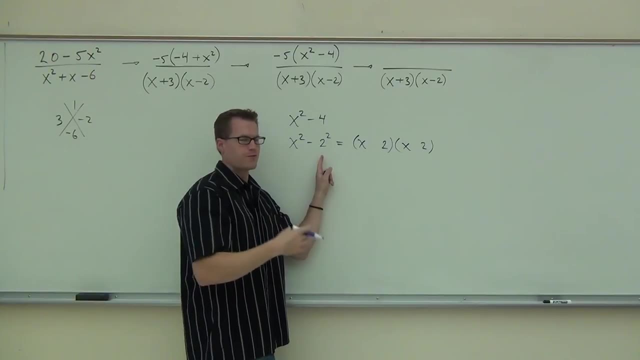 You're going to have an x in both spots. You're going to have a 2 in both spots, Not a 4, a 2, the thing that's actually being squared, That's the number you put there. I gave you the form a squared minus b squared when I first introduced this. 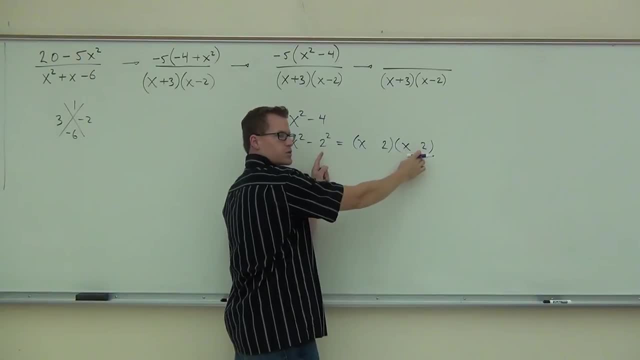 So this acts as our b. in this case, We have a 2 and a 2.. Notice, when we multiply, that's giving us the value of 4.. Are you with me on that? The only thing you have to remember is that one of these signs is a plus and one of these signs is a minus. 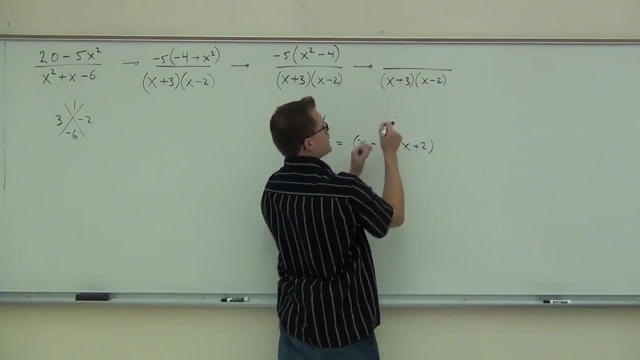 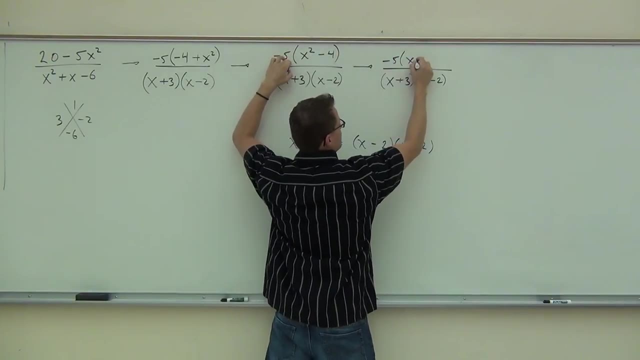 That's how you factor a difference of squares. So this is going to go on the top with this negative 5.. So the negative 5 is still there. We'll be factoring this as x minus 2, x plus 2.. 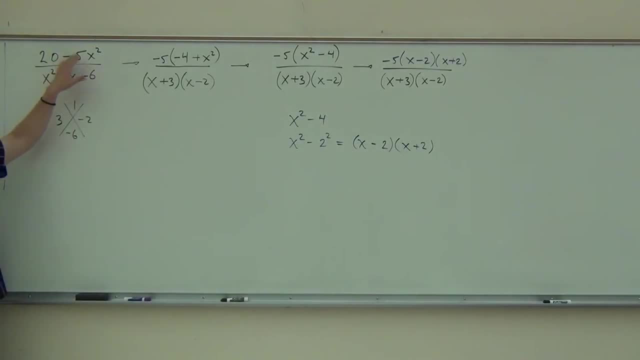 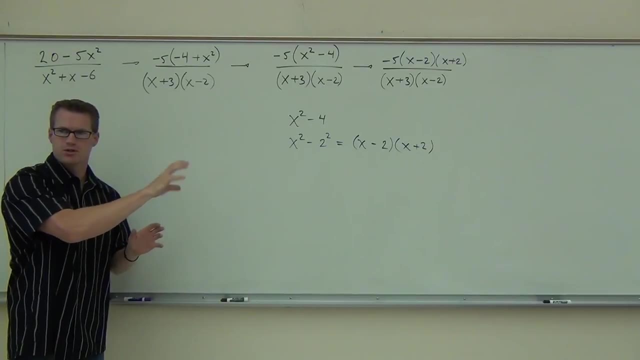 So let's take a little recap about what we did. We noticed that we really do want to make the x squared term positive. If we do that, trust me, it's easier to work with. I'll show you in a second. If you really need me to prove it to you, I'll show you that in a second. 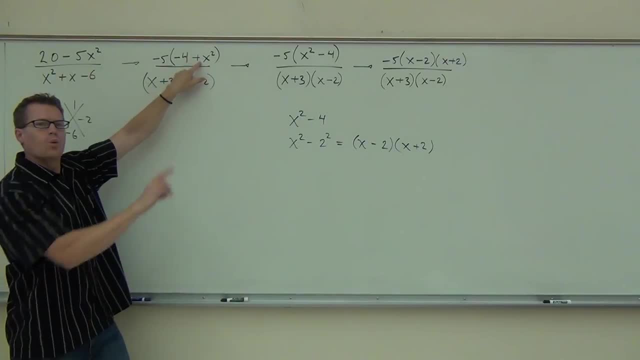 So we factor out the negative, making the x squared term positive. We're going to switch it around to write the x terms first. That way it's easy to factor. So that's the only thing we're doing from here to here. 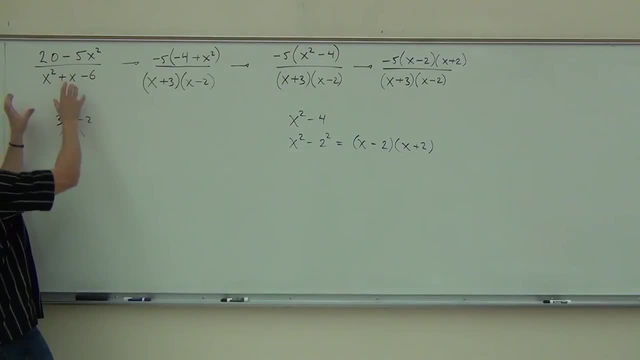 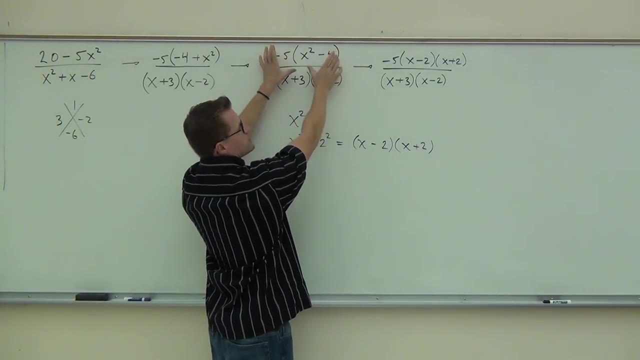 I've switched these terms around On the denominator diamond method because we have three terms. no problem, There's no extra step. That's actually a pretty easy one. We get down to here. We make sure we factor our numerator completely. 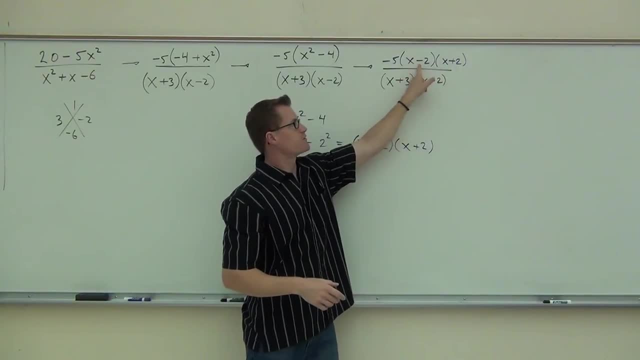 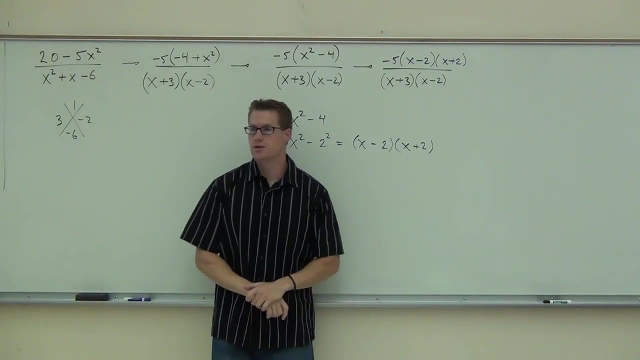 That's the difference of squares. And now we're all the way down to here. Each of these factors is factored completely. How many people feel: okay, getting down to that far, Good, All right. Is there anything else that we can do? 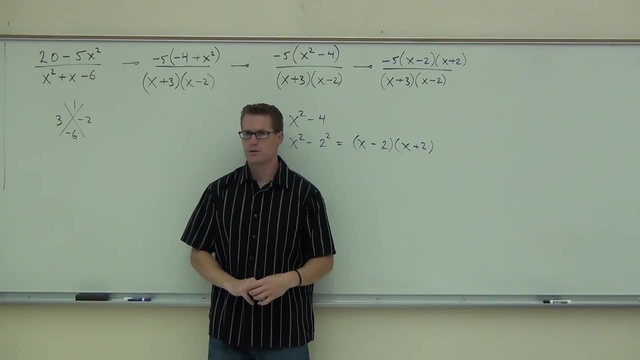 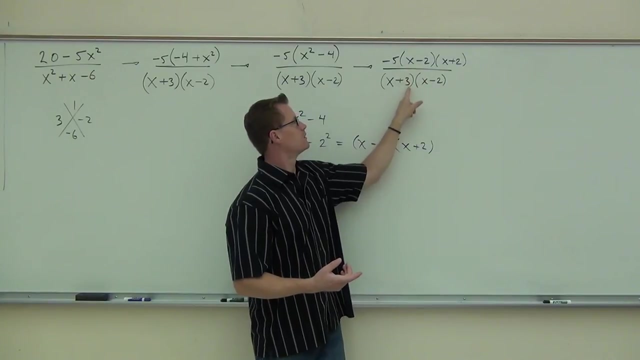 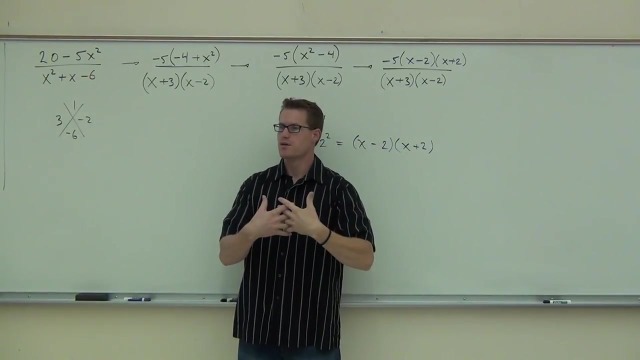 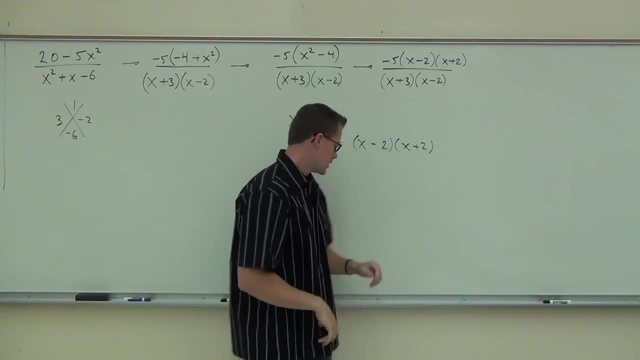 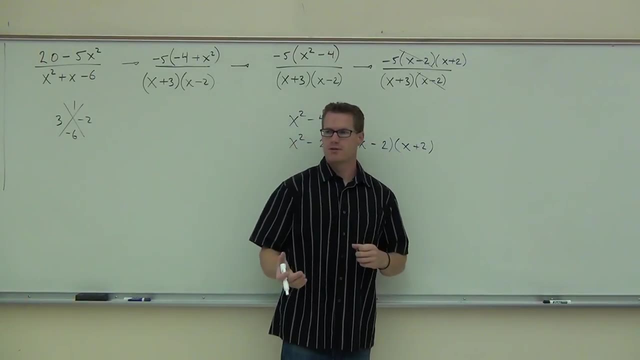 Entire things or nothing at all. That's all we need. So here, since we have our x minus 2s- you all see that Those are gone- Just rewrite whatever you have left over. You don't need to distribute. You spent so much time factoring. 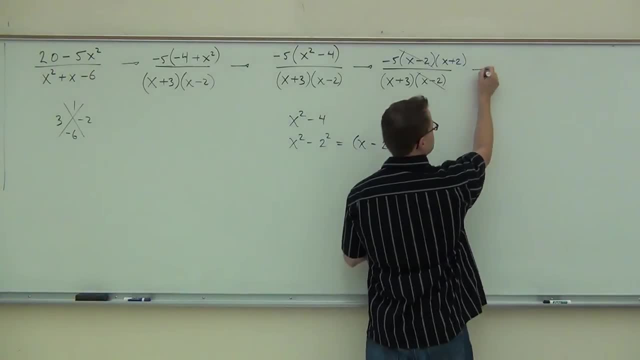 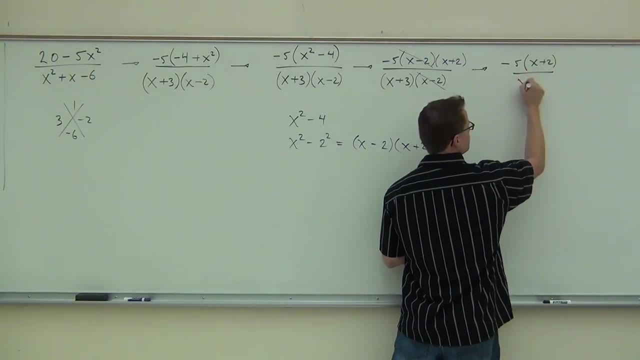 Don't distribute that back in, Just leave it. We spent a lot of time factoring this class. Leave it back here. Negative: 5 times x plus 2, all over x plus 3.. You'll notice I had to leave the parentheses here. 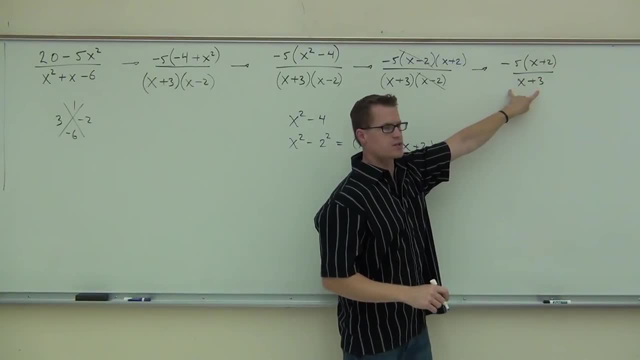 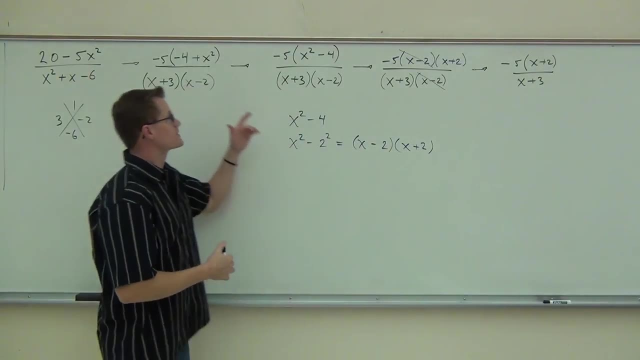 Because that negative 5 was up front, But here I don't need the parentheses because that's the only factor we had left. You feel still okay with this? Yes, Okay. Now I would like to show you why this step is kind of important. 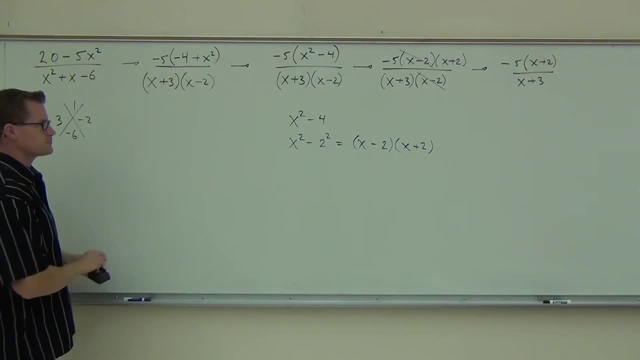 Would you like to see it real quick? Yes, Okay, Here's the why. Let's say that I did factor out the negative 5.. You're still going to have to do the problem, However. you're still going to have to factor out a negative 2.. 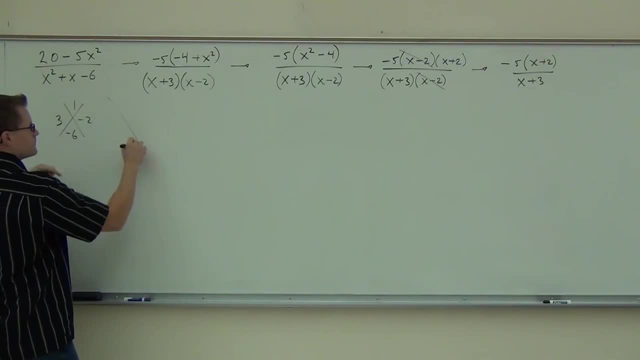 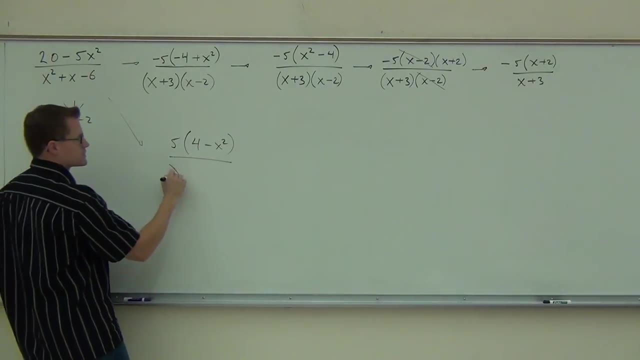 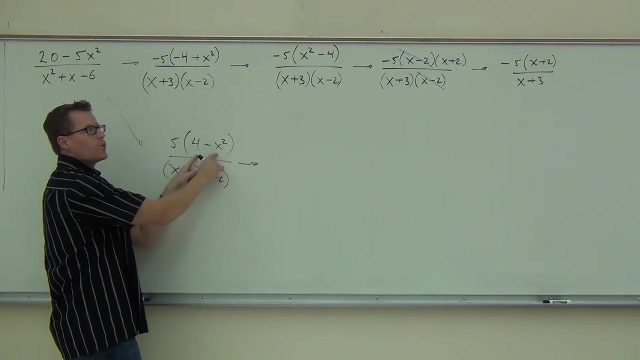 You'll see what I mean. If I go right down here and I factor out a positive 5, I'm going to get 4 minus x squared. This thing's going to factor exactly the same. This actually still is a difference of squares, only it doesn't factor as x minus 2, x plus 2.. 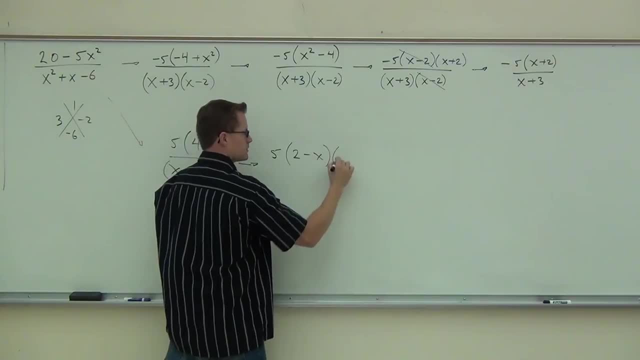 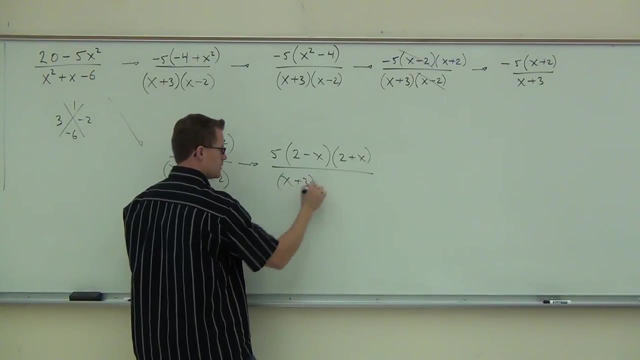 What it factors as is 2 minus x, 2 plus x. Do you see the difference there? Then, when you have down here this, x plus 3, x minus 2.. My question is: do these things simplify? No, No, they're not exactly the same. 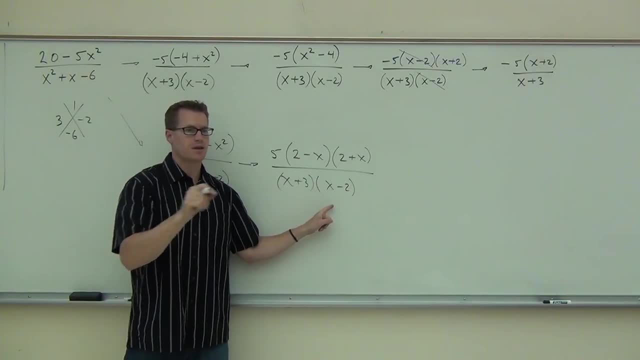 This is the thing I gave you last time. I said: oh, you know what, If you have the values exactly the same but the signs are different, you have to factor out a negative 1 here to make them the same. Do you remember that from last time? 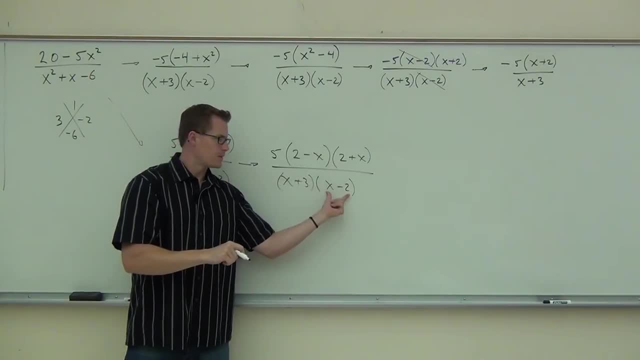 No, So you've got to do it anyway. So right here you'd go. oh, okay, From here I need to factor a negative 1. People seem not to really grasp this concept as well, which is why I gave you it this way. 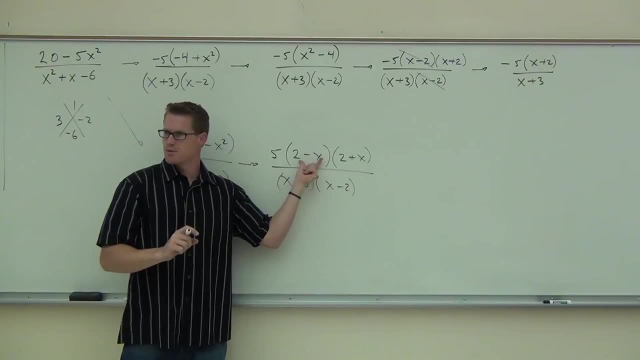 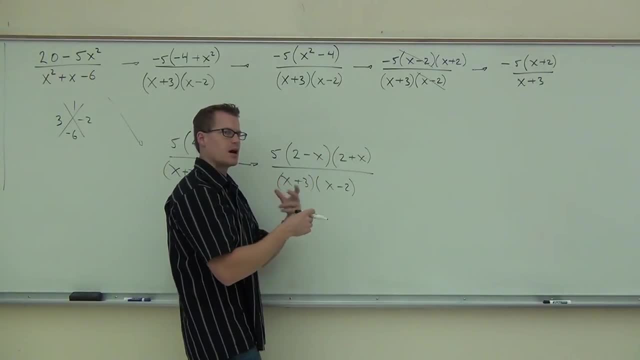 I'm going to do this. If you go, okay, I'm going to pull a negative 1 out, But what it's going to do is make that a negative 5.. Do you see that This one is going to become x minus 2, and then 2 plus x? 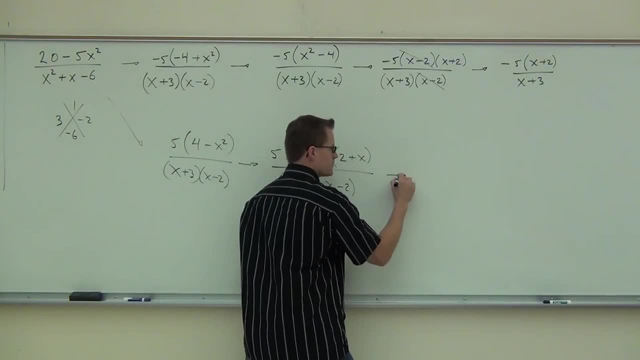 And a lot of people ask me: well, how do you get from here to here? What are you even doing? And the thing I'm doing is I'm factoring out a negative 1.. That's why I gave you this. I've got to do the same thing. 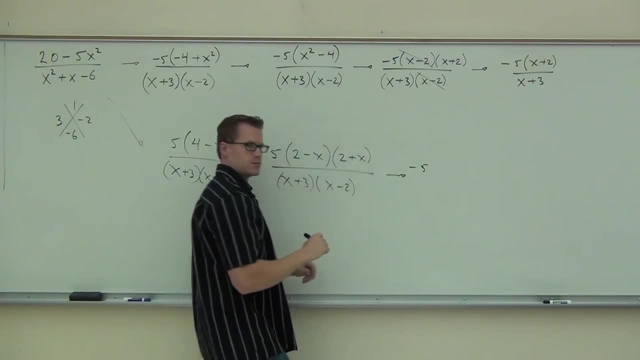 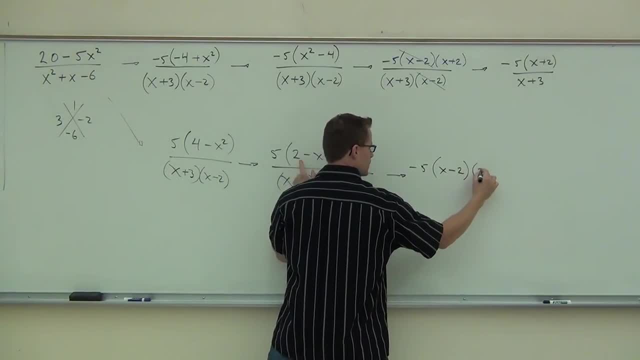 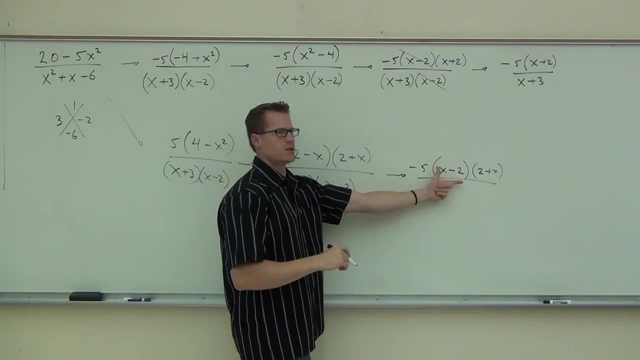 I'm going to do this minus 2, and then 2 plus x, And a lot of people ask me: well, how do you get from here to here? What are you even doing? And the thing I'm doing is I'm factoring out a negative 1.. 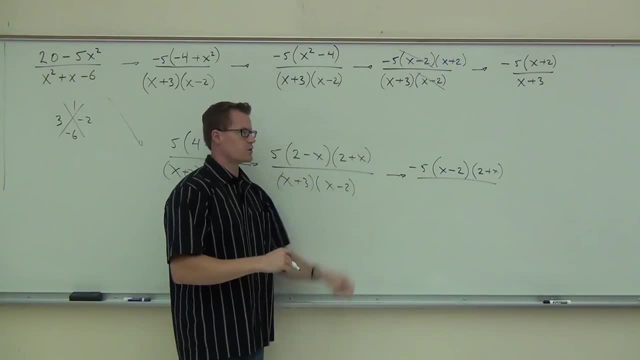 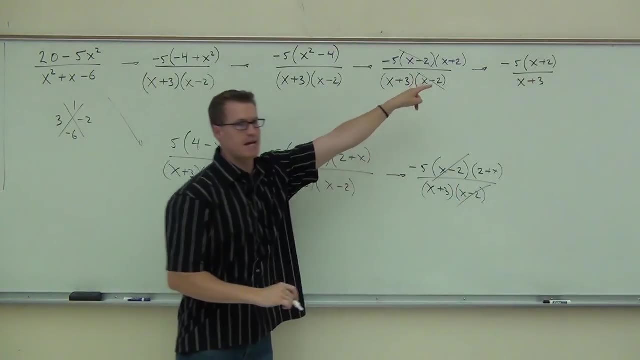 It's changing both of these signs. I'm reordering it. The negative 1 is going out front. Now you can simplify those and we get exactly the same answer. It's only these two things are switched around, which is fine, because that's addition. 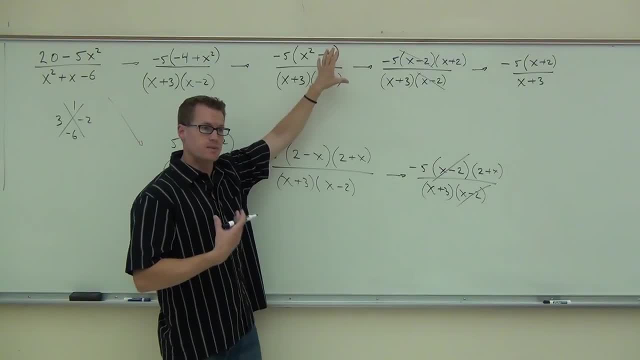 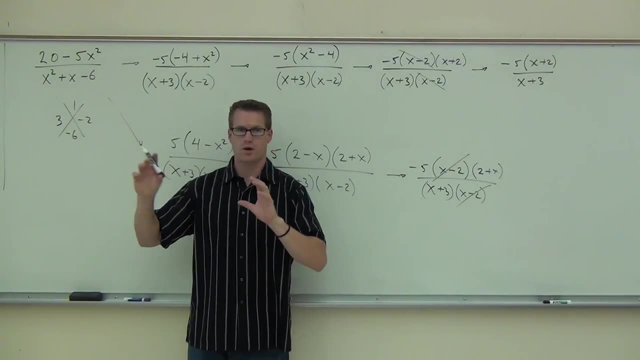 Now, to me this way seems a whole lot easier to do To me. I don't like going to the end to factor out a negative 1.. I like factoring out the negative in the beginning, making sure your largest power is positive. 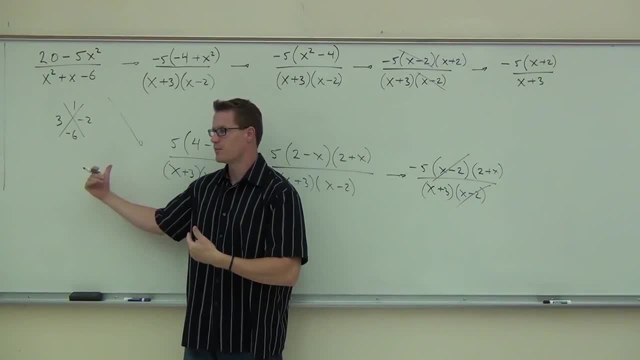 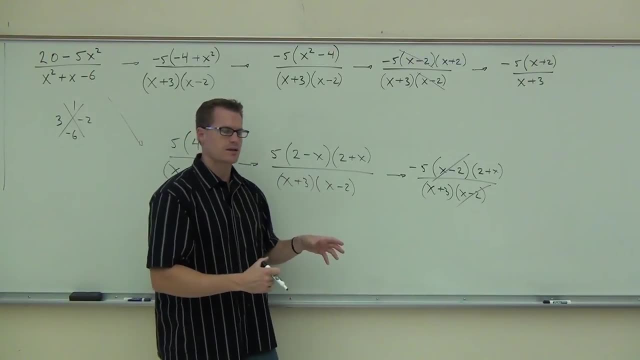 It's way easier to factor, especially if you have to use a diamond problem, and we end up getting the right answer without a whole lot of extra work. Do you see the point in that? So that statement I made last part of class. 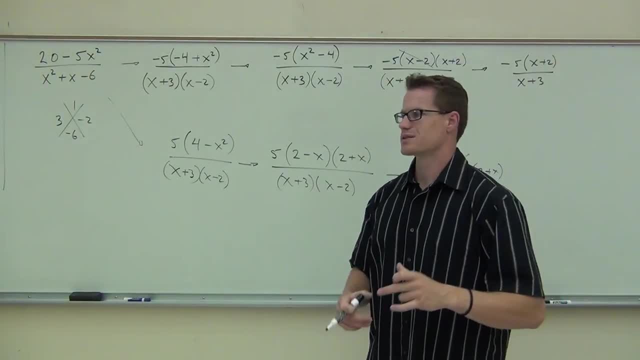 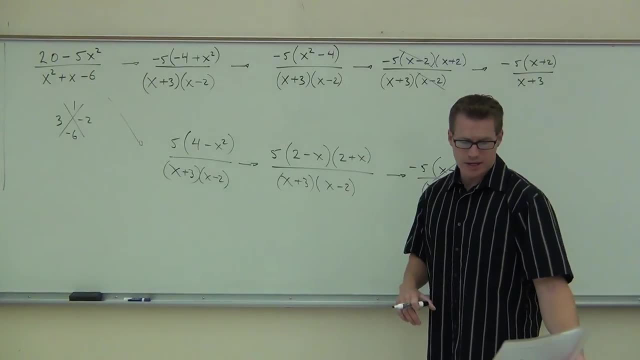 factor, so you get the term with the largest x1 positive. it's kind of a nice easy deal for us. Okay, let's go ahead and move on. What I'd like to do. I would like to give you a couple examples. 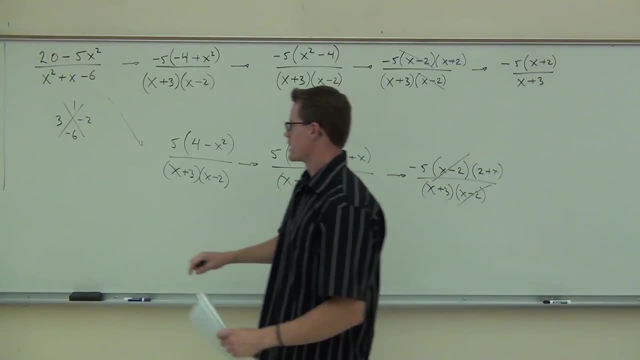 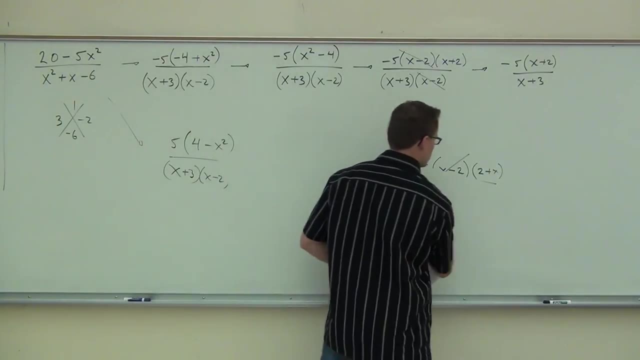 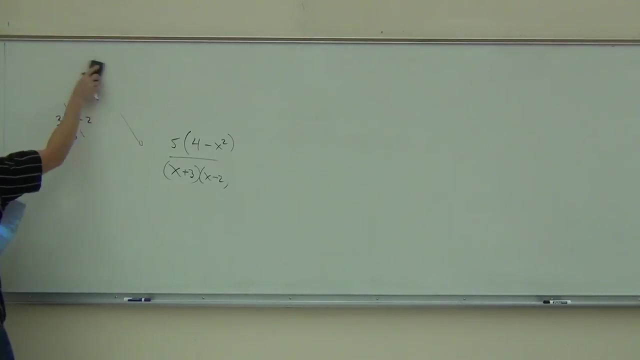 on your own. Are you ready for a couple examples on your own? One's going to kind of refresh your memory about what we did yesterday, and one's going to be similar to this one. Okay, so I'd like to do that, factor that one and simplify it. 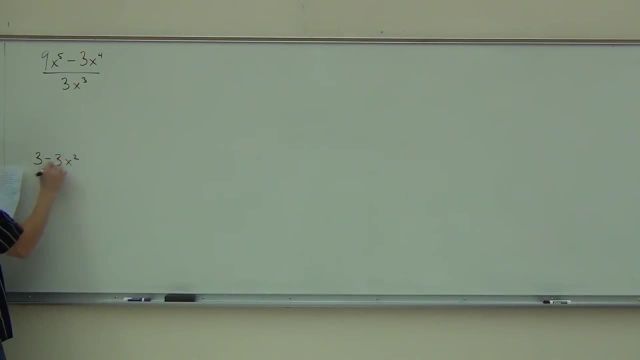 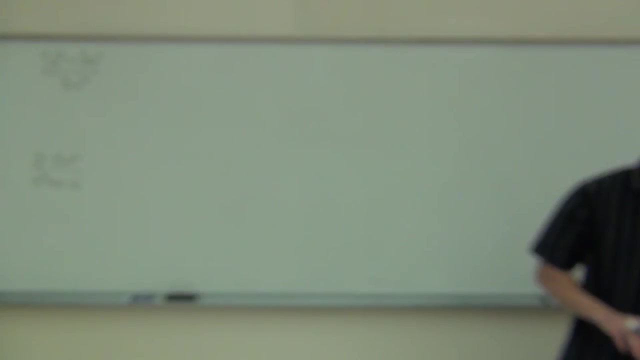 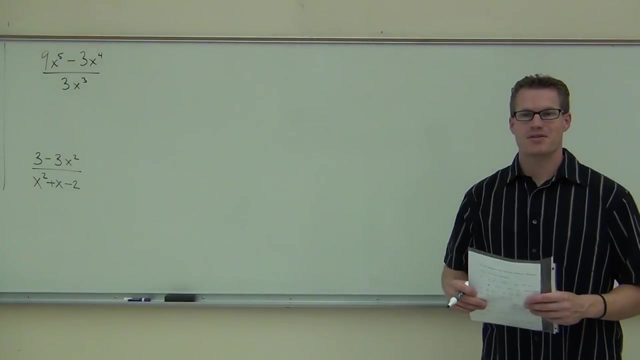 and then do this one, And if you want to be brave after that, if you finish these things early, there's another one we're going to do together. right now I'm actually going to go through and show you how to factor a sum. 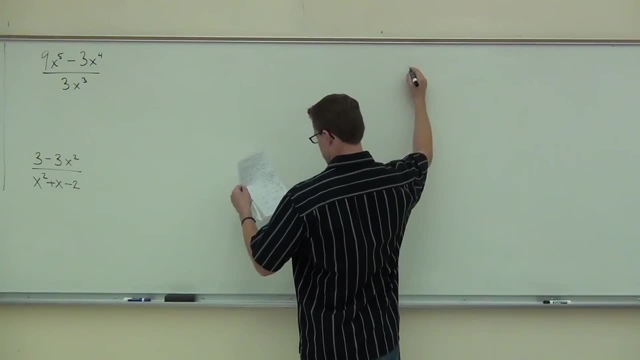 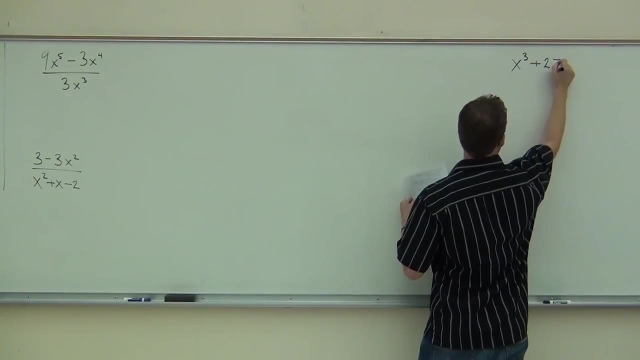 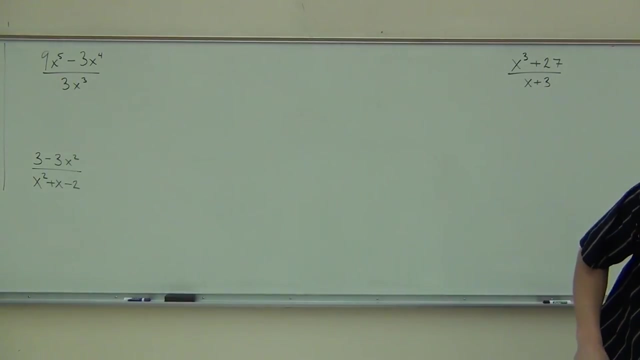 of cubes in a problem. Okay, so I'm going to go through and show you how to do that. Okay, so I'm going to go through and show you how to do that. So in each case we're trying to factor the numerator. 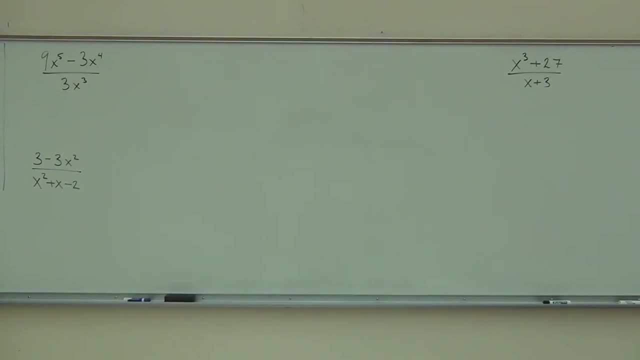 and the denominator completely. That's very important, You know. so you're going to try to factor each of the terms with the largest exponent positive. If the term with the largest exponent is already positive, well that's great, You don't need to factor out a negative. but if it's not, 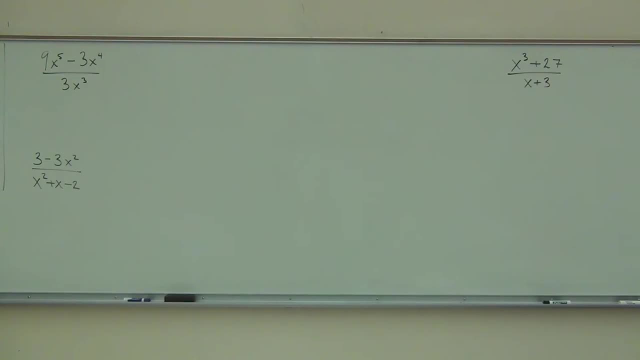 then you're going to have to do that, So you're going to want to factor out a negative. That's the whole idea here. It's barely still. It's barely still. It's barely still So in theногоing unit value four. 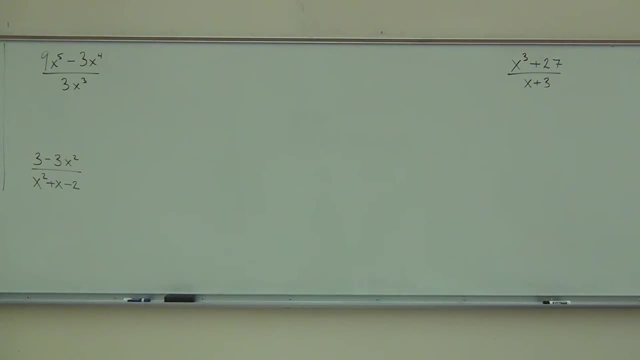 I'm going to give you about one more minute. Let's see how far we can get One more minute, Okay, so Can you see how far we've gone? I know it's been a minute, Thank you, Okay. we're going to get started here on the first one. 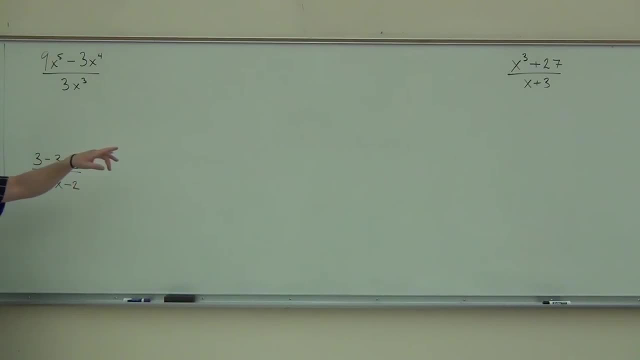 If you're still working on the second one, that's okay. If you're on the third one, that's great. If you know how to do that one, that's awesome. That's it. That's one of those cubes that we were talking about. 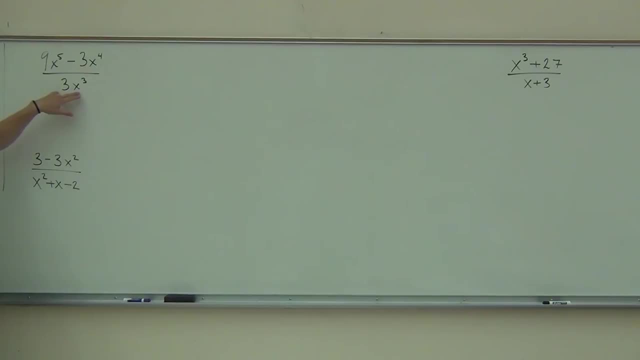 So on the first example, of course, on the denominator, we can't factor that. It's going to stay the same. Hopefully we're going to simplify that out. On the numerator, though, there are some things we can factor out. 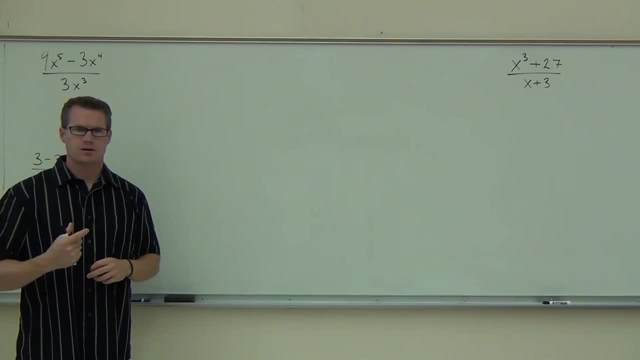 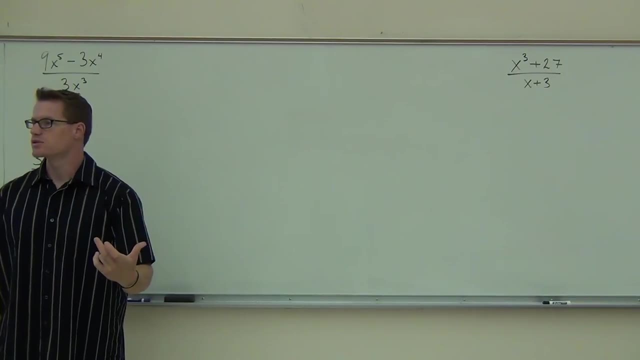 Now the question is: do I need to factor out a negative or not? No, Do you see how the largest term is already positive? The x-fold with the largest term is already positive. That's what we want to happen, So we don't need to factor out a negative there. 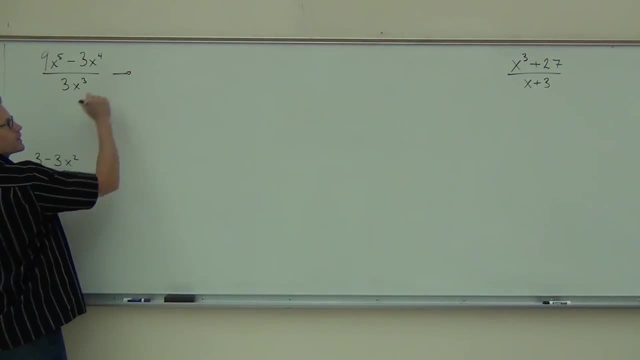 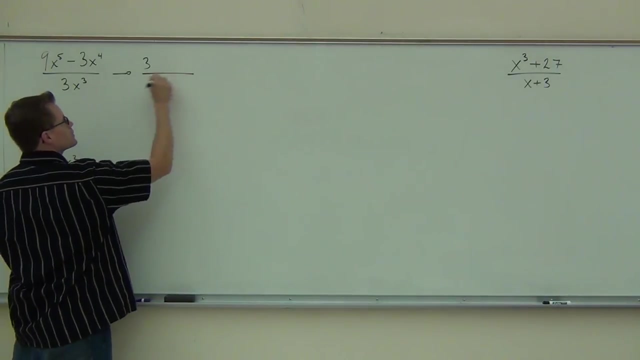 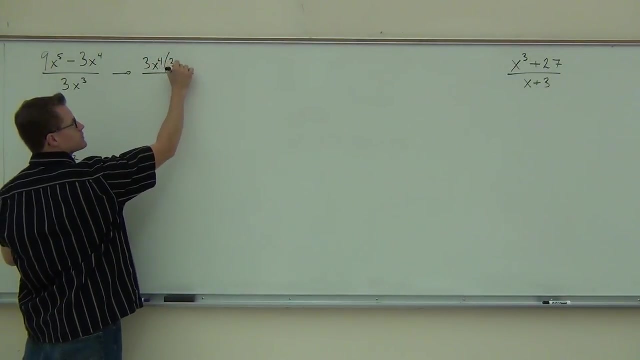 That's fine. So we're just going to factor out What Three Great Any x's You're going to take the biggest one that's common to both. What's that And what we have remaining is: Did you get that far? 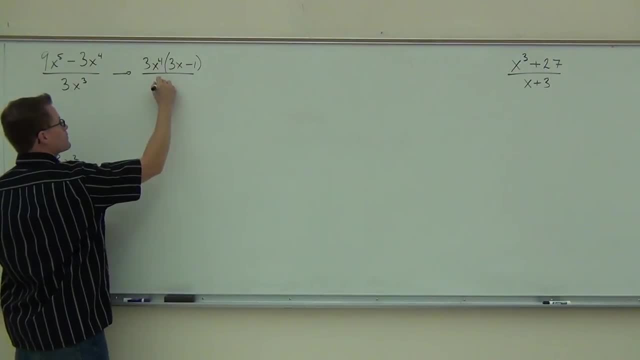 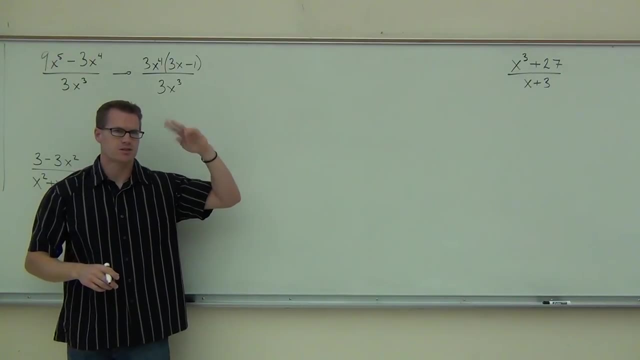 How many people did? Good, All right, On the denominator, we have 3x to the third. Does anything simplify? This is like one of those ones we had yesterday, only kind of in reverse. actually It's good We have 3x. 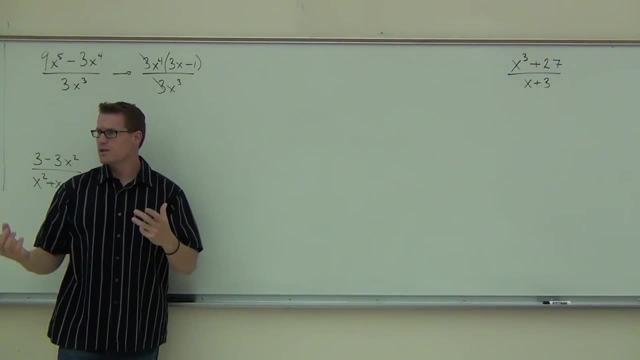 3. 3x to the fourth is gone. Yeah, 3s are definitely gone: The x to the cube and the x to the fourth. we can also simplify that. Okay, Those are factors in this case. So x to the third is gone. 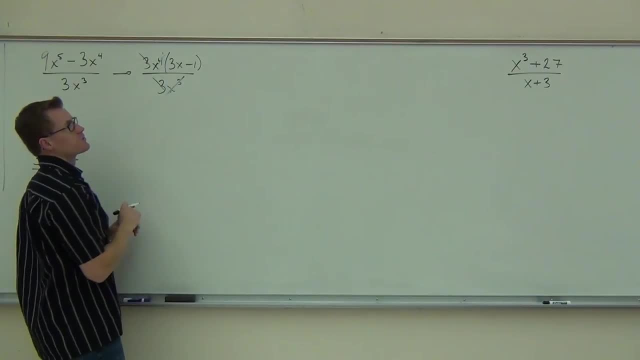 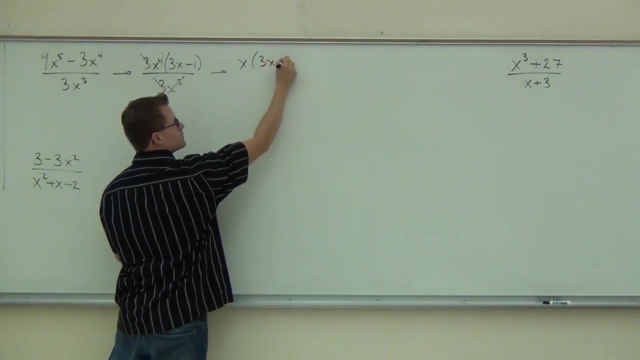 The x to the fourth becomes Negative. Just x to the first power. Just don't forget about that. Remember to write that x. So here we're going to have x, 3x minus 1.. You can put it over 1 if you'd like to. 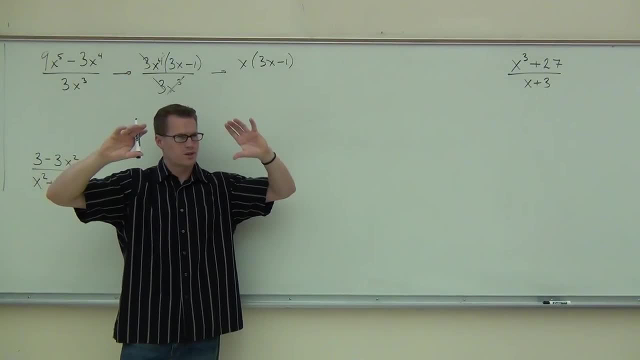 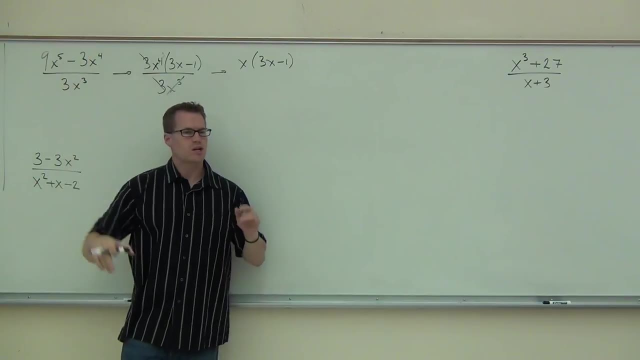 But since this is some expression over 1, you really don't need that 1.. So if you get this far, you're done. How many people did get that far in that problem? That's good, If you didn't check this problem out later. 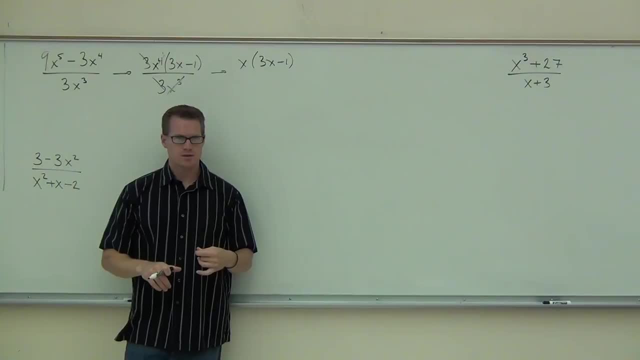 Make sure you can do this, Make sure you can get down that far. Are you guys okay on this one? Do you have any questions on this one? So if we put it over 1, you would still accept it as correct. 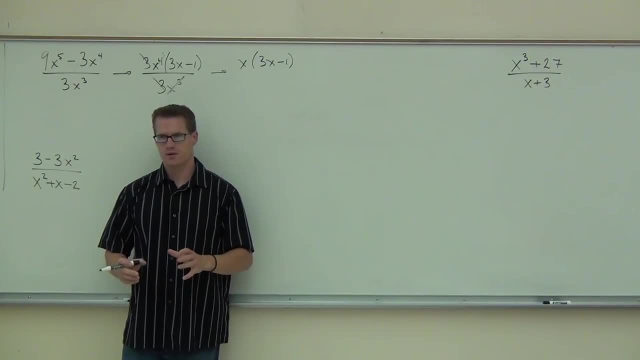 If you put it over 1, I would like for you to see that the 1 is really irrelevant here, So it's not necessary. Yeah, Under 1, that's a different story. Right, Okay, That's important. 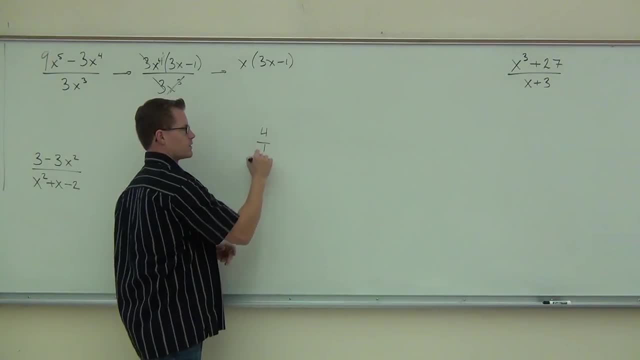 Right, But over 1, it's like doing this. My answer is 4 over 1.. What's your actual answer? You say 4.. Now, if your answer was 1 over 4.. Okay, You say my answer is 4?. 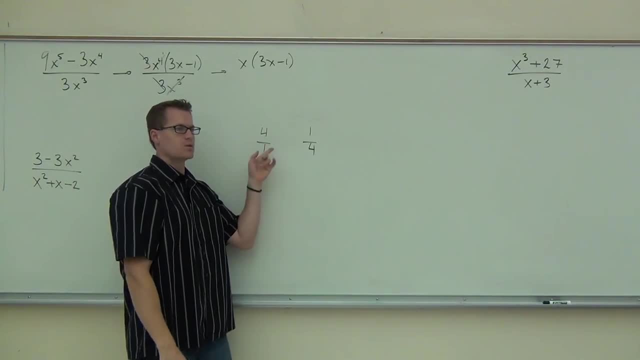 No, That's a different story. So if it's over 1, like that, you really don't need the 1.. Okay, If it's under 1, yeah, you certainly need the 1.. Okay, That's the difference. 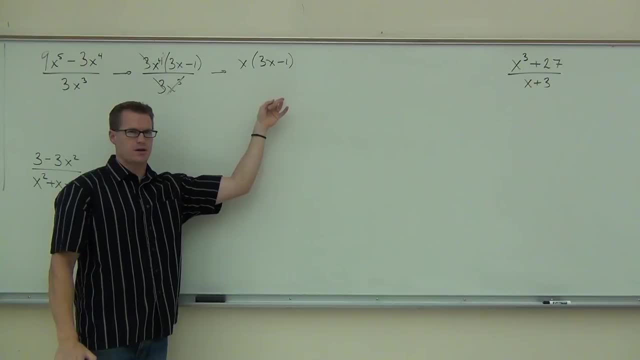 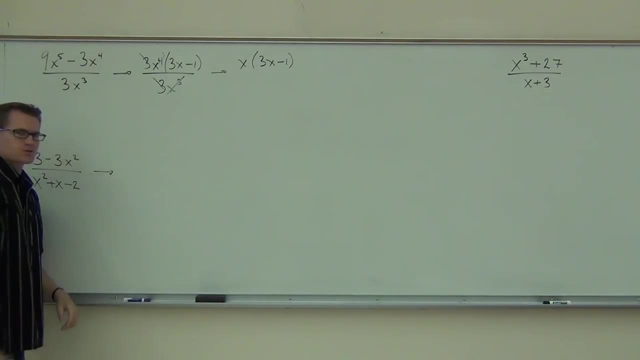 So our answer here is just like that. I'm not sure if you're okay with that. Yeah, Right Now. the next one's a little bit more work. Next one says: let's look at a numerator. Notice how our x squared term, the term with the largest power. 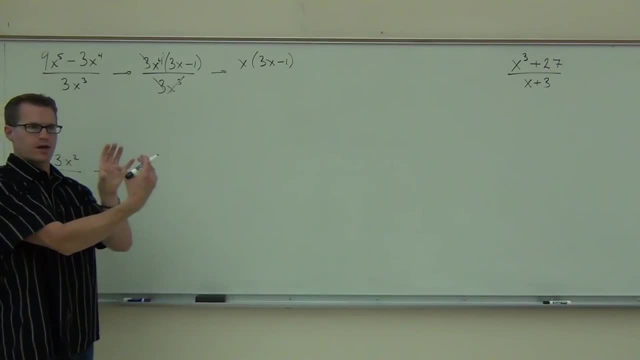 has a minus. It has a minus in front of it, or what we consider to be the negative root of that term. What we're going to do here, what that tells me to do, you're going to factor out a negative. Did you try to factor out a negative from that? 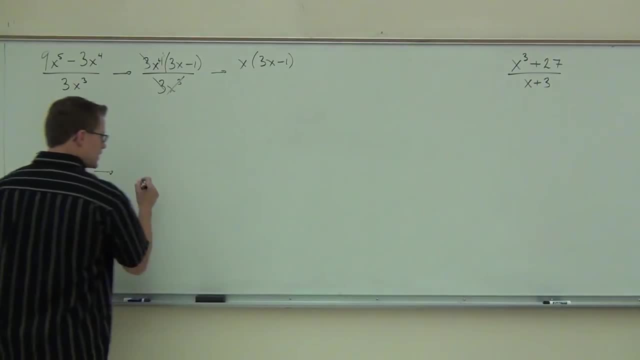 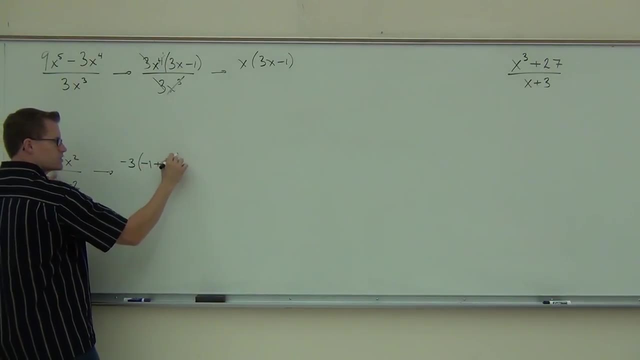 Yes, Negative, what Negative 3.. So if we factor out negative 3, you'll get: from here, you'll get negative 1. From here, you'll get plus x squared. Do you see why the signs change? 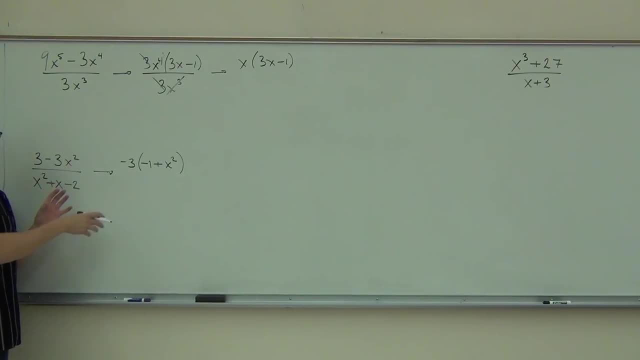 I don't know. Do you see why the signs change? folks Factor in that negative. Yeah, Why didn't the top one do that? Well, because we didn't factor out a negative. Why didn't the top one do that? 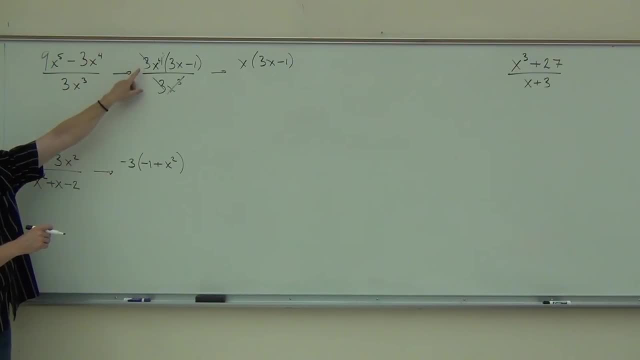 We factored out the positive 3 instead of the negative 3.. Do you see what we're talking about Here? we're factoring out negative 3.. We're dividing by a negative there. That's going to change these two inside signs. 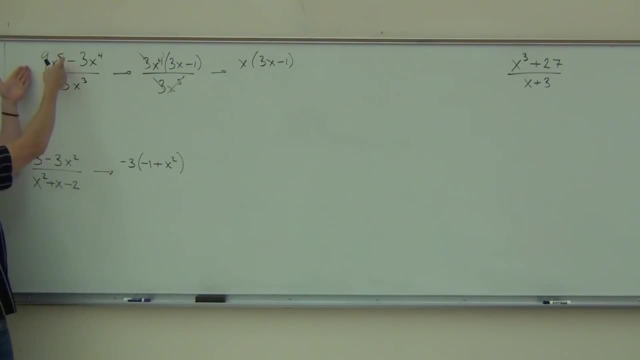 Here we're not doing that. We're factoring out positive. 3. Because the term with the largest exponent is already positive. that's what we want to see. Go ahead, Okay. So if your term with the largest exponent is negative, like right here it is. 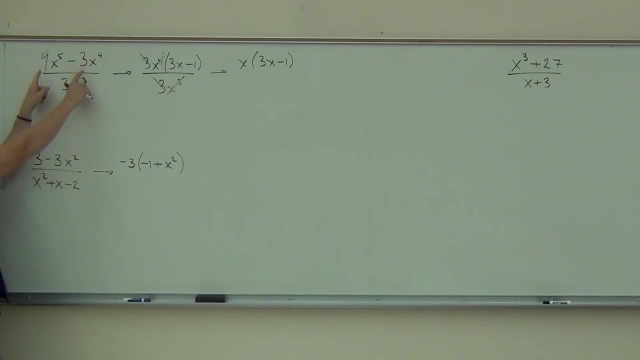 x squared is negative. Factor the negative. It's going to change the signs Here. it's not. x to the 5th is positive. You leave it alone. You factor out just a regular whole number, not an integer. okay. 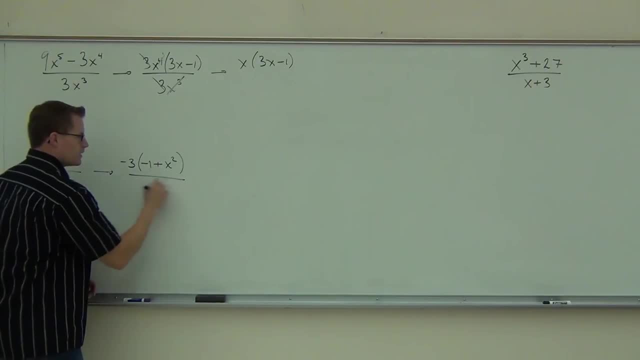 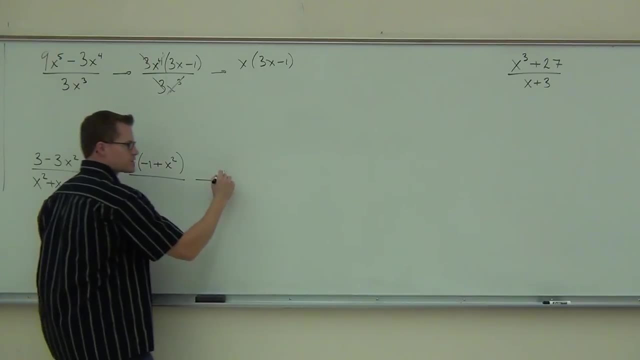 Not a negative 3.. Okay, Let's leave the denominator alone for a second. Let's work just on the numerator for now. I want to make sure we get this all the way down, So the negative 3 is going to stay there, but I am going to switch these things around. 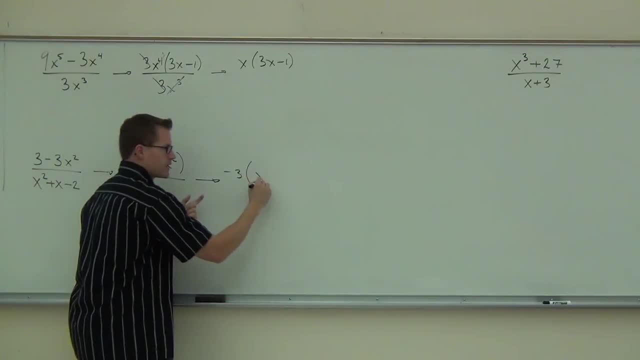 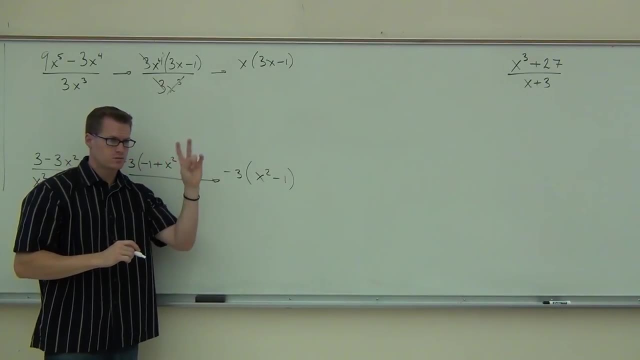 Instead of negative 1 plus x squared, I can write this as x squared minus 1.. Are you okay with that? Yeah, It's just the commutativity of. It's just the commutativity of these two terms. We can do that if we keep the signs with those terms. 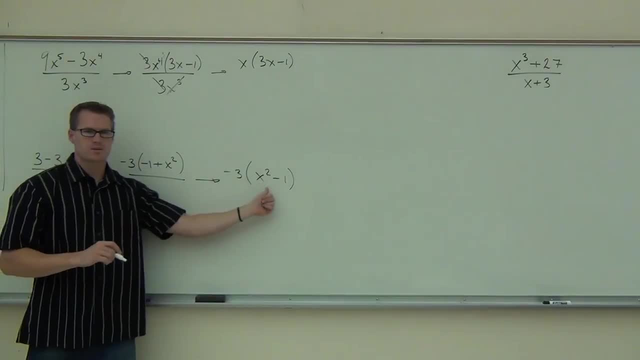 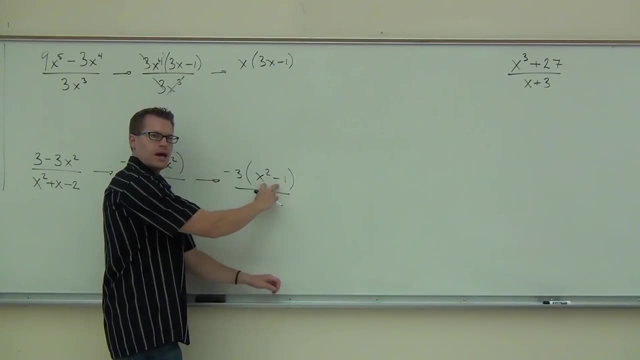 So the negative 1 has to be a minus 1.. The plus x squared, that's a positive x squared. You still okay? Okay, What is this Difference of squares? How is it a difference of squares? It's a 1 minus 1 squared, so 1.. 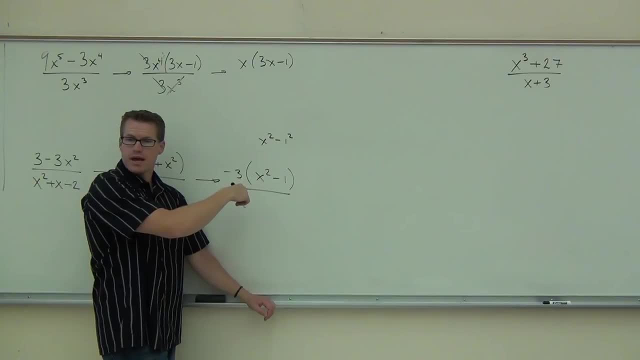 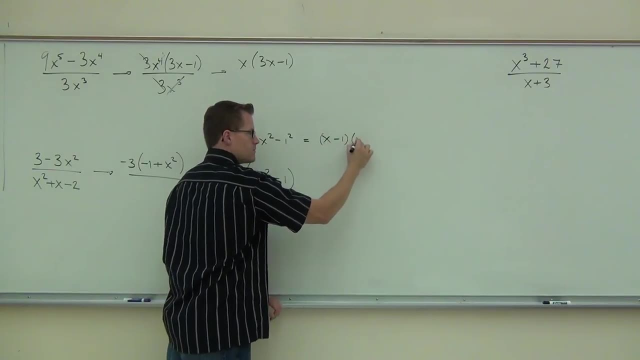 x squared minus 1 squared. That's the same thing, isn't it? So if we factor that this is certainly a difference of squares, This is going to be x minus 1, x plus 1.. x minus 1, x plus 1.. 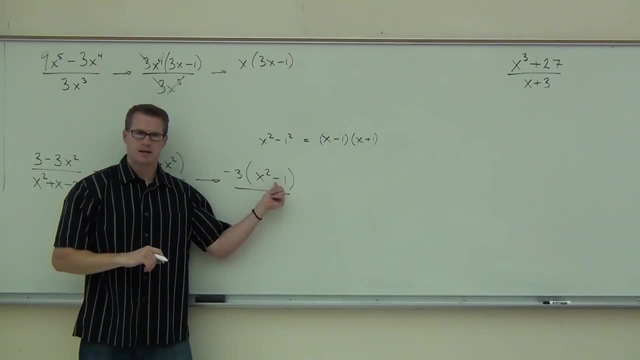 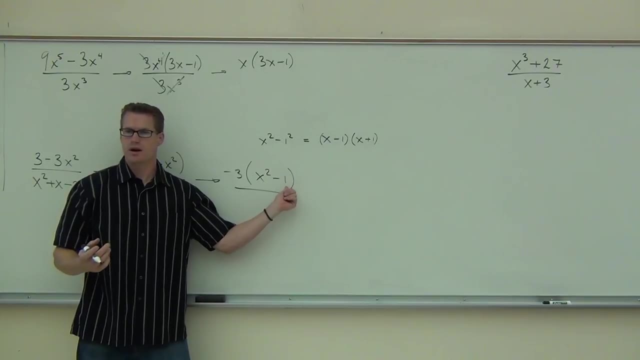 The way you can see it, it has two terms. There's a minus, This is something squared, and this can be written as something squared- 1 squared. That's trivial, but you can write it as 1 squared. If you can do that, you can factor it. 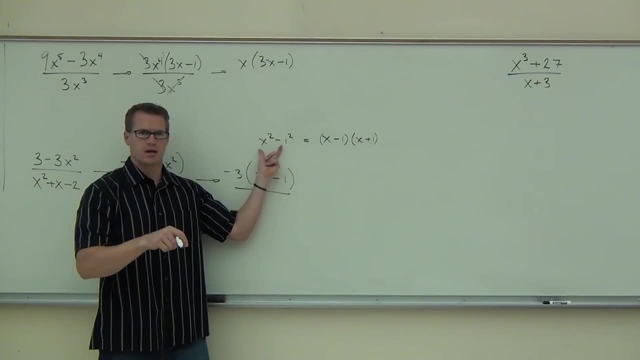 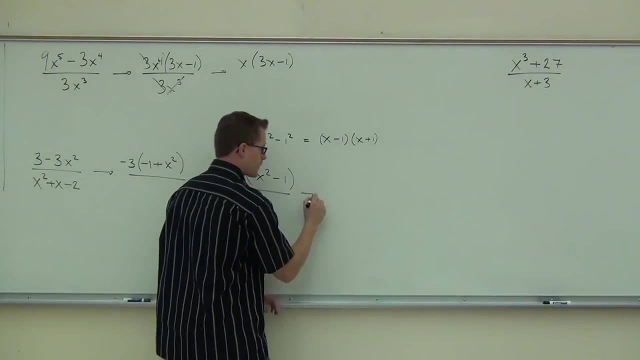 The way you factor it, it was the a squared minus b squared. Look that up on lecture C.4 if you want. Actually it's under C.1, on the lessons, and we do this a couple times in there, So we're not going to forget about this negative 3.. 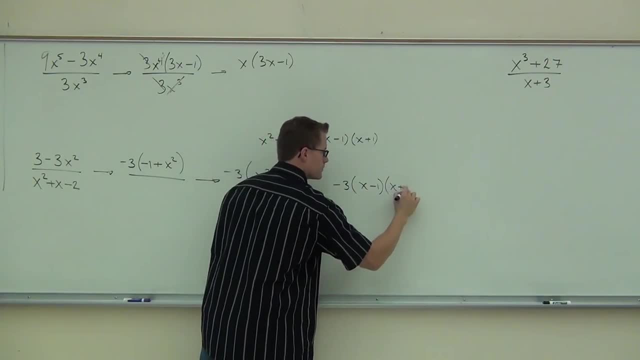 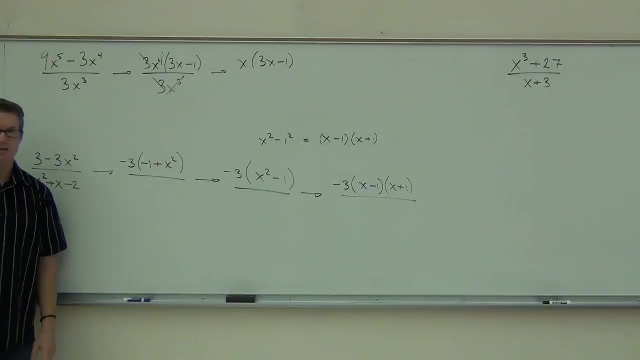 We have factored this And we're completely factoring the numerator. That's what we want to see Now. can you raise your hand and feel okay about getting there? If not, are there questions that you have on this stuff? Do you see why we're doing this? 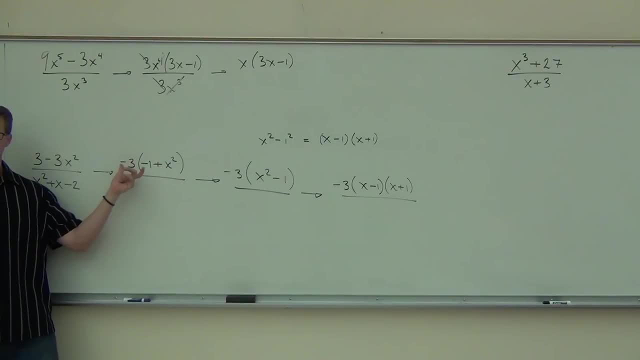 Do you see why we're factoring out a negative? 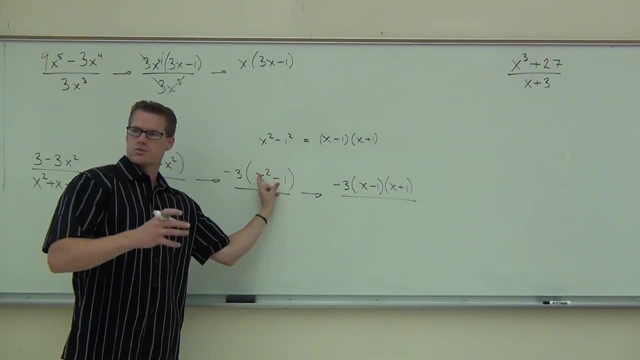 We want to write that in the correct order. We want to write the x-squared first. That way we can factor it easier, Because when you see this, that eventually will be easy for you to factor. 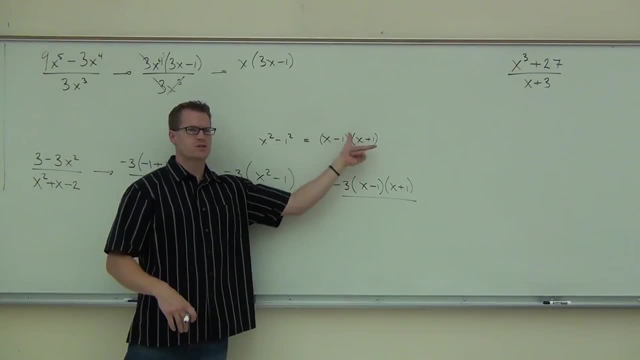 You'll go: oh yeah, it's x-minus 1, x-plus 1.. No big deal, You won't even have to do this stuff, It'll be in your head. We do this, we're completely factored on top. 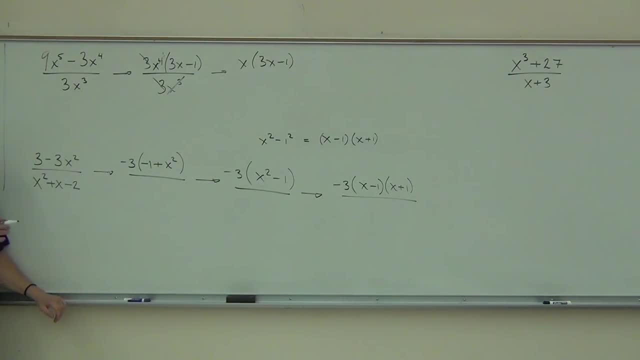 On the denominator. we have a basic diamond problem. You're not going to have an extra step. There's no number out front. We've got 1 and negative 2.. The two numbers that I'm thinking of are 2 and 1, somehow. 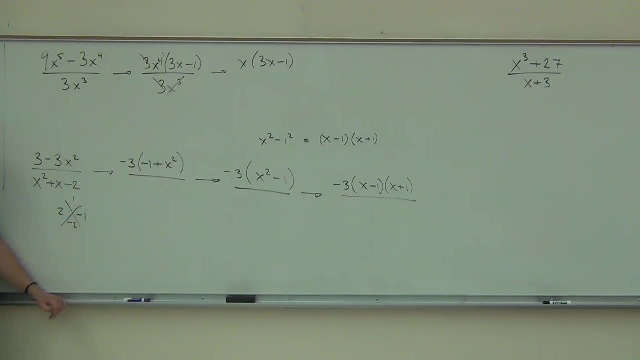 Did you find 2 and 1 somehow, Like that, probably, Or switch around? It really doesn't matter. So we'll go directly to the factors. We don't need to factor by grouping, because there's no term out front, There's no coefficient out front. 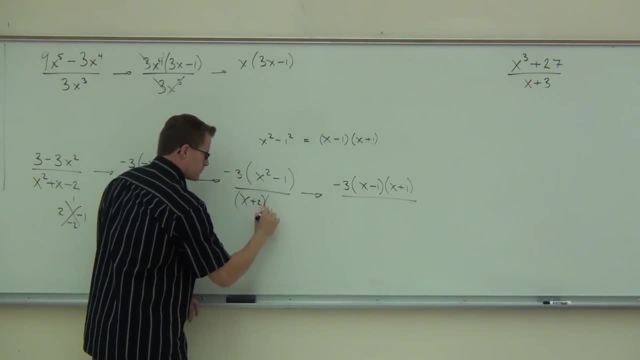 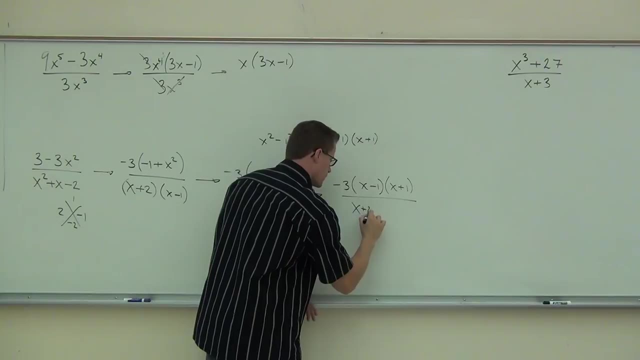 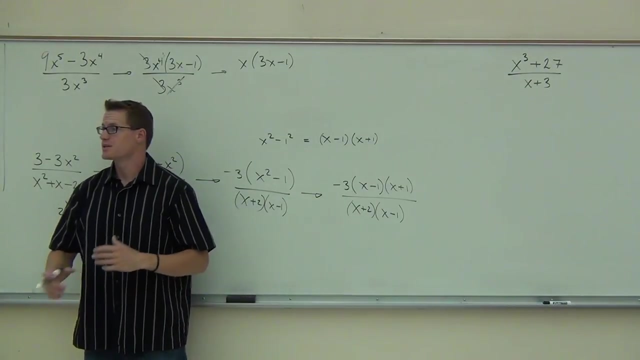 We continue on, So we'll just keep writing that until we get down to the part where both of them are a complete factor. So we just carried this one all the way through. Now, is there anything that we can simplify out of that? 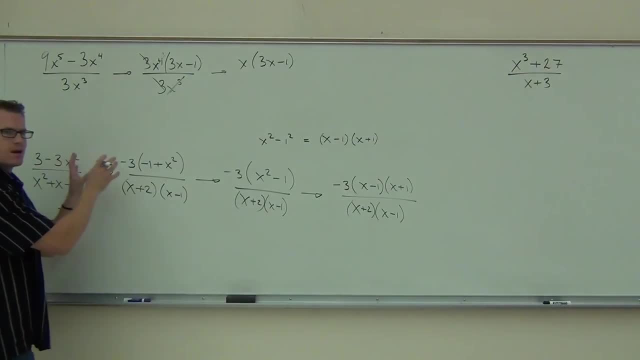 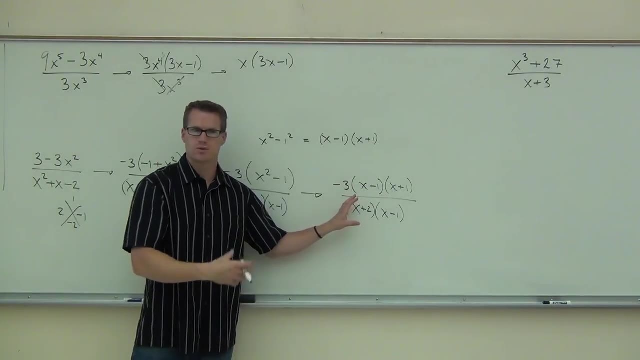 And you know what, If you hadn't factored out this negative 3, you probably wouldn't see it immediately And you'd have to factor out a negative 1 anyway. Did you guys get the picture on that? You'd have to do it anyway. 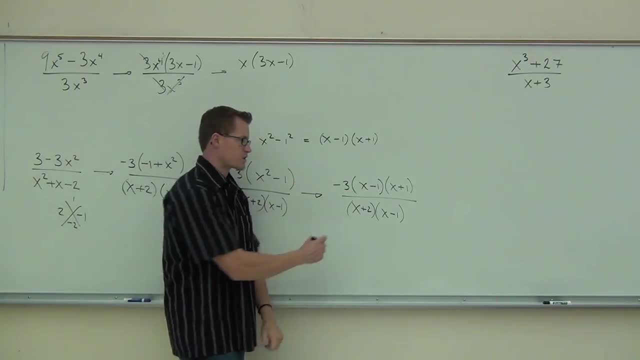 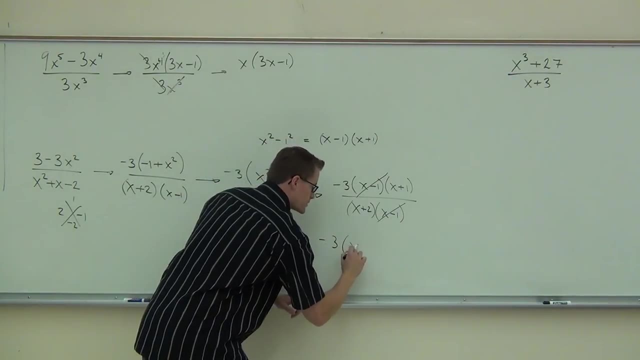 So you may as well do it at the beginning, because it makes things a whole lot easier. So we're going to simplify out this negative 1. We'll rewrite exactly what we have left: Negative 3 times x plus 1. You don't have to distribute. 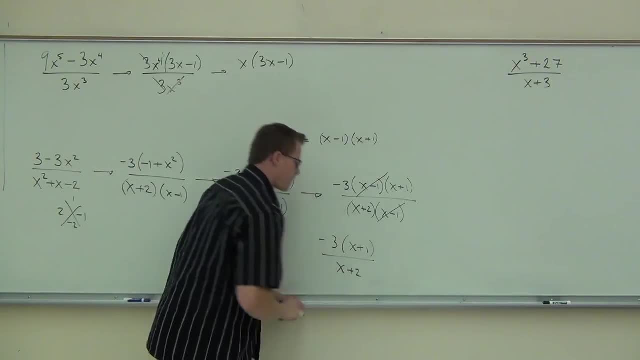 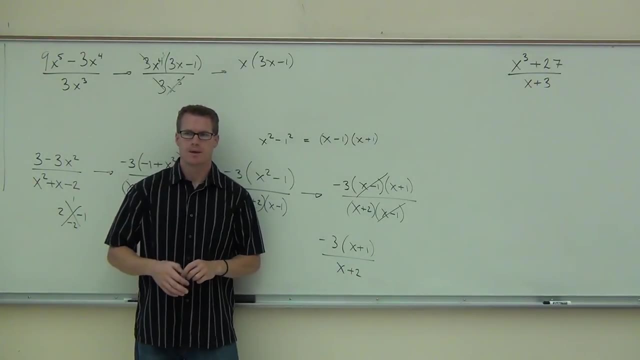 Just leave it. Leave it factored, And then x plus 2. And you're done. That's as far as you can go. We can't simplify any x's or anything like that. We're done. Would you raise your hand if you're okay on these two problems. 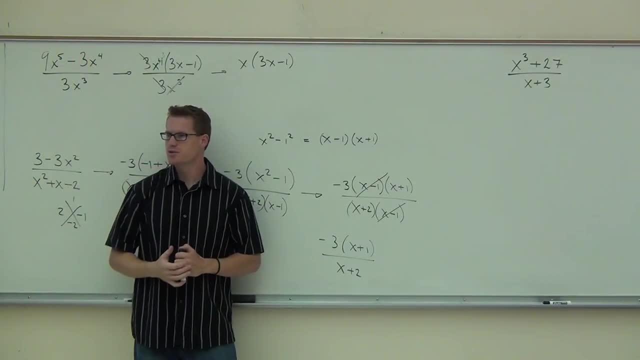 If you don't, if you're still a little worried, you're like, oh my gosh, come and see me or something. I'll walk through this with you. I'm in the math lab or the office. You can always come by and see me. 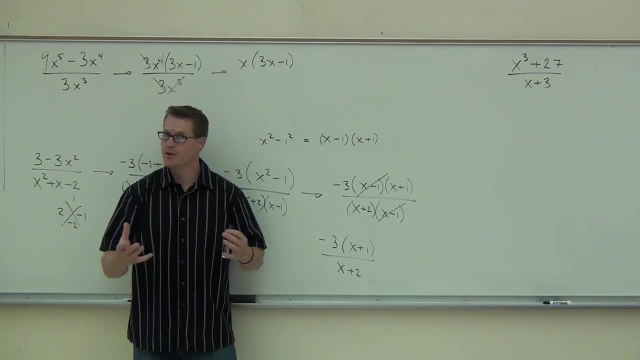 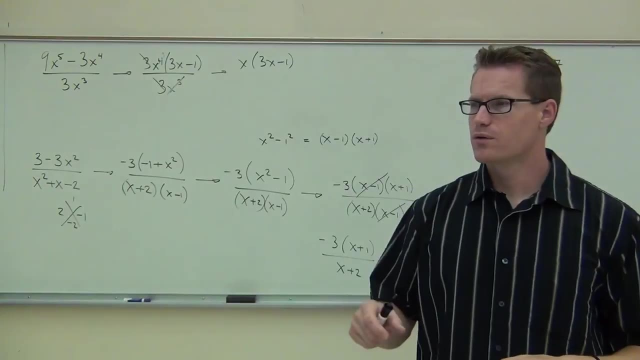 I haven't had very many people do that yet, But I'm there, I'm available to you if you need that resource. Okay, now this one's kind of an interesting one, because what I told you is I'm not going to go over a sum of cubes. 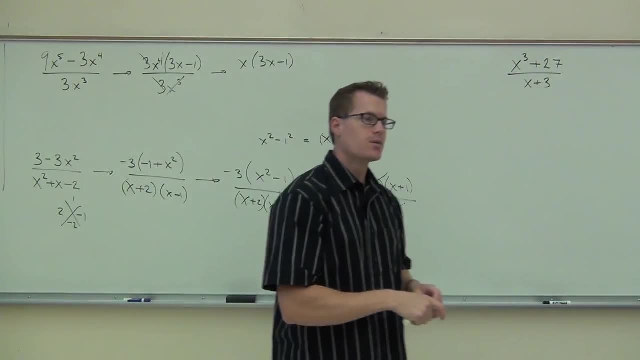 or a difference of cubes in class. I want you to look at it. I hope that you did, because we're going to do this one right now. And guess what? That's two terms, right? That's not a difference of squares. 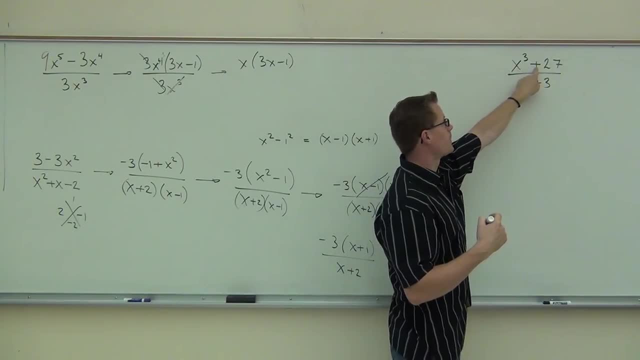 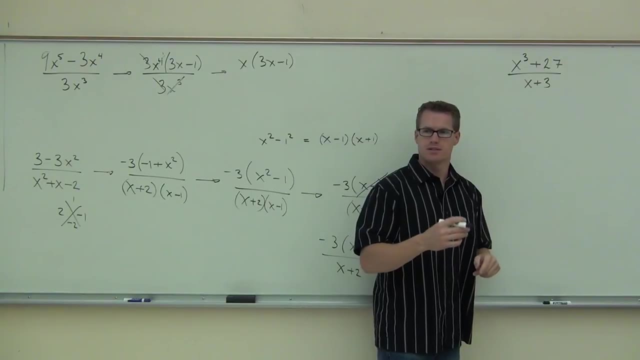 It's not going to factor the same way. This is actually a sum of cubes. That's a cube. Can this be written as a cube? Yeah, Here's how you deal with a difference or a sum of cubes. If you have something written as: 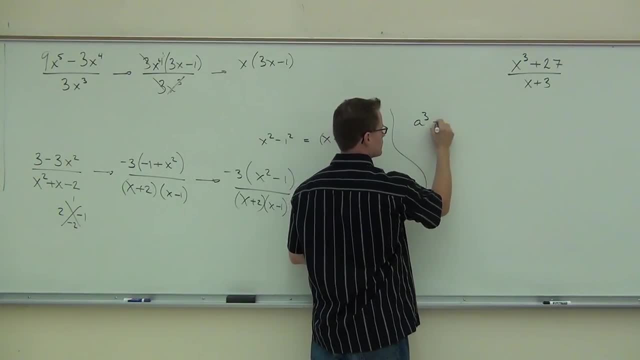 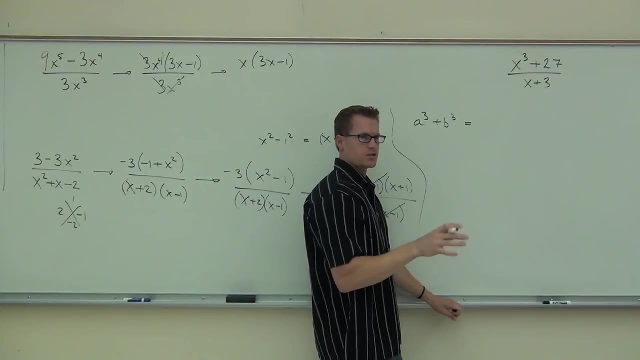 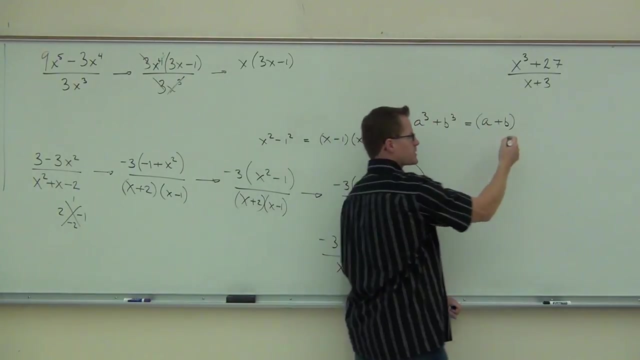 A cube plus B cube. I've given this to you in class. You don't need to rewrite it, It's in your notes somewhere. You write this as A plus B, Remember: the same sign, different sign, thing, Same sign. The next part is: 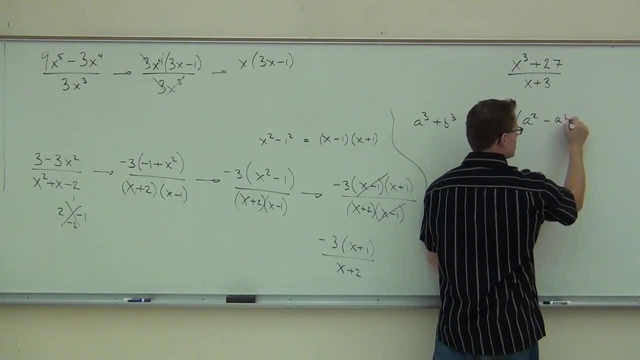 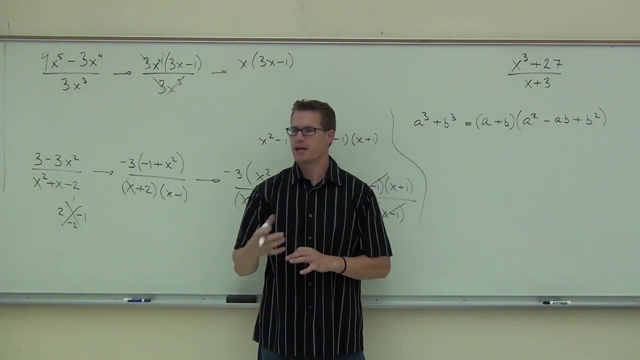 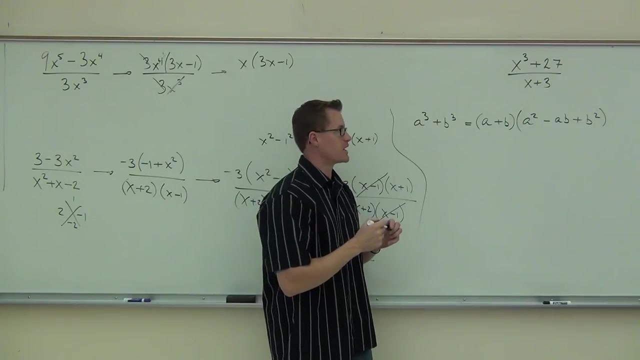 A squared. different sign: minus AB, plus B squared. So essentially, all you have to do is figure out what A and B are, then fill in this formula. It's a formula for you. Let's see if we can practice this on this example up here. 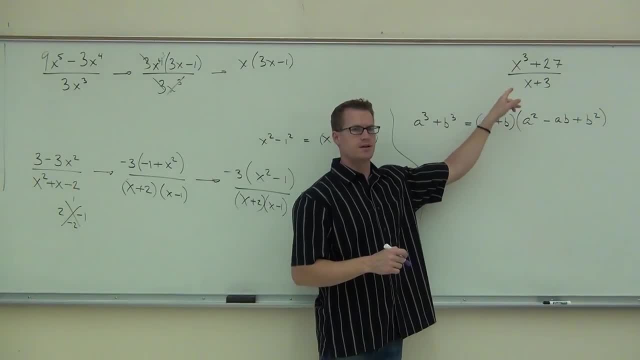 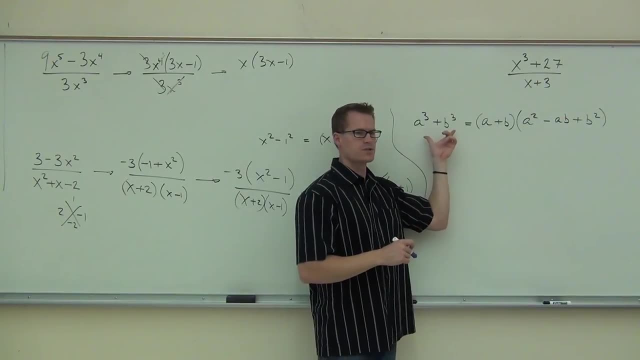 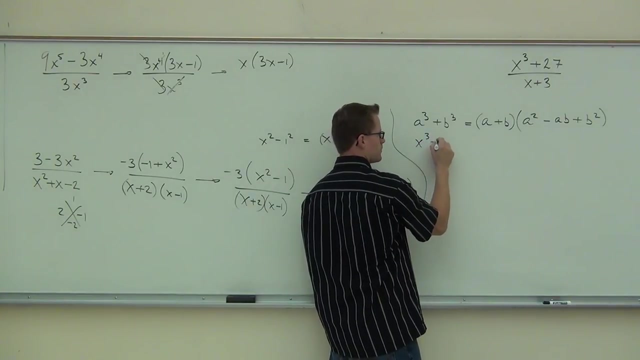 Instead of X cubed plus 27,. instead of X cubed plus 27,. can you tell me again how I can write that As this form: Something cubed plus something cubed. So the X cubed stays the same: 3 cubed instead of 27.. 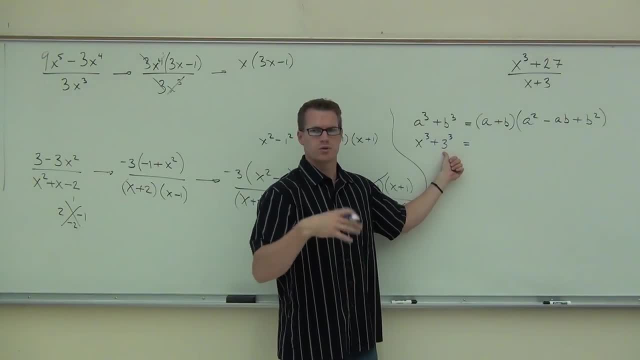 Do you see how this is 27?? It's not 9, right? We don't just multiply those things. It's 3 times 3 times 3.. That gives us 27.. You with me so far. So you see how this fits in this formula, right? 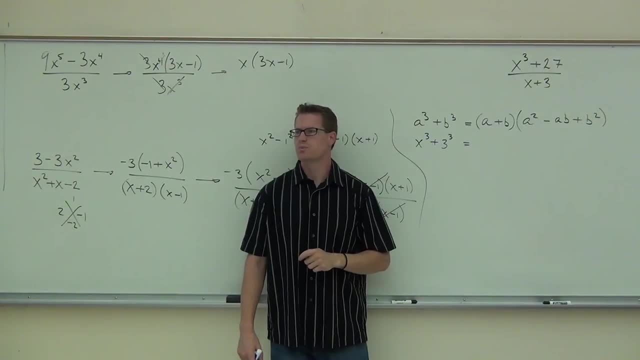 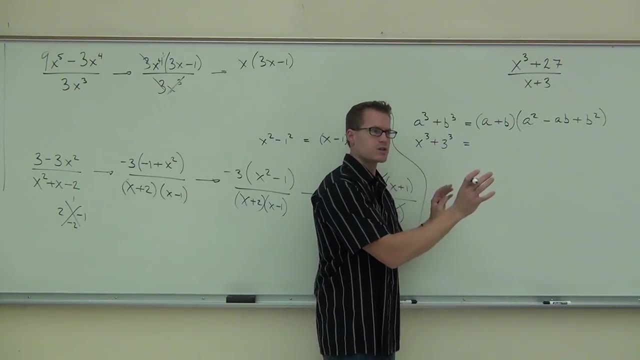 Okay, What's our A in RQ? What's our B in our case? What's our B in our case? Let's fill that out. All you have to do is replace A with X and B with 3. And it'll work itself out. 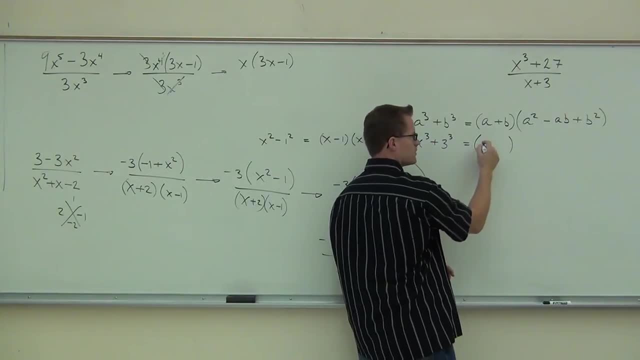 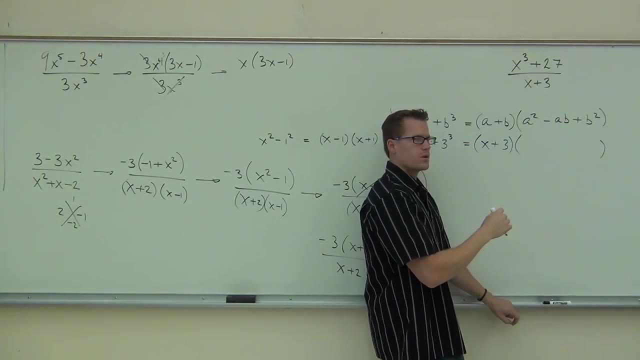 Watch, I'm sorry. what was A again Plus what was B. Now the next part. we're going to fill this out. What was A again? So we're going to put X squared. You see what's squared, right. 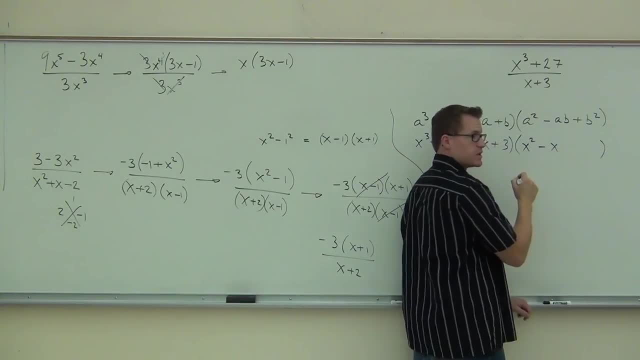 Minus what was A, again What was B, 3 times 3.. We're going to rewrite this in just a second. We don't write X3, do we? No, We write 3X. That's not a problem, though. 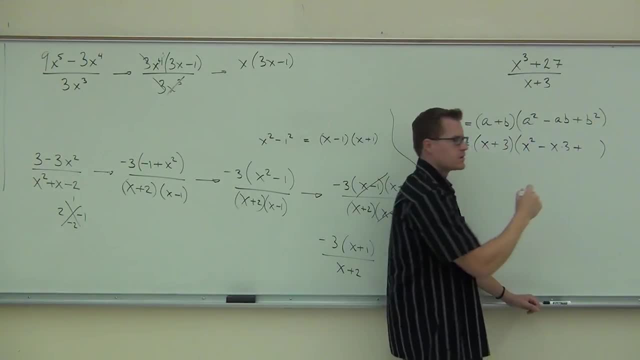 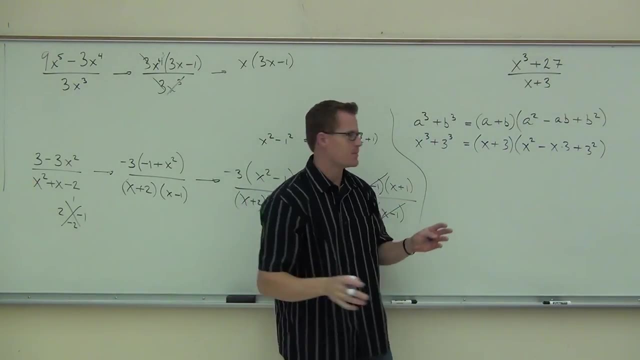 Plus B squared. B squared, How much is B again 3.. So we're going to write 3 squared. That's how you use the sum of cubes idea. The difference of cubes is exactly the same, It's just. this becomes a minus. yeah, a minus, a plus. 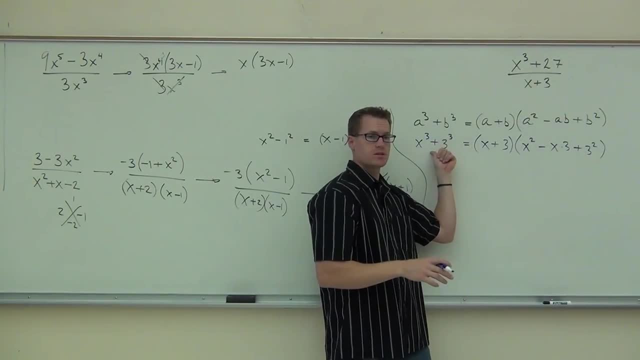 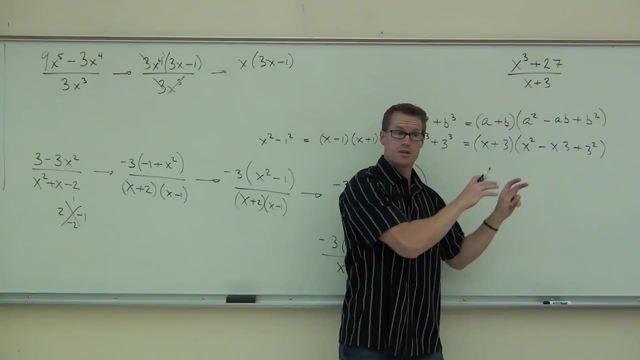 and a plus for a difference of cubes, The sum of cubes, that's with this plus. If this was a minus, these two signs would switch. That's the only difference there. So hopefully you can draw some conclusions from this example for that. 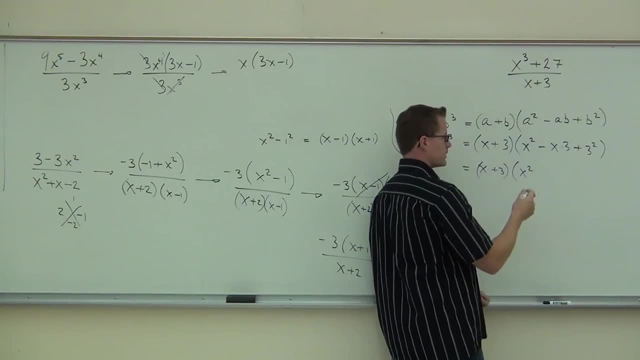 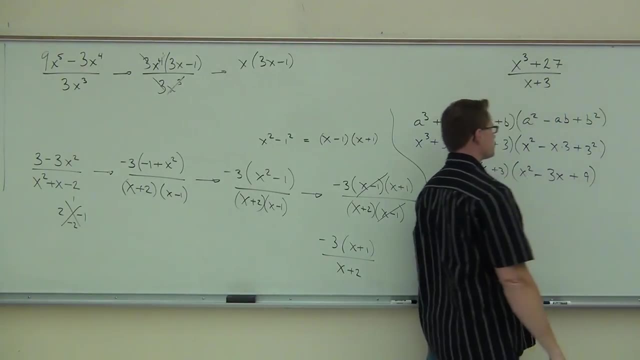 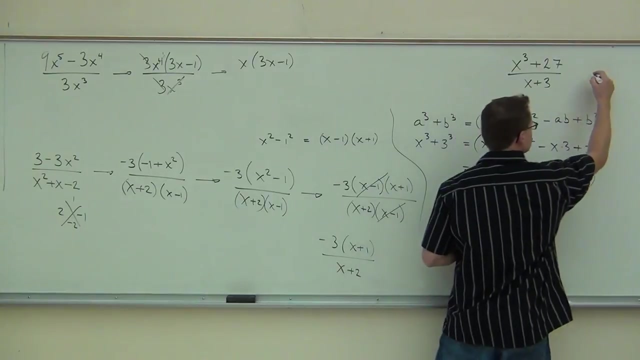 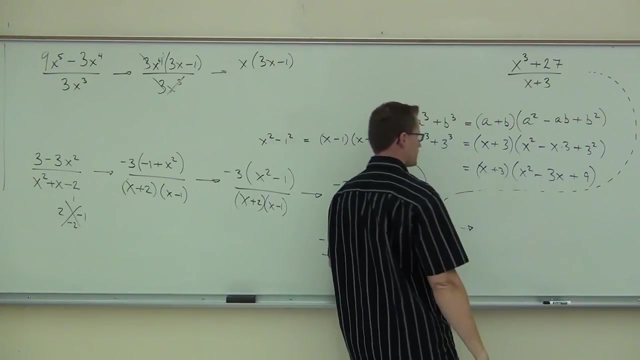 So X plus 3, that's done. X squared well, that's done. We're going to rewrite this a little bit. We're going to do 3X and at the very end we're going to do So. we have just completely factored the numerator. 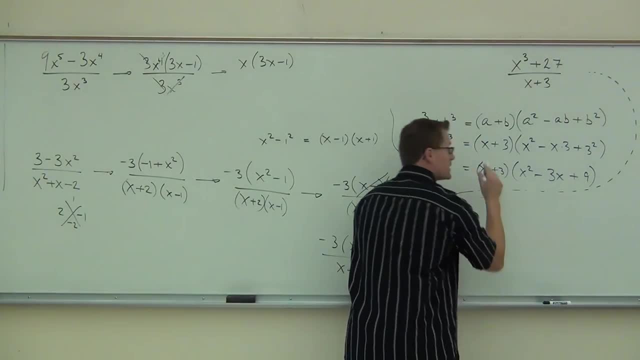 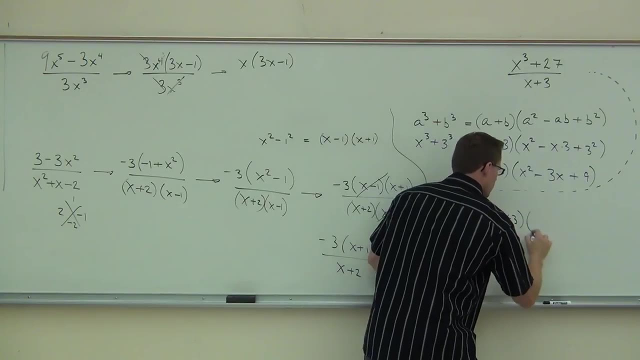 Can't go any further on this thing. We're going to have, instead of X cubed plus 27,. this sum of cubes worked for us. We're going to have X plus 3, X squared minus 3X plus 9,. 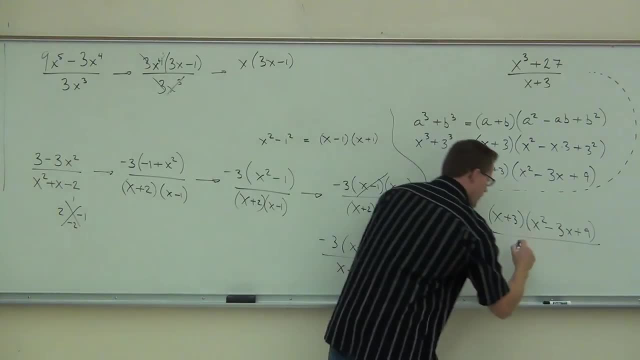 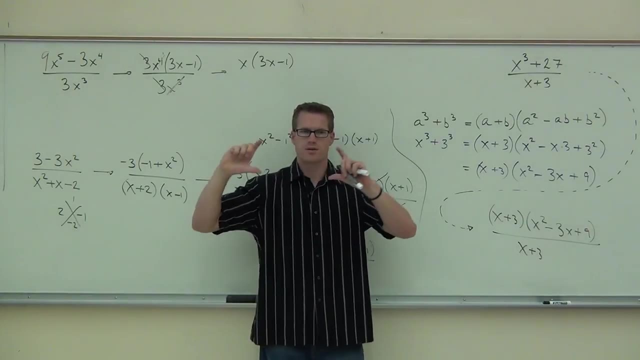 all over. what's the denominator? still X plus 3.. We couldn't simplify that. Does anything simplify? X plus 3.. That's great. We've got two complete factors that are there on the same, on the numerator and denominator. 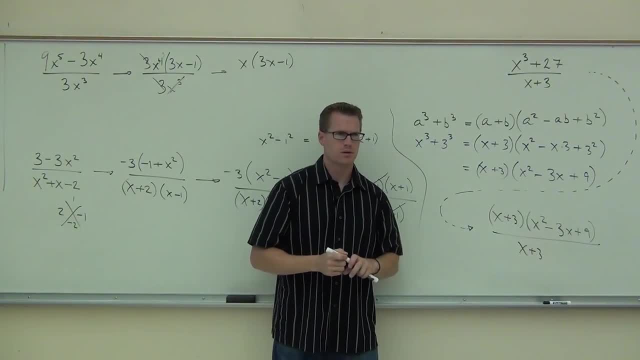 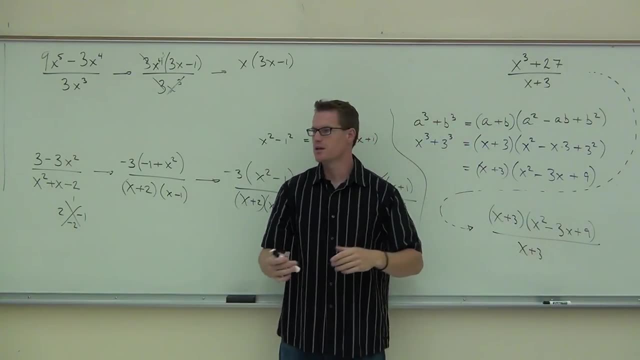 We can simplify out the X plus 3.. Are you with me on this one? Are you sure? Fancy math, right, But it's just a formula. I mean it works Well. I've given this to you before, We just haven't done it in class. 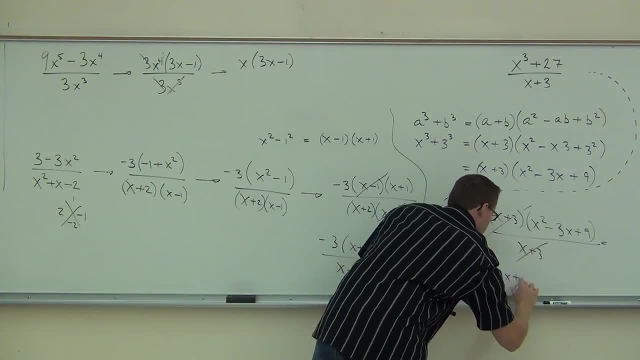 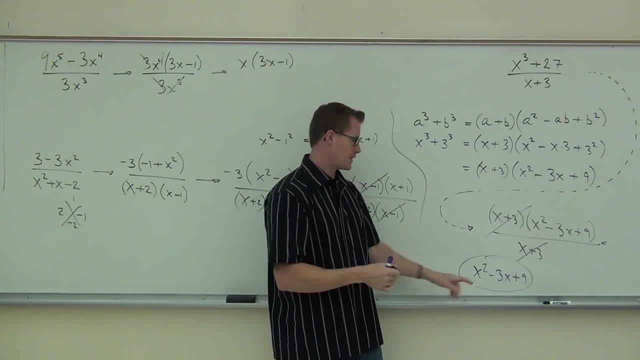 So our answer is X squared minus 3X plus 9.. Of course it's not. Of course that would be over 1, but the 1 doesn't matter, so we're just going to leave it like this: That one. 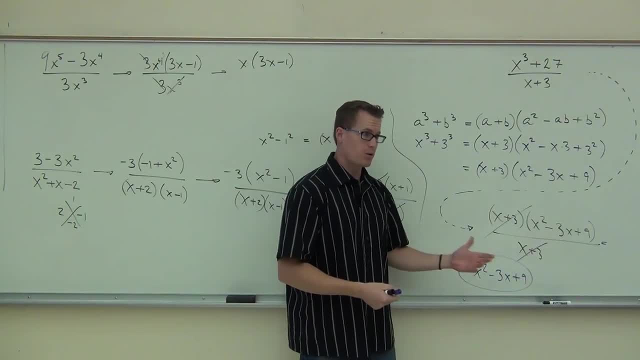 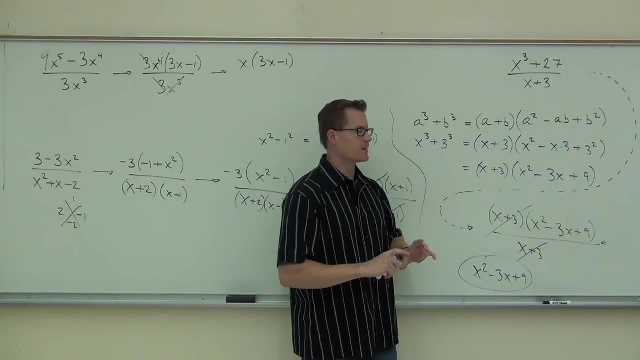 Simplify, you mean like factor it even more. Well, you can try. right, That would be a diamond problem. but what you're thinking of is two numbers that add to negative 3 and multiply to positive 9.. The only things I can think of that multiply to 9 are like 3. 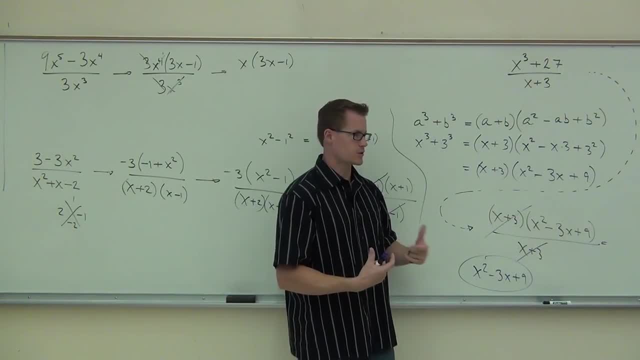 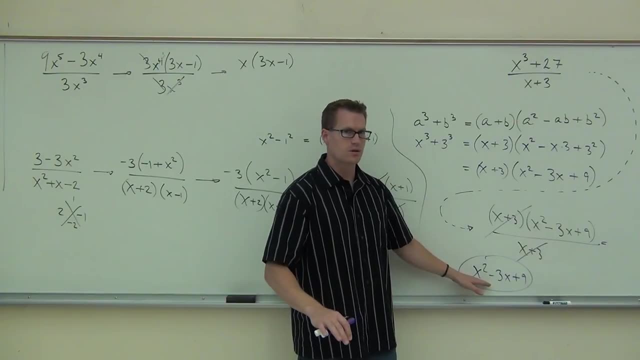 and 3, or 9 and 1, right, And none of those are going to add to negative 3, so you can't factor it anymore. This is one of the three term polynomials that you can't factor. You know, not all of them you can. so some of these things. 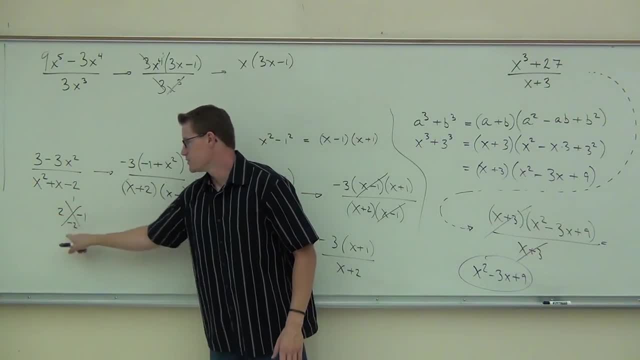 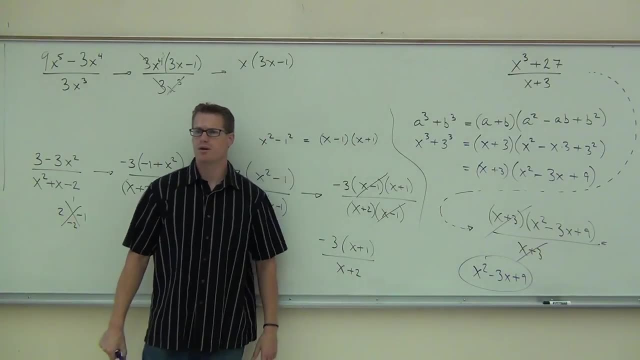 that look like this. you might not be able to factor. It all depends on whether you can find these two numbers. If you can, you can factor it. If you can't, then you can't. That's a good question. Any other questions before we go on? 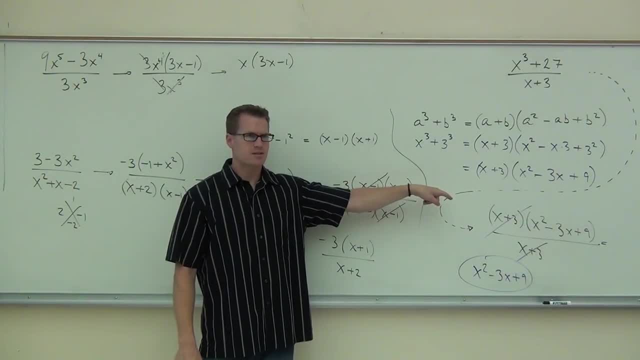 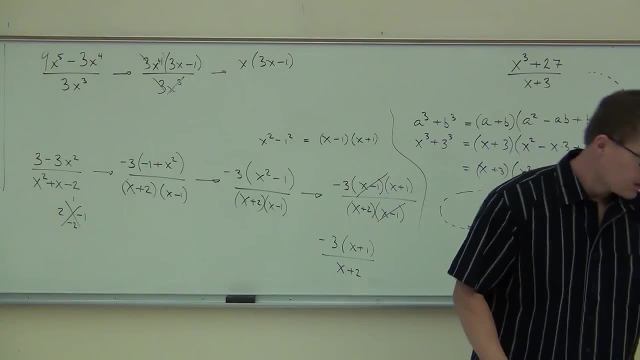 Were you able to follow that one? That's good, That's kind of an advanced stuff. That's the difference of cubes and sum of cubes, stuff That's good for you, Very fantastic. Okay, one more thing in our section, then we'll move. 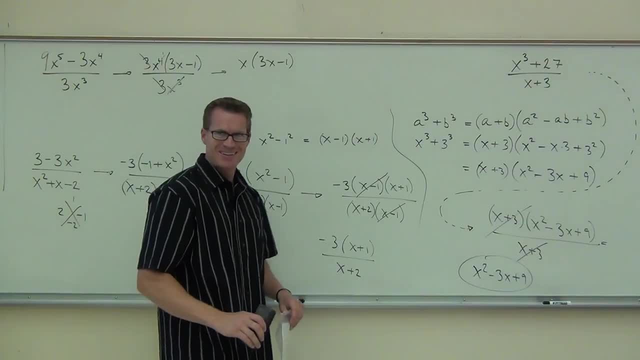 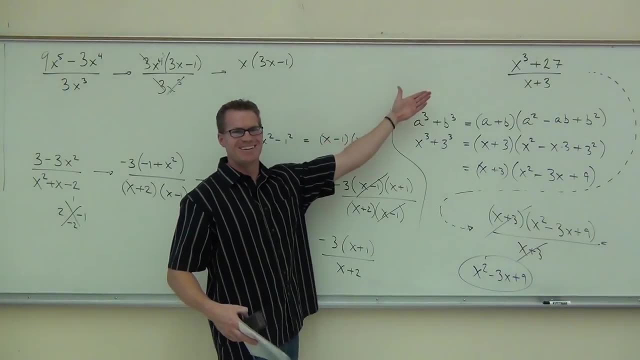 on to 7.2 and have some real fun. Are you ready for this? Are you ready for some real fun? Of course you are. Fun Friday, right? Oh, it's Fraction Friday, See. See, I knew there was something good about today. 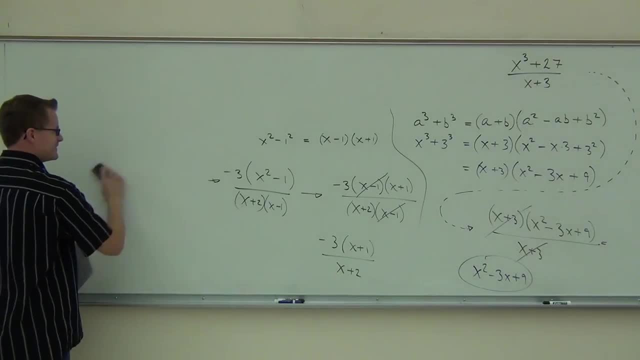 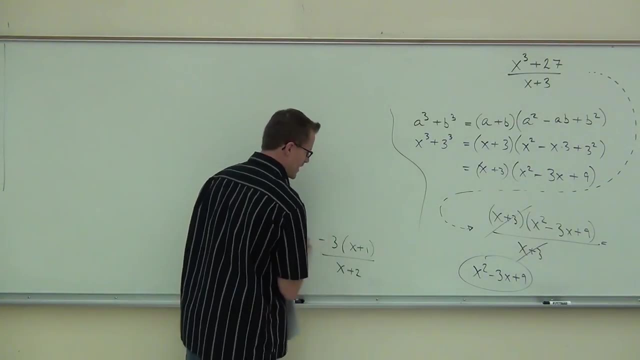 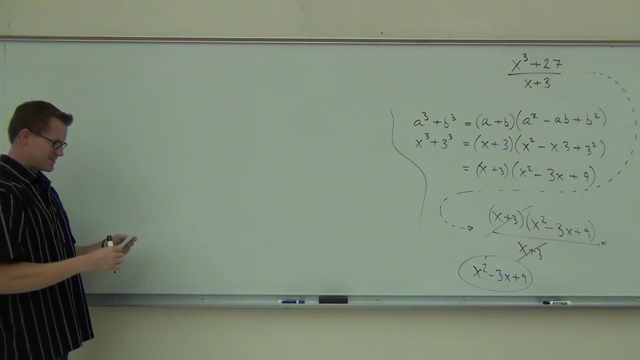 Okay, Some of you are like: I hate you. Not only do you make us do fractions, you make stupid jokes about them. I know You ruin my Fridays. That's what I do to you. Okay, Yeah, you're welcome. 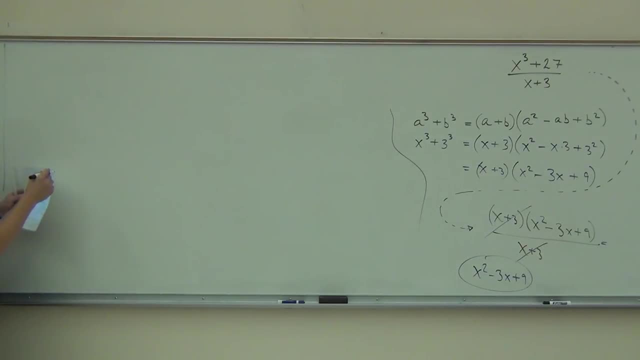 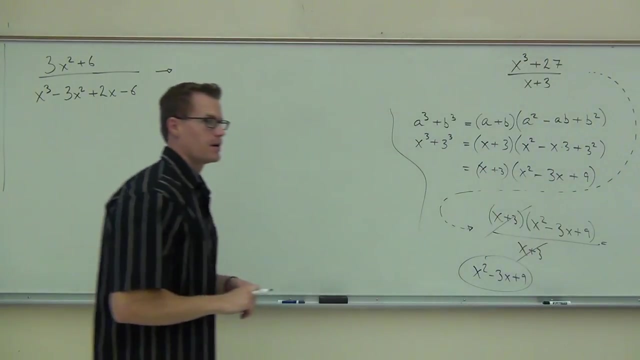 You're welcome. That's all. Last one I want to show you before we move on: 3x squared plus 6, let's do that one over, Let's do this one together. We're going to go through it kind of quickly. 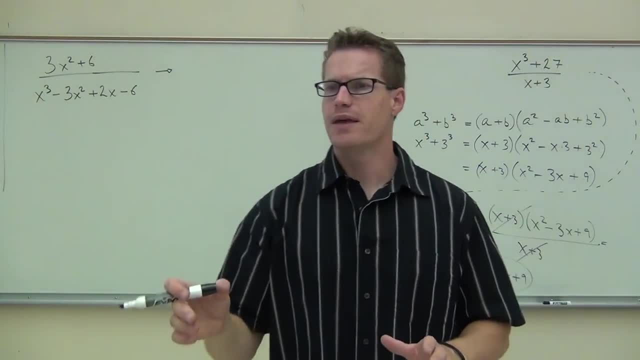 because there's one thing I really want you to see about it. Let's look at the numerator and the denominator. Of course, we're trying to factor this completely. Look at the numerator. What factors out of the numerator, please? Three. 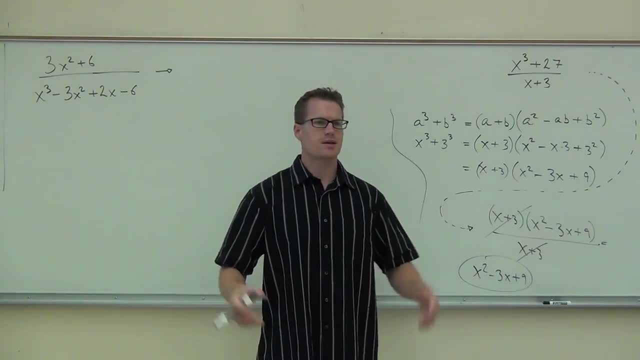 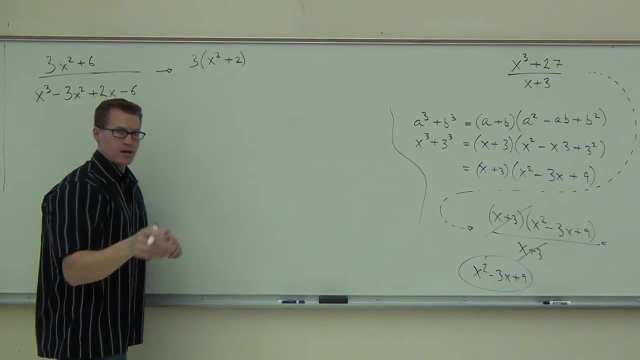 Do I need to factor a negative 3 or not? What do you think? No, That's already positive, Don't worry about that. Factor the 3 out. We get x squared plus 2.. Did you get x squared plus 2?? 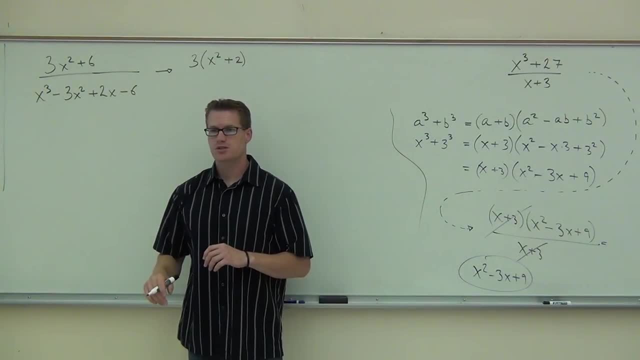 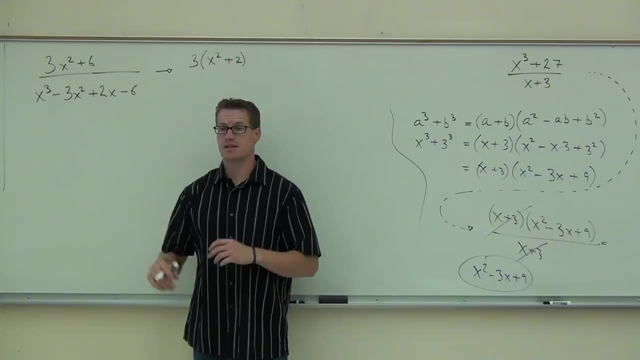 Uh-huh. One question I have for you: Is x squared plus 2? Factorable X squared plus 2?? Absolutely not. No, it's not a difference of squares. It doesn't have a cube, so it doesn't fall. 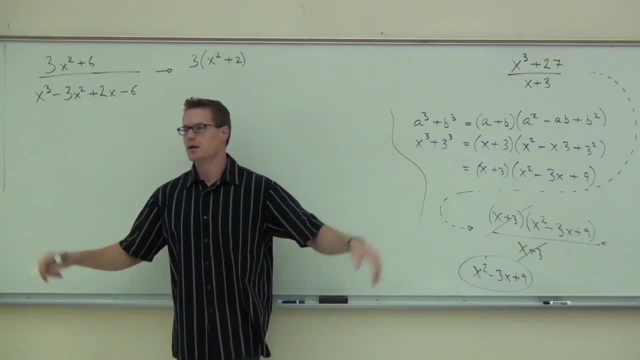 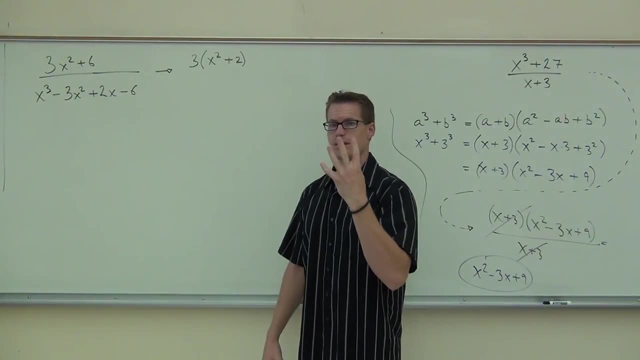 into this category. Are you with me on this? You can't do anything with that. That's done. So we look at the denominator. How many terms are in the denominator? Four? Don't forget what we do with four terms. Say that louder. 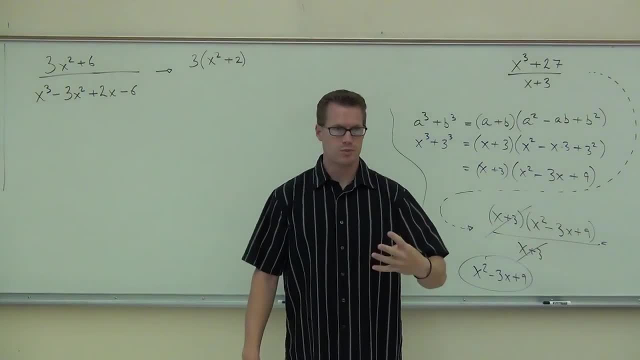 That's the only thing we can do. So in this class, when we have four terms, you are grouping, So that's the only thing we can try is to group this thing. Remember how to group. You don't group. Look at the board. 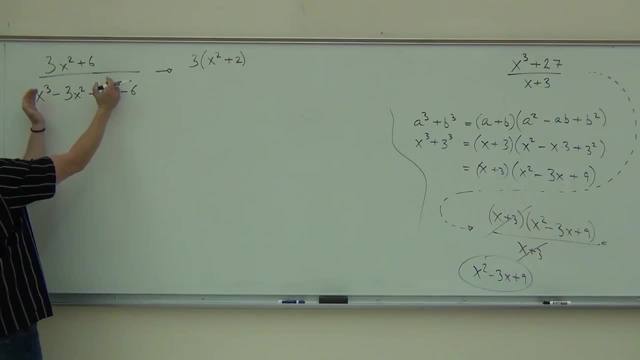 You don't group the first three. You don't do that. What you do is you group the first two and the second two. That's how grouping works. If you group the first three, this thing is going to be left by itself and you're not going to know what to do with that. 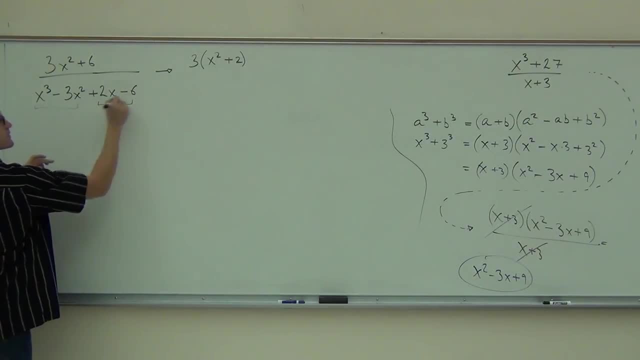 So you factor by grouping the first two and the second two. What factors out of the first two, please? X squared plus squared, And we're going to get x minus 3.. Out of here we have a positive, so we're factoring a positive 2. 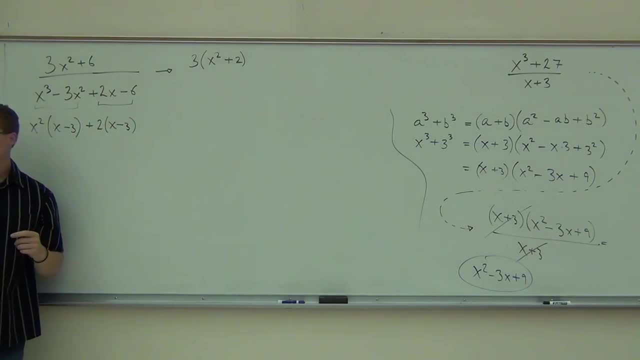 and we get x minus 3.. Does it look like it's going to work for us? Yes, Yeah. If these aren't exactly the same, it's not going to work. But here we've done this a lot now. We use this every time we have an extra step on a trinomial. 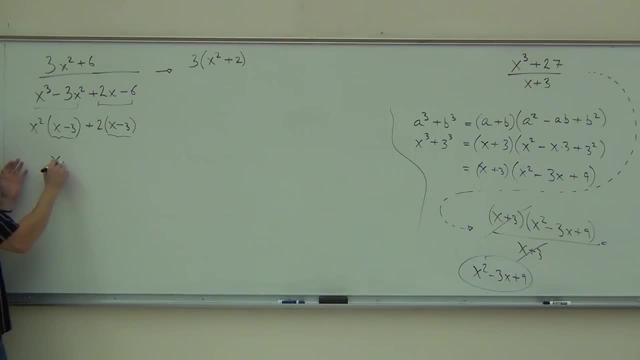 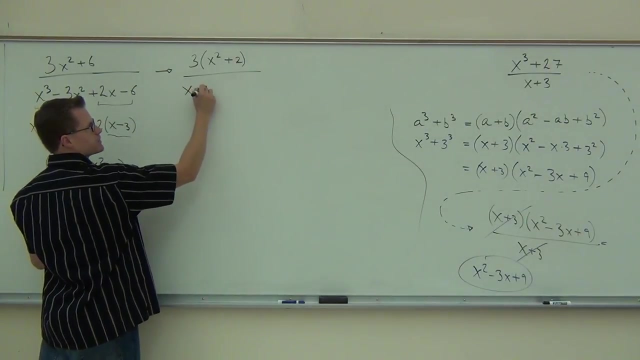 a three-term polynomial, So we're going to factor the x minus 3.. What's left when I factor out the x minus 3? Can you tell me that X squared plus 2. Perfect, So on our denominator we have our x minus 3.. 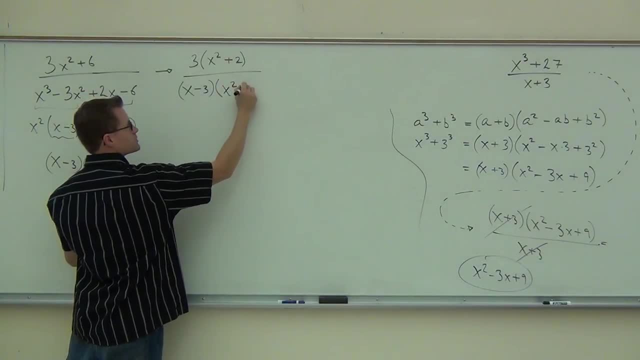 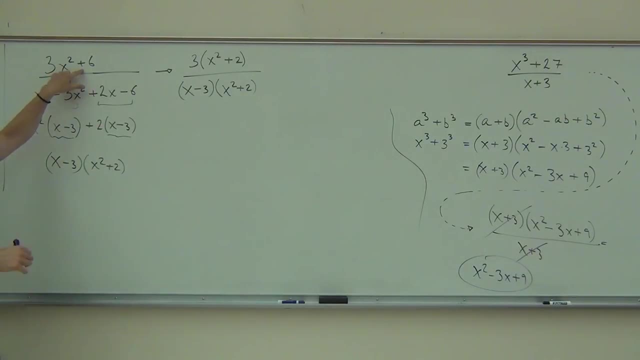 X squared plus 2.. X squared plus 2.. So just a little recap out of the numerator. the only thing we can do is factor a 3 and we're done with the numerator. There's nothing else we can do. On the denominator, whenever you see four terms, the thing you're going. 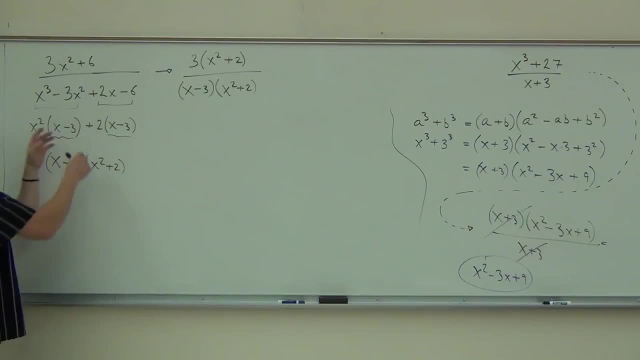 to try to do is factor with grouping. That's it. So. factoring by grouping means the first 2, x squared, comes out of that, No problem. Second, 2, only 2 comes out of that, No problem. When you have exactly the same thing, you factor it out. 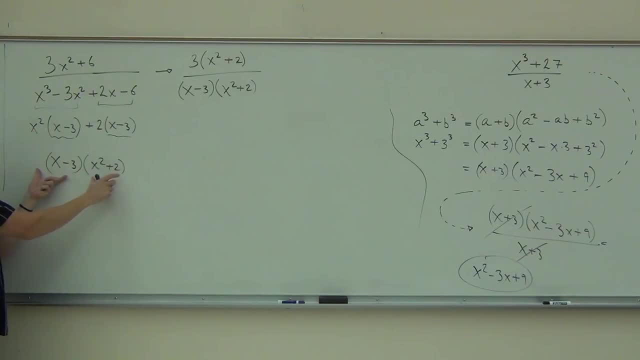 You write what's remaining in your second parenthesis, just like we do with the extra step on the diamond method. That's really the exact same thing we're doing here. The terms look a little different, but it's the same idea And that is our new denominator. 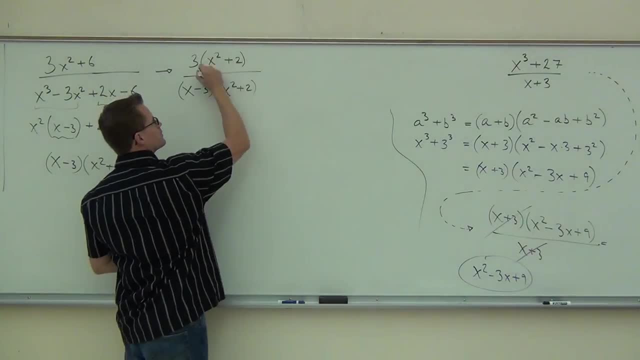 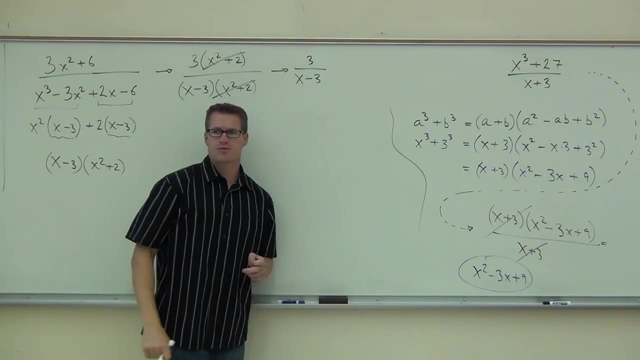 Does anything simplify? Yes, Perfect, We got that. We'll write what's remaining, That's a 3 over x minus 3.. And now the 3 is simplified, right, Yeah, Why am I not right? Because you can't. 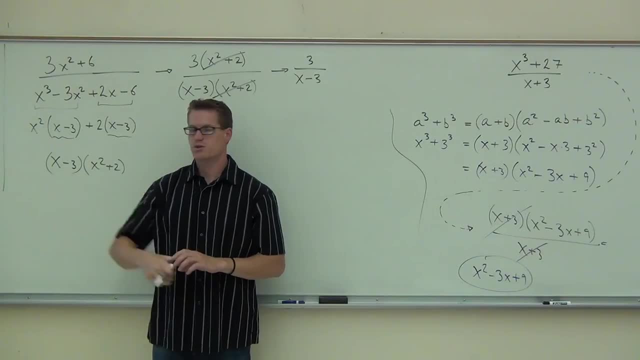 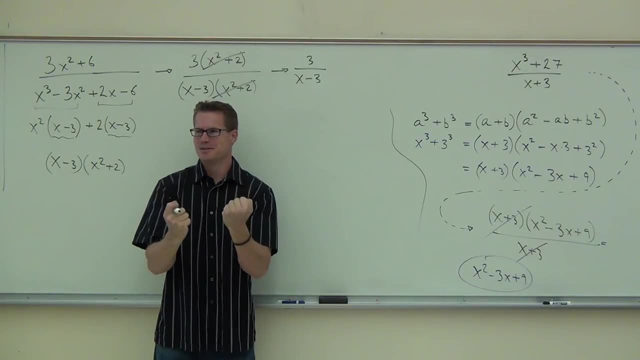 Ah, those are terms. they're not factors, So I cannot simplify those 3's. Are you with me on this? I've got students in calculus who still do that. That makes me so mad Going- oh your paper's- screaming at me. 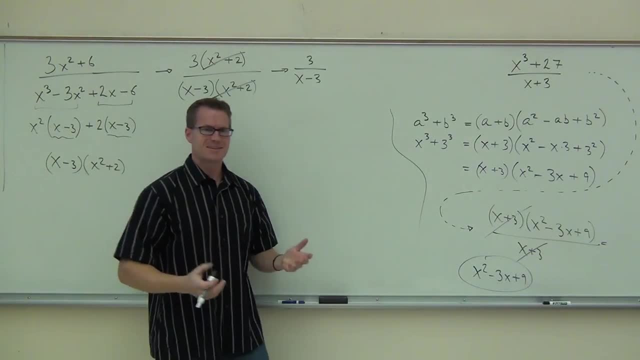 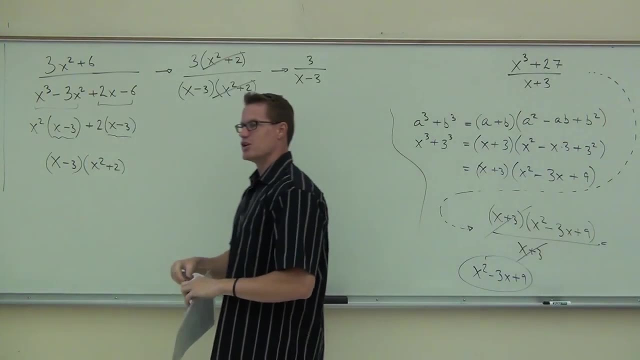 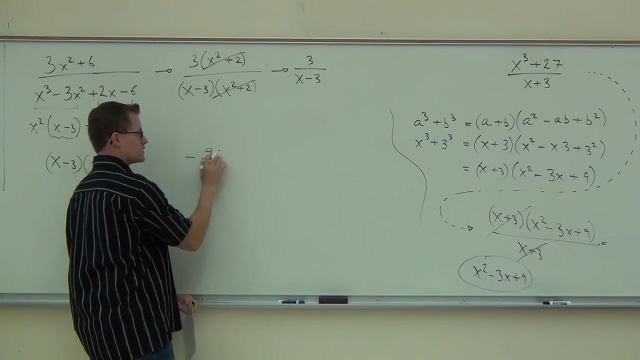 Why are you looking at me? See, It makes me cry a little bit, All right, Oh yeah, there's one more thing I need you to know about fractions. Here's the thing I need you to know: I need you to know that this, it's supposed to be an 8.. 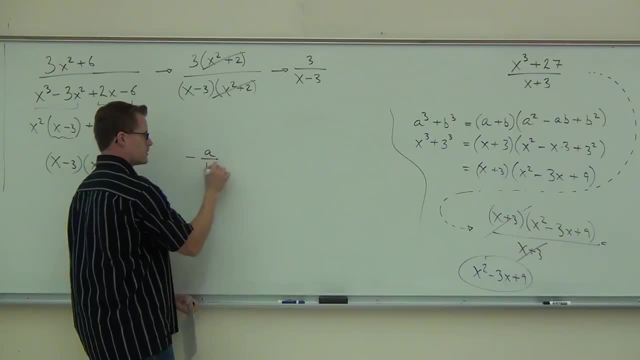 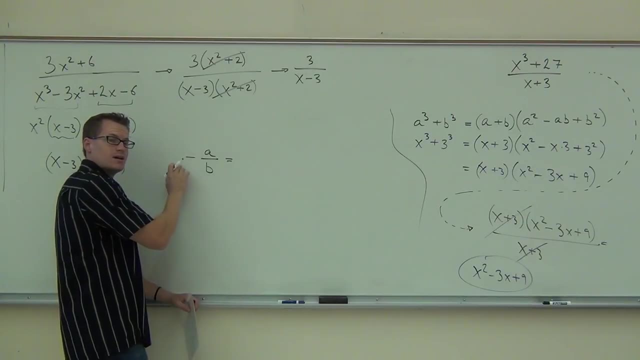 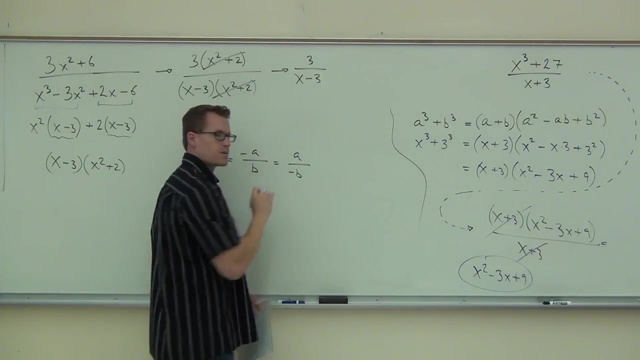 This is the same as wherever you put this negative. it really doesn't matter in a fraction. So you can have a negative out front of a fraction, or on the top of a fraction, or on the bottom of a fraction, and it means exactly the same thing. 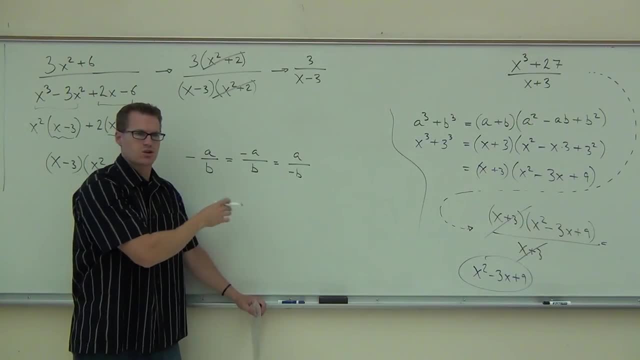 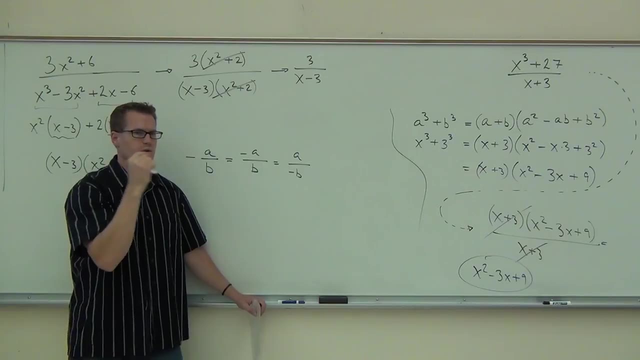 Did you know that already? So there's some equivalent forms of fractions that you're going to be dealing with, And essentially all it's going to ask you to do is move the negative from the middle to the top, to the bottom. Just move it around and see that you can get different-looking fractions that have the same value. 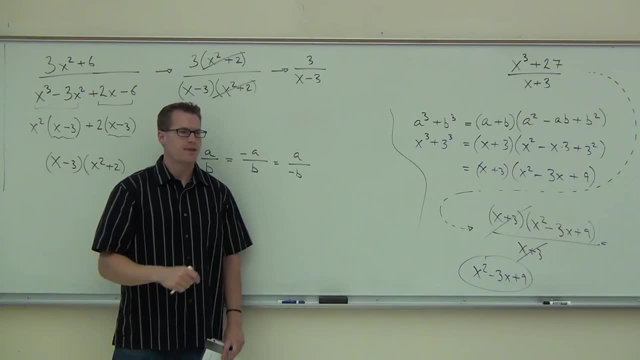 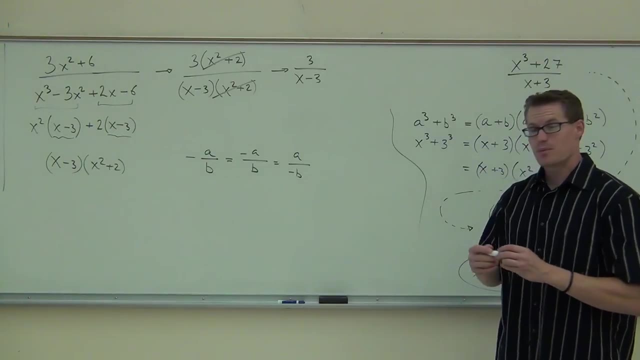 Does that make sense to you? Different-looking fractions that have the same value. That's going to be the little process that you're going to do in the last part of this section. Now, how many people feel comfortable simplifying fractions? We're okay with this. 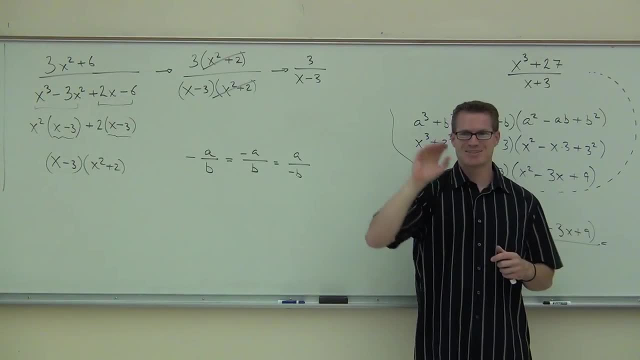 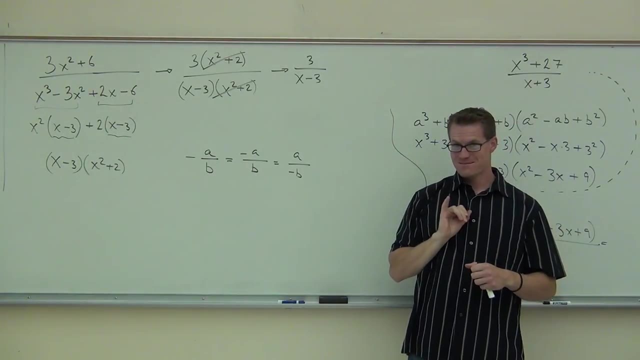 So we're factoring: is that, is that the hand raising? No, I love it, It's so amazing. So we're all going to do this now. So we've done the simplifying fra-. I was just kidding. by the way, you know that.